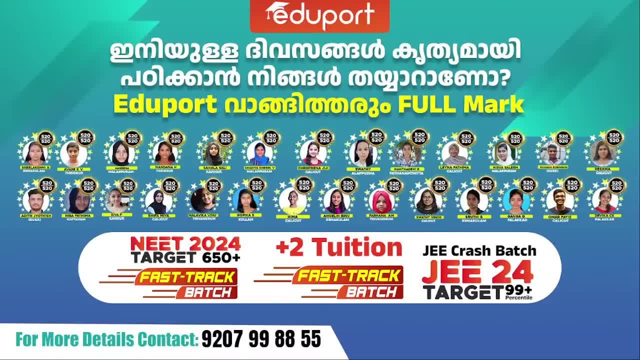 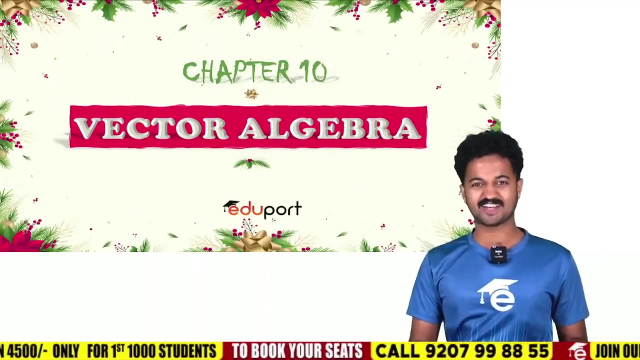 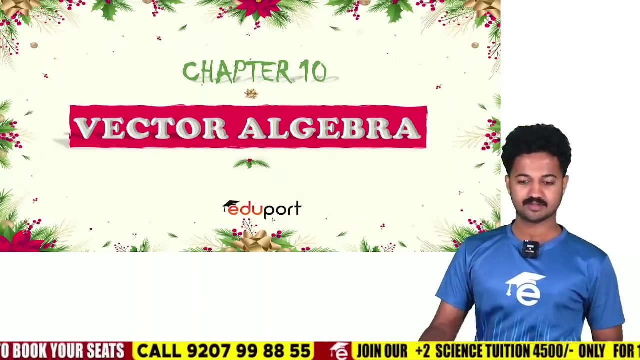 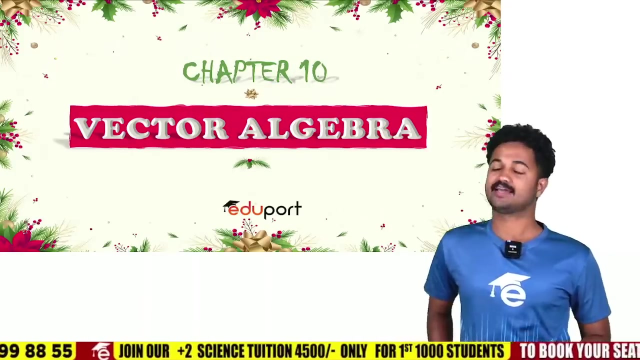 Thank you, Thank you, Good morning, good morning. good morning, Hi, hi, All of you, Hi, all of you Ready. Good morning sir. Good morning, Good morning my dear friends who came to see live in the morning to sleep. Hi, good morning, Is it a set? Is it a set? 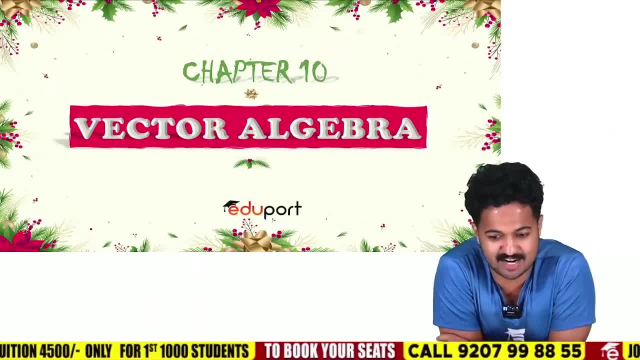 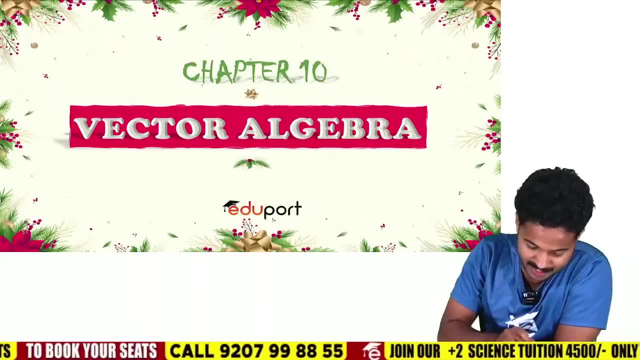 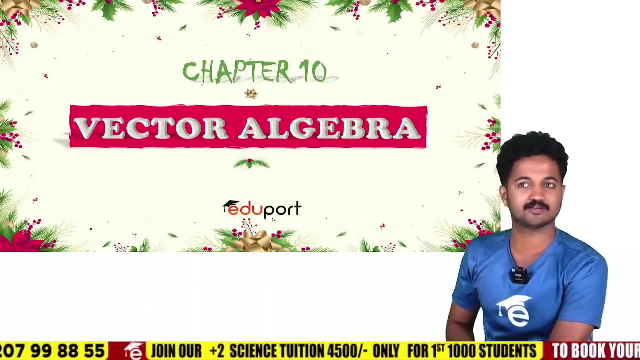 Sharmil sir hi, How are you? Is everything fine? Are you doing well? So we have learned two chapters today: Vector algebra and the same three-dimensional geometry. Both are quite simple chapters You can easily study with algebra. You can study it quickly and score marks. Are you ready? Okay? 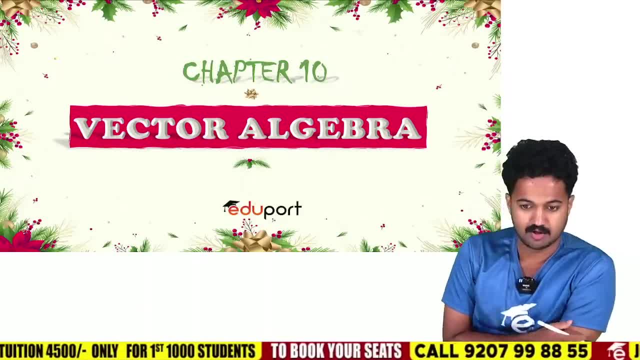 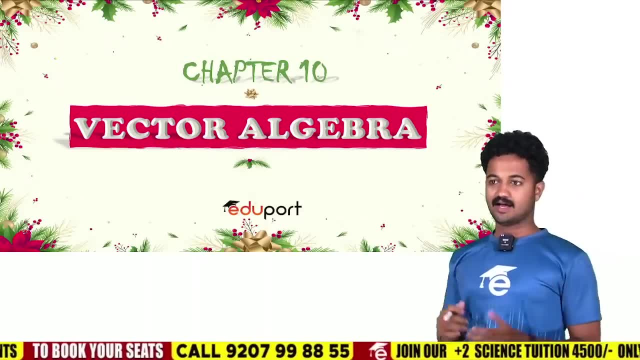 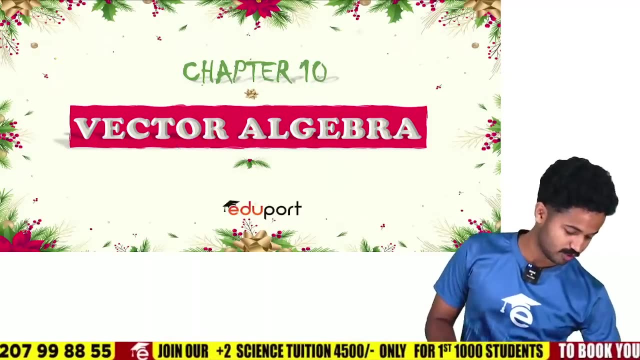 If so, let's start. Okay, there are a few more people coming to the live. Hi sir, Hello sir, Hello sir, Okay, fine, Ready, If so, there is no problem. Great, It is very beautiful and comfortable, So let's start, No problem. 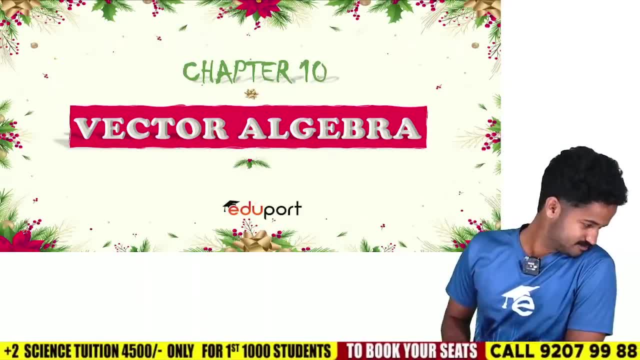 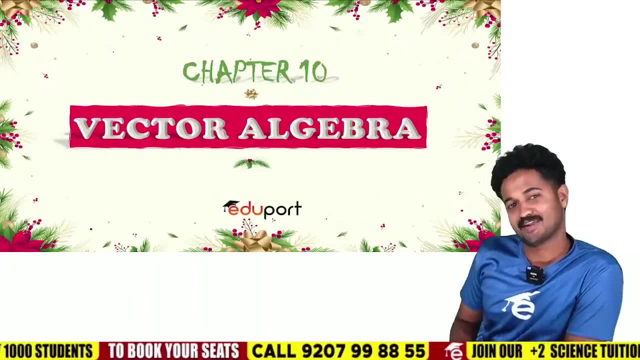 If that's the case, then check it out. Yes, good morning sir. Good morning to everyone. Isn't it an experiment? It's the best experience. Isn't it an experiment? It's the best experience, Isn't it an experiment? 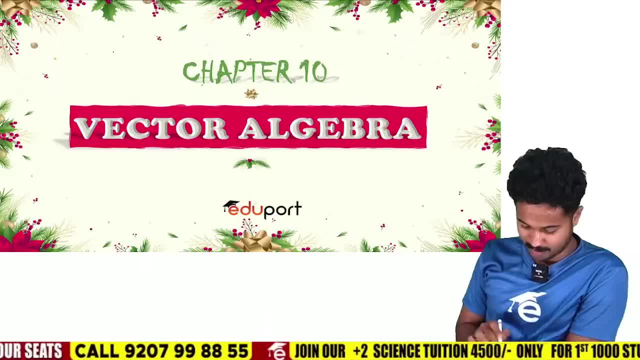 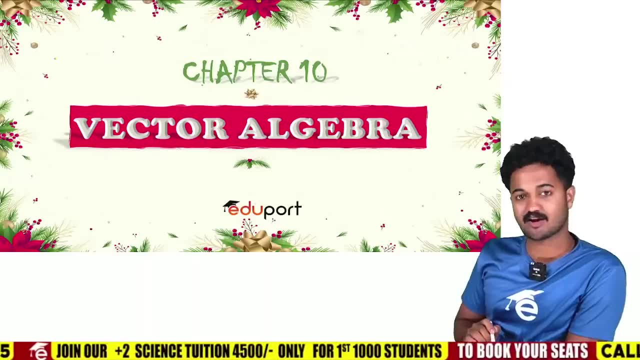 It's the best experience because it's an experiment. It's not an experiment, Don't worry. I think you all are a little scared. So what we are discussing today is the first chapter, number 10,, that is, vector algebra. 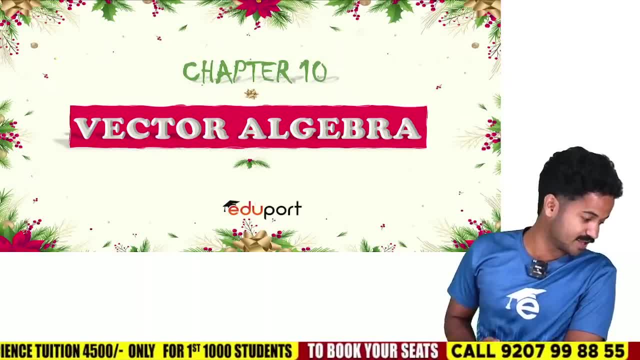 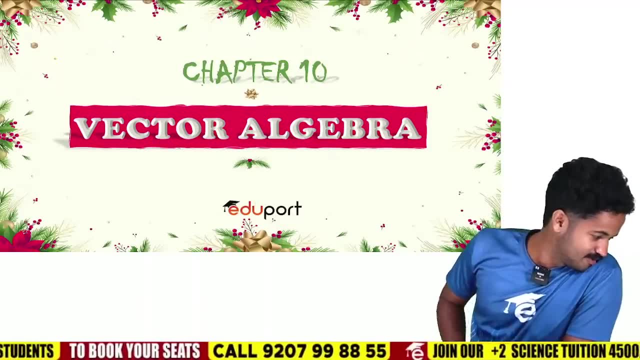 The 10th chapter is vector algebra and the 11th chapter is the same, Which is three-dimensional geometry. I said that both are simple chapters. Okay, So a lot of people are sitting like this for the live? Yes, Hello, sir. 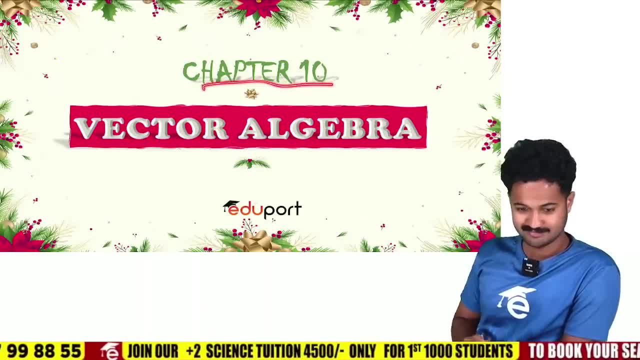 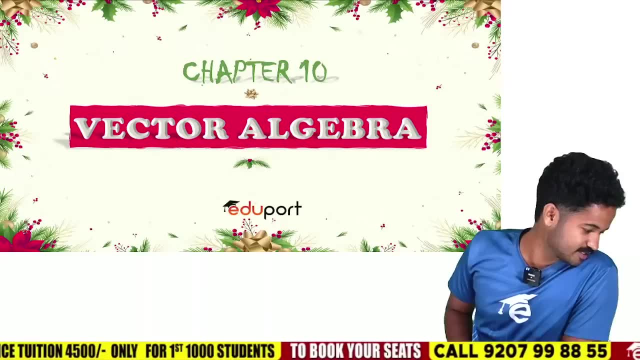 Hey, a mallu vlogger is coming. Can I vlog? Ready, So ready. Okay, Since it's morning, I'm not saying a lot of things. I'm not saying that you should share this with your maximum friends. 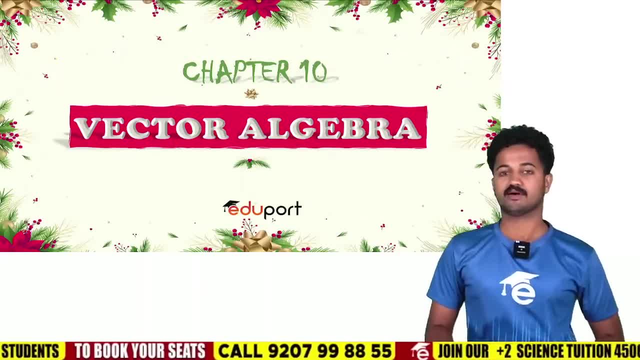 When will it end? We have to finish by 7.30.. We have to finish two chapters in one and a half hours. I said that both are simple chapters. We have to finish two chapters in one and a half hours, So okay. 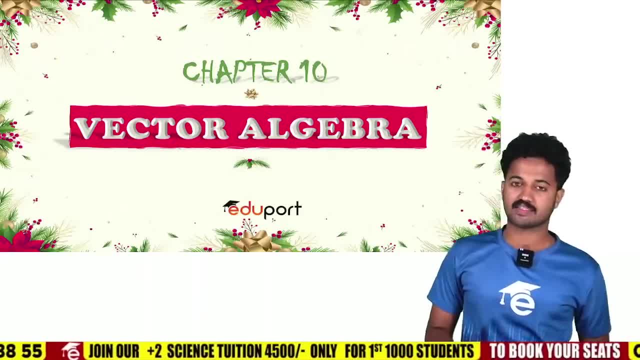 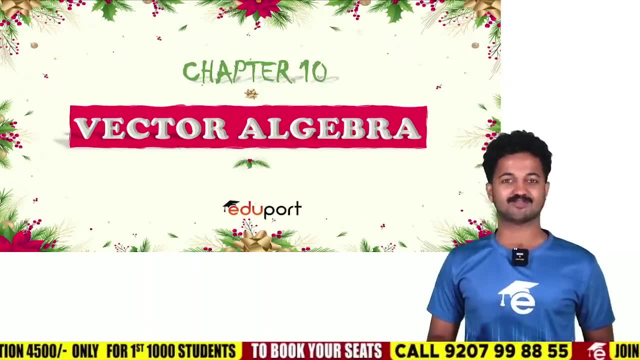 Okay, okay. A lot of people have come, So first, all of you who came, please like the video. All of you who came, please like the video. It's very, very, very, very happy that so many people came in the morning. 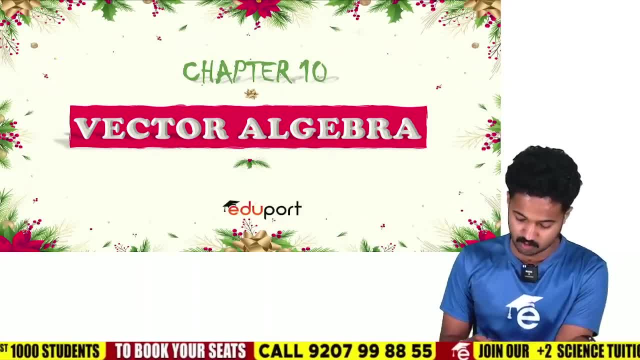 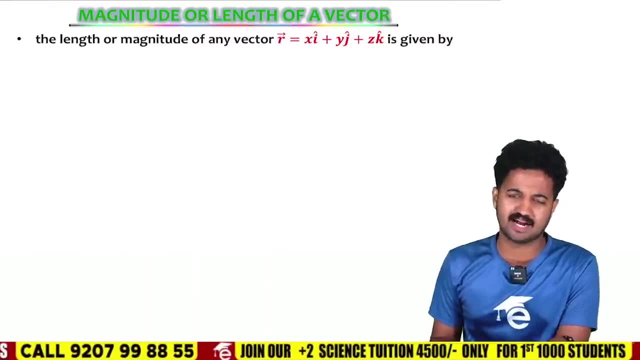 So if that's the case, let's start. We are not saying a lot of things. We can see the rest directly. So first we are talking about vector. So when you study about vector, you should first understand how to represent it. 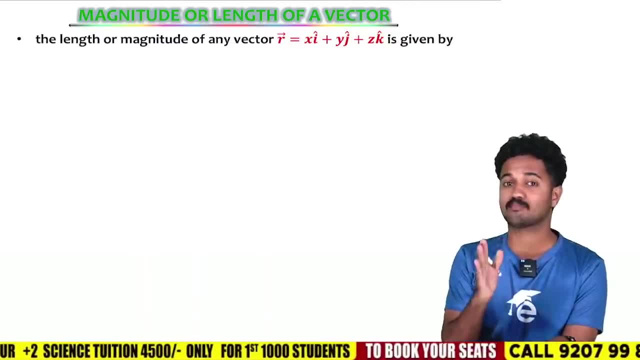 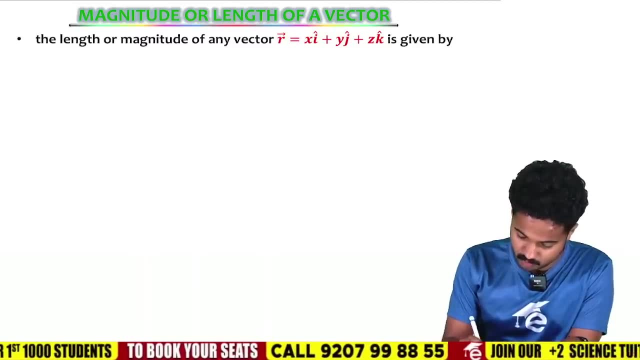 You should understand that Vector. So what do you know? A quantity having both magnitude and direction. That's what we call vector. So you saw the same thing in physics. So look, Here we have a vector. What does this mean? 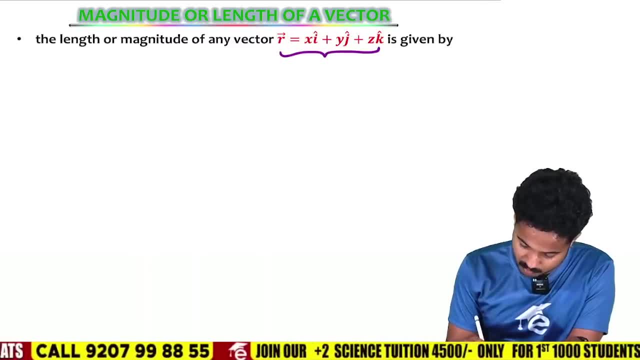 We call it the component form of a vector. Right, This is the component form of a vector. This is the component form of a vector. Okay, Ready, This is what we call component form. Component form, No problem. So this component form. 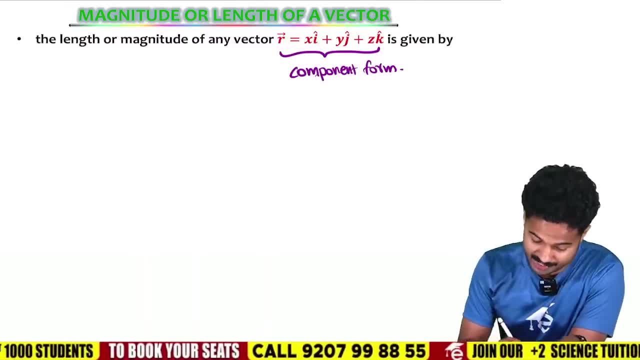 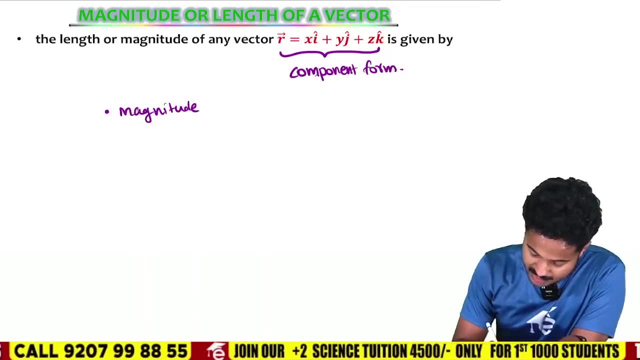 the component form of a vector. if we have given the component form of a vector, how do we find its magnitude? The magnitude of a vector is very simple: The magnitude of that vector. So if the vector is R, how do we denote its magnitude? 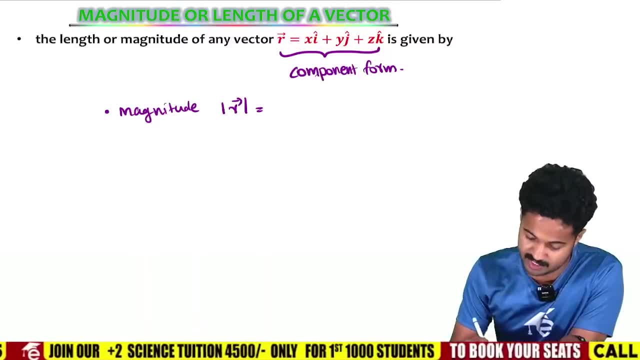 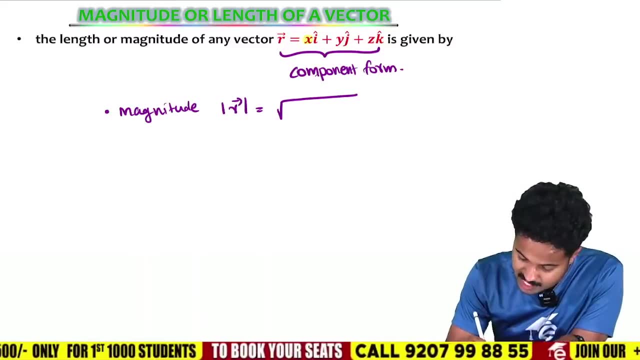 Magnitude R. Sir, how do we find this? It's very easy. What do you do inside that root? The scalar components of that? the scalar components are x with i, y with j and z with k. These are the scalar components. 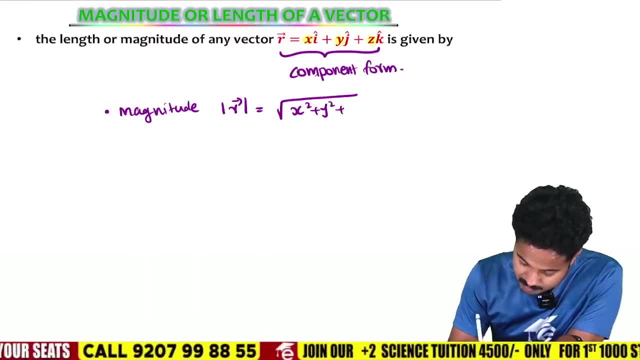 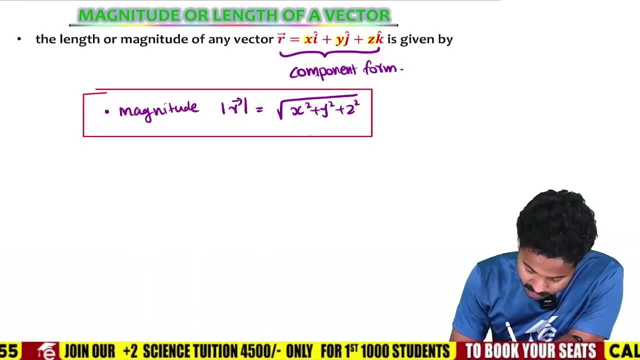 Take the squares of all these and the sum of them, This is the magnitude of that vector. So this thing should be known first: How to find the magnitude of a vector: The root of x square plus y square plus z square. 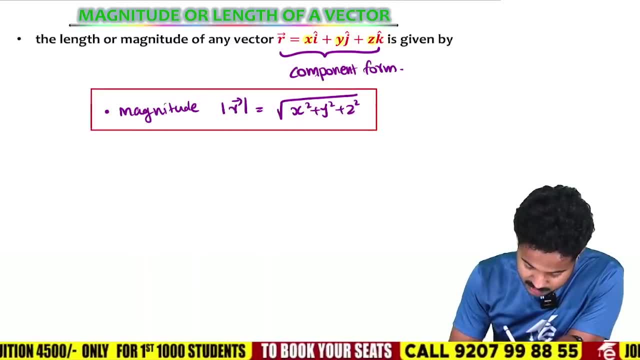 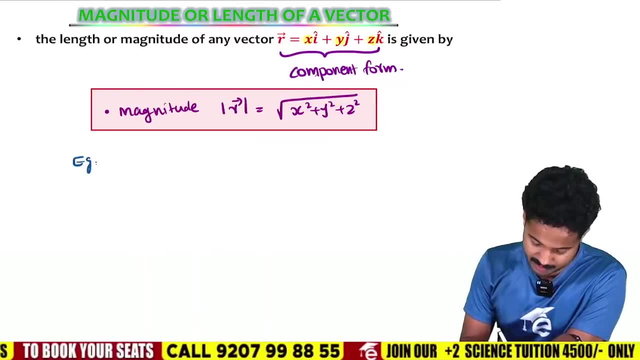 Okay, The root of x square plus y square plus z square. You should know this thing first. This should be known as the basic. So I'll tell you the example. We have a vector If vector a is equal to i plus 2j plus 3k. 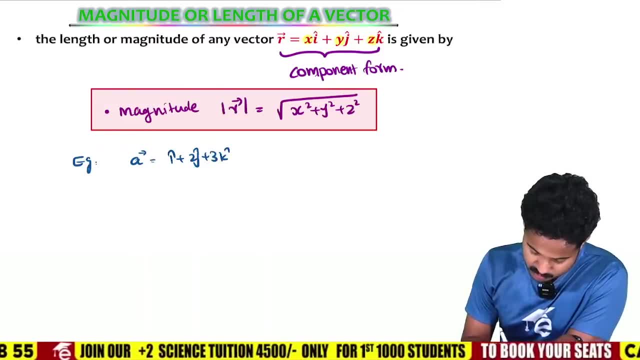 if it is i plus 2j plus 3k, its magnitude is the magnitude of a is the root of i is 1.. 1 into i is i, So it is 1 square Plus j is 2.. 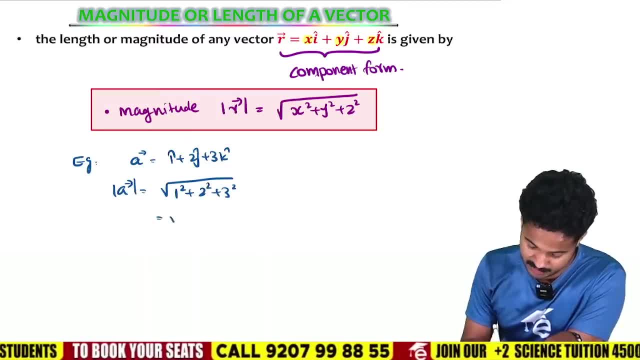 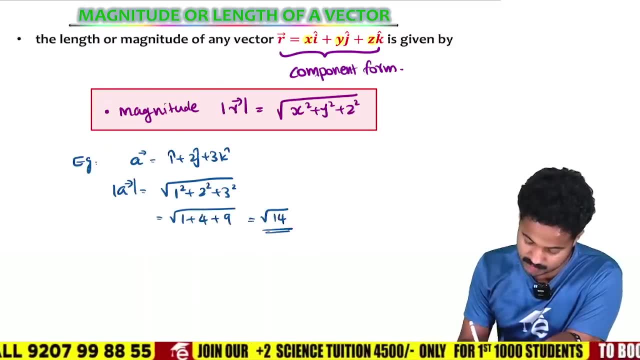 So it is 2 square Plus k is 3 square. So when you add them all together, 1 plus 4 plus 9, will come. That is your answer- is the root of 40.. So like this: 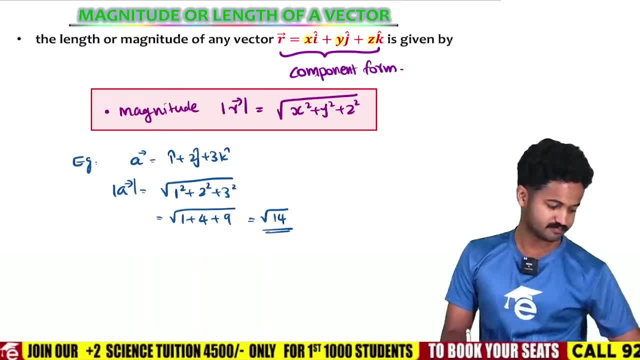 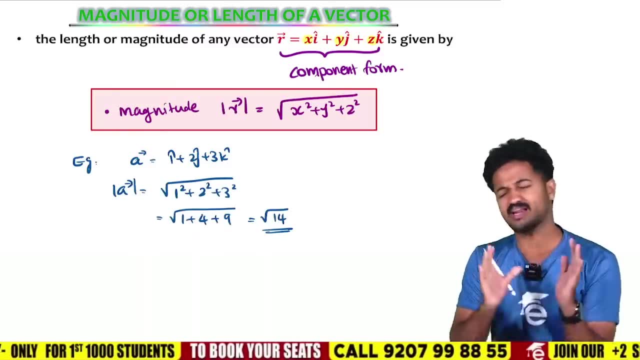 Yes, Okay, This is enough. Is it enough? Yes, So that's how we do it. Are you ready? Is it okay? Yes, The root of 40.. So this is the magnitude. It is a very simple and easy thing. 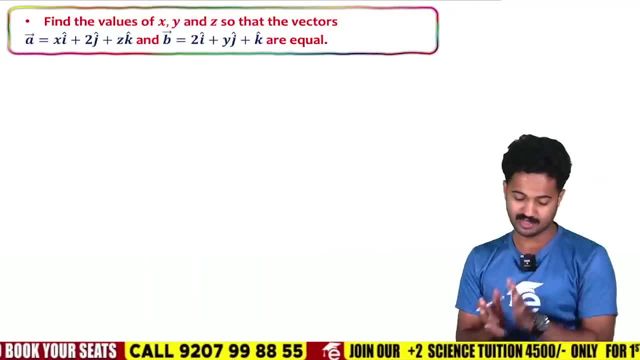 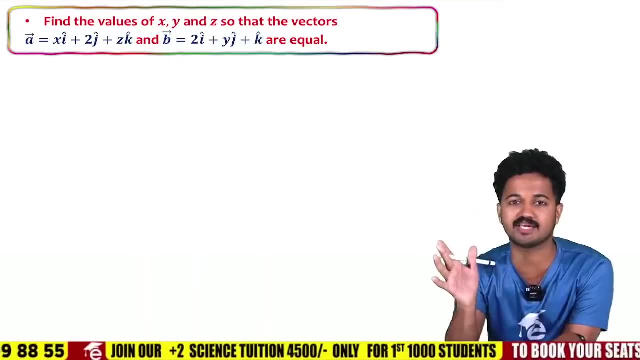 You just need to know all that. It will give you the component form. You will find the magnitude. Now, sir, when do we say that two vectors are equal? Hey, I have two vectors in my hand. If those two vectors are equal, 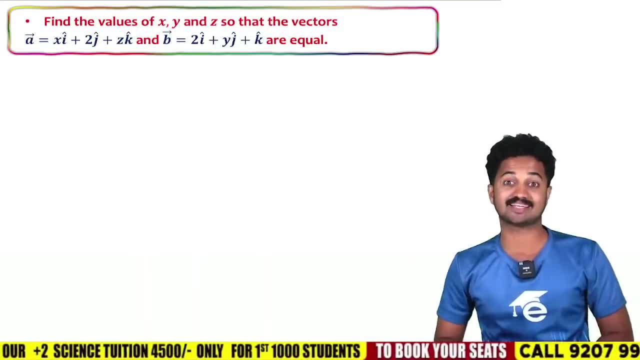 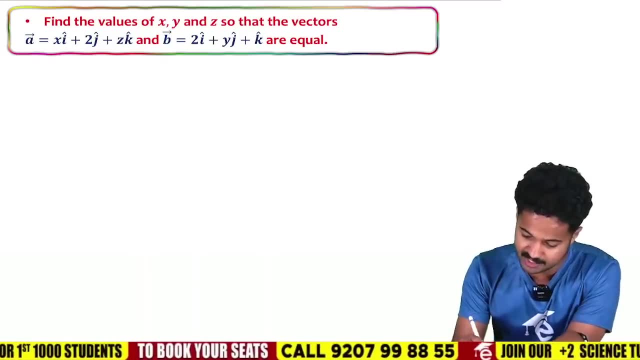 the scalar components of both should be equal. What are the scalar components? What is greater than i and j and k? That is the scalar components. So look here. Here the two vectors, a and b, are equal. That is vector a is x, i plus 2, j plus z k. 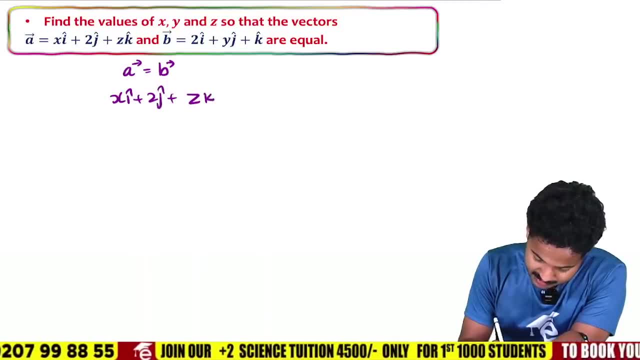 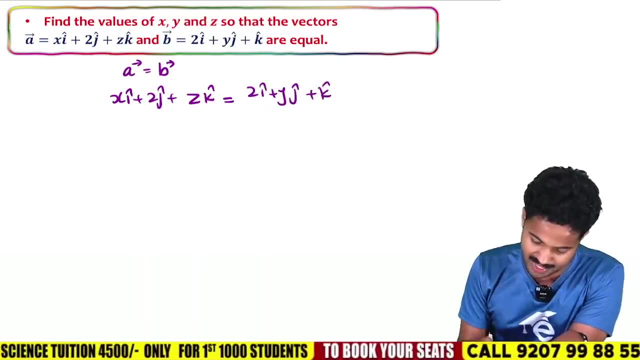 Similarly, vector b is 2 i plus y, j plus k. If these two are equal, what will be the value of x, y and z? Easy, You can find it simply: x is greater than i, Who is equal to x. 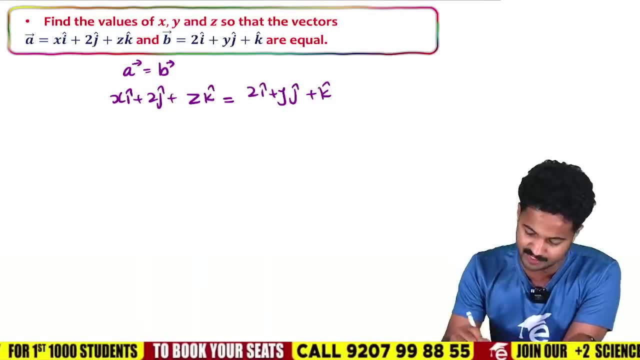 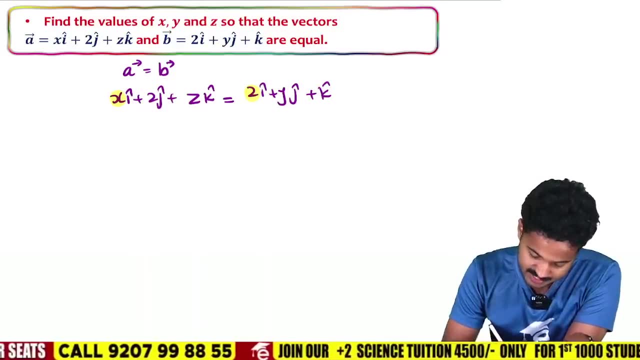 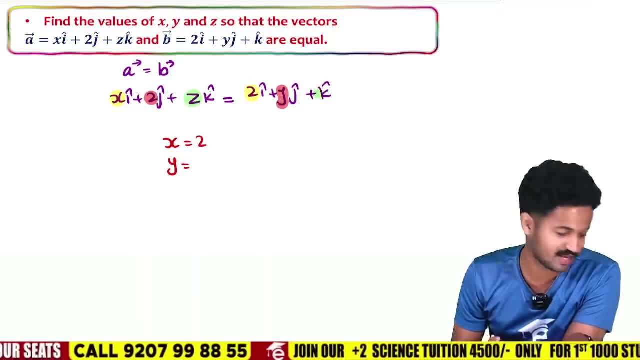 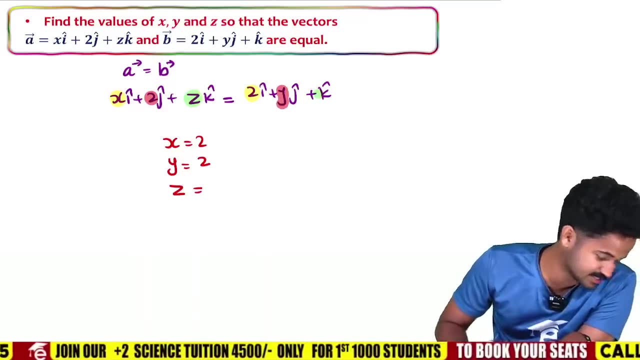 20., 21., 24., 25., 26., 27., 28., 29., 30., 31., 31., 32., 34. Or 1, z equal to 1. Easy. 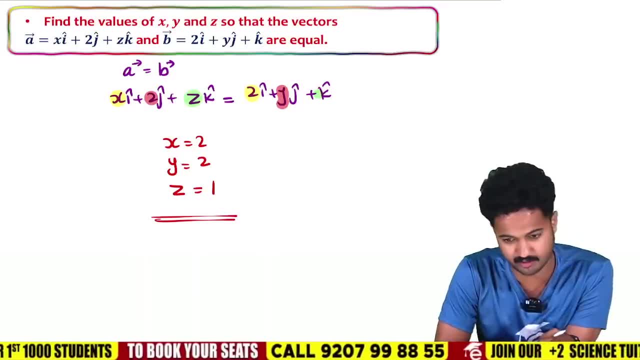 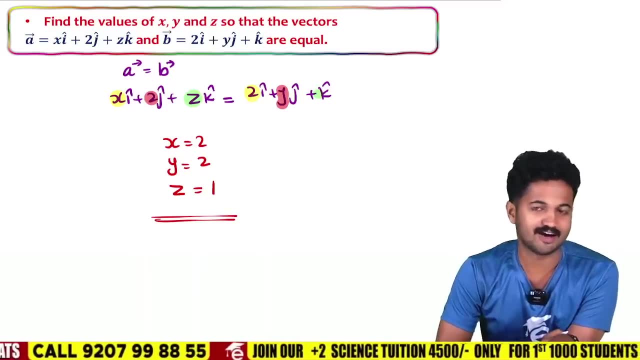 Ready. Yes, it's 1, it's 1.. Answer is commenting: Very good, very good, Awesome, right, Awesome. answer is commenting: Everyone is commenting. Okay, Plus 2 is broken. If you first change that, thought half is over. 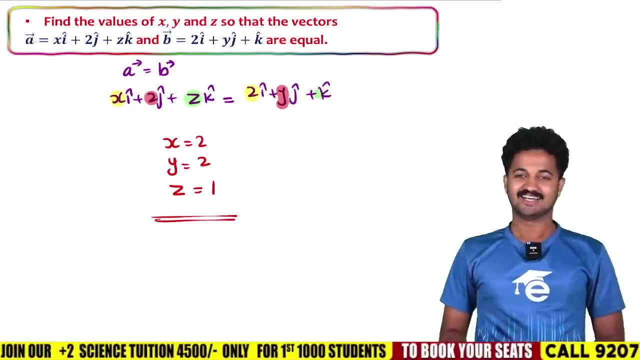 Hey, plus 2, do whatever you want. No one is going to lose. No one is going to lose in this time. No one is going to lose, Everyone will win. You have to get the maximum mark right. You have to get the full mark after A plus. 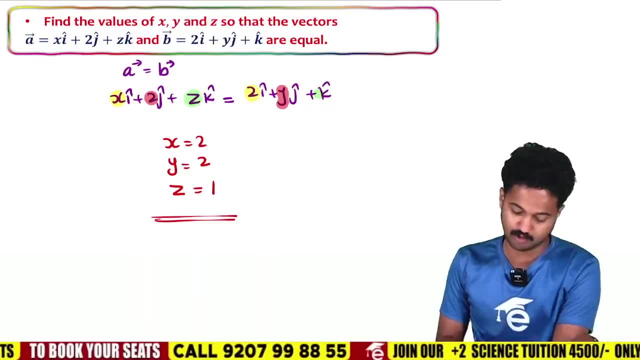 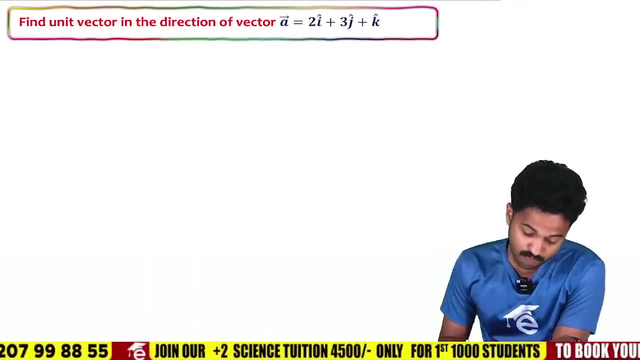 Do whatever you want, No worries, So ready. So y equal to 2.. This is how two vectors are equal, No issue. These are simple basic things. Now the next one. This is important: Find a unit vector in the direction of the vector A. 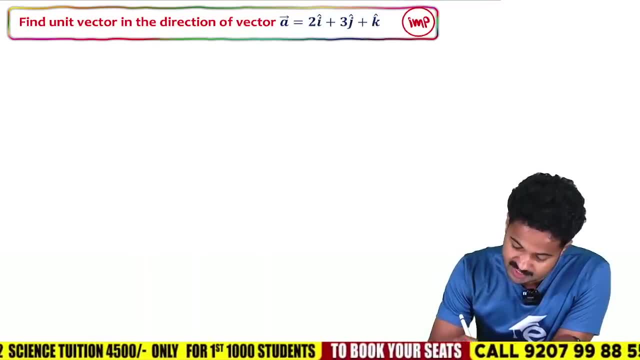 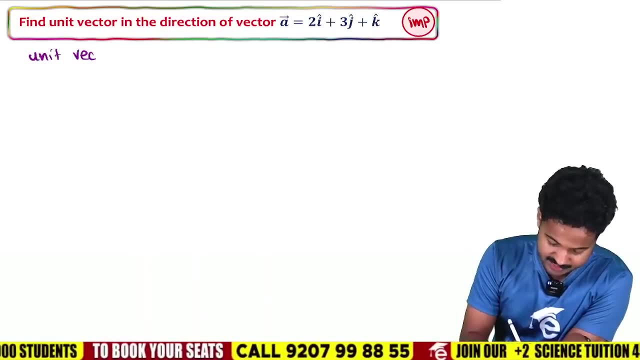 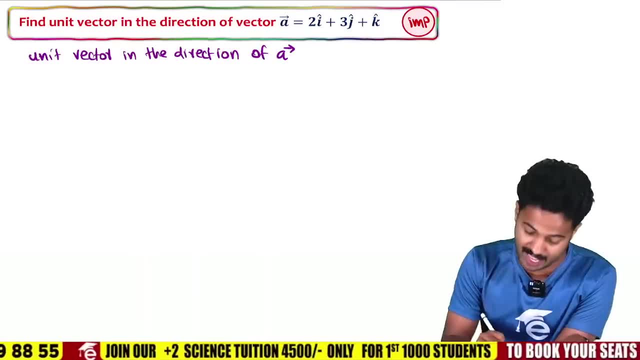 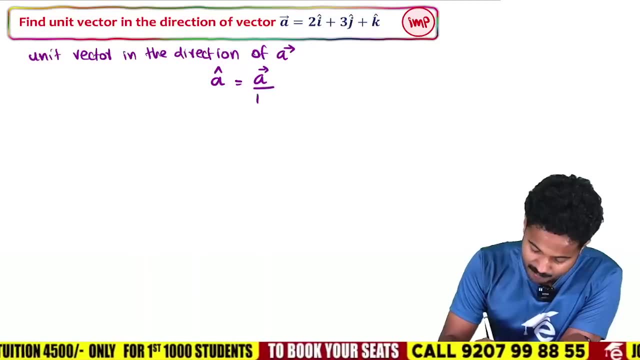 Unit vector in the direction of a vector. We denote it like this: A cap, A cap. Sir, how does A cap represent Vector A by magnitude of that vector. So is this enough to learn? That is enough to learn. 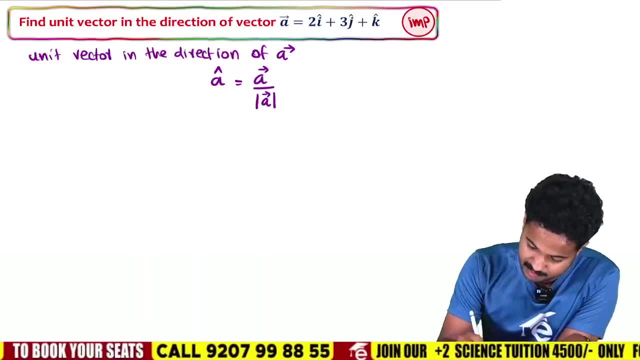 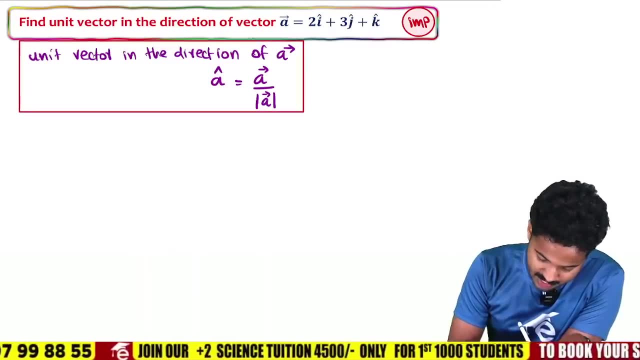 If you want to find a unit vector in the direction of a vector, you can use this equation: Sir, what is unit vector? I don't understand What is unit vector. It is easy: Unit vector is the magnitude of a vector. 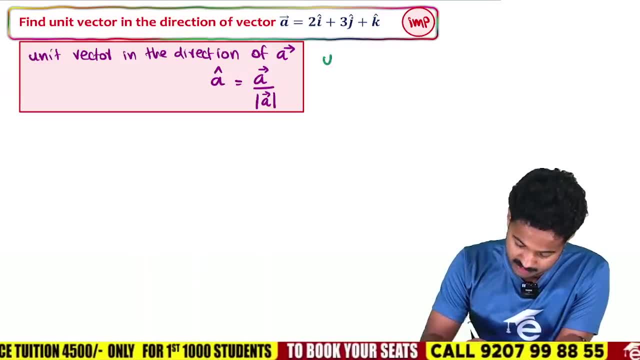 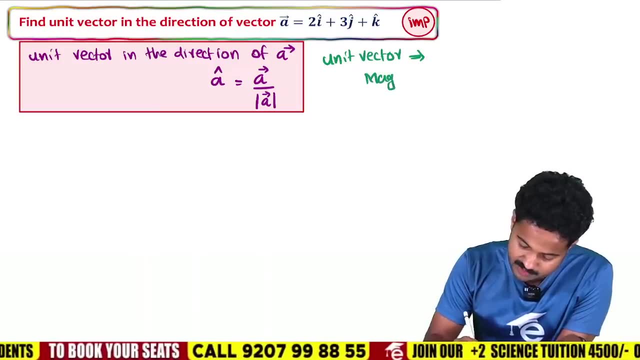 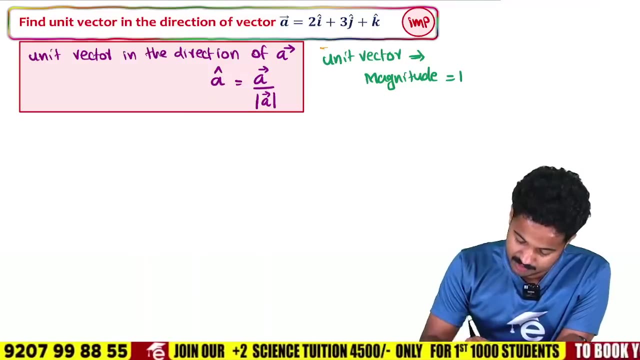 If it is 1, that is called unit vector. Unit vector is this here Unit vector? Unit vector means magnitude of that vector is 1.. What is magnitude of that vector? Magnitude is equal to 1.. Sir, that is how you can say. 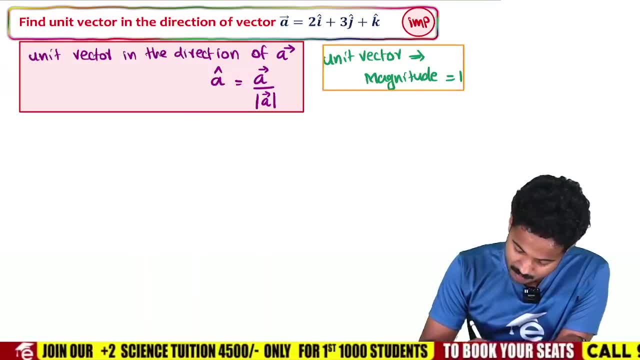 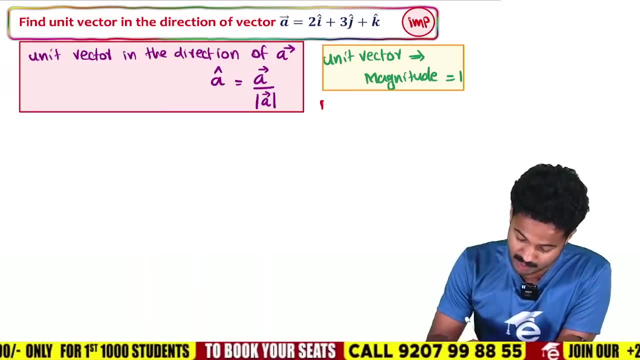 unit vector. Isn't it easy? Yes, it is easy. Is there any vector that is magnitude 1?? Those are unit vectors Easy If magnitude is 0, then you know another name: Null vector If magnitude is 0,. 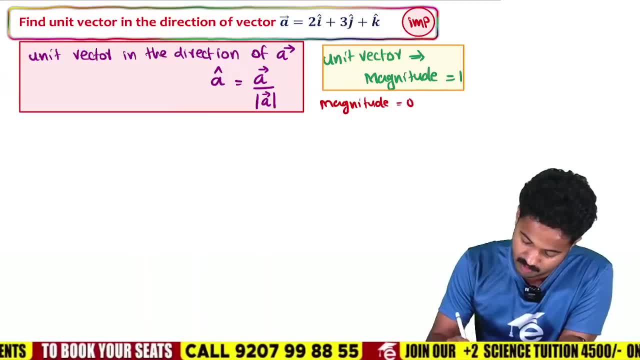 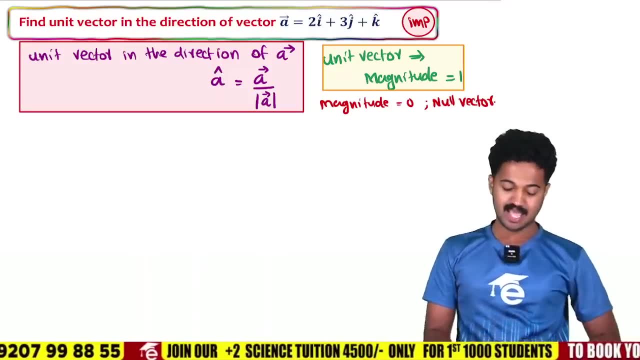 then you know another name: Null vector. Magnitude equal to zero is known as null vector. You just need to know these things. Magnitude one is unit vector. So, sir, there is a vector called A. We need to get a unit vector in the same direction. 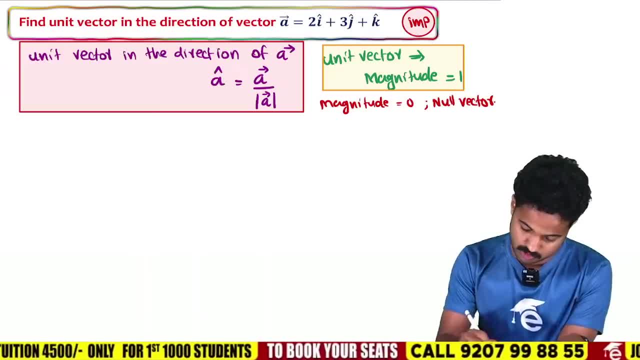 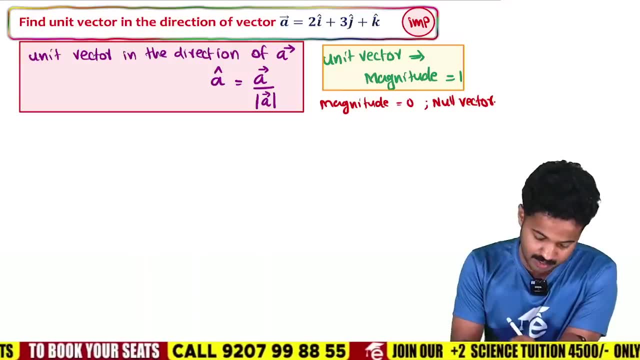 What is a unit vector? Magnitude one. So we have learned the equation. Easy, isn't it? This is the equation to find the unit vector, Vector A, by magnitude of A. Easy, isn't it? So look here. 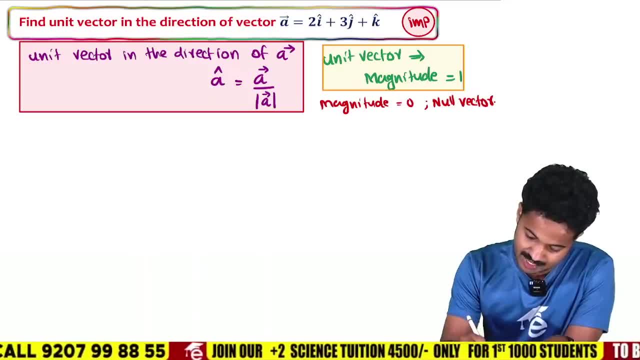 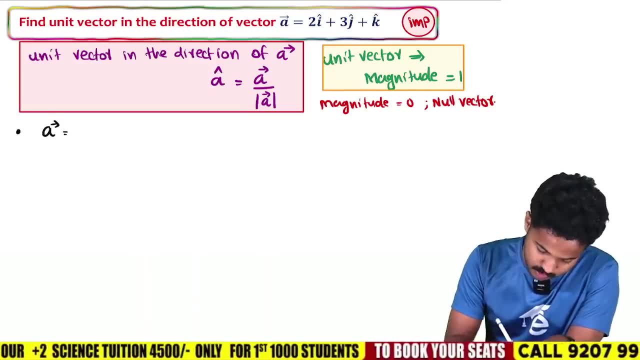 In this question you have given what is A. You just need to tell what is A. What is A, Sir? A is 2i plus 3j plus k. Okay, easy, 2i plus 3j plus k. 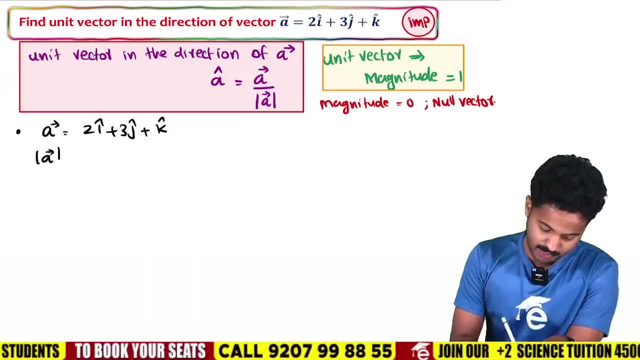 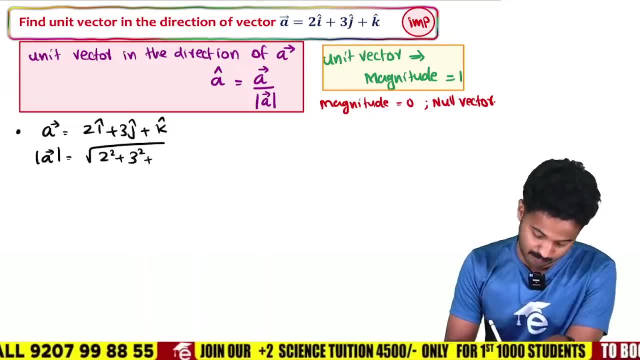 Okay, simple, isn't it? What is the magnitude of this Magnitude? is its length? Magnitude is 2 square plus 3 square plus k. The coefficient is 1. So 1 square. That is the answer. 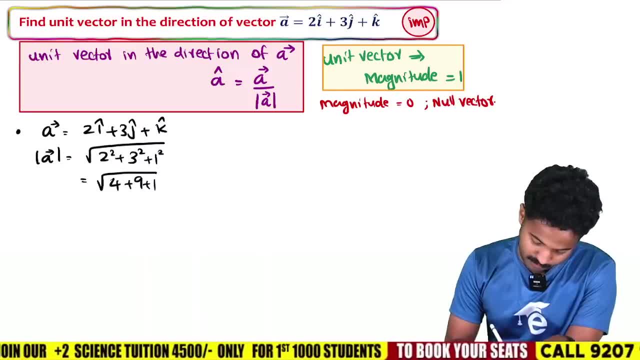 4 plus 3. 3. 3 square 9 plus 1. That is 4 plus 9.. 13 plus 1., 14. So the root is 14. Magnitude of that vector. Okay, isn't it? 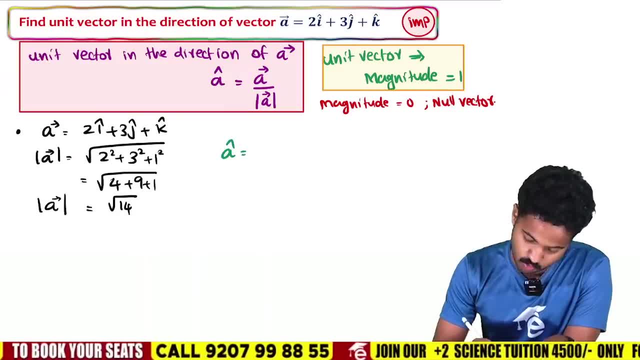 Easy, isn't it? Now, this is your question. This is what you have seen: Unit vector in the direction of A, That is, we call it A cap, Which means vector A by magnitude. A Easy, isn't it? 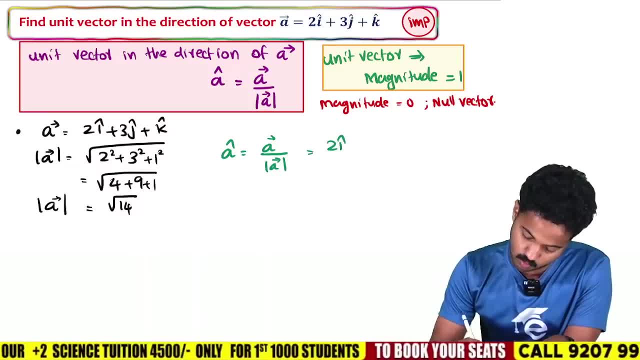 So look here, Vector A. The vector A is 2i plus 3j plus k, And what is magnitude of that vector? That is root 14.. If we make it even better, we can write it like this: 2 by root 14i plus 3 by root 14j plus. 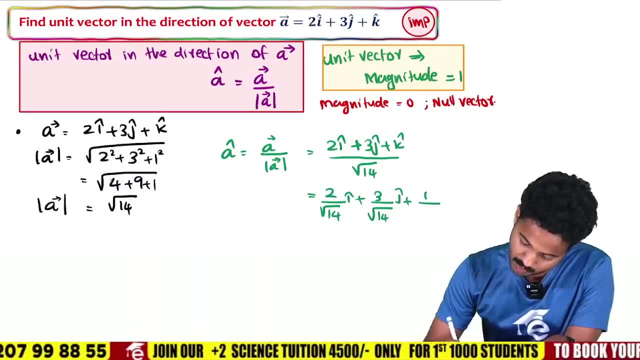 Then what is the next one? There is 1, there isn't it? The coefficient of k, So that is 1 by root, 14k. This is the answer Ready. This is the answer, So don't forget this equation. 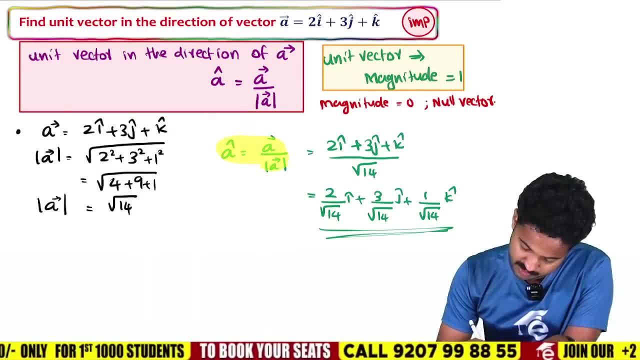 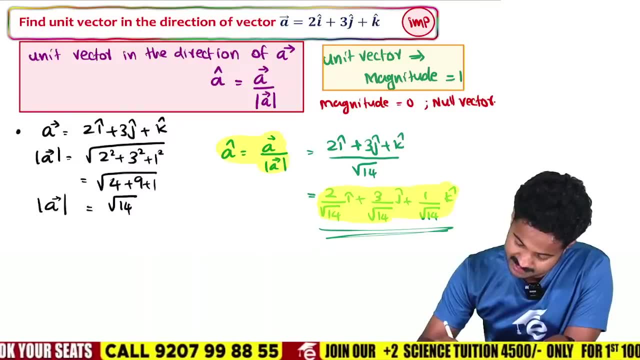 See, don't forget this equation. This is the equation to find the unit vector, And this is the answer to this. Okay, isn't it? It is simple, isn't it? There is no problem, isn't it? All those who got it will get a green ticket soon. 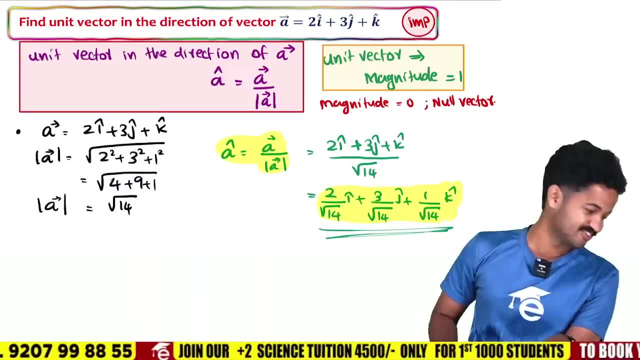 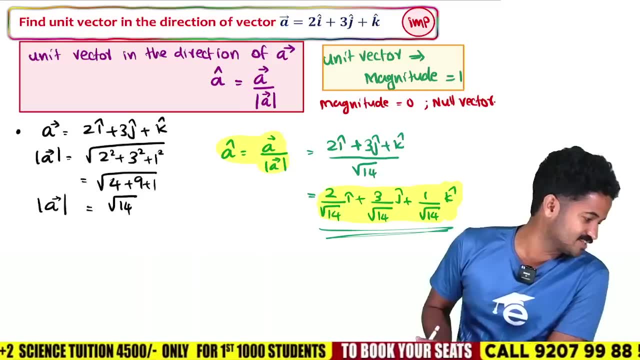 Green ticket. They said to get a green ticket in the morning itself. This person must be asking where this is coming from. Yes, very good, It is 1 by root 14.. To make sure that you got it, it is necessary that you have studied this. 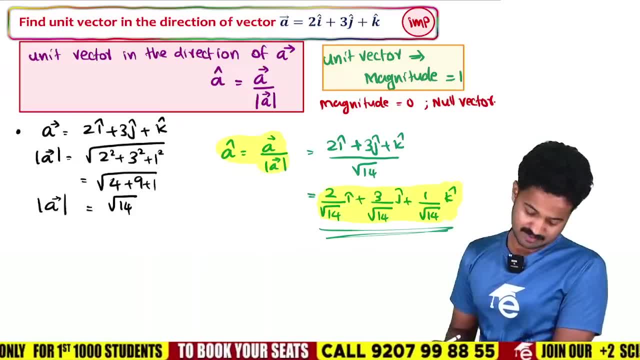 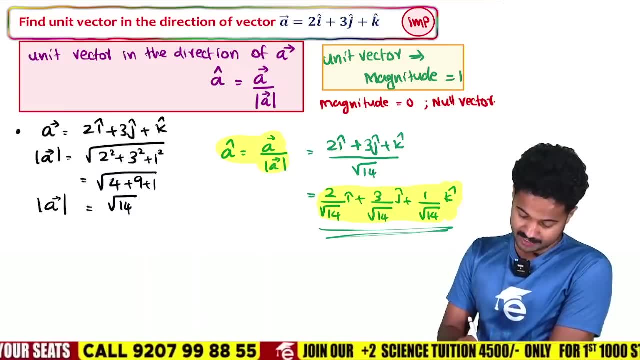 All those who got it will get a green ticket soon. It is simple, sir. All these are simple. You just need to learn the equation, There is no problem. Remember unit vector. Now, if you have taken the magnitude of this vector, 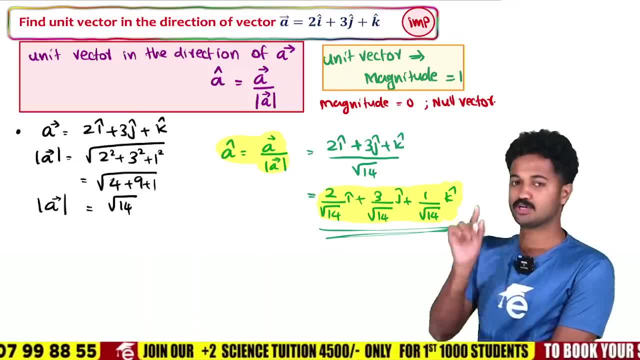 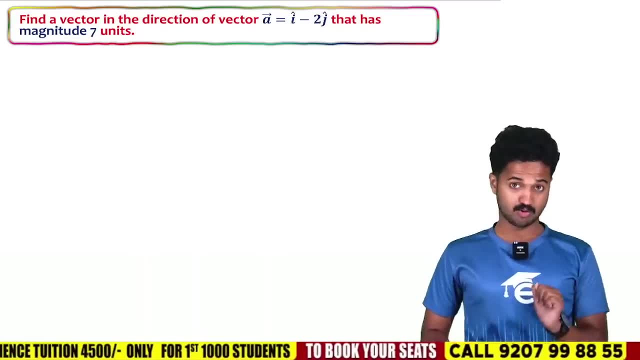 if you have added all these together, if you have added it into the square, if you have added it, you will get 1.. That is unit vector. Okay, sir, There is no problem. Easy, Easy, Simple. Now look at the next one. 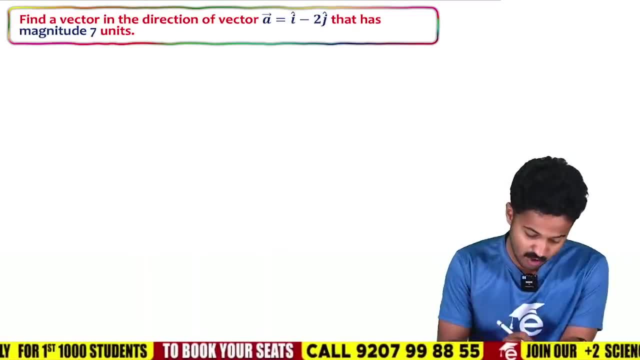 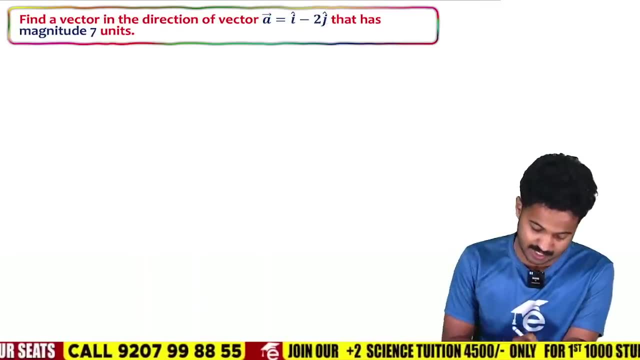 It is a question like this, Ask like this: Find a vector in the direction of the A vector, in the same direction of this vector. It is a vector in the same direction That has magnitude 7 units. So do you know what you have to do? 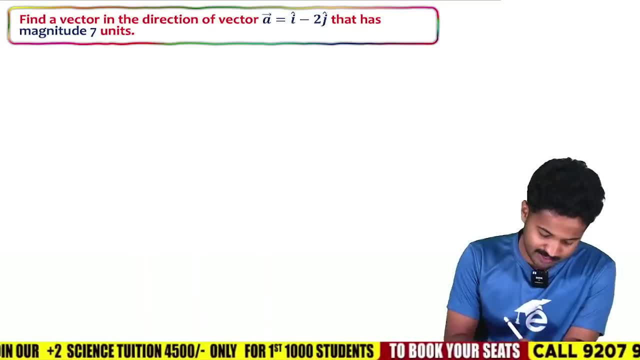 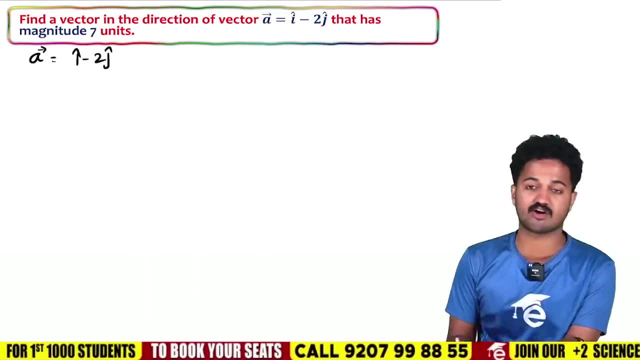 There is nothing. It is easy. The thing is easy. We have a vector in our hand. There is a vector called a. So this is your a. The vector that is called a is equal to i-2j, It is k and the coefficient of k is 0.. 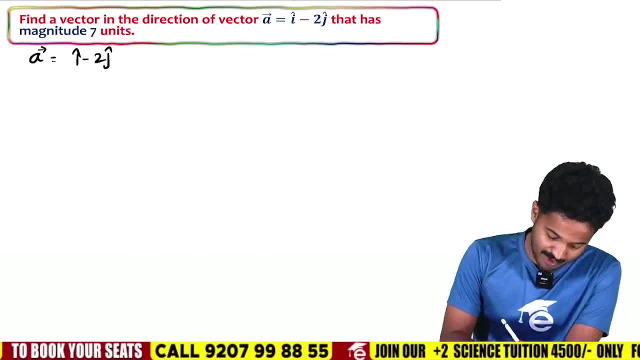 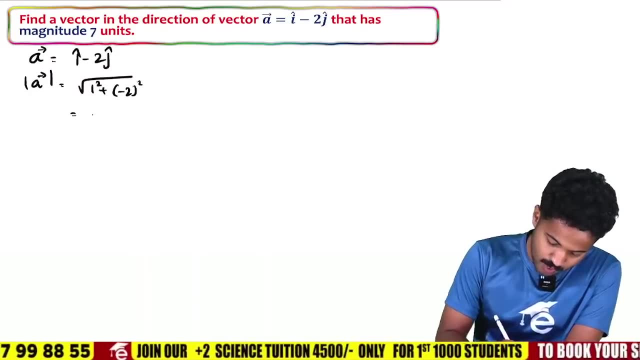 That is, the scalar component of k is 0.. So you can find the magnitude of this If you find the magnitude of this root of 1 square plus minus 2, all square, That is 1 plus 4, is root 5.. 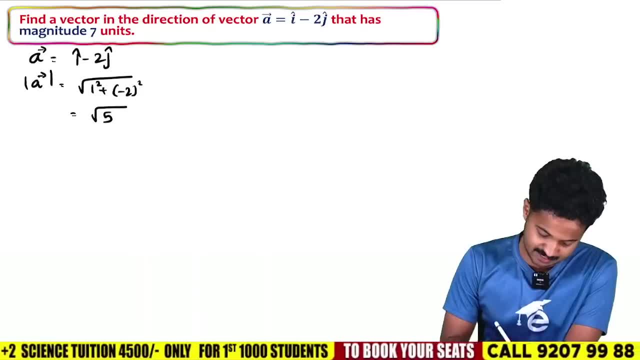 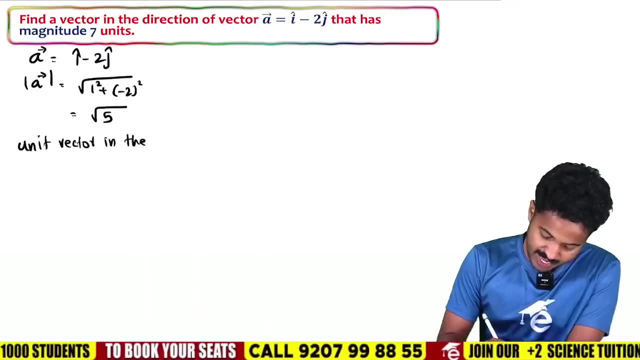 Right Root 5.. Now you have the magnitude of this. You don't know what you have to do. Unit vector in the direction of a. Unit vector in the direction of a. Find the unit vector in the direction of a. 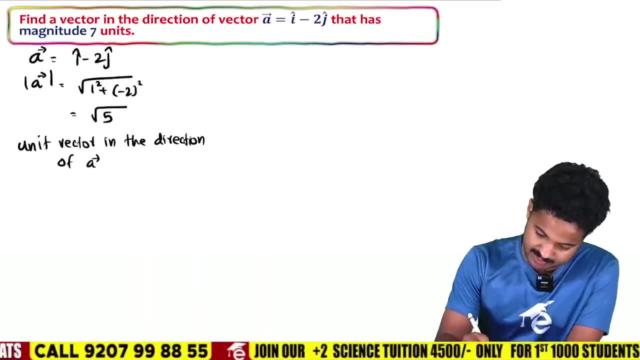 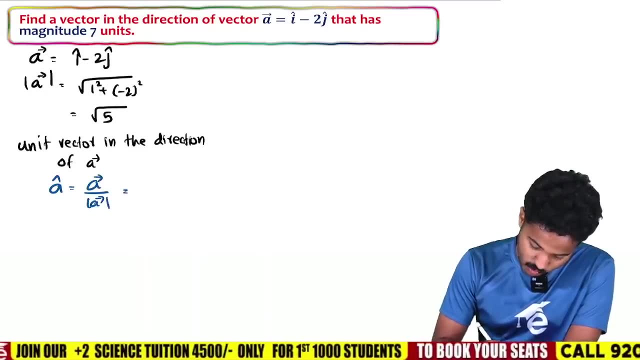 Unit vector in the direction of a. Sir, how is that? This is a cap. A cap means vector a by magnitude a. So what is your answer? Vector a, i minus 2j. What is magnitude of that vector? 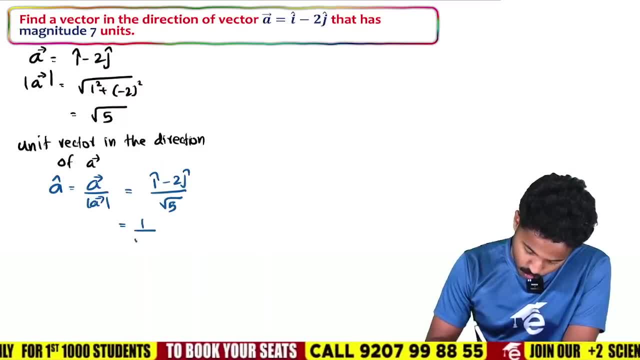 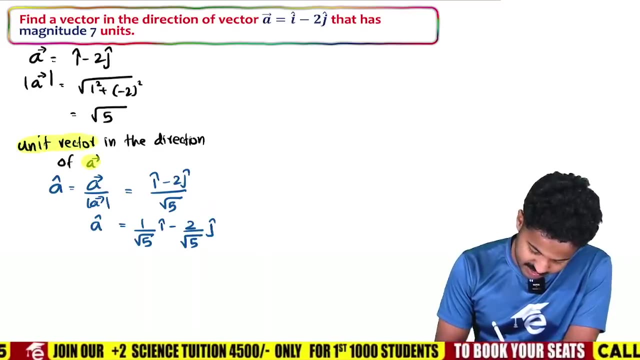 That is root 5.. That is 1 by root 5 i minus 2 by root 5 j. This is the unit vector in the direction of that vector. Okay, sir, No problem. See, we found the unit vector in the direction of a. 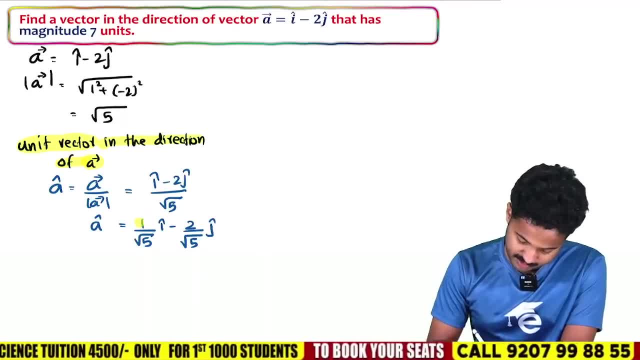 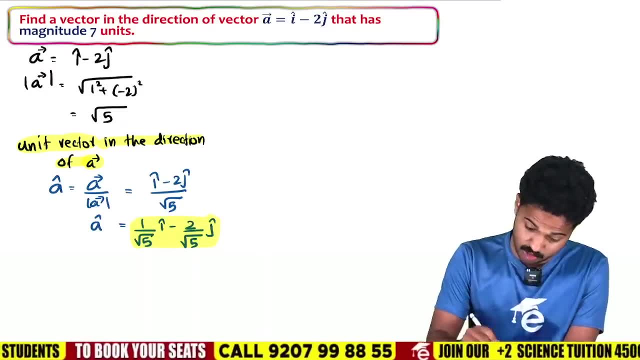 Unit vector in the direction of a. What is the answer? 1 by root 5 i minus 2 by root 5 j. This is easy, This is not a problem, But you have to understand the question properly. See what did you ask. 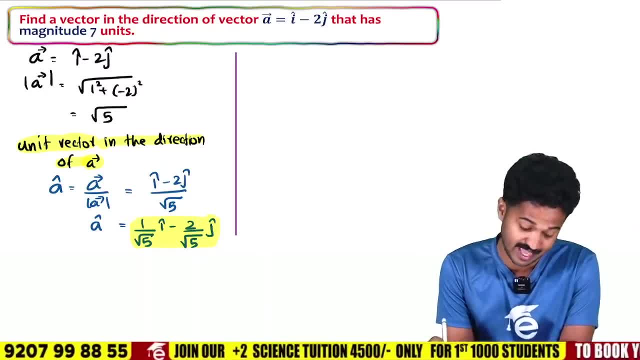 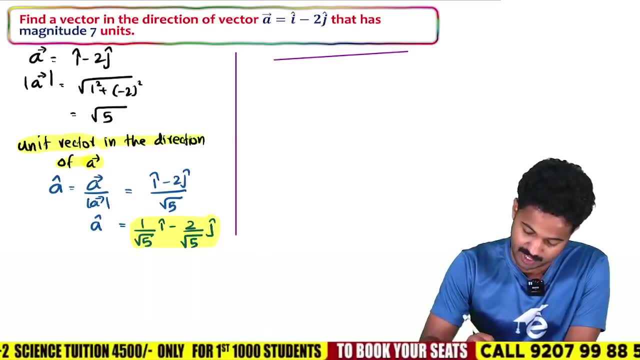 See, find a vector in the direction of a that has magnitude 7 unit. Isn't it great, See? this is a vector, A vector. Its direction is like this: The vector of a goes like this: This is the vector of a. 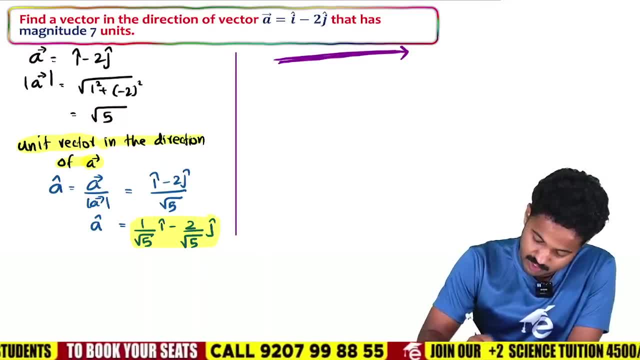 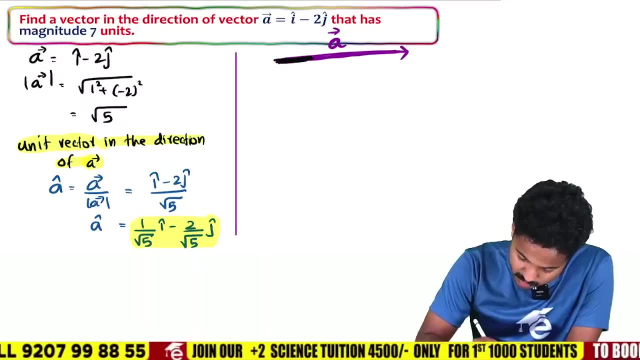 So the vector of a in the direction of that vector is very beautiful. This is the vector of a. This is the vector of a. So see this distance. this is the vector. sorry, this is the a cap. If we say a cap, the distance of this will be how much? 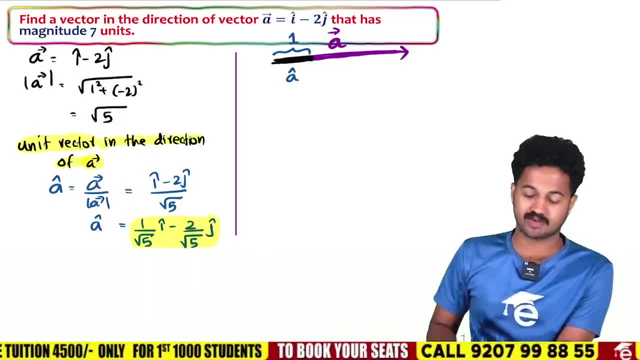 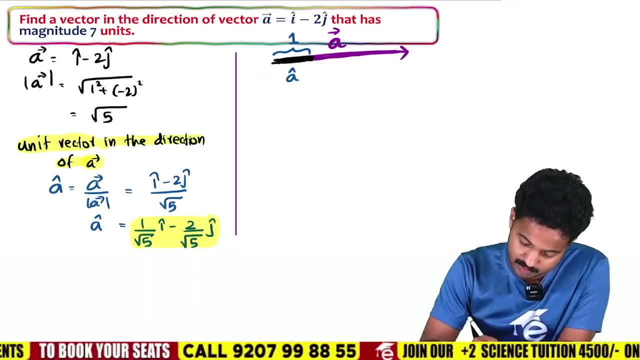 This distance will be 1.. That is why we call it a unit vector, So we have a vector with magnitude 7.. So when I took it like this, I understood that this is not a 7.. So I took this distance. 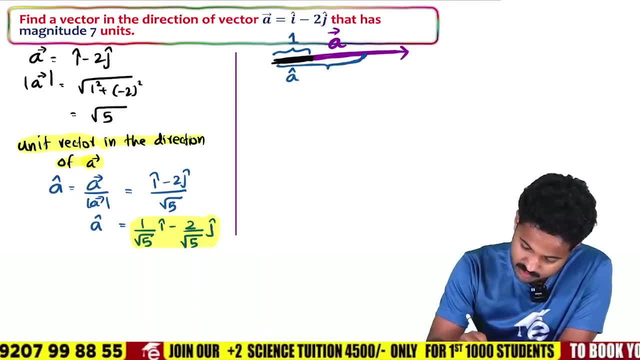 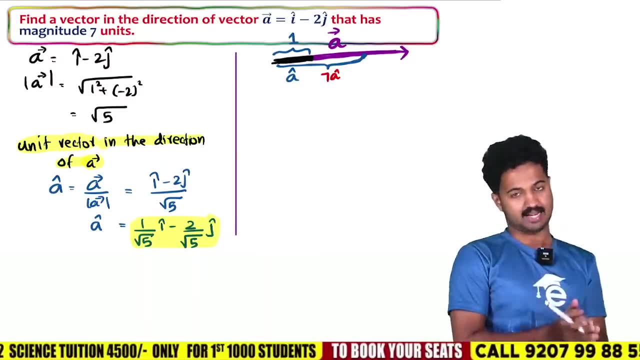 So this is the vector with magnitude 7.. This is the vector with magnitude 7.. That is, we have to find 7a, Isn't that right? So we know the vector a. We got the unit vector in the same direction. 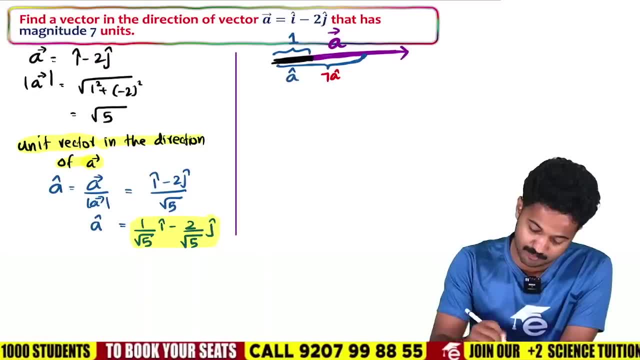 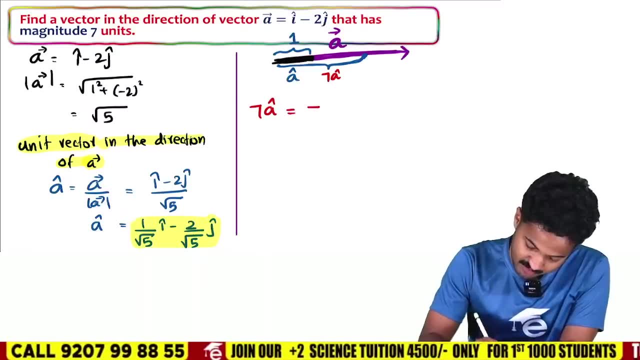 We got the a cap. So if you want to find a vector with magnitude 7, you just have to do this, You just have to do 7a. So 7a cap. We have got the a cap. What is a cap? 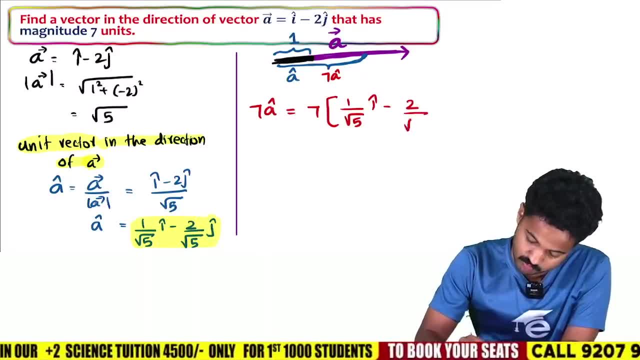 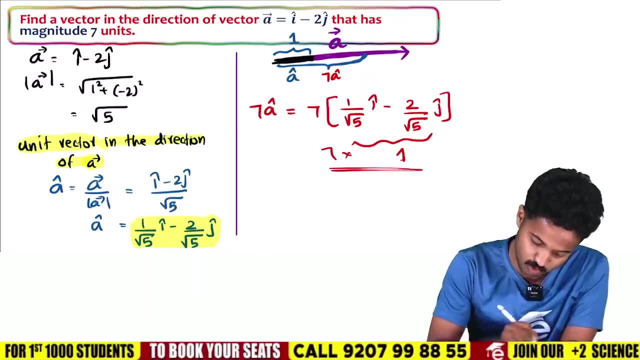 1 by root 5i minus 2 by root 5j. Simple sir, The magnitude of this will be 1.. So when you say 7 into 1, what is the magnitude of that? You will get only 7.. 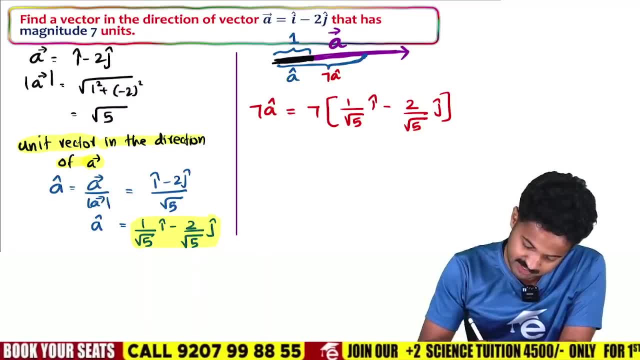 No issue. So you just have to multiply this. If you multiply this, you will get the answer 7 by root 5.. So multiply it to the bracket 7 by root. 5i minus 7 into 2 is 14.. 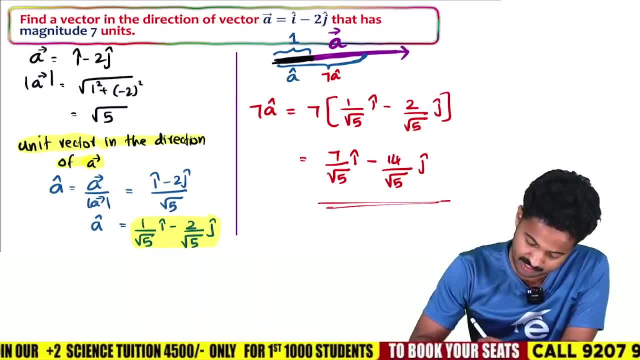 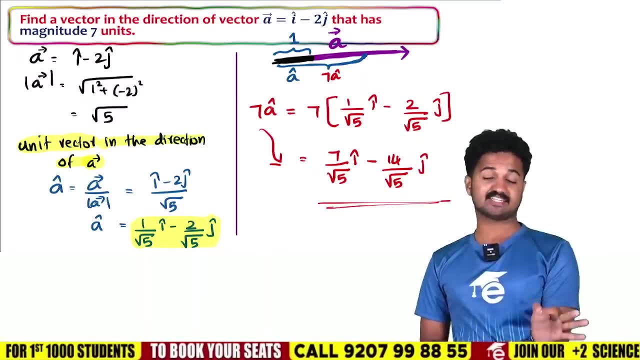 14 by root. 5j. Easy, Easy, It's over. So what is this? This is the vector with magnitude 7 in the same direction as the a cap. So whichever direction we find the unit vector, we just have to multiply it with 7.. 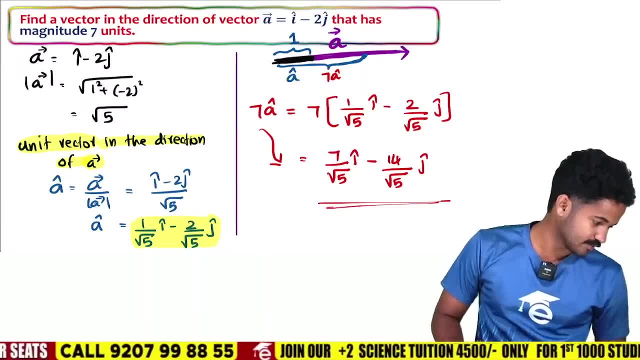 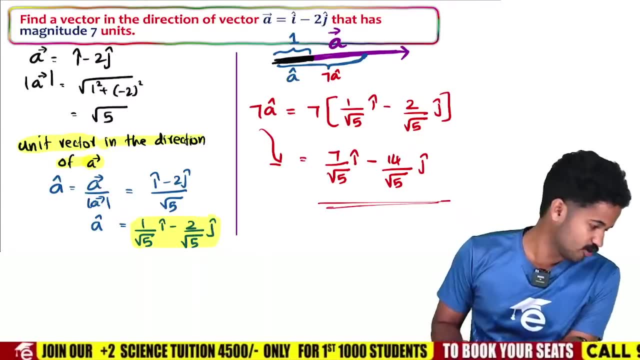 Easy, No problem, Okay, Ready. Okay, No problem, Easy, Simple. You can answer it easily. Okay, sir, Ready, Okay, 14 by root, 5. Okay, Simple, Hey, quickly, Let the green tick come. 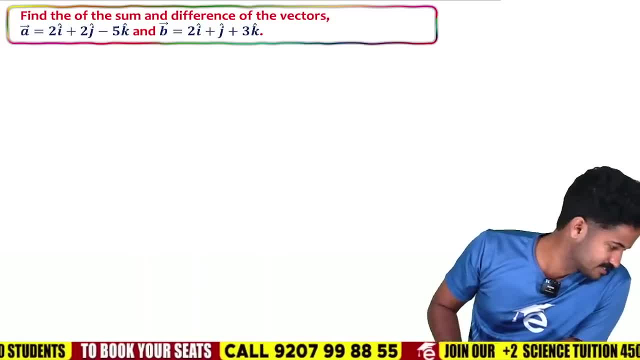 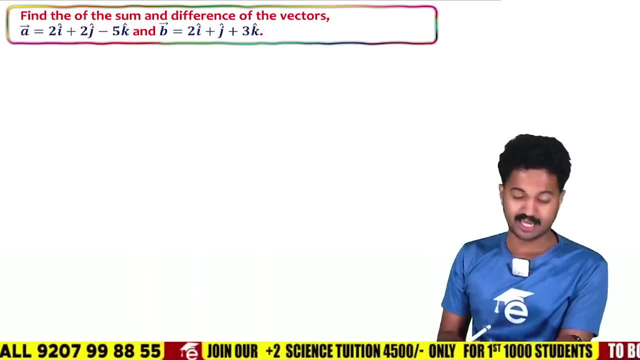 All the people put the green tick. Okay, If it's set, it's set. Yes, it's set. Quickly put the green tick. Okay, If it's set, quickly put the green tick. Quickly put the green tick. 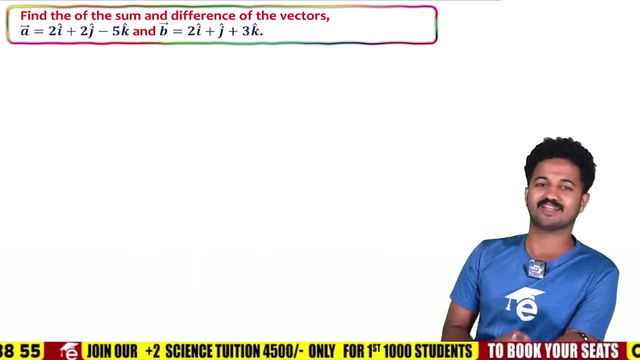 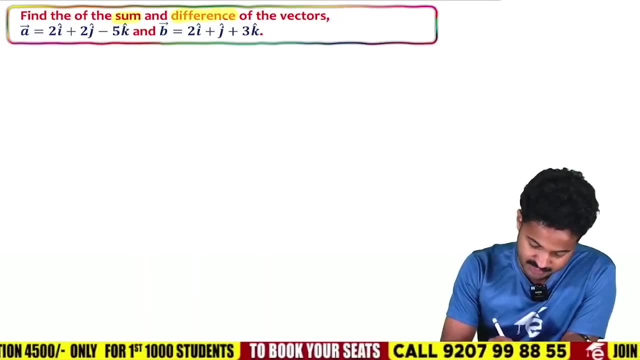 Next, If you ask a lot of questions, you'll learn everything. Next, look, Find the sum and difference. This is a little simple: Sum and difference. I've given two vectors. You have to find the sum and the difference. 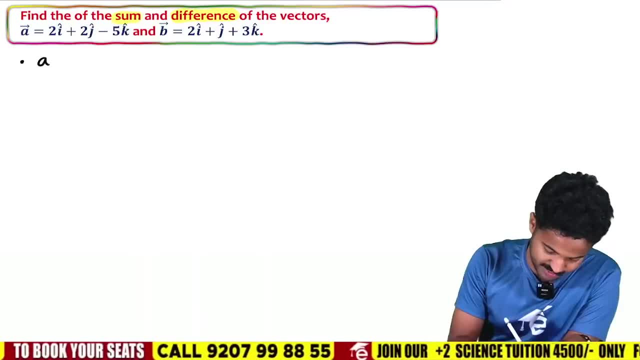 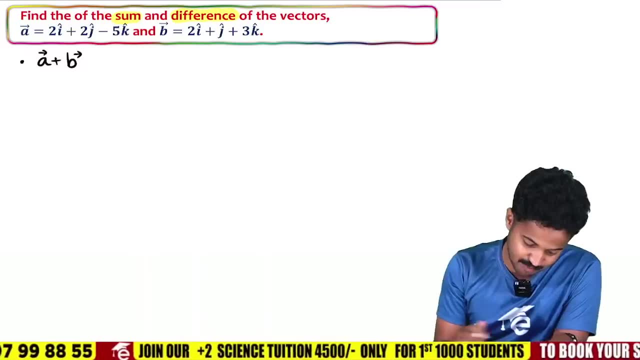 How is that, sir? It's so easy. First we have to find the a plus b. We have to find the sum of both a and b. That is very simple. If you have given a and b, if you have said sum, find. 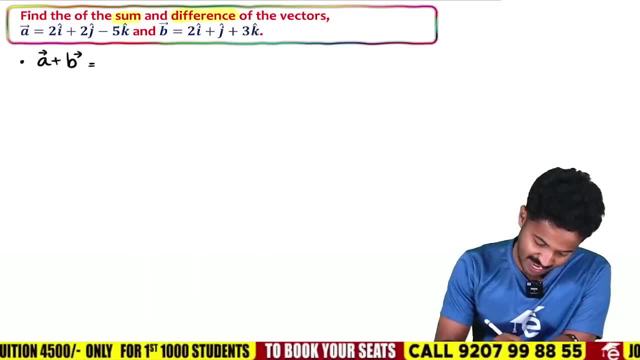 you can take i's scalar components and add. Look at this First: you can take this 2 and this 2 and add. Then the next one you have to consider is this: This 2 and this j's is 1.. 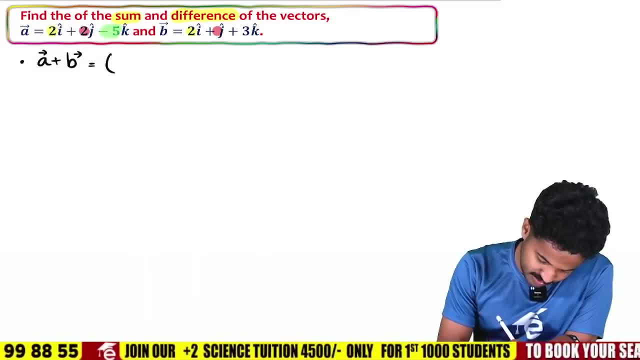 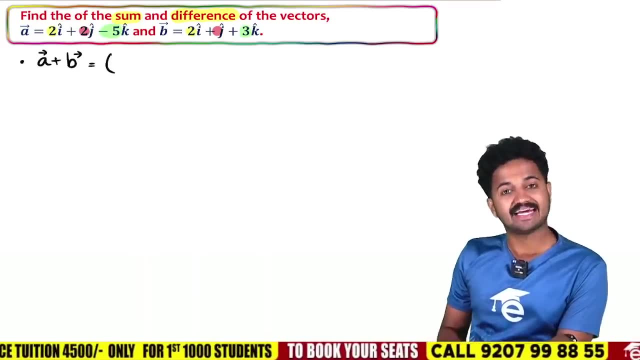 The next one you have to consider is this minus 5 and this 3.. Okay, So look at this. So first you have to add two vectors, You know, to add matrix. When we add matrix, we add corresponding elements. 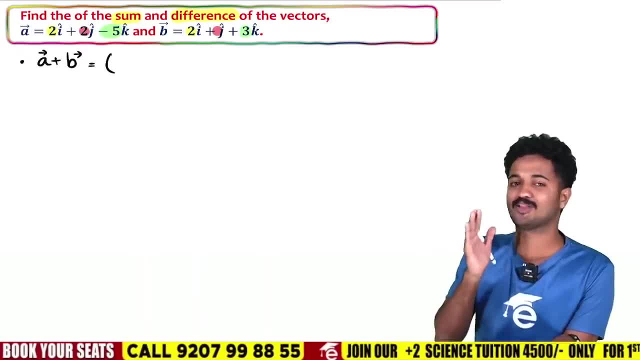 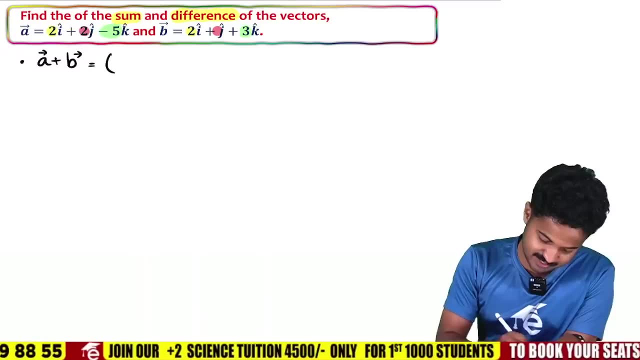 We add elements in the same row and same column. If we subtract, we do like this: First row, first column element, First row, first column element. Similarly, if you have said to add this, that is very easy, sir. 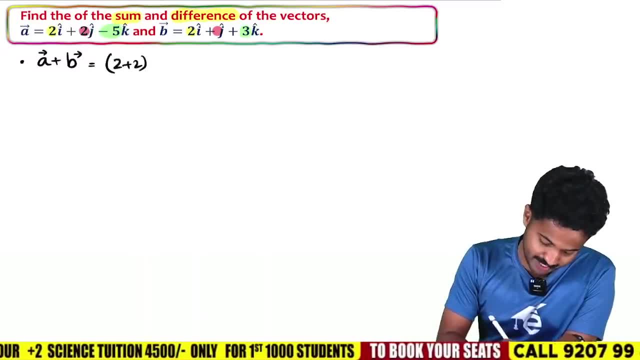 Here i's are 2 and there is 2.. So add this 2 and 2. Then i's are added Easy. Then both of you are plus. Why are you adding plus? We are adding vectors. 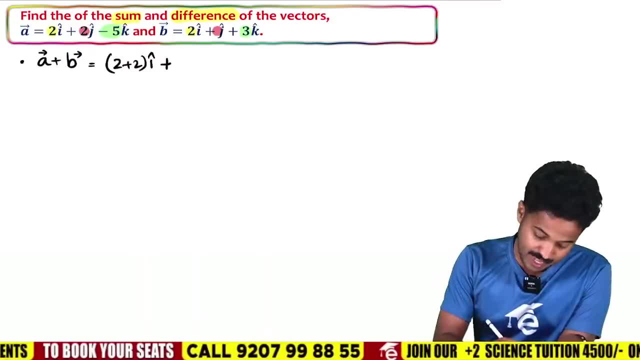 So when we add the component form, this is always xi plus yj plus zk. So easy. Then look at the next one. Here j's are plus 2 and here j's are plus 1.. j's coefficient is 1, right. 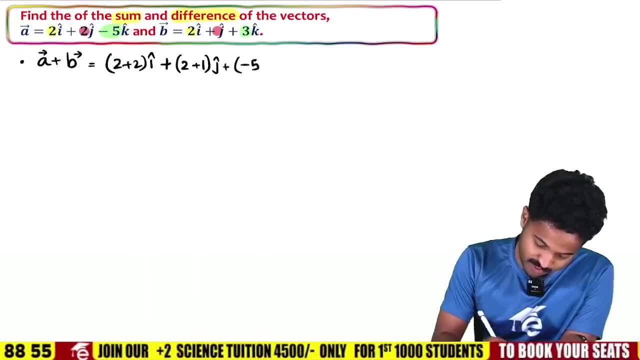 So j Plus: Here k's are plus minus 5 and here k's are plus 3.. So that's k Okay Easy. So look at this: 2 plus 2.. 2 plus 2 is 4.. 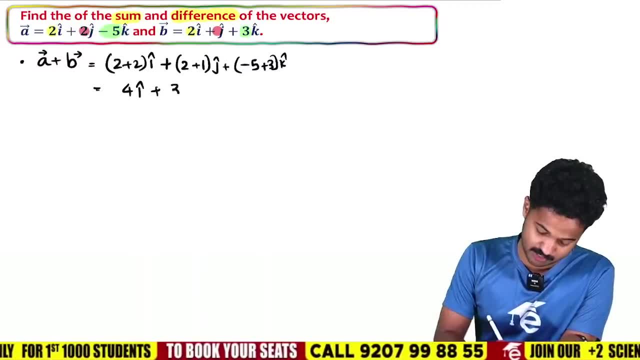 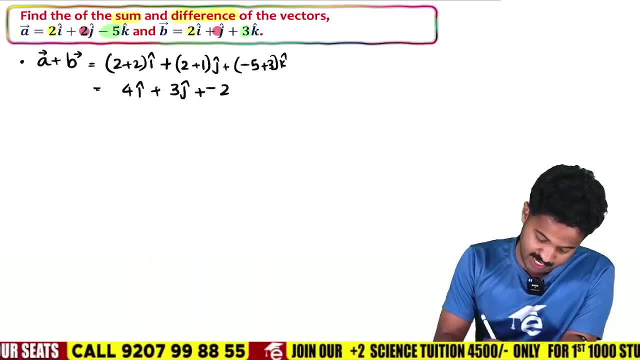 So 4i Plus 2 plus 1 is 3.. So 3 into j is 3j Minus 5 plus 3.. Minus 5 plus 3 means minus 2, right. So plus minus 2 is required. 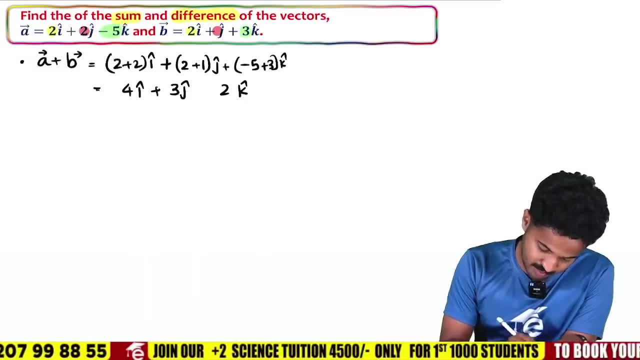 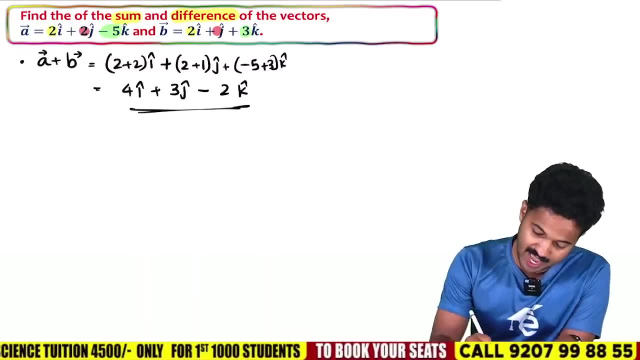 No, There, what is required? Minus 2 is required, So minus 2k. This is the answer. This is the answer Easy, Got it? Yes, Okay. And if that's the case, just like this: 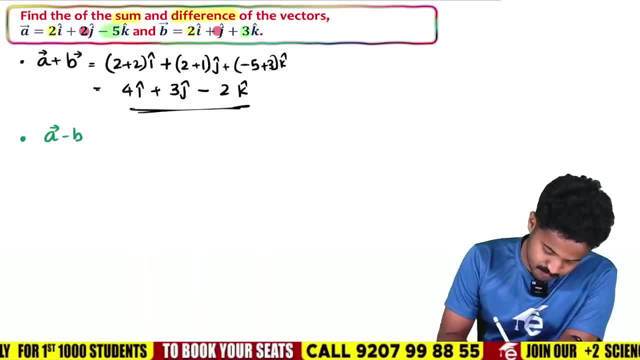 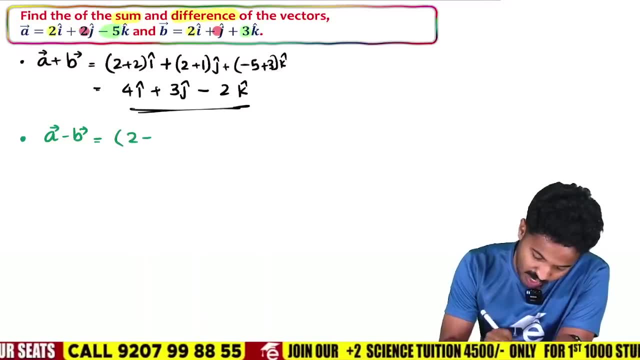 comment the answer of a minus b. What is a minus b? a minus b? When we do a minus b, the same method. Same method, Don't change anything. i plus 2.. There, i plus 2.. So 2 minus 2i. 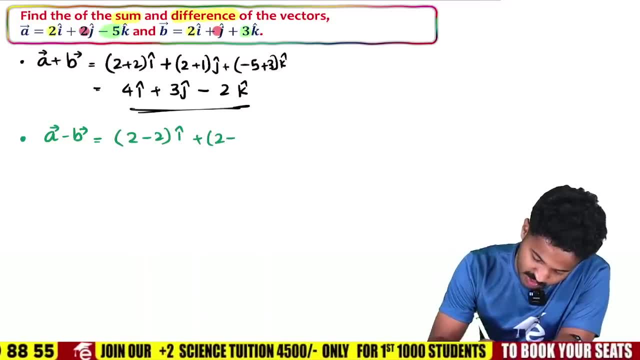 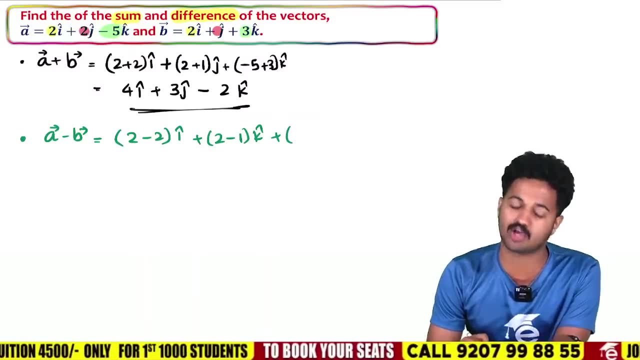 Plus Similarly j plus 2.. There j plus 1.. So 2 minus 1k Plus Everything. This is also a plus in the middle, Because it is a plus in the component form. Okay, Ready. 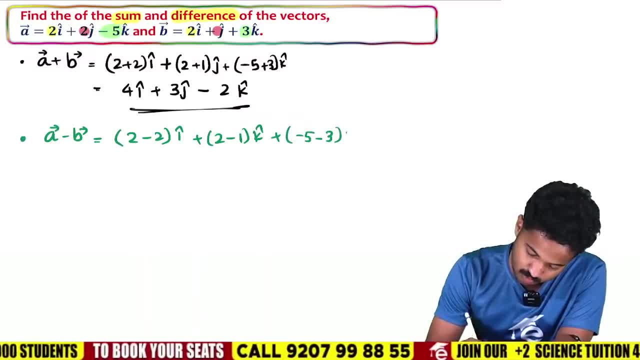 So here k equals minus 5.. Minus Here k equals 3.. Okay, So k See, 2 minus 2 is 0.. So 0i Plus 2 minus 1 is 1.. 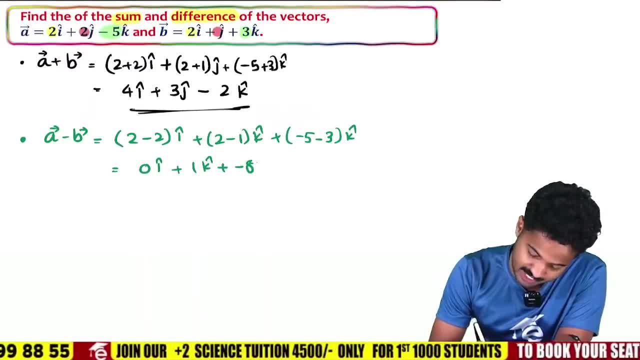 So 1k Plus Minus 5 minus 3. That is minus 8k. If we write it one more time, this is not the same. 1 into k is k Plus minus becomes minus, So minus. 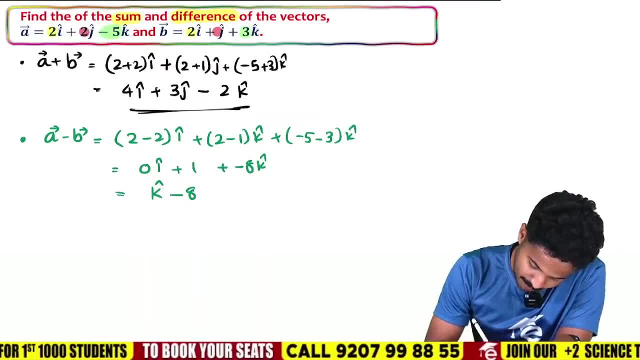 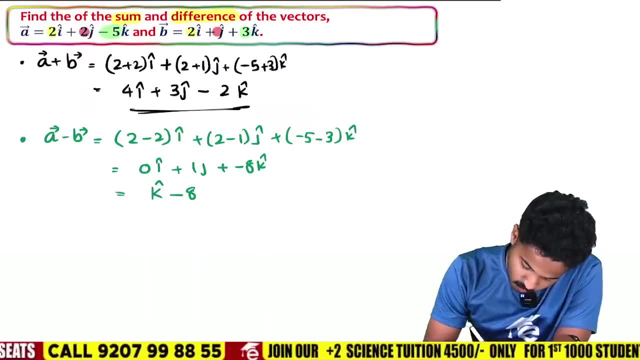 It's not j here, See See. So 1 into h i j It's not k here. Sorry, It's not k here, It's j See 1 into j. If we say 1 into j. 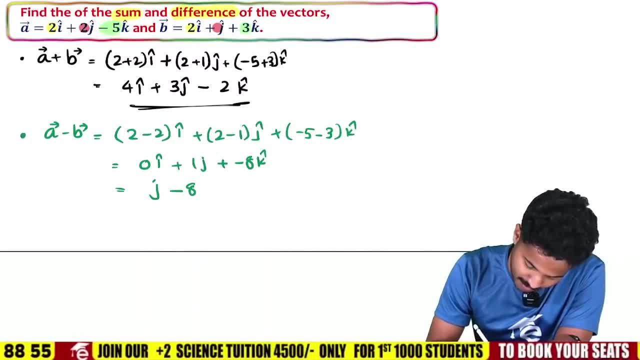 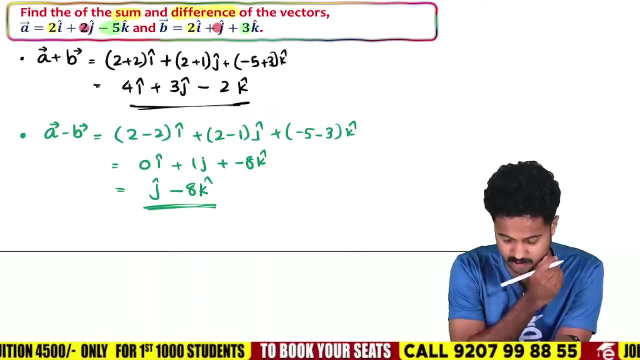 that is j right. So j cap minus 8k cap It's okay, right? If the answer is quickly okay, it's j right. Yes, It's j. It's j Sorry, Sorry, Sorry. 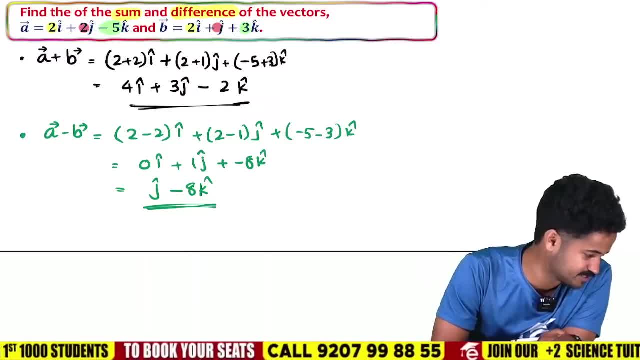 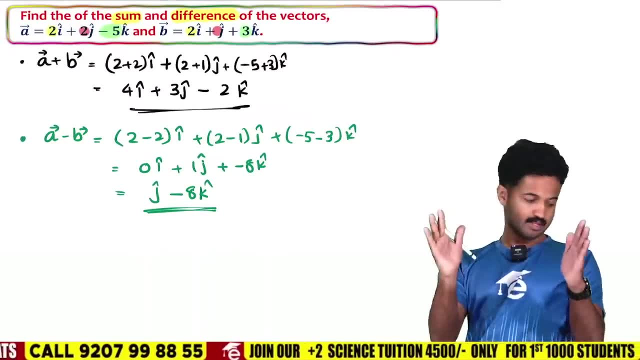 So ready. So that's it, It's easy Comment. Comment the answer: j minus 8k. Very good, Very good, There is no problem in giving 0.. The answer is easy, sir, Ready, Okay. 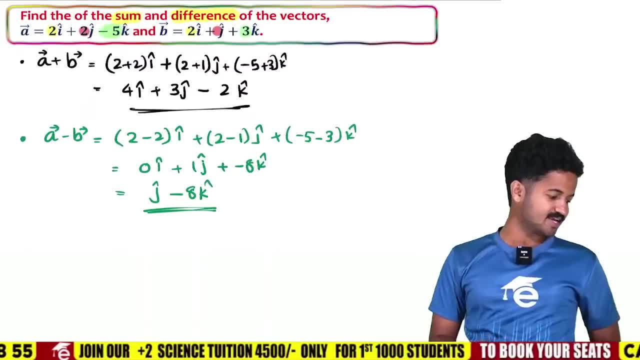 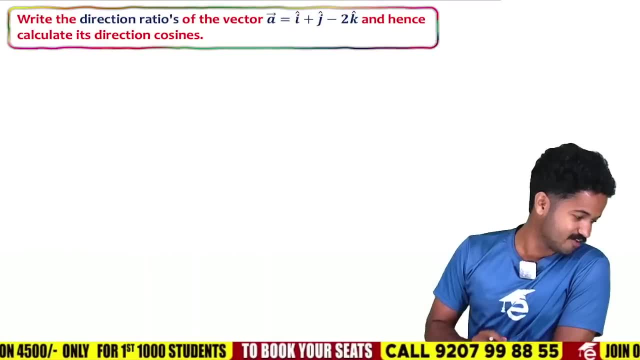 If you got it quickly, you will get green tea quickly. These are very simple things, Easy things, Easy, Easy, Ready, Ready. It's okay, right. All the questions in vector in the morning: Aiva, It's great, right. 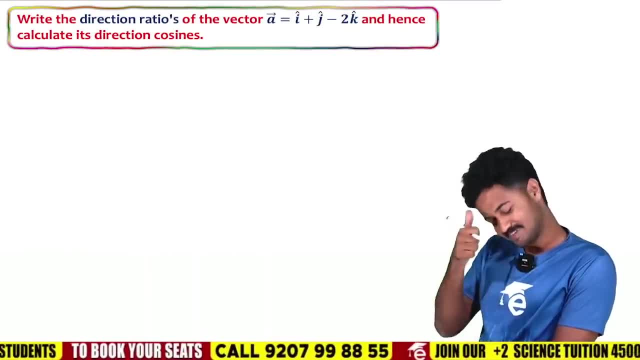 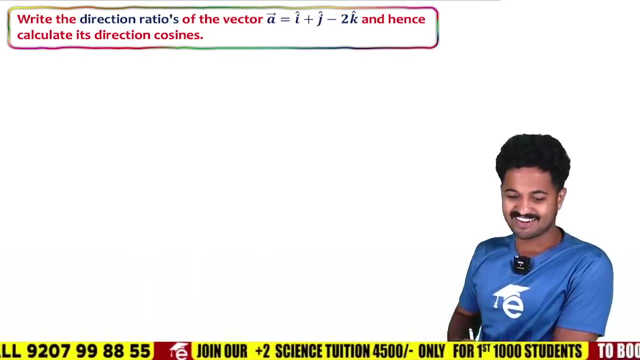 Almost 470 students are here in this live, Still in the morning. It's great, I liked it. Those of you who came in live, please like it. Those of you who came in live, please give me a like. Those of you who came in the morning. 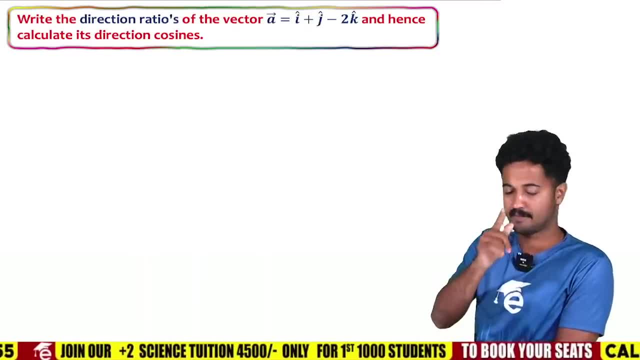 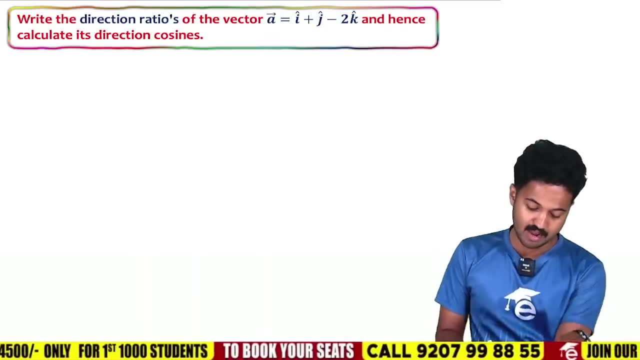 I came in the morning. Everyone, please like it. If you don't like it, please like it. Please minimize it. Please like it. How many likes for this poor young man? Let's see. So look Next. It's a very easy thing. 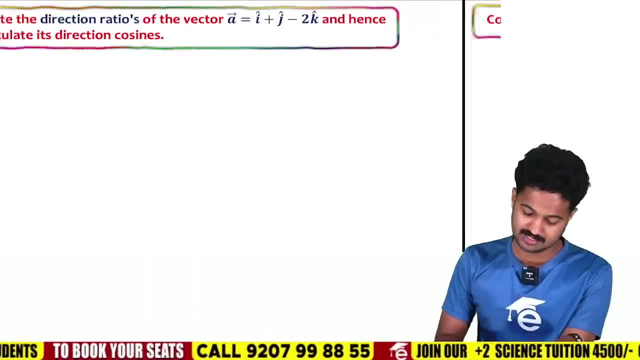 Direction Ratio. Direction Cosine Easy. You can do cancer easily. If you have given a vector, if its direction ratios are said, there is nothing called direction ratios. Do you know what direction ratios are The scalar components of that vector? 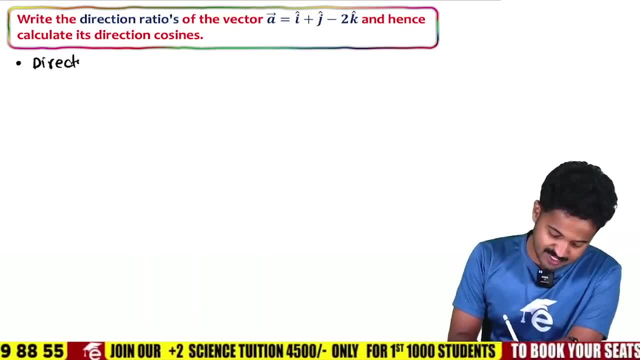 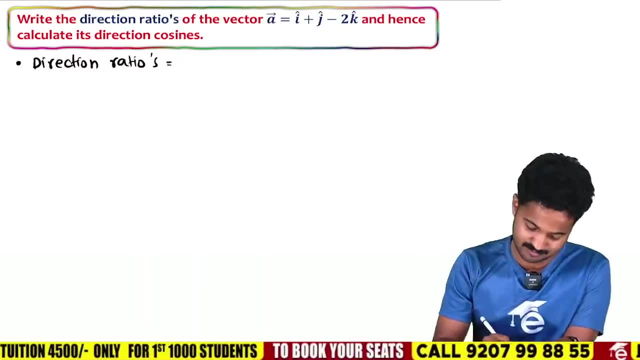 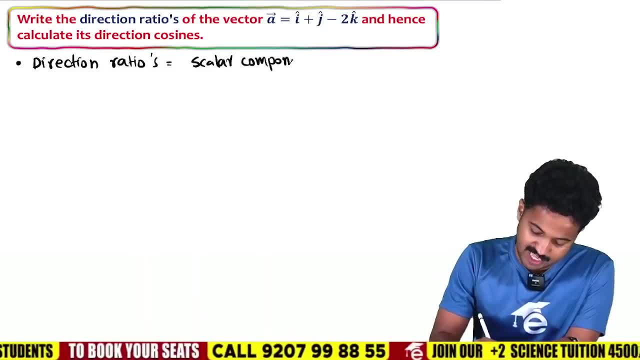 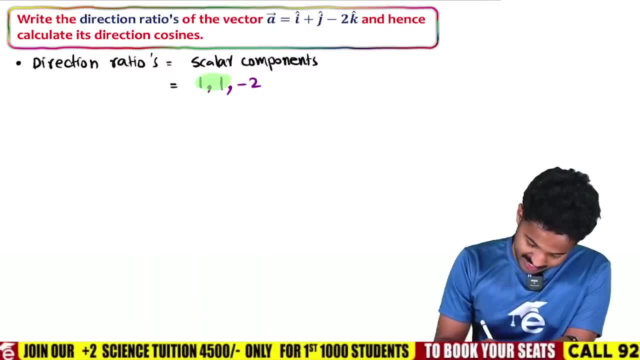 What if it's scalar components? It's greater than i and j. Here, it's greater than i and 1, the greater than j is equal to 1.. Okay, Ten over k is minus 2.. Then, If its direction ratios are: 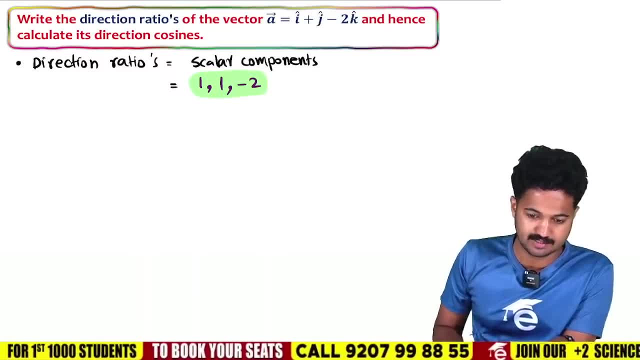 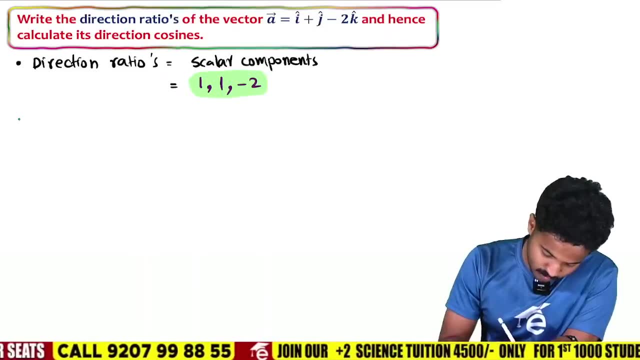 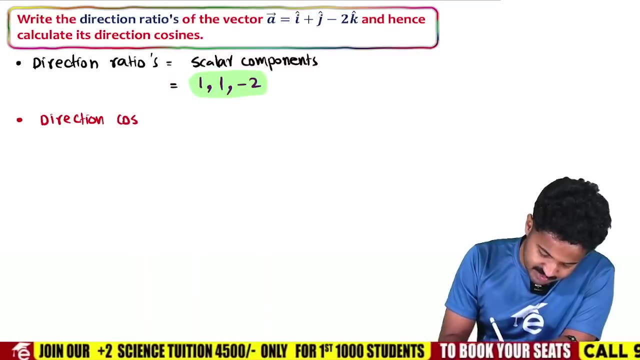 What is it? 1., 1. Minus 2.. Isn't it easy? There is no problem. Got it Simple Easy. PC Direction Cosines. Direction Cosines is very easy. The first thing you need to do is: 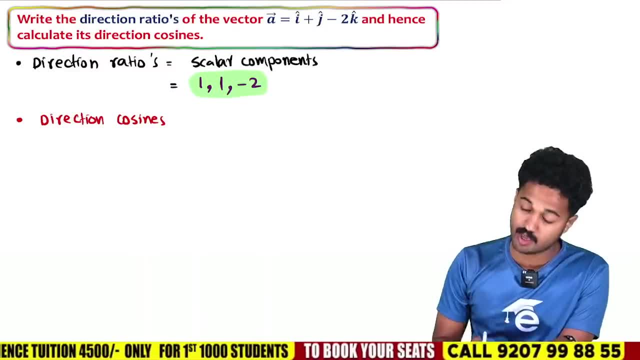 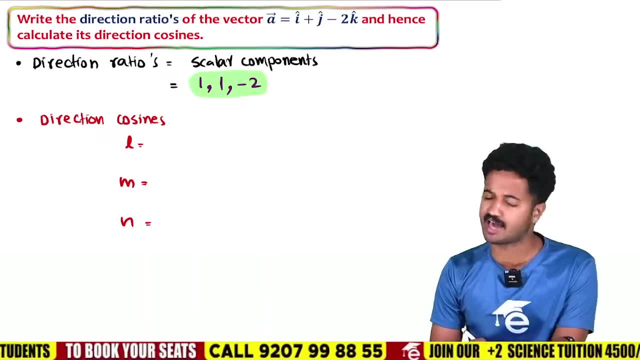 There are 3 Direction Cosines. Direction Ratio is 3, Direction Cosines is also 3, 1 is L, 2nd is M, 3rd is N. You need to know how to find these, The letters we give for Direction Ratios, xyz. 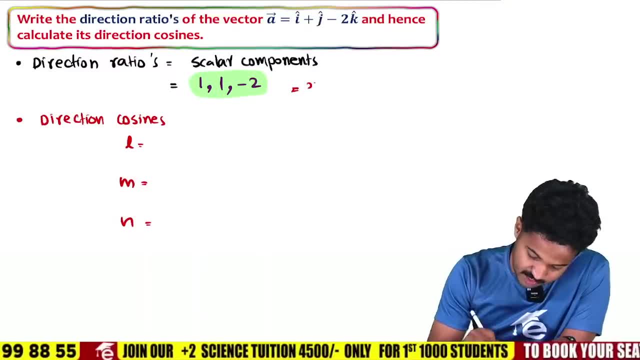 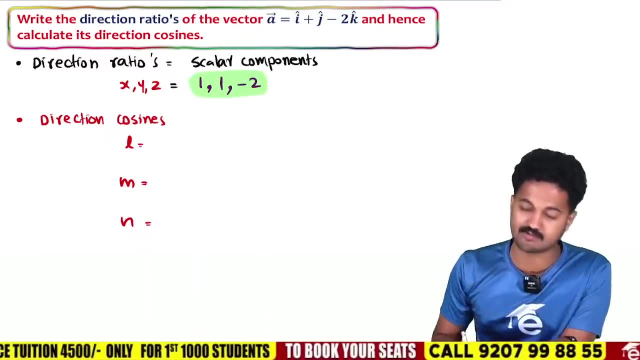 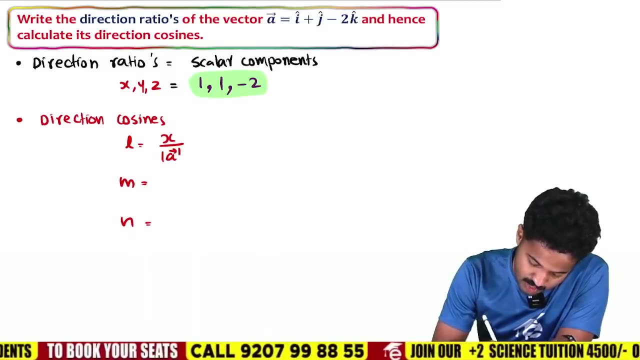 equal to xyz. Direction Ratios. You can give any letter. We always take xyz, xyz. Then how to find Direction Cosines x by the magnitude of the vector. y by the magnitude of the vector y. by the magnitude of the vector. one more person is there. 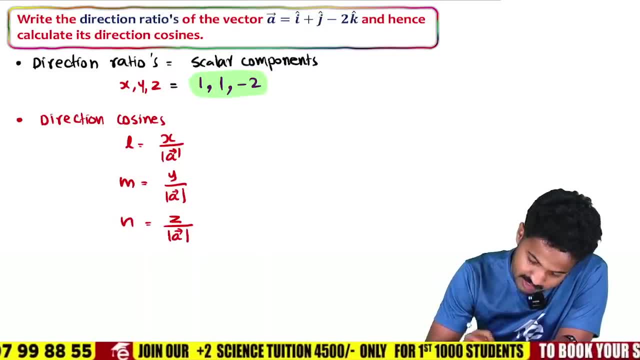 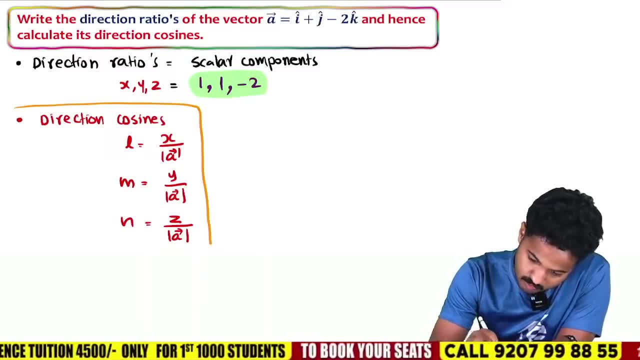 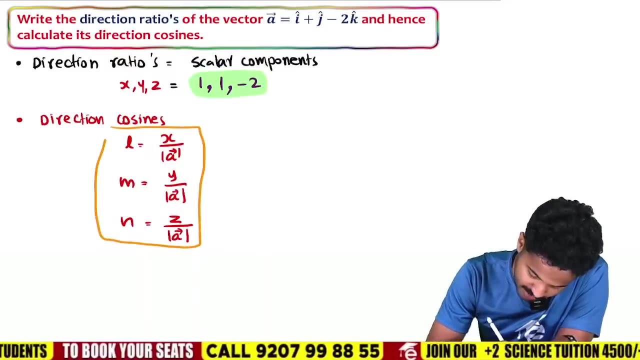 z by the magnitude of the vector. So this is what we do. Direction Cosines is the equation used to find Direction Cosines. Direction Cosines is used to find Direction Cosines. This equation is very easy To understand. Then, what about Magnitude of multifactorial u? 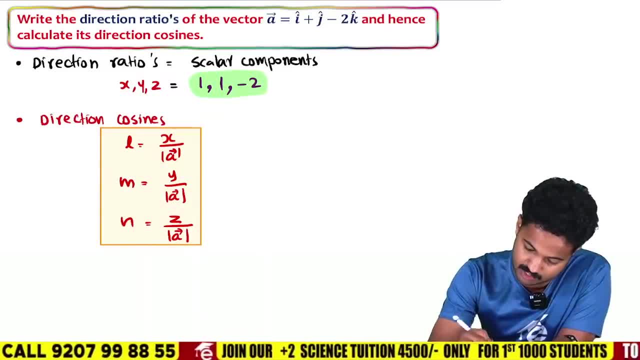 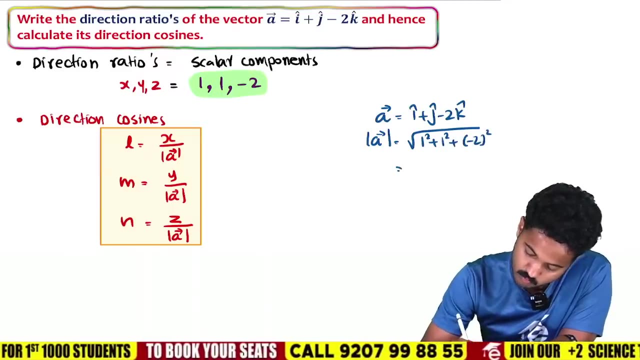 Yes, mine. Then If we try to find the magnitude of u, Magnitude of A, If we take the myself I plus J minus 2, What is the magnitude of that vector? A is thousand. it means 1 square plus 1 square times minus 2, all square. 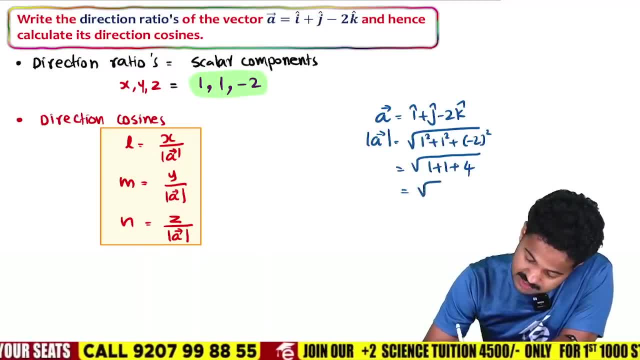 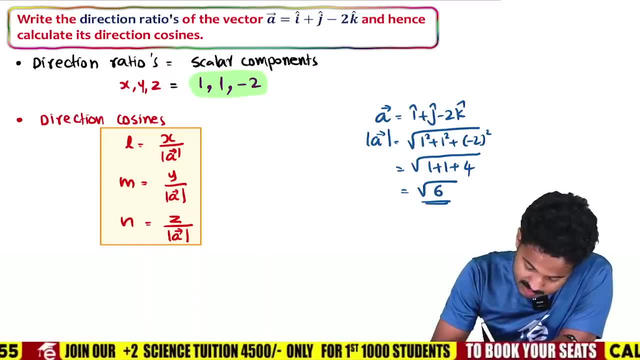 which means So your magnitude will be root 6.. So if you look at it, you are going to get each answer here. If L is said, X by X means 1.. So 1 by root 6.. 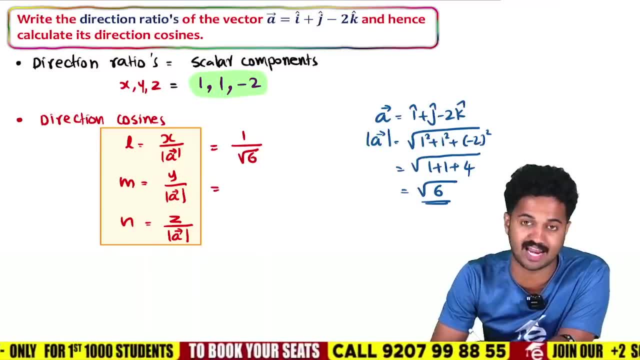 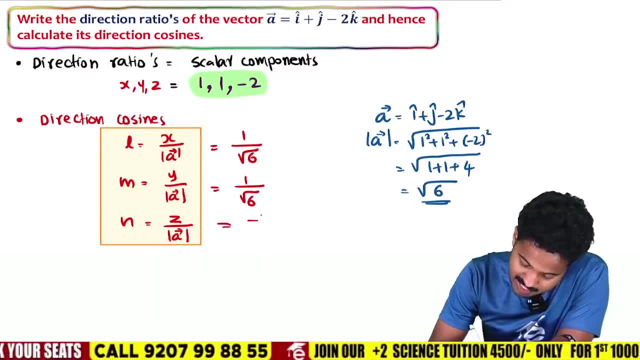 If M is said Y by root 8.. So if you look at it, magnitude is root 6, 1 by root 6.. Y and 1. And Z is minus 2, so minus 2 by root 6.. 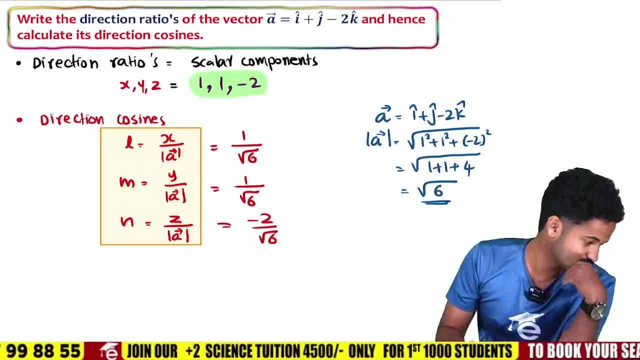 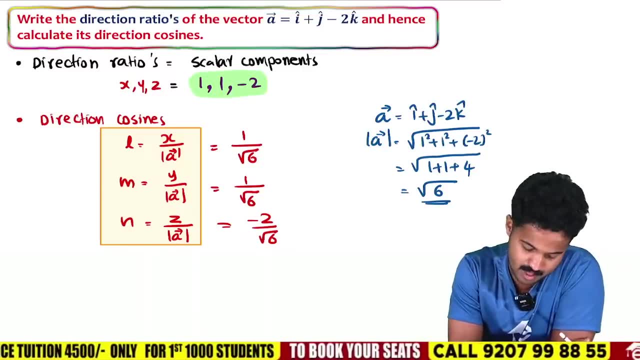 This is your direction, cosines. Yes, got it. Got it. Simple, Easy, isn't it, Sir? this is easy, This is easy, No problem. It's okay, isn't it? It's okay, isn't it? 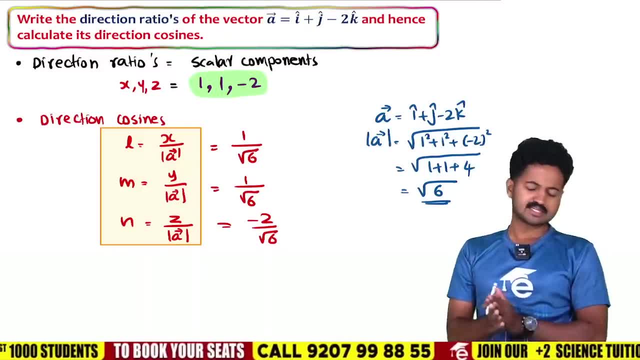 Tell me quickly Those who got it quickly. give me a tick, Give me a tick. Give me a tick quickly. 1 by root 6, 1 by root 6, minus 2 by root 6.. So direction ratios. 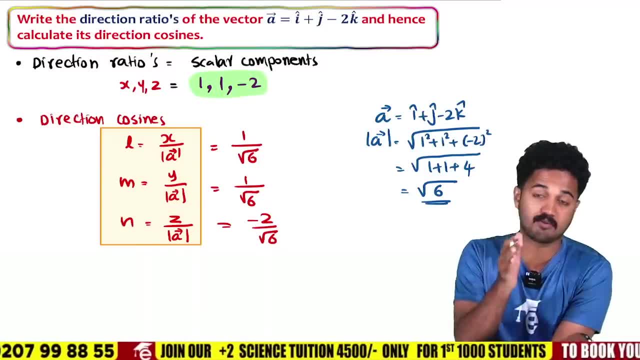 If you have given direction ratios, you have to learn to do a vector. Similarly, if you have got direction ratios, you have to learn to do direction cosines. Easy, isn't it? So 1 and 1 are minus 2.. 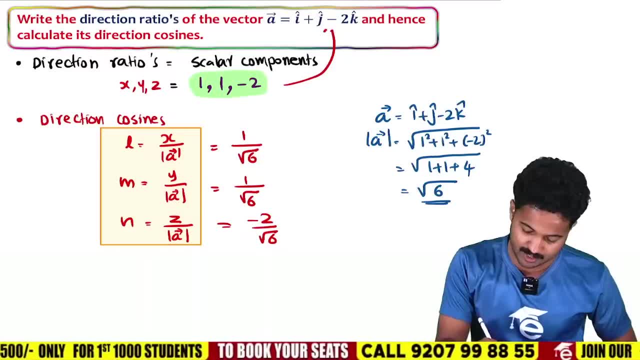 If it's direction ratios, that vector is 1.. How do you do a vector like this: i plus j minus 2k, Easy, No problem, right, Okay, it's ready. Okay, sir. So that's how you look at it. 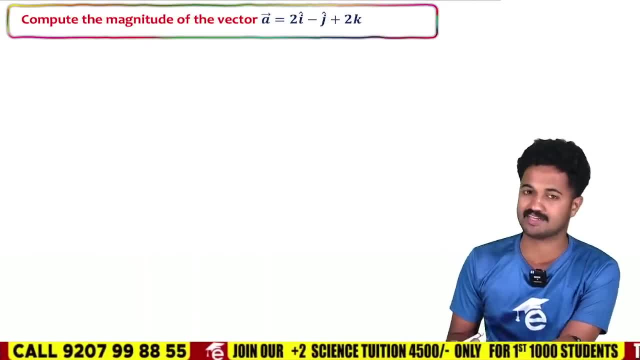 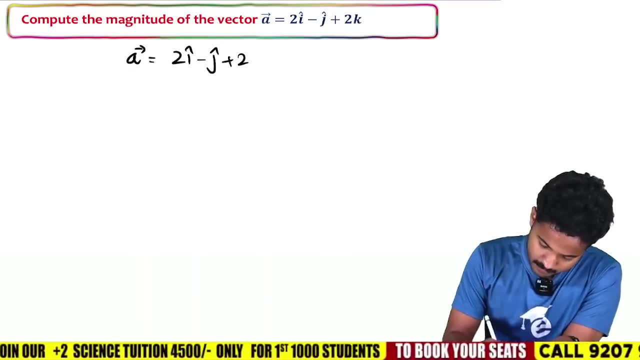 Compute the magnitude of the vector. So far we have talked about magnitude. How do you find the magnitude of this vector? The vector called a is 2i minus j plus 2k. Sir, what is its magnitude? How do we find its magnitude? 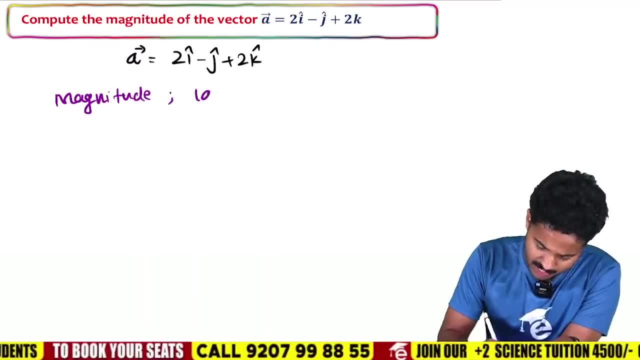 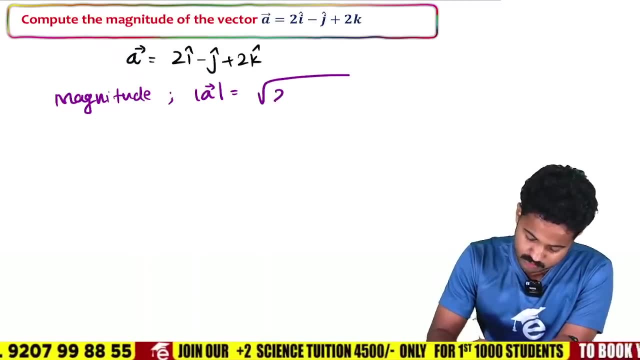 It's easy to find magnitude. It's easy to find magnitude. So far, we have talked about magnitude, right, Magnitude of a equals. Oh, we have crossed 500.. Thank you. So look at this Root of 2 square plus minus 1 square plus 2 square. 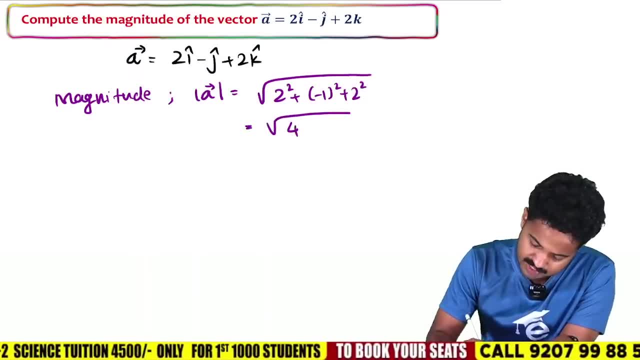 This is easy. So 2 square is 4.. Minus 1 square is 1.. 2 square is 4.. So the final answer is: 4 plus 1 is 5.. 5 plus 4 is 9.. 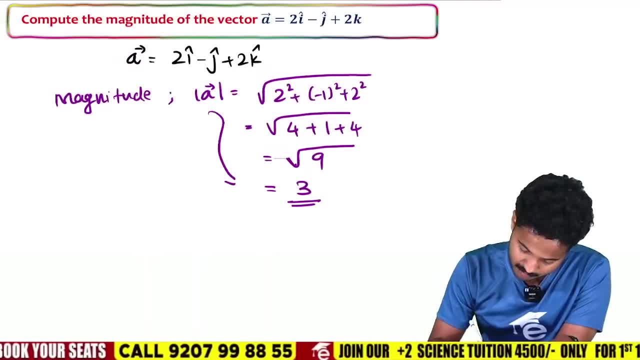 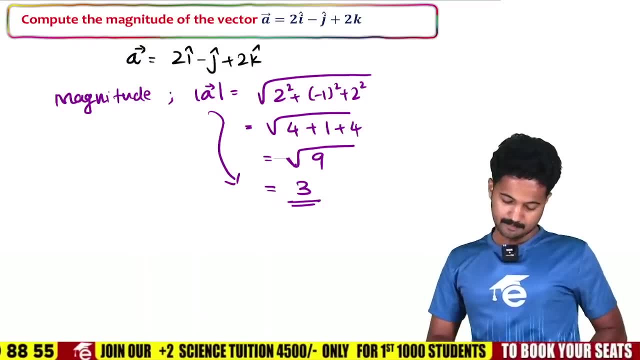 So the root of 9 is this, Root 3.. So what is the magnitude of this? 3.. Very good, Everyone has said that the magnitude of this is 3.. Easy, It's easy, There is no problem. 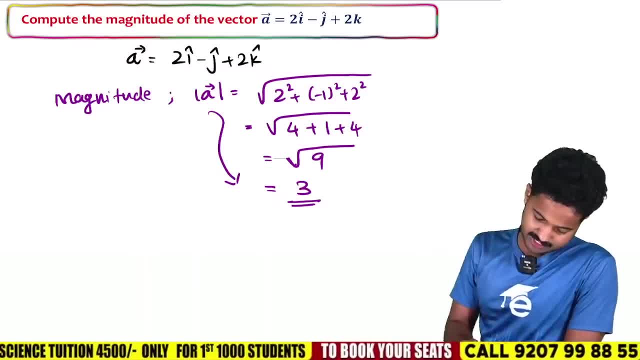 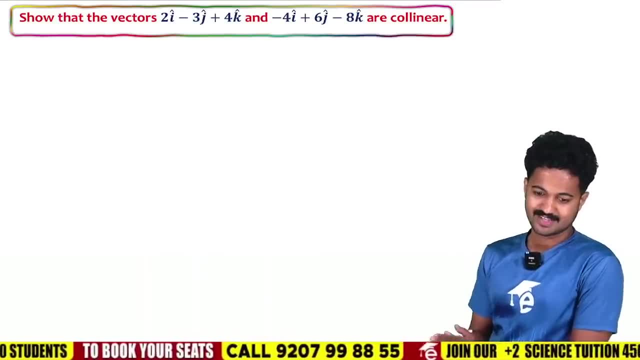 Okay, Okay, Ready, Ready. Did you get the ticket? Did you get the ticket? Did you get the ticket? Comment the answer quickly. Comment the answer quickly. Okay, Okay, Simple, Easy. Look at the next question, sir. 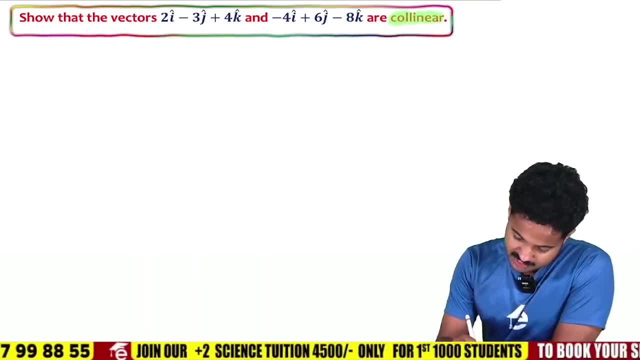 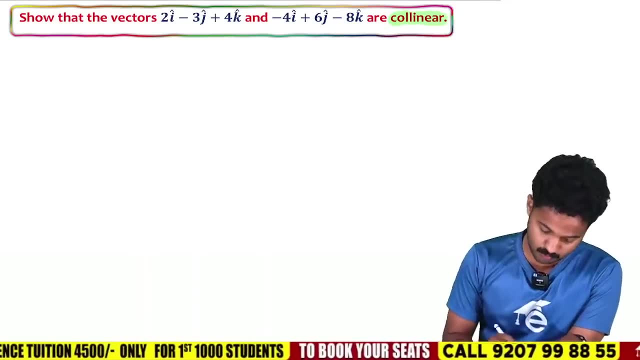 The next question, sir, This is also easy: Show the vector, Show the vectors. There are two vectors. They are collinear. If two vectors are collinear, you have to do this much, That is, look at this: The vector A is X1, I plus X2, J plus. 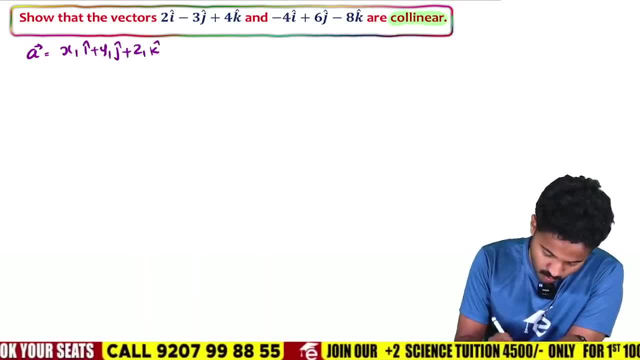 or X1, I plus Y1, J plus Z1, K. Think of it like this: The vector B is X2, I plus Y2, J plus Z2, K. Think of it like this: 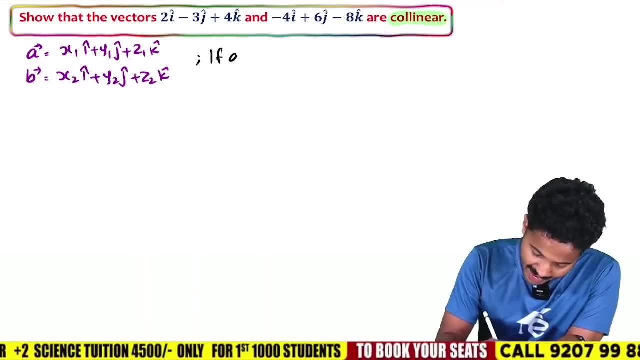 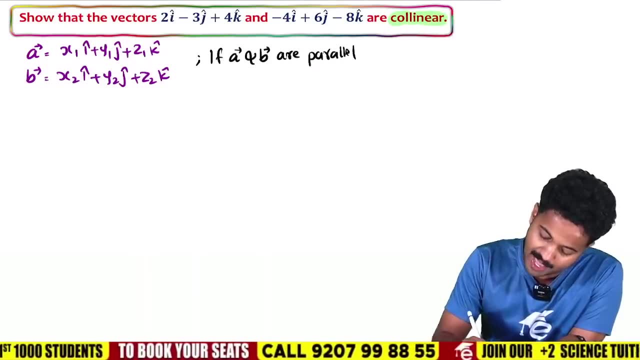 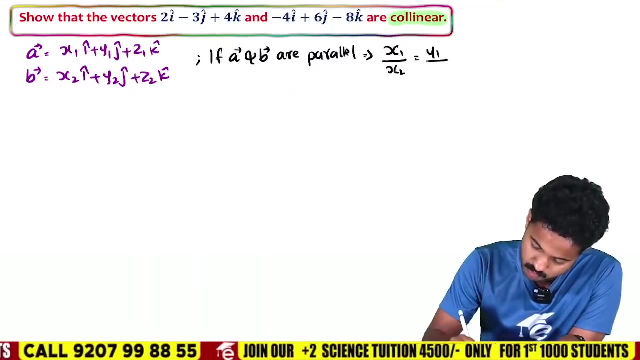 Okay, Now, this is it. That's it. If A and B are parallel. if A and B are parallel, remember two conditions. If A and B are parallel, you write this much. This much is enough. X2 is equal to Y1 by Y2 is equal to Z1 by Z2.. 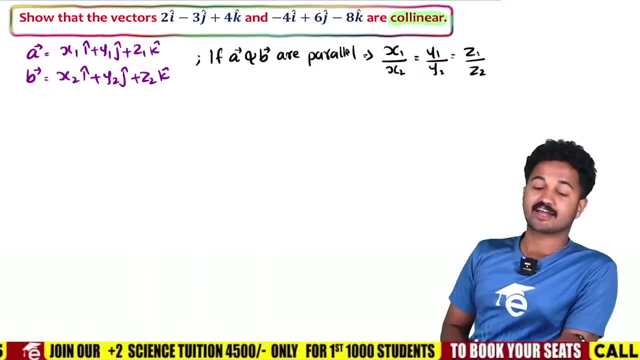 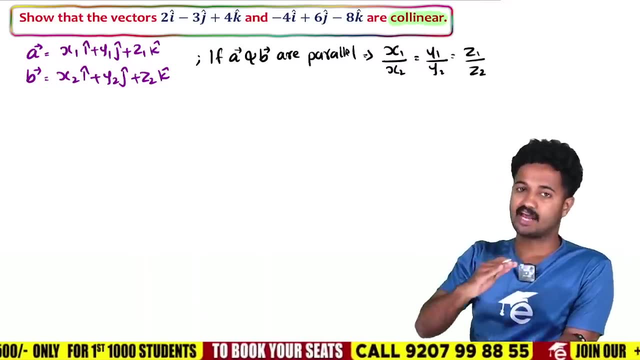 Think of this. Think of this: If two vectors are parallel, you can take the scalar components I and I. The first is by the second. Now, the component of J is by the second, The component of K is by the second. 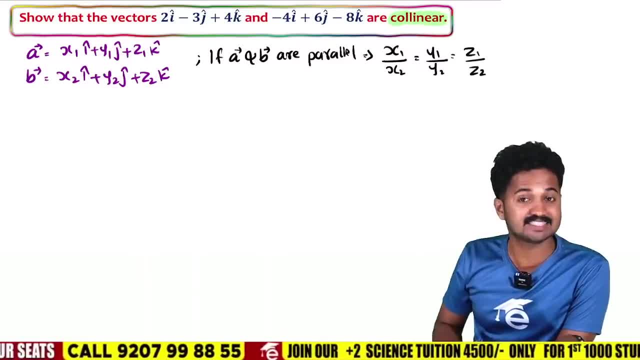 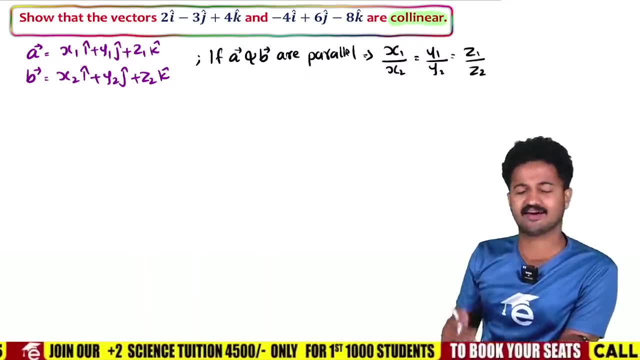 If you take that, the answer you are about to get will be the same. The ratio will be the same. If the ratio is the same, then the vector is parallel. Now, that is not the case. You can write it in another way. 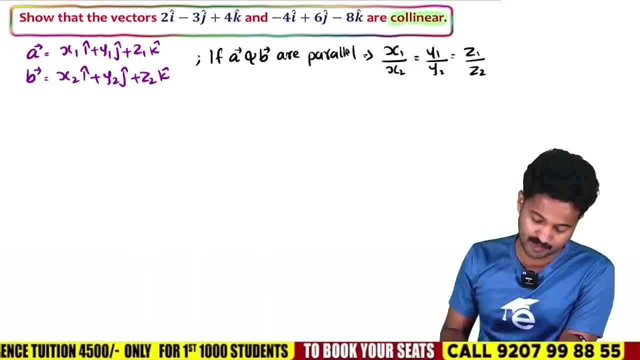 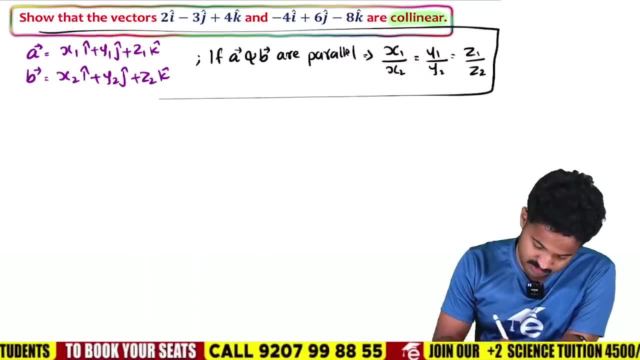 If the two vectors are parallel, you can write A equal to lambda B, Or you can write lambda equal to A B. So the first is like this: You can write it like this. There is no problem. This is the first. 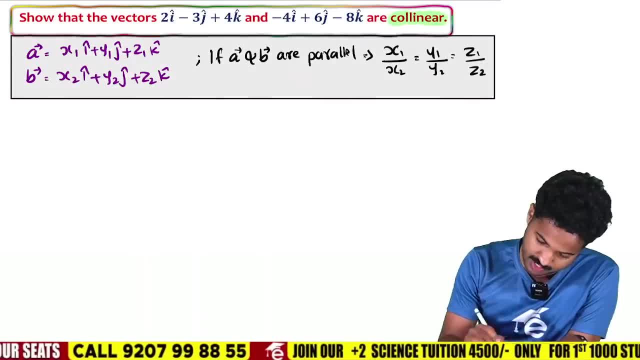 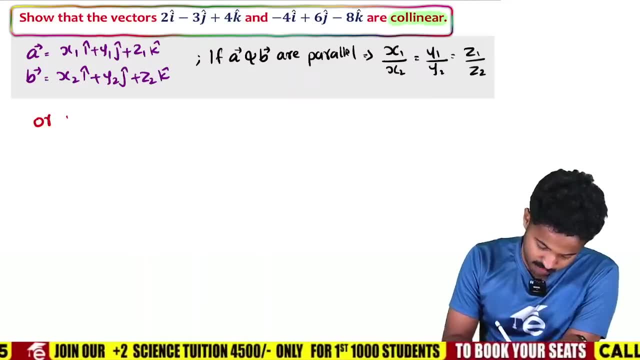 There is no problem for you to write it like this. Okay, You can write it like this: No issue. Or, or, or. Or. you can write it like this: Or if A and B are parallel. if A and B are parallel. 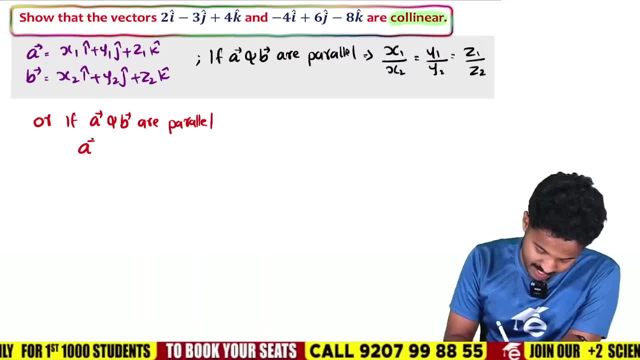 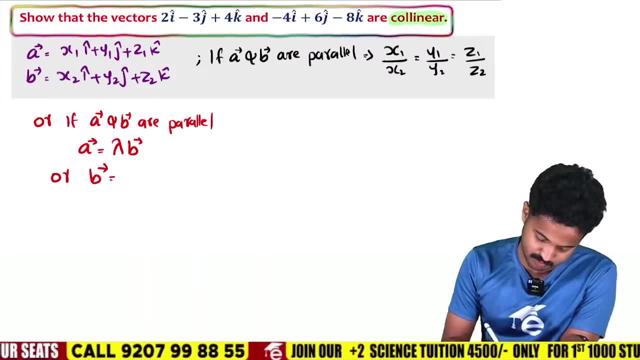 then if A and B are parallel, you can write it like this: A equal to lambda B. That is, if you multiply the vector called B with any constant, what will you get? You will get the vector called A Or B equal to lambda A. 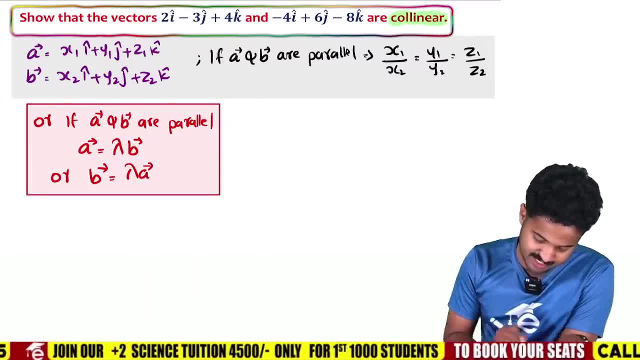 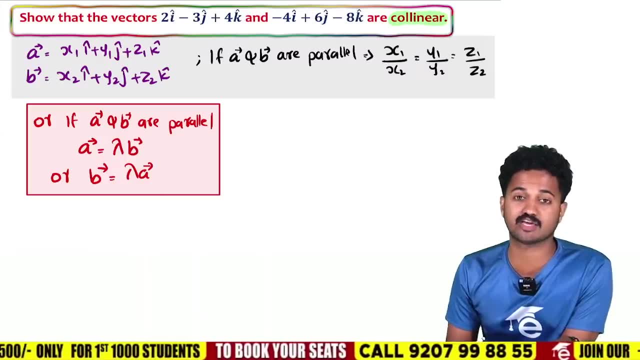 You can write it like this: So if the two vectors are parallel, the condition is like this: There is no problem in writing these two. You will get the answer anyhow. Okay, It is easy. Here you can check if everything you get is equal. 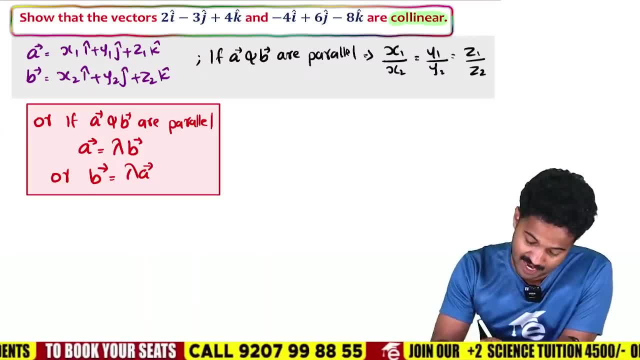 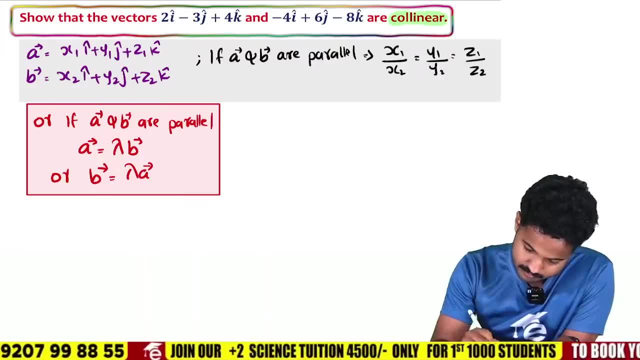 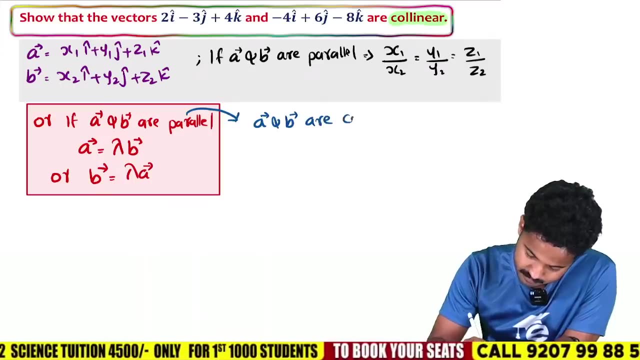 If it is parallel, it will be collinear. If it is parallel, then collinear. If it is parallel, then what will it be? It will be collinear. Okay, There is no problem. If it is parallel. A and B are collinear. 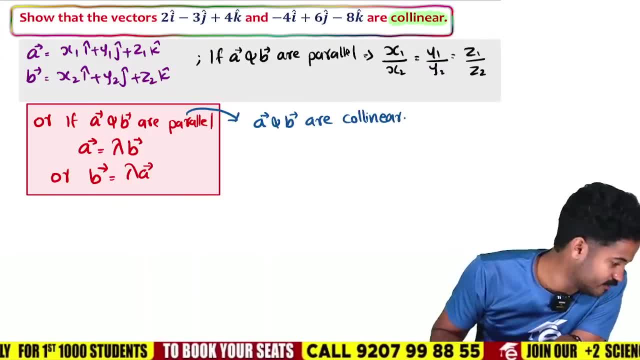 If it is parallel then it will be collinear. So you check: Is it correct here? Check: Is it correct here? 2A equal to B. Yes, Very good, Is it correct here? Minus 1 by 2, 1 by 2, 1 by 2.. 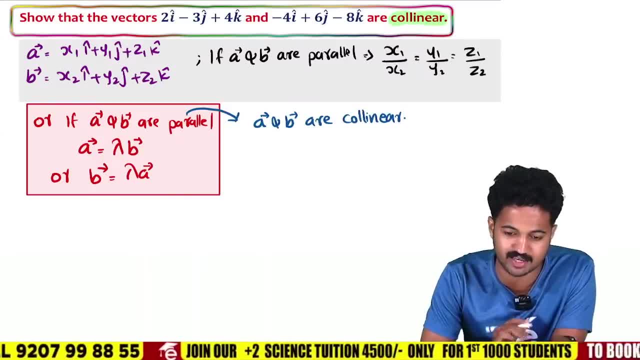 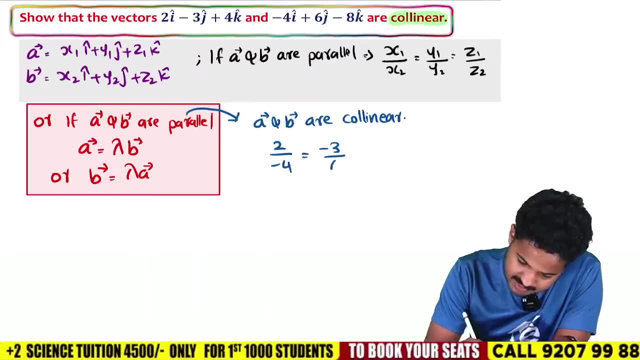 Minus 1 by 2.. You will get it everywhere Ready. Check if it is correct. Check if it is correct. Look It is with I: 2 by minus 4, equal to minus 3 by 6, equal to 4 by minus 8.. 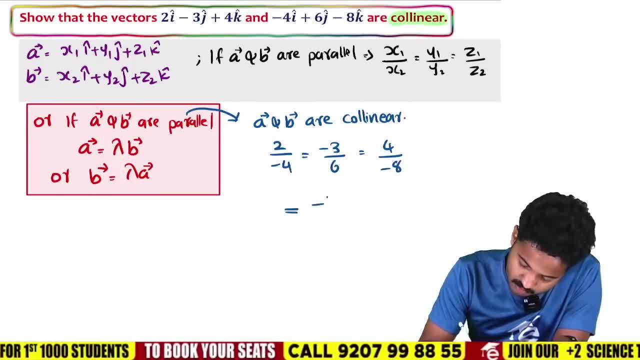 What will you get if you do everything? 2 by minus 4 is minus 1 by 2.. Minus 3 by 6 is also minus 1 by 2.. 4 by minus 8 is also minus 1 by 2.. 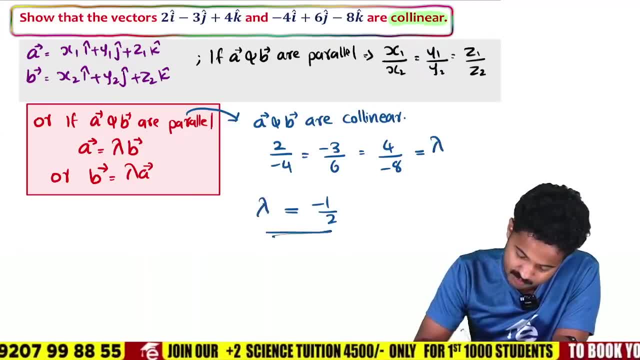 You can write equal to lambda. How much is lambda Minus 1 by 2.. Everything will be a constant. You just have to check if that constant is the same. So. So What should our answer be? So There? 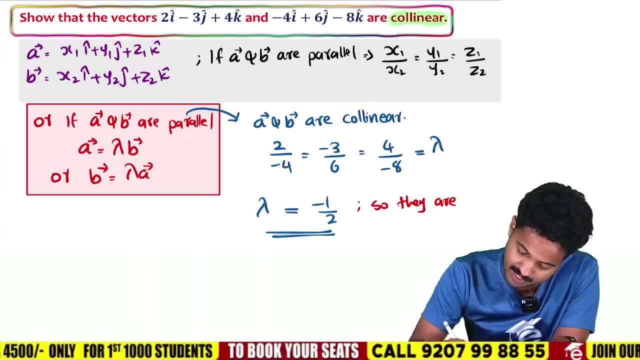 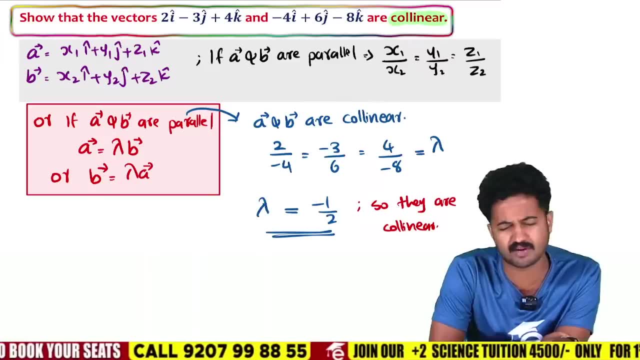 You have got your randomthest examples. Take this There. So what is B? It is here Here, So you do and you write Here Here. Thank you, Yes, And the answer is sin squared. It is not sin squared. 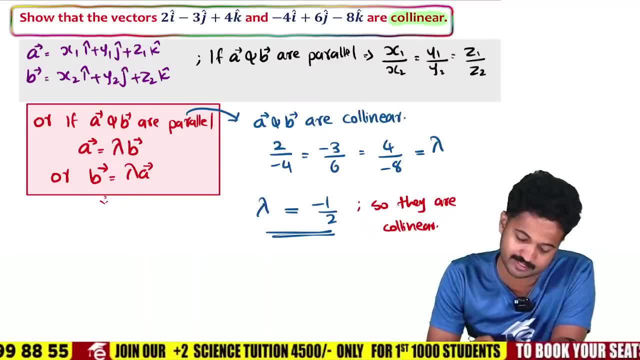 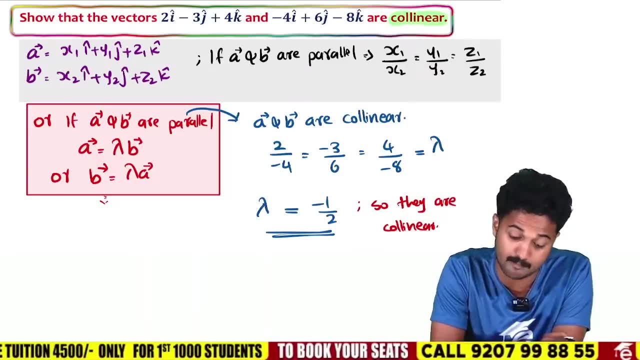 It is not a定 quantum. It is de tão Crown in kommtiback E uno selber Bullet держa E uno transfers Emus the information to Pl Worlds. here You transfer the information to Pl 12. If you do that, your answer will be correct. 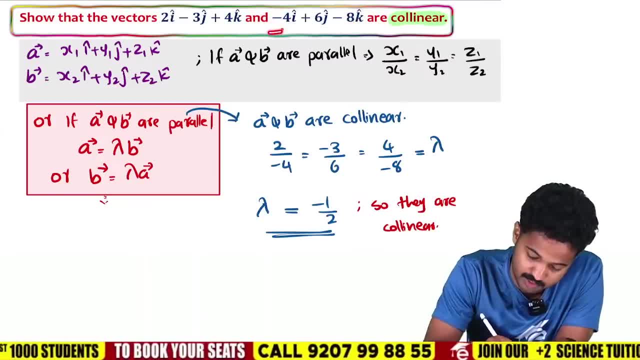 So there is no problem in doing Confencent is also Brownian, Confencent is alsoしか minus 2, we get 2i plus 6j, sorry 3j, If we take 2 common. if we take minus 2 common, we get 2i minus 3j plus 4k. 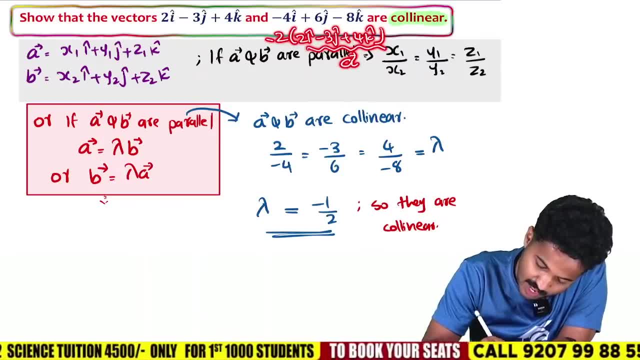 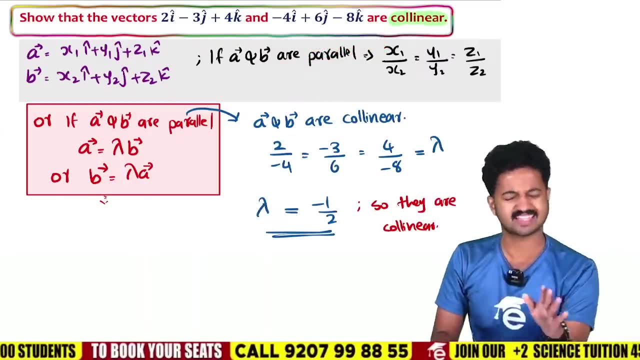 So look what is this. This is the vector a, So you can write the vector b as minus 2a. Even if you write it like this, there is no problem. That's it. Just do that, It's easy. There is no problem. 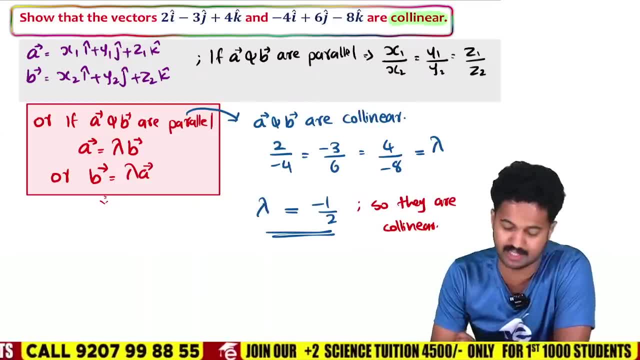 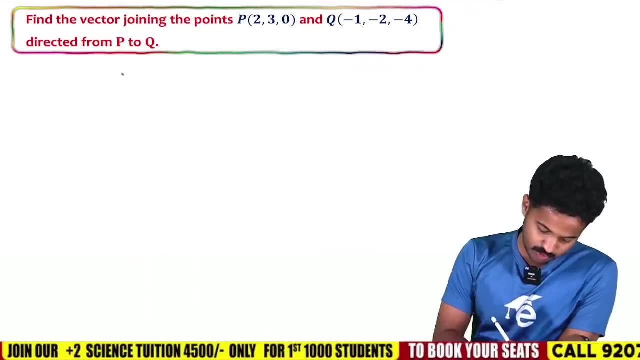 So the ratio is equal. No issue, So they are collinear and parallel. Okay, Next, when two vectors join, pay attention: P and Q have two points. P and Q have two points. P and Q have two points. This is P and this is Q. 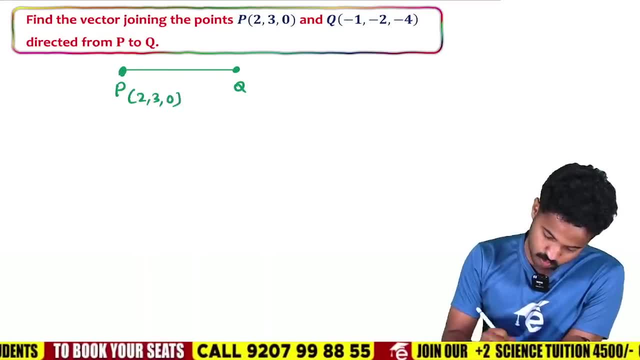 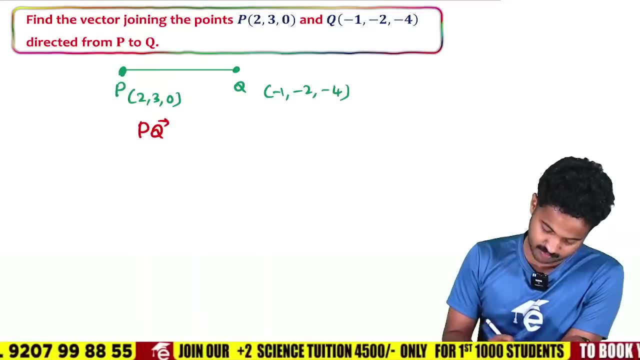 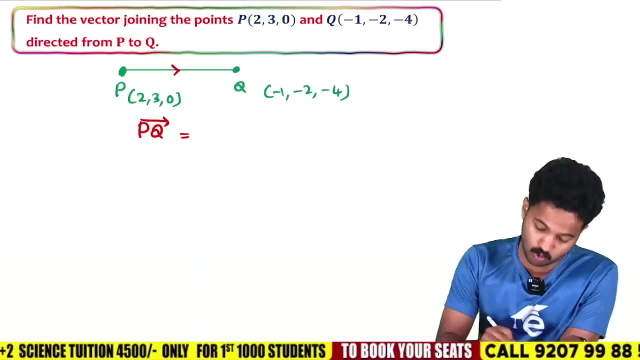 If you are told that the coordinates of this is 2,, 3,, 0,, this is minus 1,, minus 2,, minus 4, then what is PQ? What happens to the vector PQ? So the vector that goes from P to Q is PQ. So how do you find PQ? There is nothing. 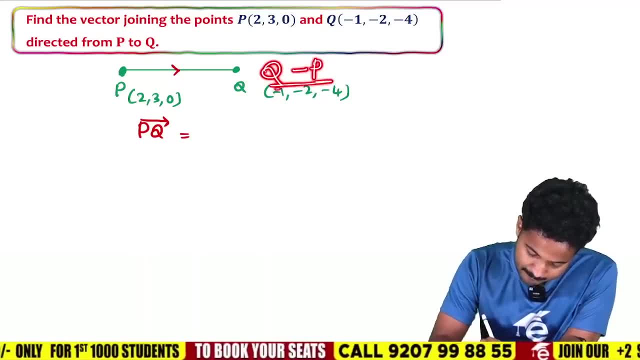 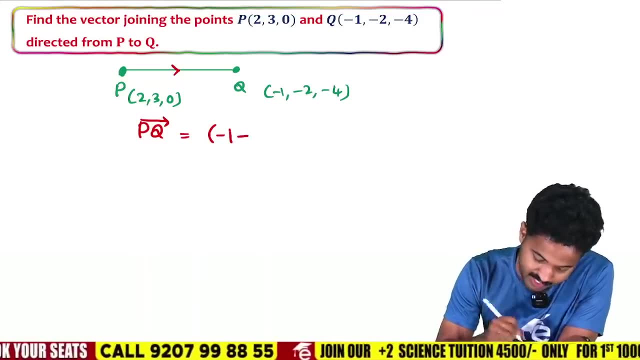 Here. what do you do from Q, P minus E? Simple, Easy. So how do you find this Here? the first one is Q and that is minus 1.. That minus 1 minus the first one over P is 2, i cap plus. 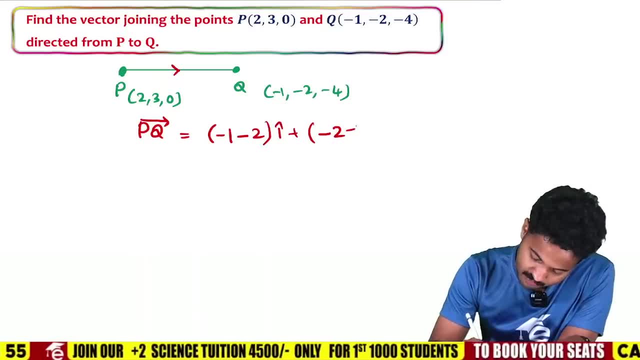 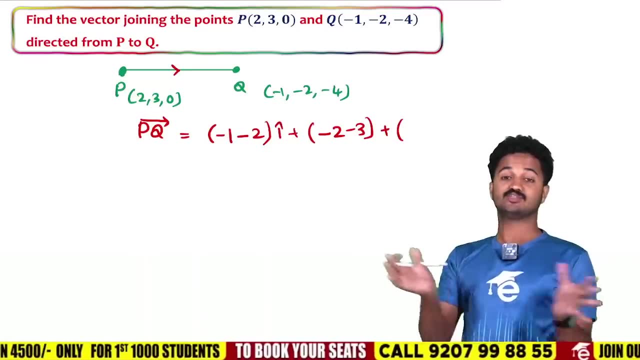 The second one, j, has to come over Q and over P minus 2 and over P minus 3.. This is minus E Plus. This is all you have to do. You have to give two points If you are told to find the vector that joins them. the second point is minus the first point. 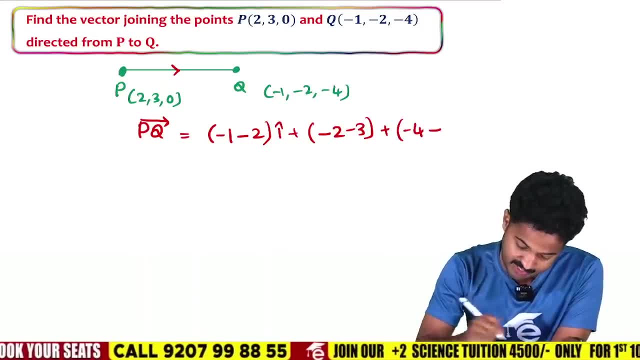 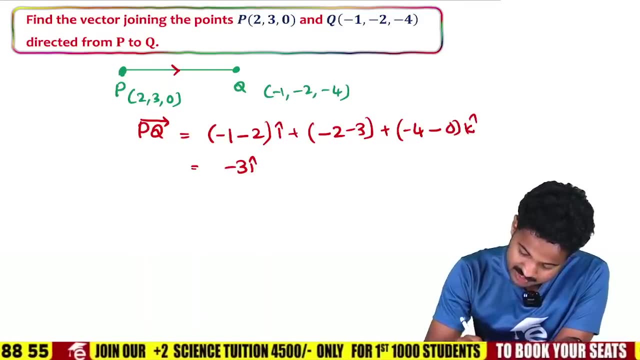 If it is corresponding, you just have to do minus. What is this? Minus 4 minus 0, k cap. Answer is minus 1 minus 2 is minus 3, so it is minus 3.. Minus 2 minus 3 is minus 5, so it is minus 5, k cap. 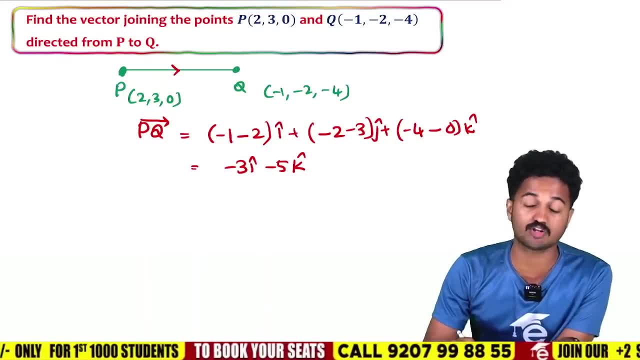 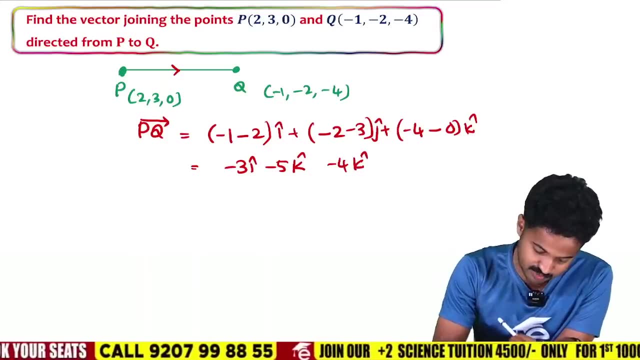 Plus is there. Plus and minus are minus Minus 4 minus 0 is minus 4.. So you don't have to put plus minus 4.. No, it is not. You don't have to put minus, You just have to put minus. So it is minus 4k. 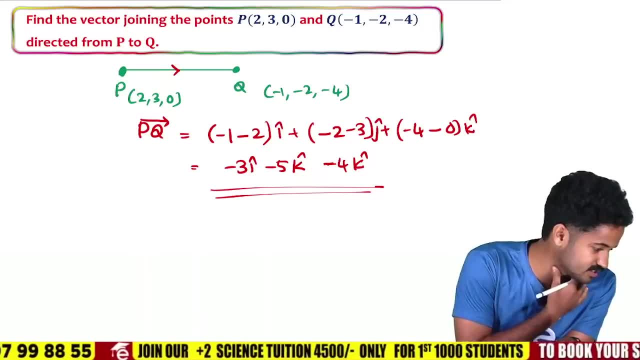 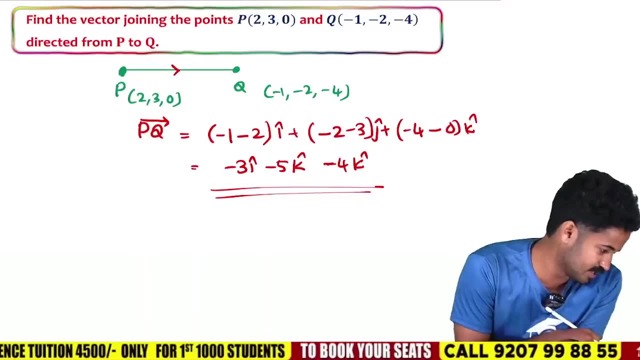 This is how you do two vectors. Yes, Yes, Yes, Yes, Okay. Minus 3,, minus 5,, minus 4.. Okay, Ready, Simple, Easy. This is how you do two vectors. Now let me ask you a question: What is QP? 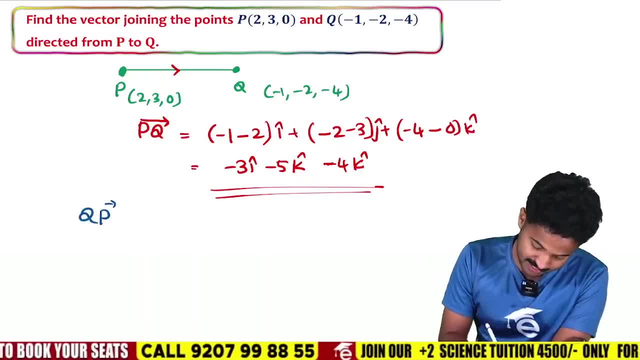 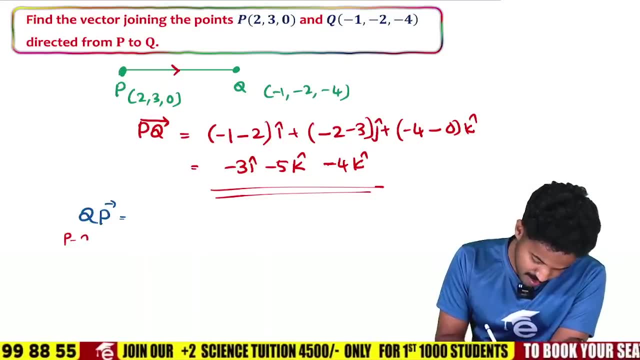 If you are asking this with your head turned, what do you know about QP, QP, QP? If it is QP, you have to do minus. You have to do minus. I will tell you the side. No one will see it. 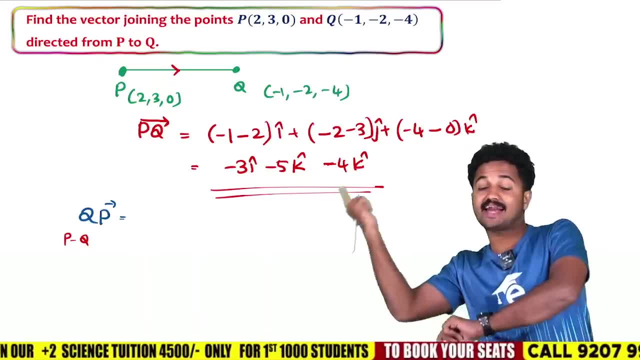 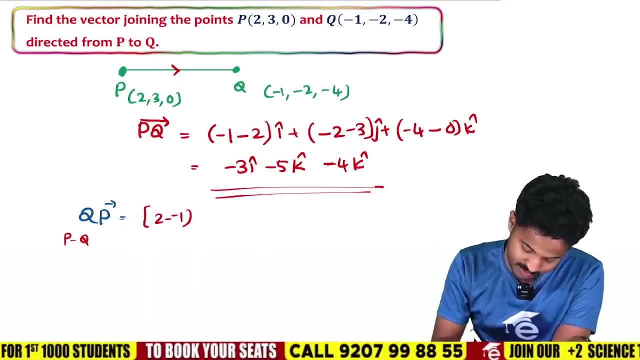 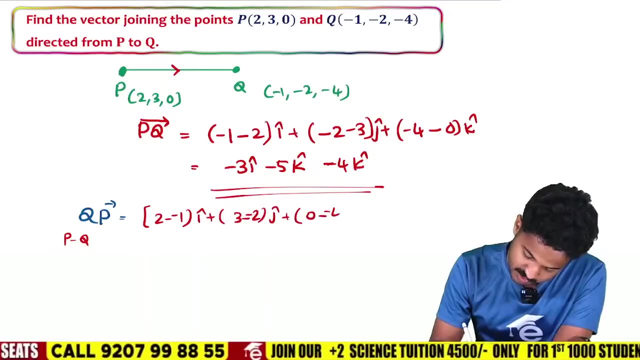 Yes, Q is minus from P. QP is not the second one, Q is minus from P. So how does it come here? How does it come here? Look: 2 minus minus 1i plus 3 minus minus 2j plus 0 minus minus 4k. 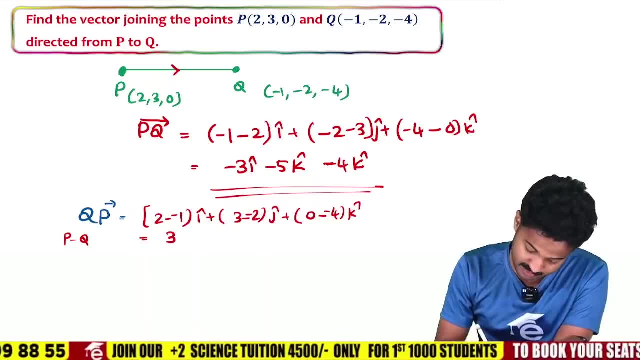 That is the answer. comes this much: 2 minus minus 1 is 3.. So 3i plus 3 plus 2 is 5j. 0 minus minus 4 is 4.. That is 4k. 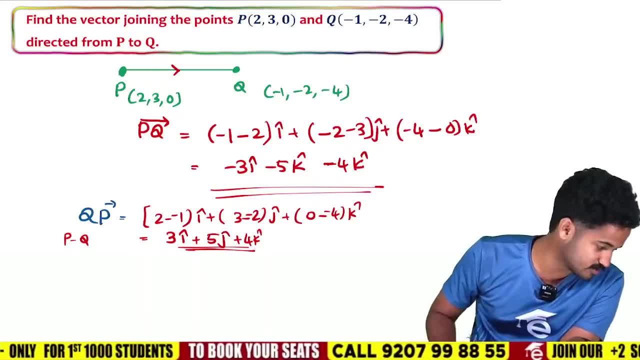 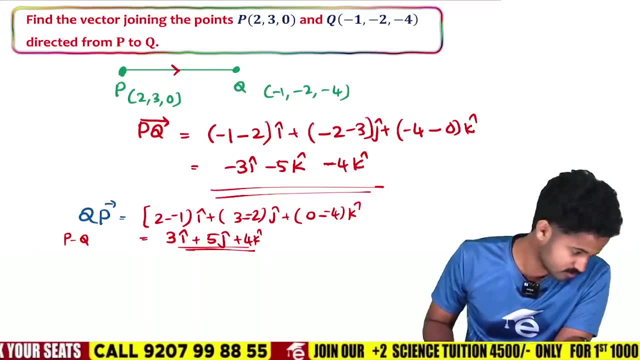 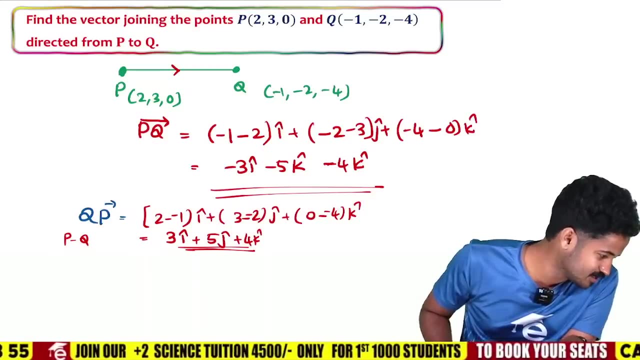 This is how it comes. Did you understand the difference, Sir? it is not minus 5k. It is not minus 5k. It is not minus 5k, Sir. I am missing the board. It is not minus 5k. 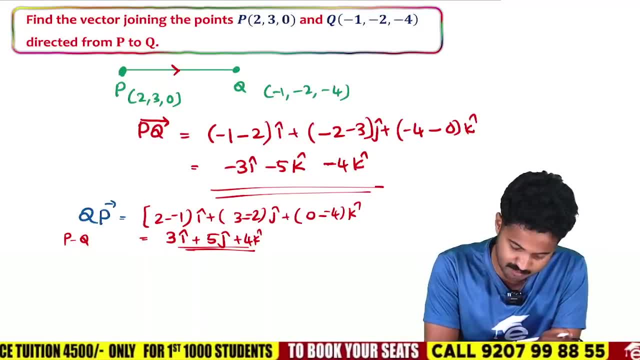 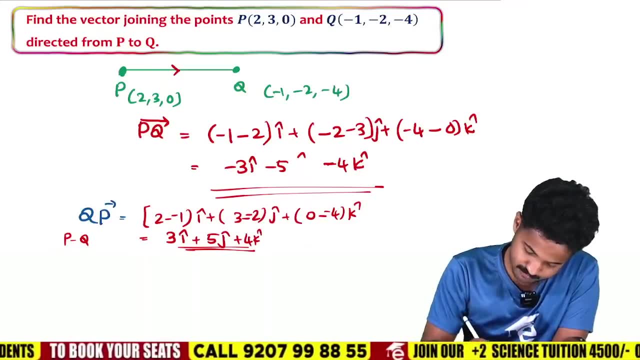 It is not minus 5k. It is minus 2, minus 3.. It is minus 5.. It is not minus 5k. I have put j Okay, Yes, Yes, That is good. Yes, It is minus 5j. Okay, Sorry. 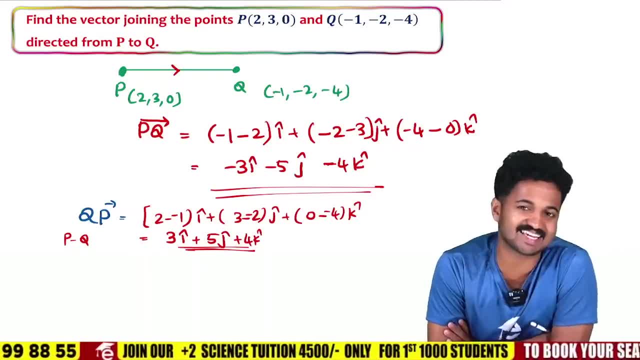 Okay, I understood. I understood. It is not k. It is j, Okay Ready. I forgot k earlier. k and j are different. Shamil sir, Okay Ready, So ready Children. did you understand the thing? 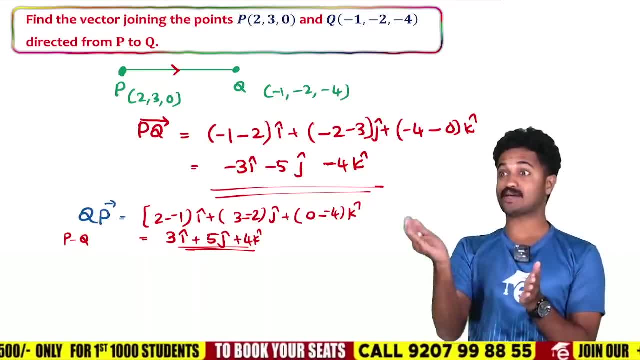 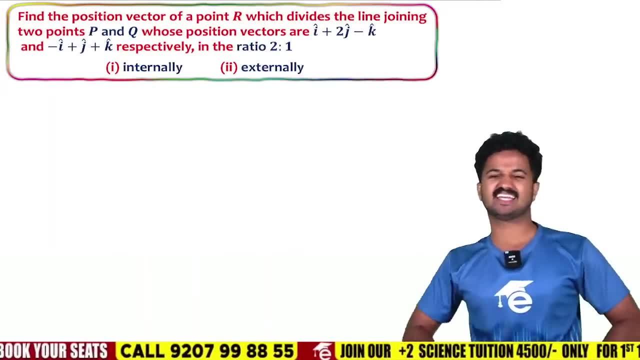 So one vector, Q is minus from P, QP is minus from Q. That is it Ready, Okay, sir? Simple, Easy. Next look: Internal and external division. Sir, how to do this? Easy, No problem, Simple. 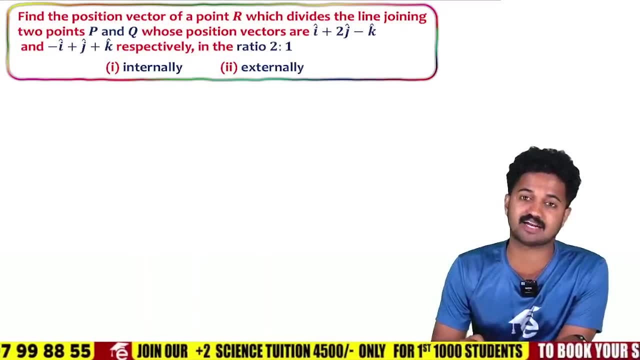 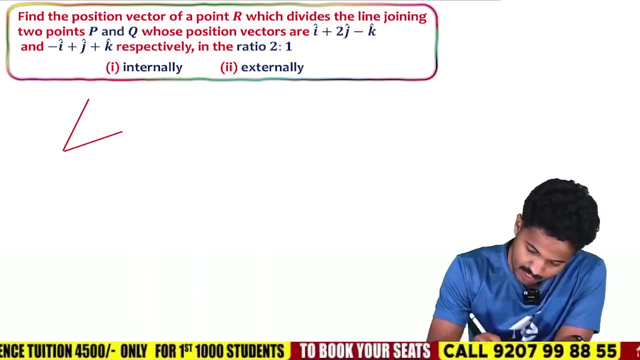 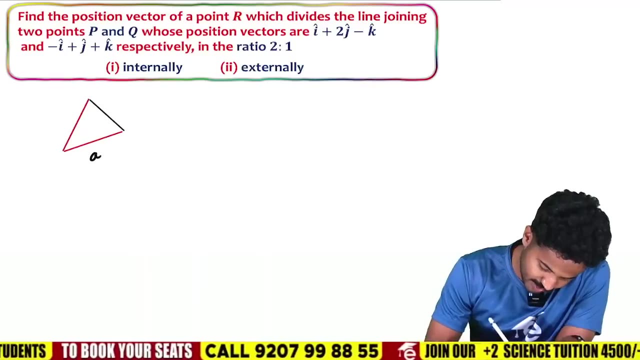 You can learn it. Internal division and external division. We have two position vectors in this form. Look, Two position vectors. Okay, I marked a point here. Here is a line: Look, This vector is a. This vector is b. 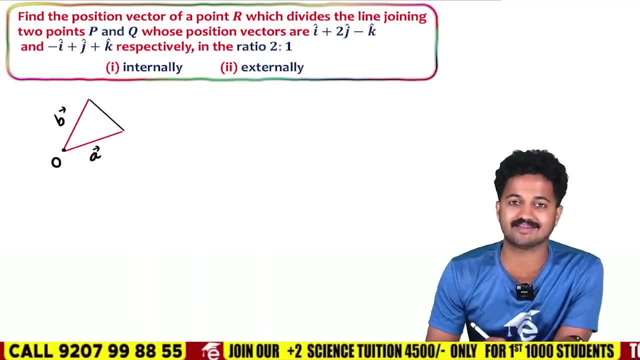 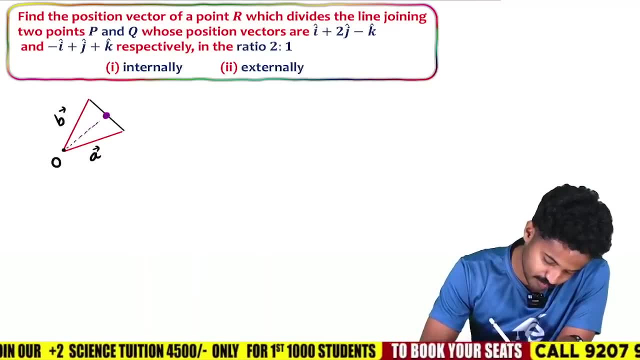 These are two position vectors. If you call it a position vector, you can start it from the origin. So look Here. I marked a point, This point, Here I joined this point. This is also a position vector R. Okay, No problem. 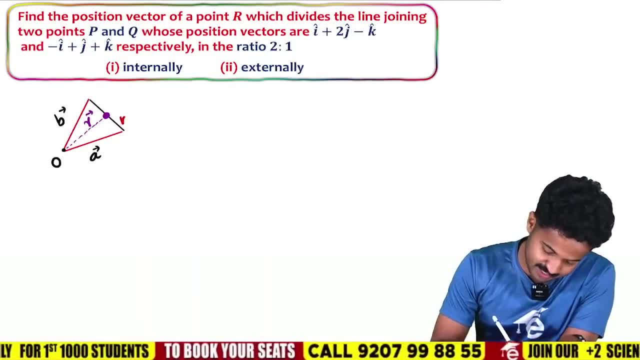 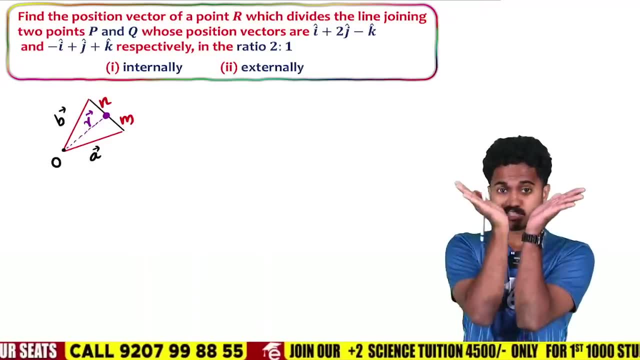 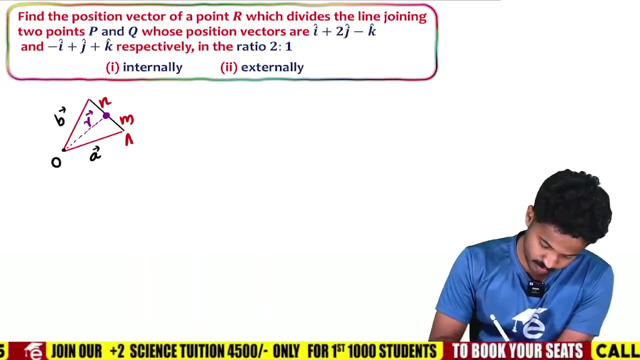 No problem. If we divide the ratio, we will get m and n near a. If you have a line with two position vectors and if you want to give both the position vectors as o and a, you can give o as a and o as b. 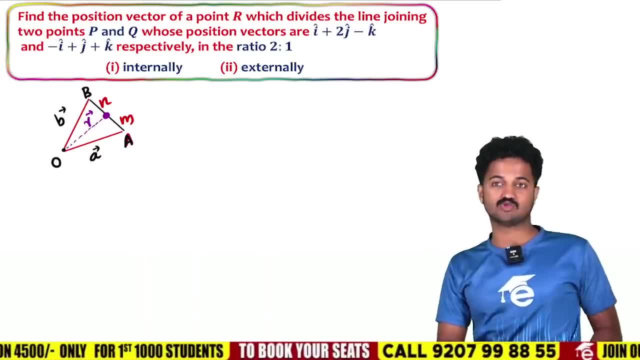 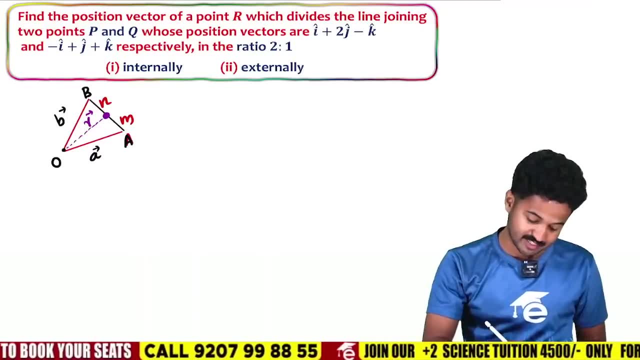 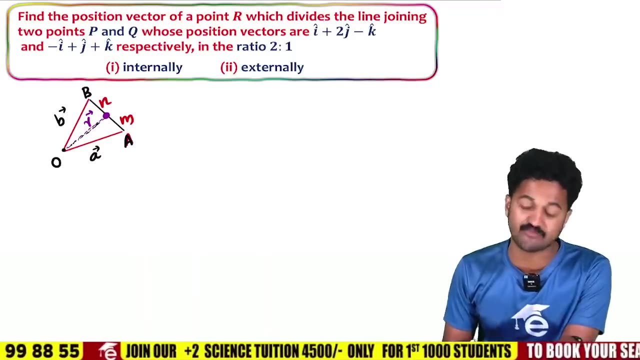 There are two position vectors. Both the position vectors go like this: When both the position vectors join, the line gets divided by a point. The position vector divides that point. The vector called r is the equation. This is the section formula, If it is internally. 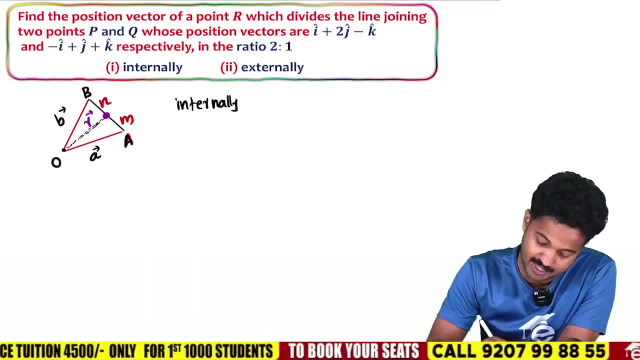 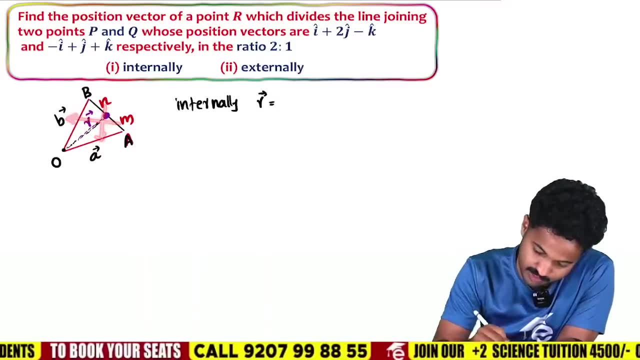 we can divide it within that line itself. If it is internally, r is equal to. It is simple. We can do it like this: Multiply what is here by what is here. Multiply what is here by what is here. That's it. 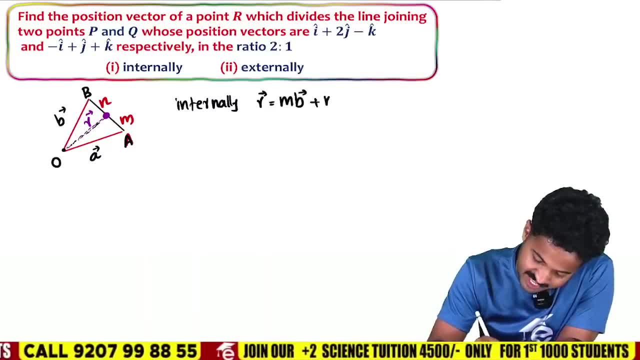 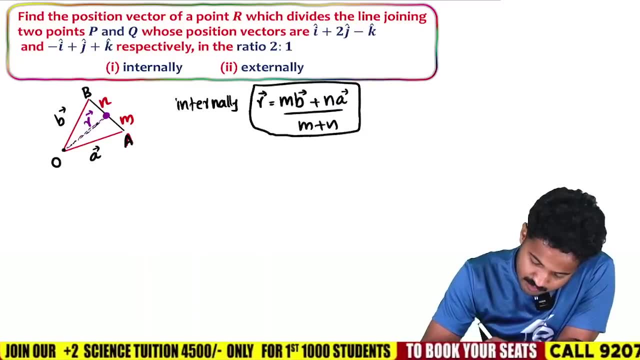 mb plus nn, That's it. mb plus na by m plus n, That's it. mb plus na by m plus n. mb plus na by m plus n, That's it. mb plus na by m plus n, That's it. 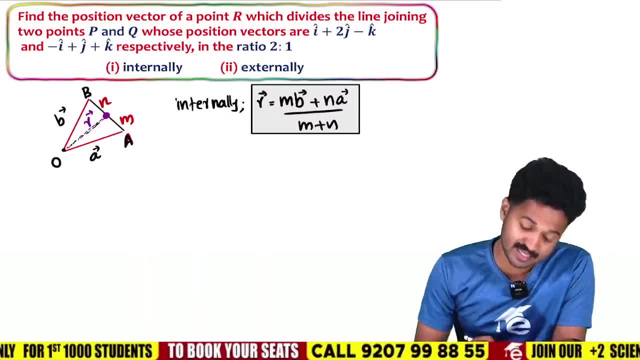 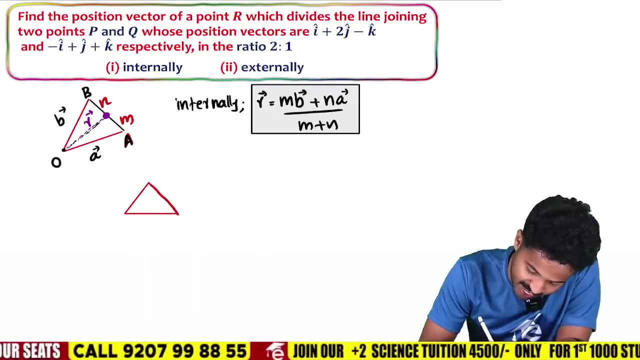 That's the case if it is internally. If it is externally, it will not come out. It will be like this. It will be like this, And dividing this will not be here. This is your o and a vector. o and a. 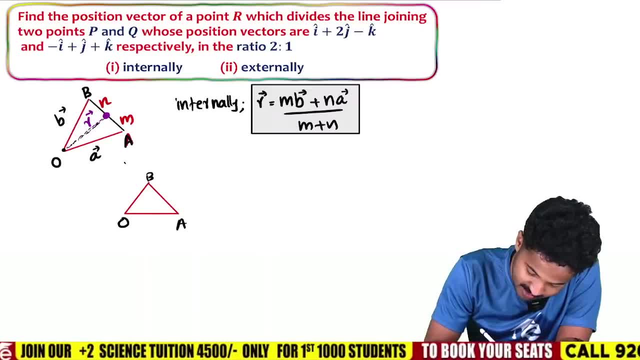 And this is b. So divide it here. It will go like this And divide it at some point outside. So divide outside. This one is m and this one is n. This is our, This is our vector, So we have to find it. 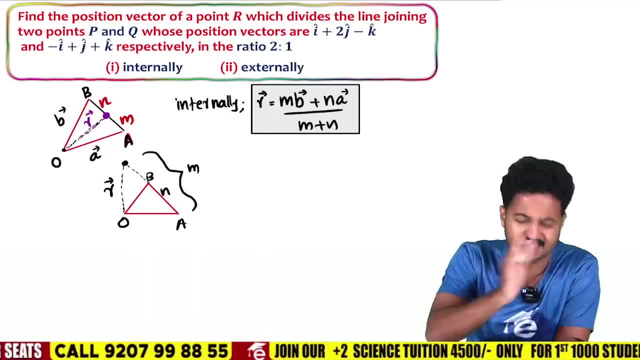 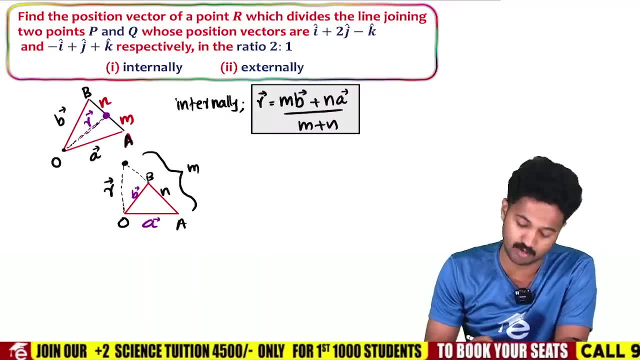 This r this vector, if we have to find it. you don't have to learn anything. You just have to learn the equation: This is vector a, This is vector b. So what do you have to do? As I said earlier, 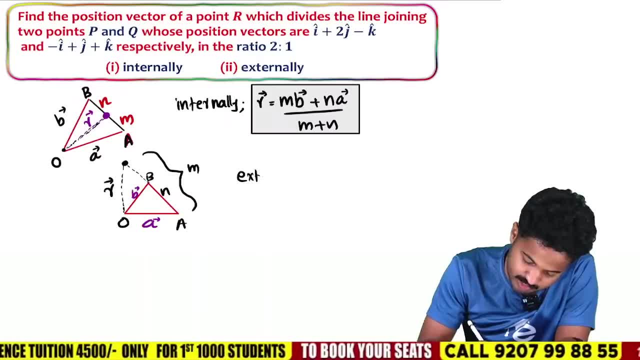 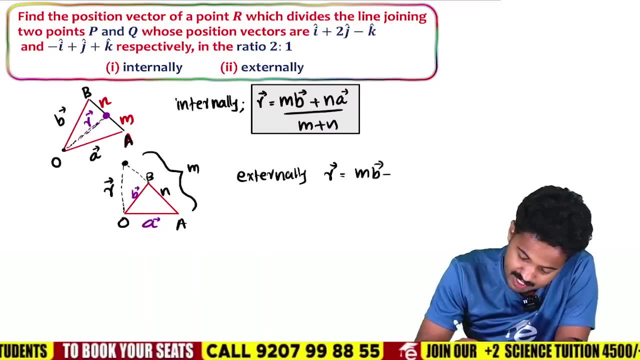 if it is externally? if it is externally, there is an equation: If it is externally, you just have to give a minus. You just have to know this equation. That's the equation r equal to m b minus n. a by m minus n. 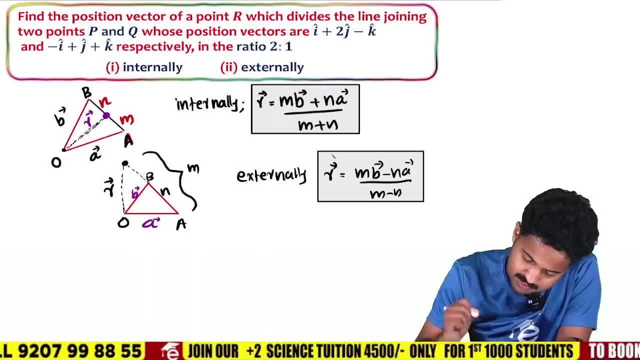 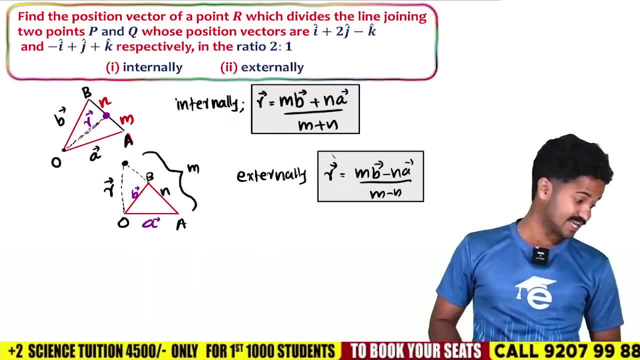 m b minus n a by m minus n. Ready, Easy. So learn these two things properly: m b plus n a by m plus n. and m b minus n a by m minus n. Okay, Ready, So it's simple. 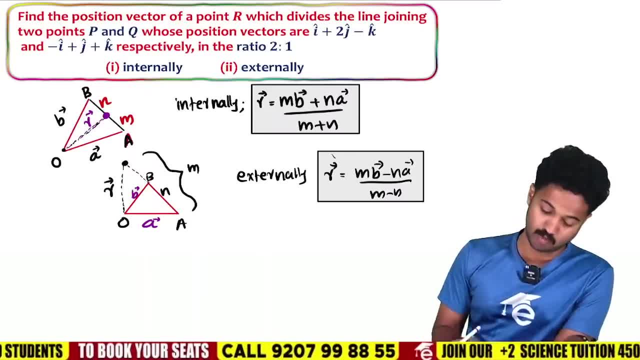 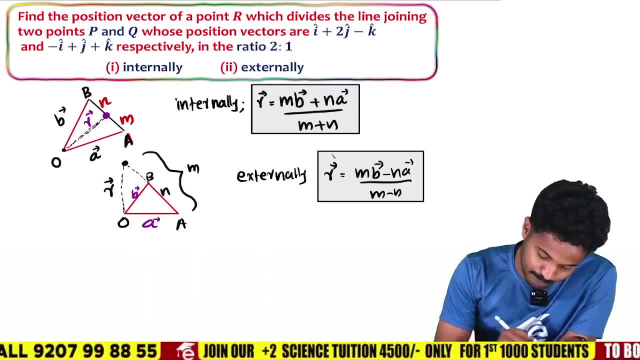 Now look at the question here: External division and internal division. So guys look at what I asked. Find the position vector, The position vector of a point r which divides the line joining the point p, q. Whose position vector is r? 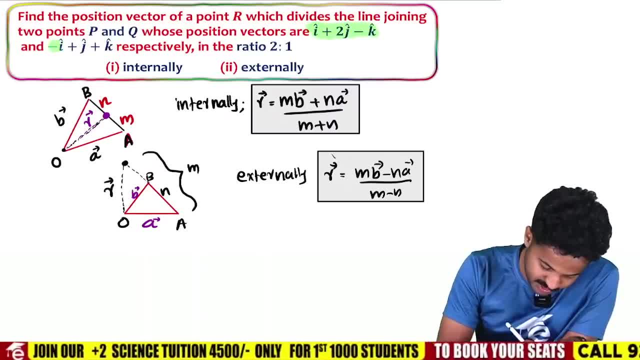 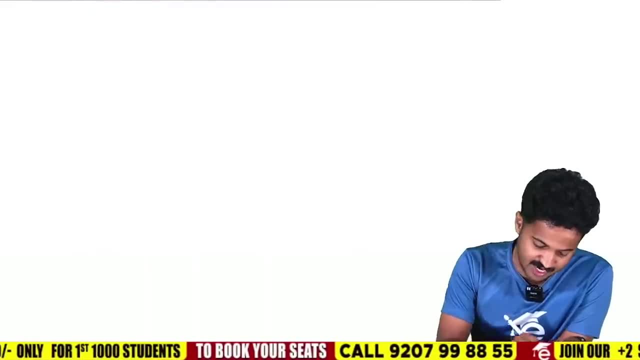 Sir, you have given it here. So you have given one vector, You have given the second vector. You have said that the ratio is 2 to 1.. So do you want it internally or externally? So, sir, if it is internally, 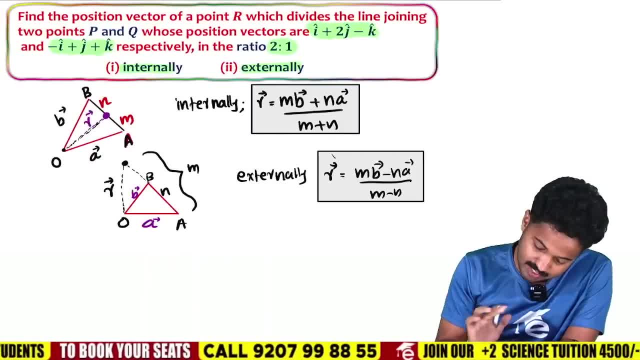 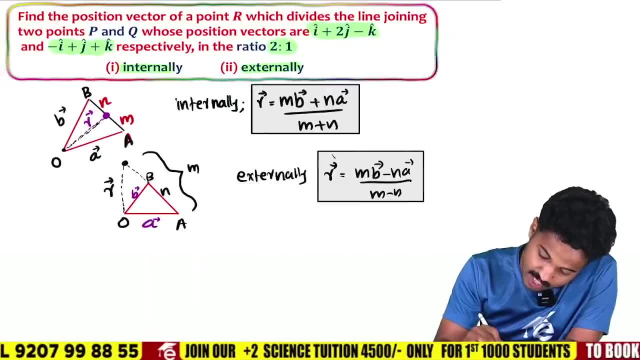 if it is internally dividing. you just have to look at it. First of all, write a and b together: a and b. What is the vector? The vector called a, The first vector. The first vector is i plus 2j, minus k. 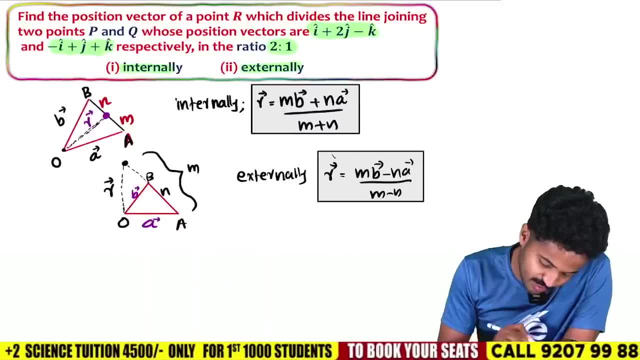 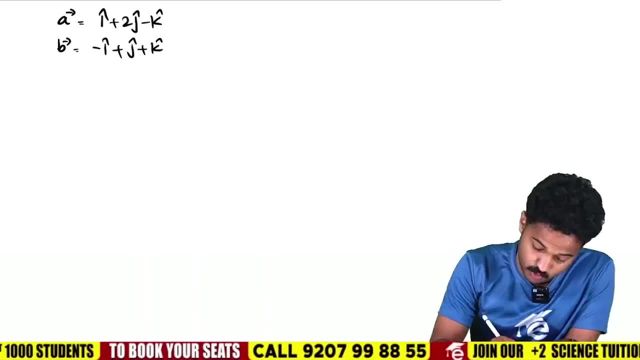 What is the second vector? The second vector, What is vector b? If you have said vector b, it is minus i plus j plus k. Easy, easy, easy, easy, No problem. What is the ratio, The ratio dividing these points? 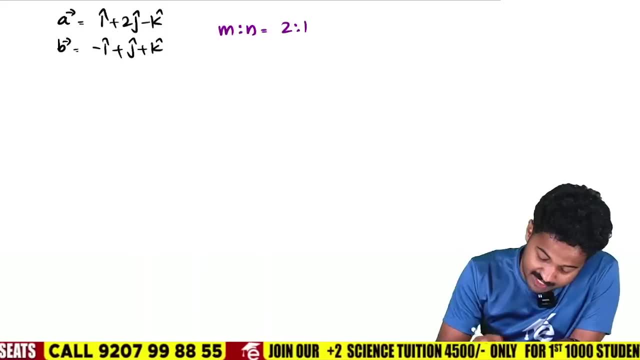 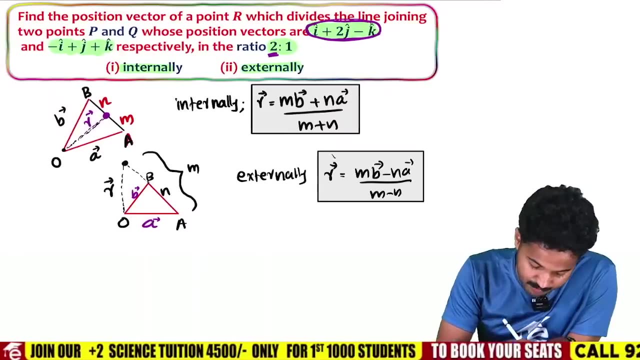 if you say m is to n, it is, 2 is to 1.. You have to take it that way. The first point, which is the first position vector, the part that cuts, it is 2.. Which is the second point. 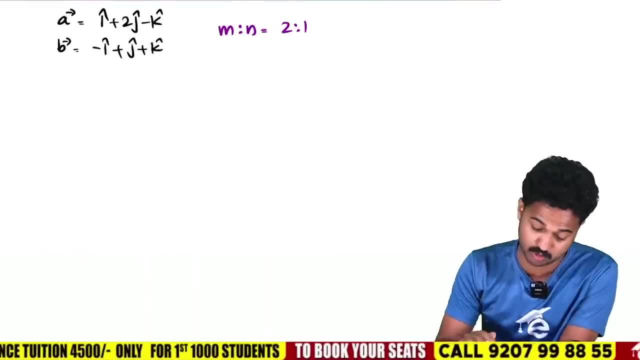 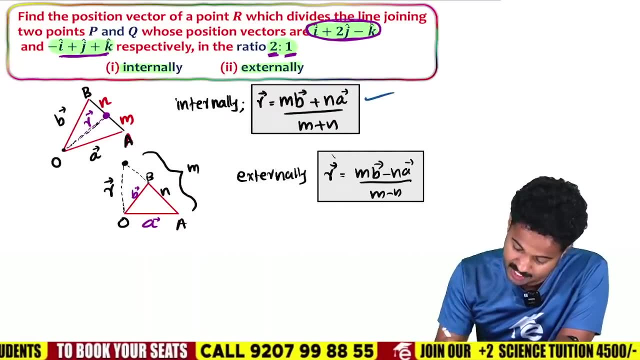 The part that cuts, it is 1.. So if that changes, the answer is wrong. So look, It is 2 and n is 1.. If that is the case, whatever it is here, mb and na are there. 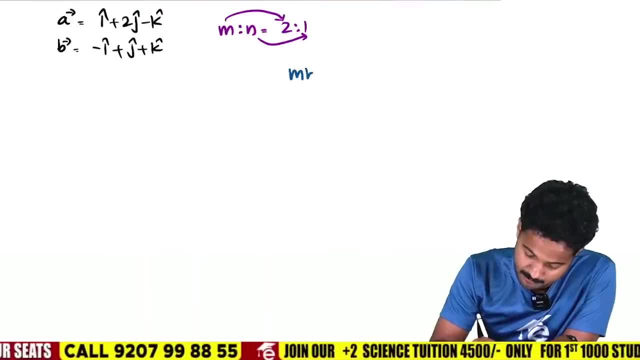 In this also mb and na are there. So I am going to see mb, mb. If we say mb, m is 2, right. So 2 into b is minus i plus j plus k. Right, Minus i plus j plus k is. 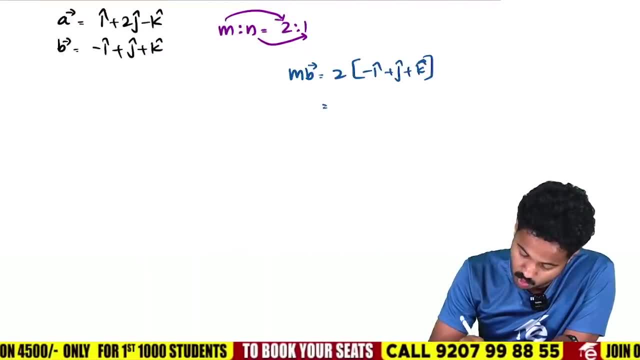 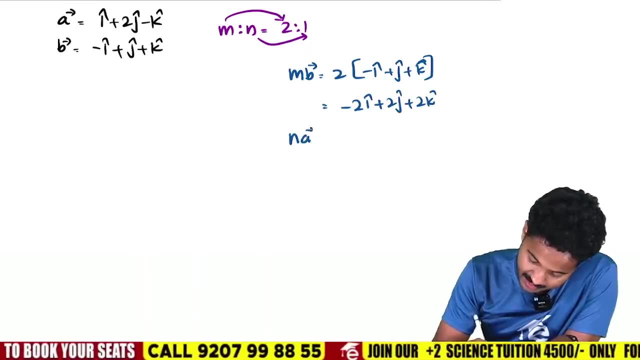 our b. So look, Your answer is multiply by 2.. So minus 2i plus 2j plus 2k, So we got mb. Now what is na na? 1 is 1, right. 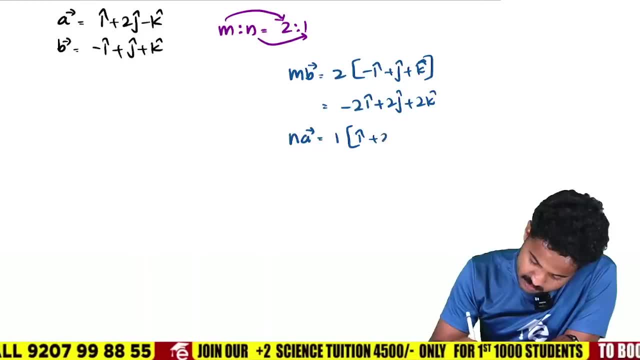 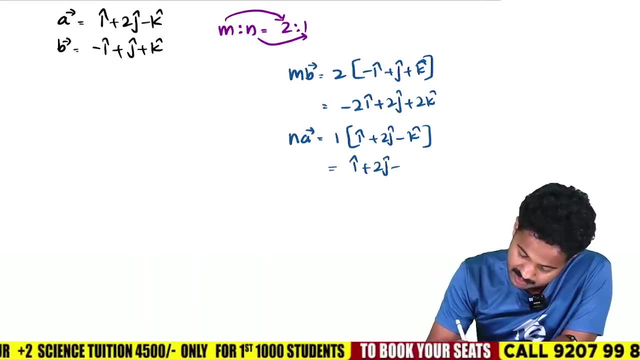 So 1 into A is your same vector. i plus 2j minus k, Easy right. So look, You got the same answer. Multiply by 1.. So i plus 2j minus k, Easy right. 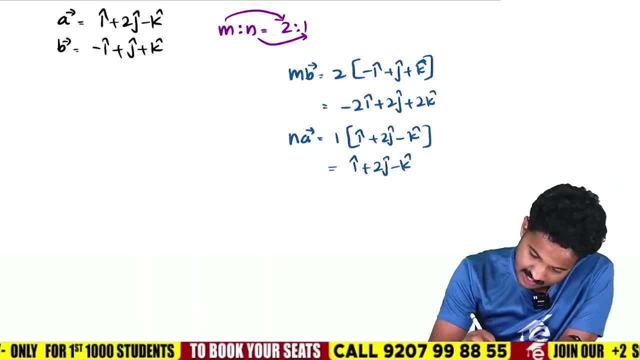 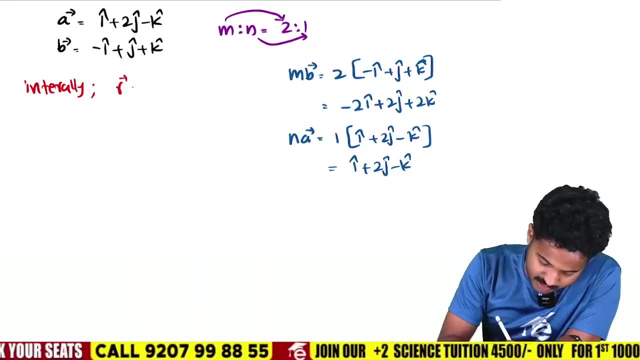 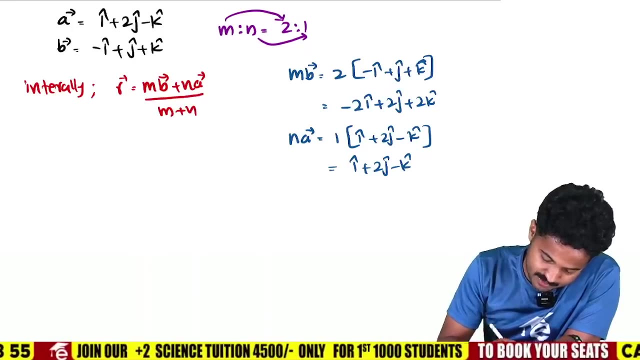 You got the answer quickly and commented it. You got the answer quickly and commented it. So, internally, internally, if we divide, internally, if we divide r, equal to what is the equation? mb plus na by m plus n, mb plus na by m plus n. 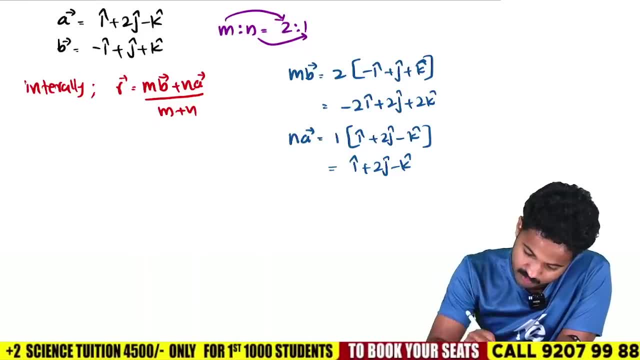 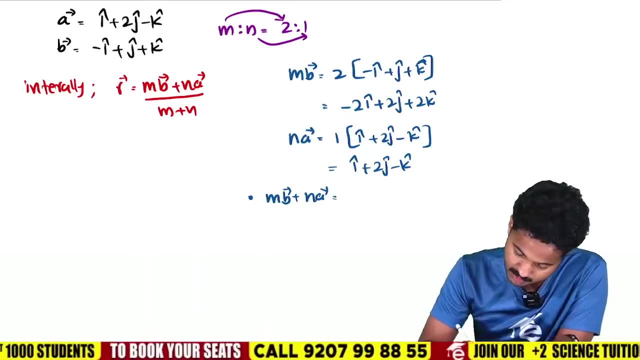 That's how it should be. For that we need to add mb and na together. If we add mb and na together, we get the answer there. So, mb plus na, what do we get? Minus 2i plus 2j plus 2k. 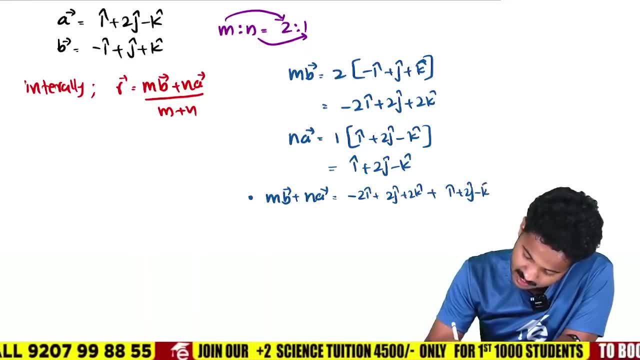 Then plus i, plus 2j, minus k. These are the two vectors we need to add, So the i's are minus 2 plus 1i. Similarly 2 plus 2j, Similarly 2 plus minus 1k. 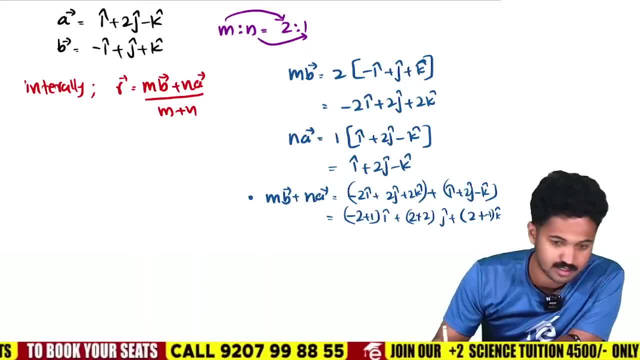 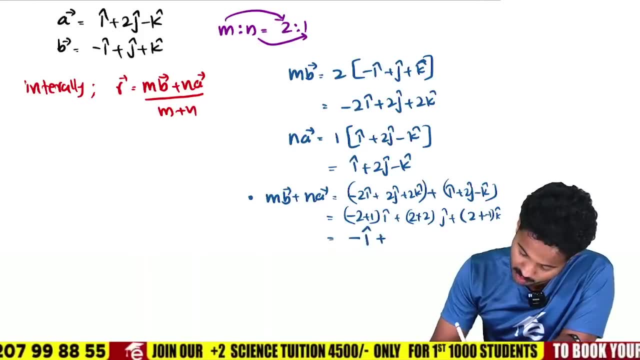 Okay, ready, Easy, No problem. No problem, Can you see? Okay, got it. So look: Minus 1.. So minus i, 2 plus 2,, 4.. So 4j And 2 plus minus 1.. 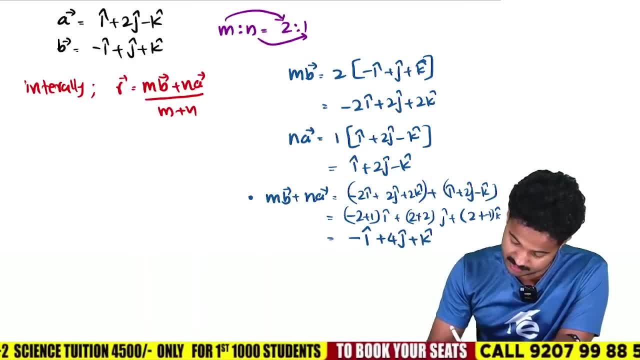 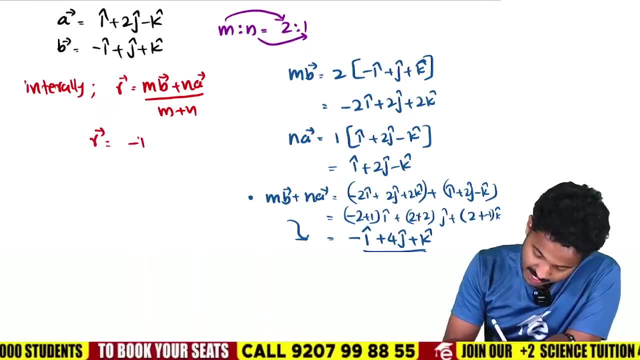 2 minus 1, 1.. So 1 into k, that is k. So this is hijk. This is mb plus na. So you got the answer. r equal to Look Minus i plus 4j. 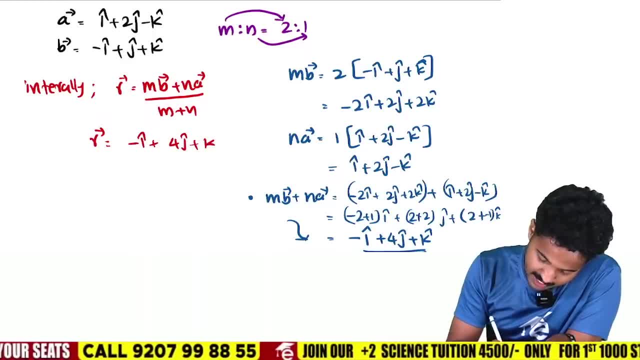 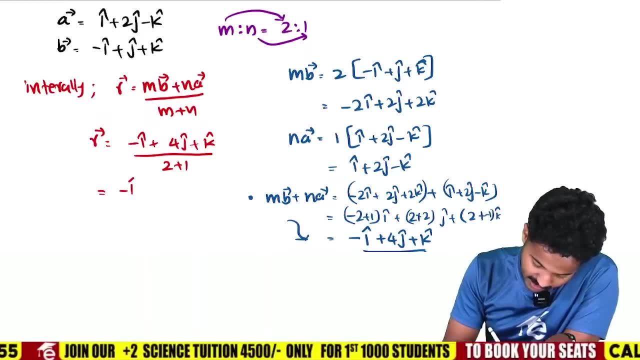 4j plus k And m plus n. is this much? m plus n means you got 2 plus 1. That is 3.. So your answer is like this: Minus i by 3. Or minus 1 by 3i. 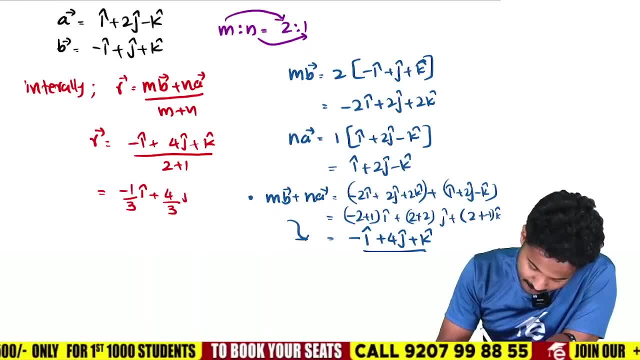 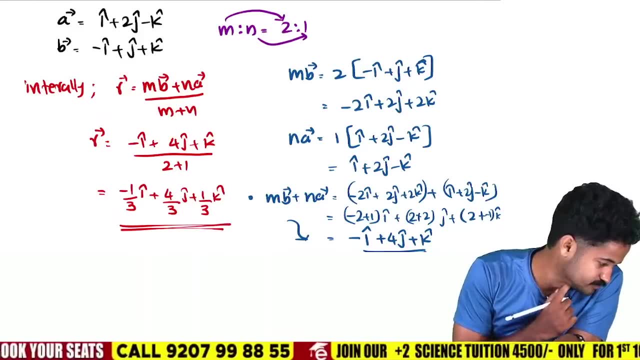 Minus 1 by 3i Plus 4 by 3j Plus 1 by 3k. Look, Look, This is the point where it is internally divided. Yes, Yes, Answer is coming. Okay, very good. 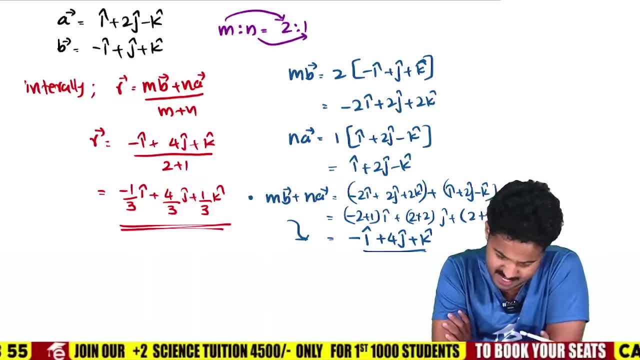 Very good, Okay, Okay, No problem. So this is how you have to do it. After doing this, you will get the answer correctly. It is easy, There is no problem. So you understood the things correctly, right? 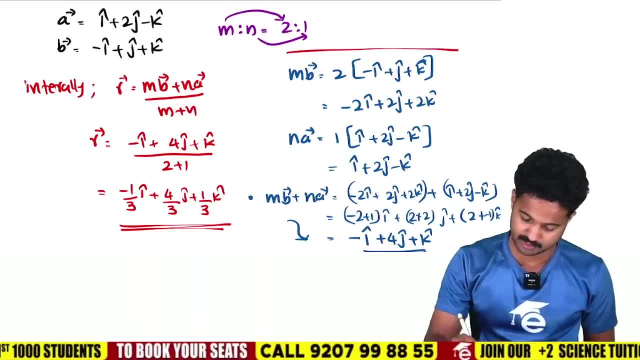 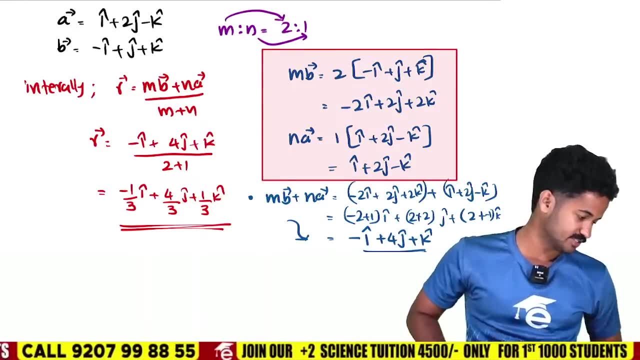 So mb and na are written here. You can write anything here Using this. we can see the point where it is externally divided. Okay, It is easy. mb and na are given. Okay, Yes, Yes, Ticket, Quickly ticket. 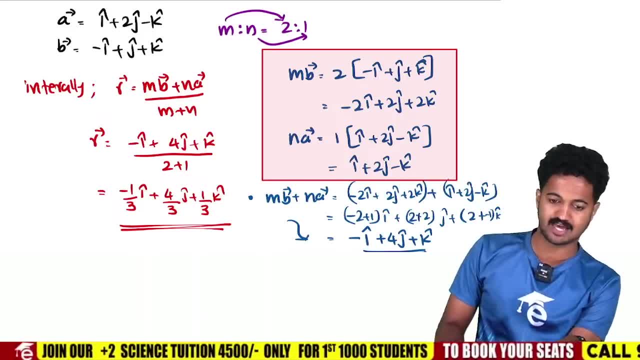 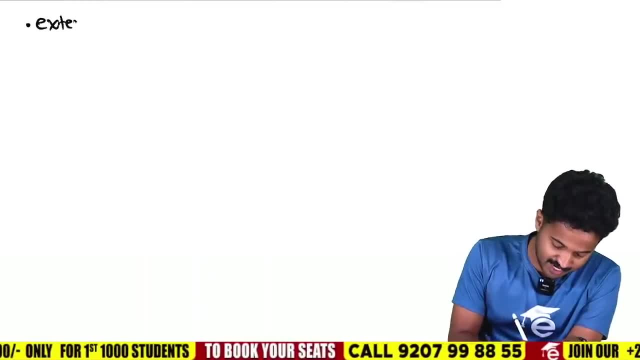 Ticket Tickets. Tickets are coming. So this is it, sir. It is easy, Sir, if it is externally, if it is externally, If it is external, you have to make some changes. If it is external, the position vector. 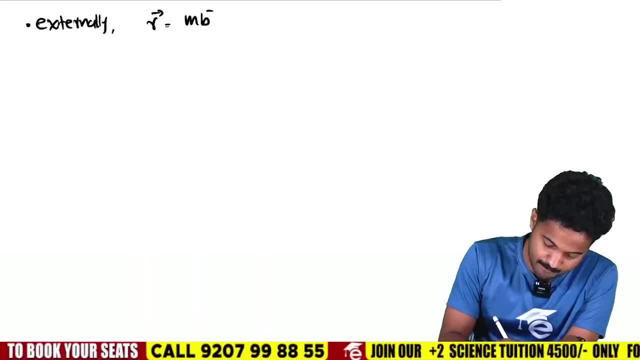 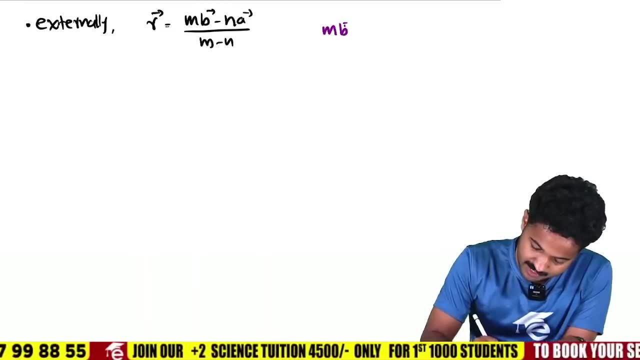 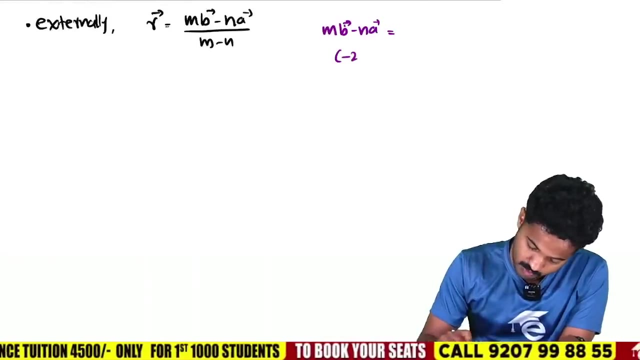 the position vector is r. r is the position vector mb minus na, by m minus n. So what is that mb minus na So mb and na sorry mb and na you have already found. So that is minus 2 minus 2, i plus 2j plus 2k. 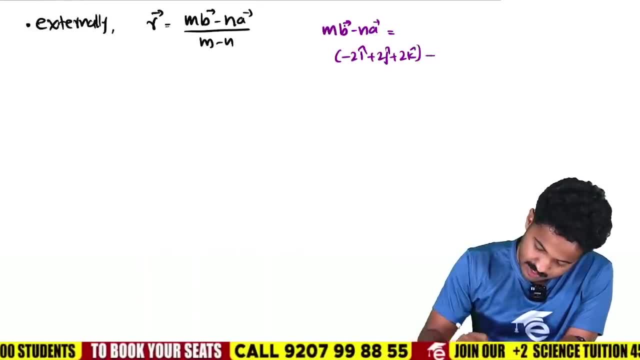 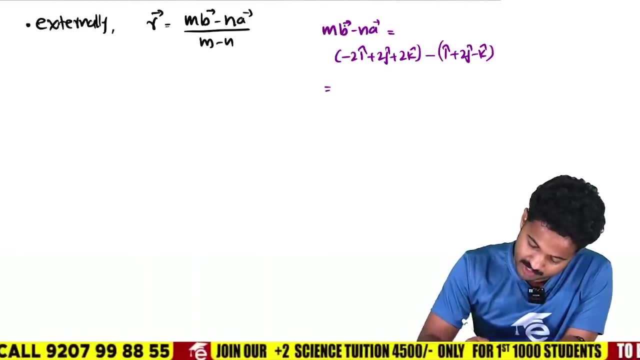 Who has to do minus in this? na na is i plus 2j minus k. i plus 2j minus k. So you have to do minus quickly. You have to do minus quickly. Minus 2 minus 1 is i. 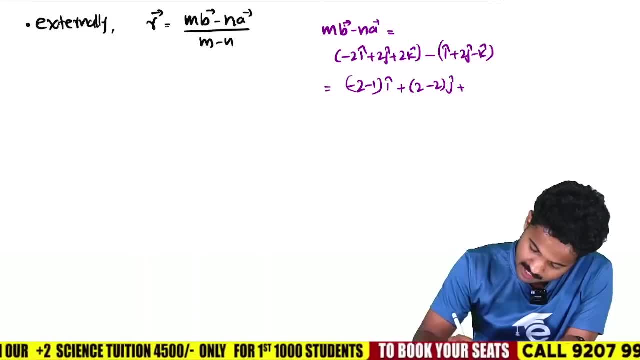 Next is plus 2 minus 2j. Next is 2 minus minus 1k. Easy Minus 2 minus 1 is minus 3i. 2 minus 2 is 0.. So 0j Plus 2 minus minus 1 is 3.. 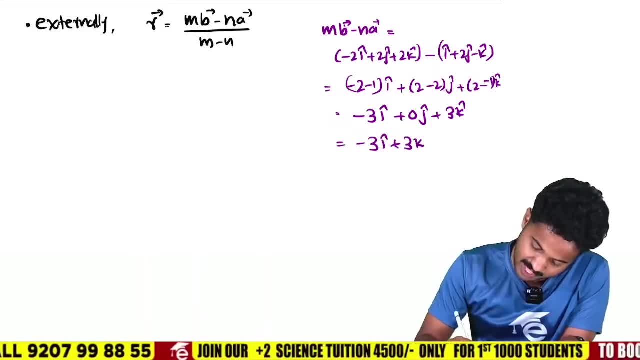 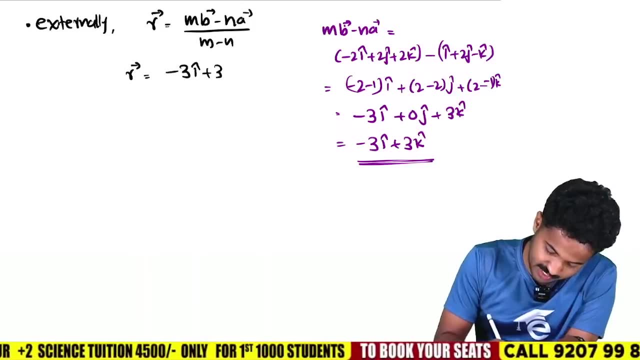 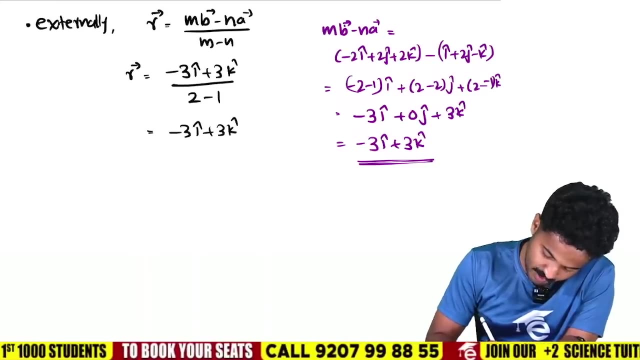 So 3k i plus 3k. This is the answer. Got it? So our answer is r equal to minus 3i plus 3k divided by m2, which is 1.. That is minus 3i plus 3k. 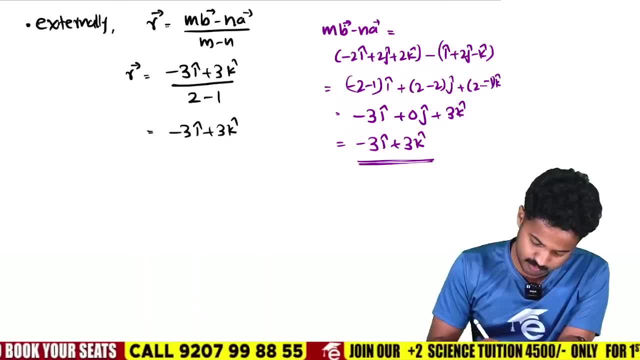 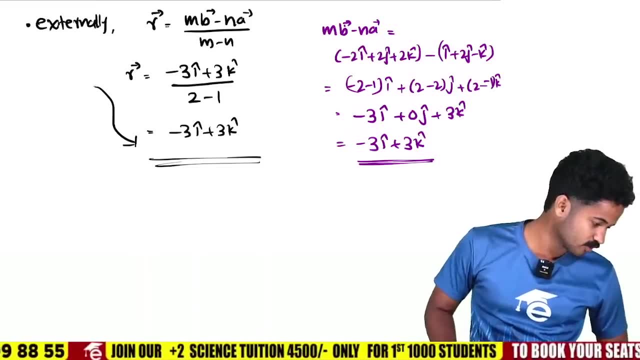 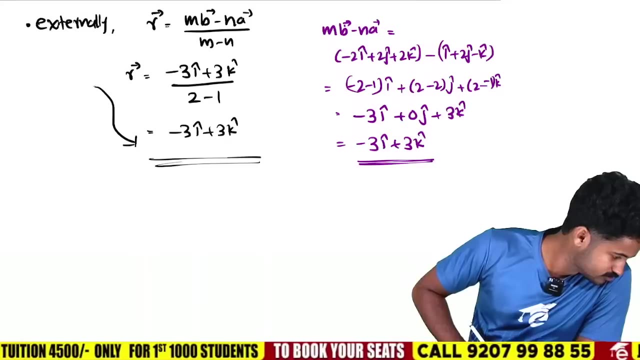 divided by 1.. Do you need to add 1?? No, Even if you add 1, you will get a similar answer. So when you divide externally, this is the position vector. Do you get a green tick? Is it mandatory to write separately? 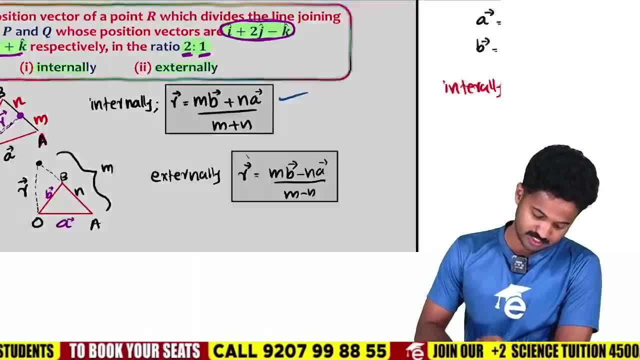 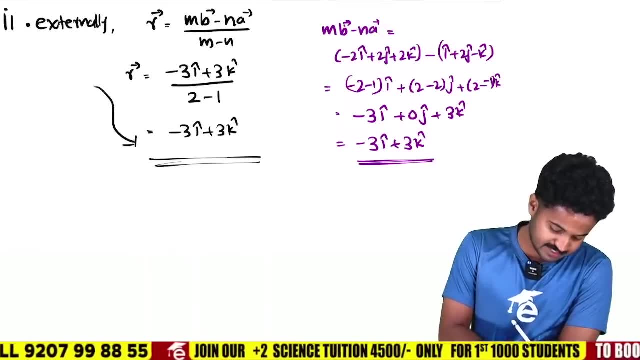 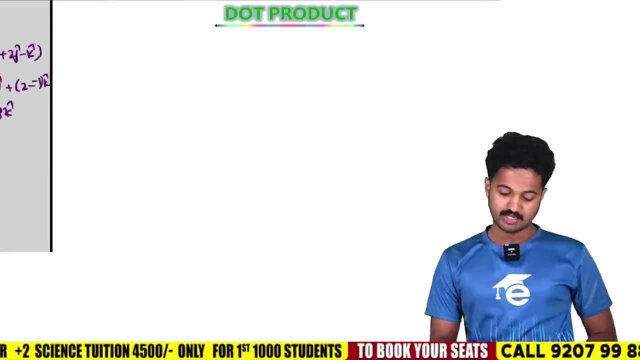 You have to write separately Because the first question is internal. So the first answer you found is the answer that is internally. The second question is the answer that is externally. So the answer that is externally has to be done separately If you ask internally and externally. 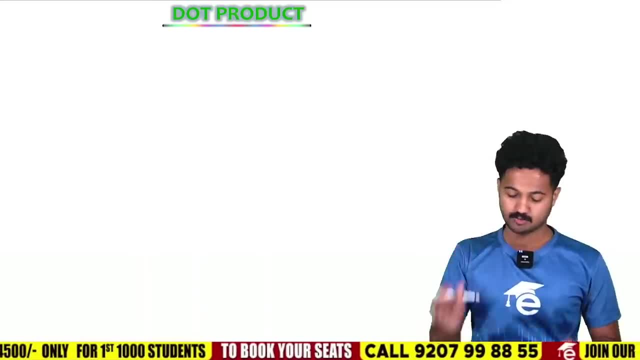 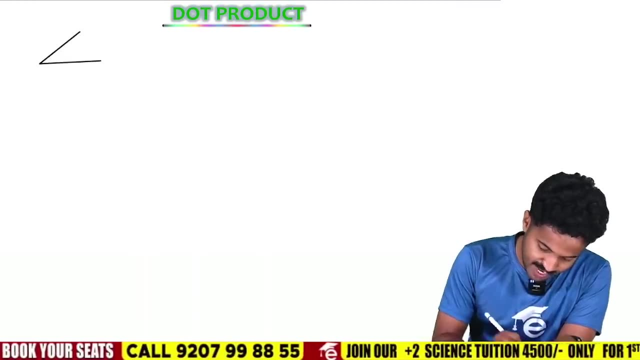 it has to be done separately. The next important thing in this chapter is the dot product. Sir, what is dot product? There are two vectors in this. A is a vector, B is a vector. One line is drawn. The second line is drawn. 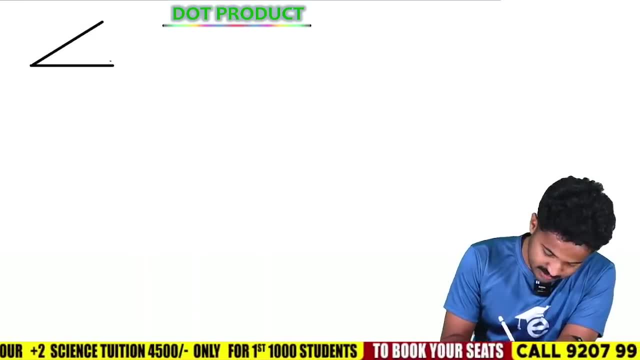 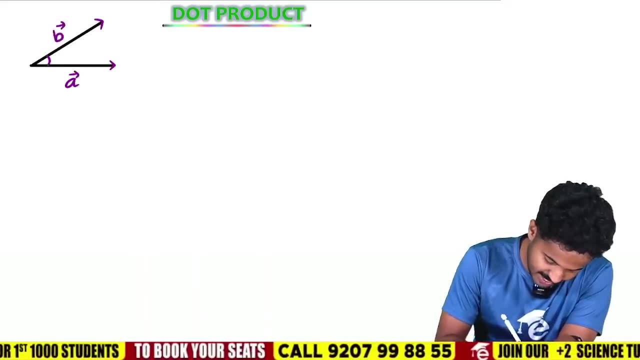 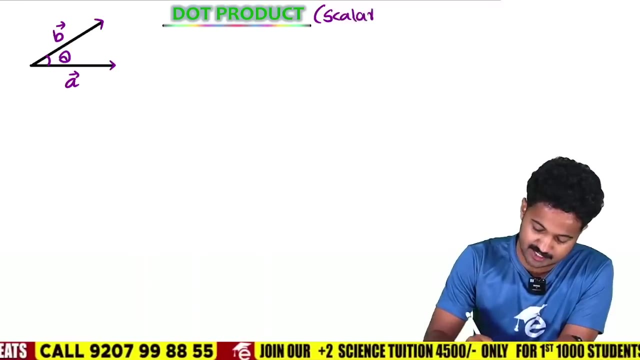 See, it is easy. It is simple. This is vector A, The first is vector A, The second is vector B. The angle between these is theta. Another name for dot product is scalar product. If you do this, you will get a scalar answer. 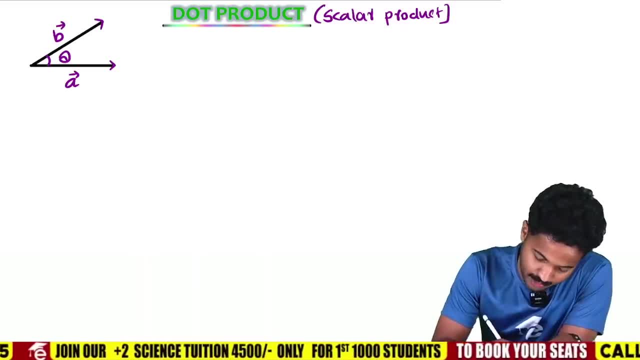 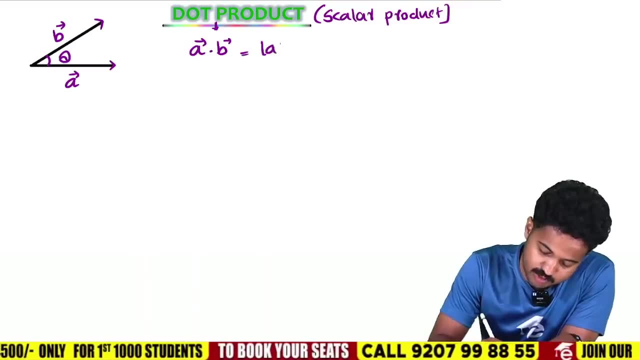 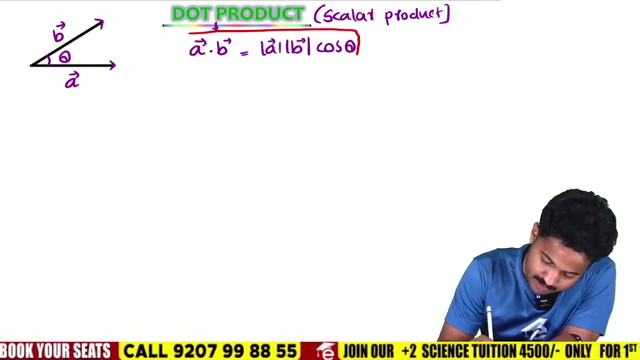 which means a constant. Sir, what is A dot B? There is nothing. A dot B is the dot product. A dot B is magnitude A into magnitude B, into cos theta. This is the dot product. This is the dot product. It is easy. 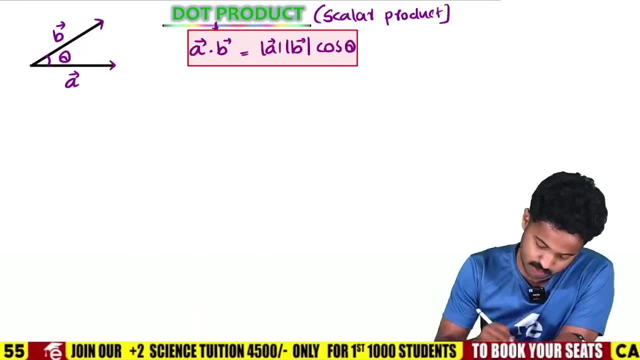 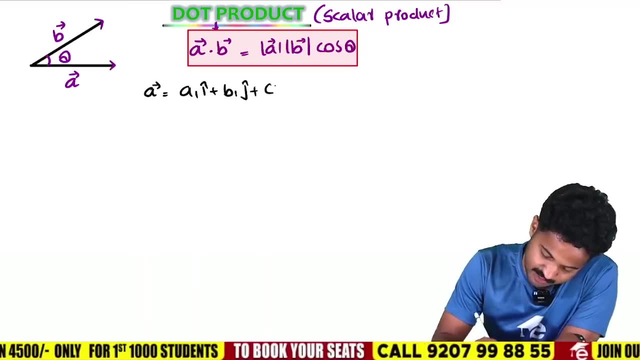 There is an easy method. We often use this. That is, a equal to a1 i plus b1 j plus c1 k. Similarly, b equal to a2 i plus b2 j plus c2 k. This is the first method. 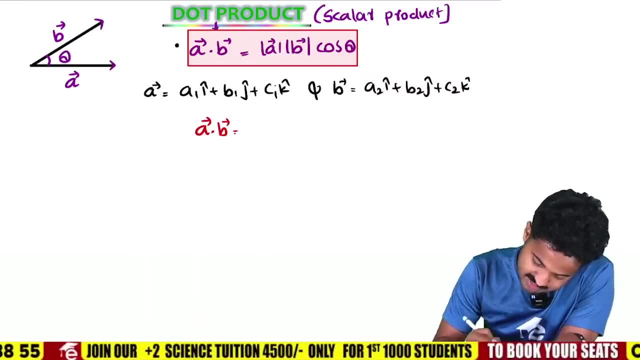 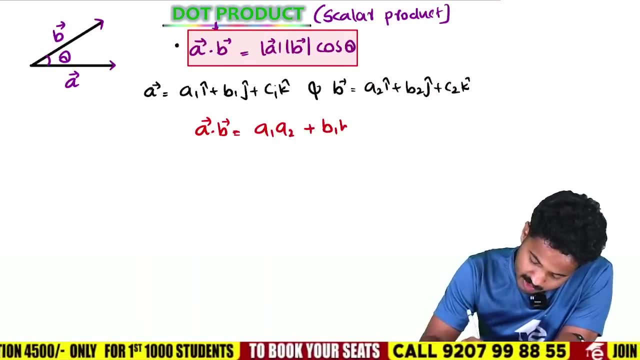 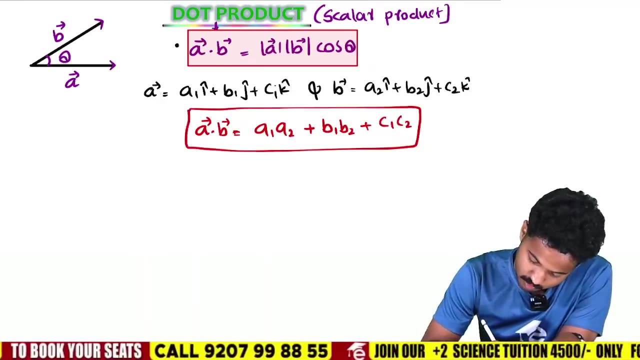 How do we find a dot B after this? It is easy, It is very simple. i components: multiply a1 and a2.. k components: multiply c1 and c2.. That is all. This is what you have to do. Similarly, 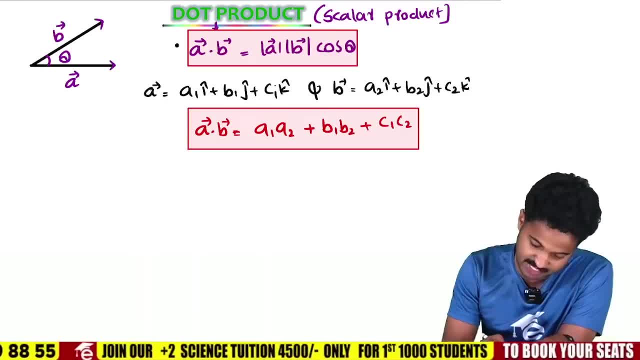 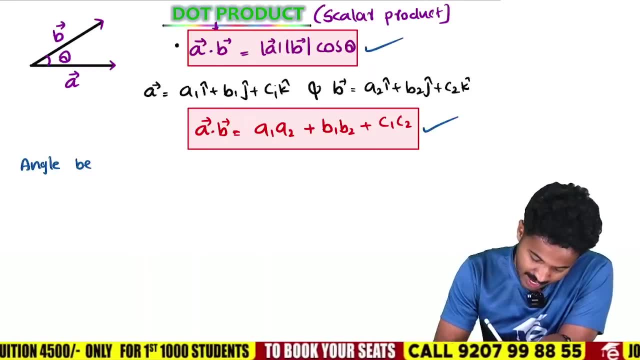 I will ask you to find an angle from this. Angle between two vectors. Do you know what to do? Angle between two vectors. This is important: Angle between two vectors. You don't have to do anything. Put that cos theta there. 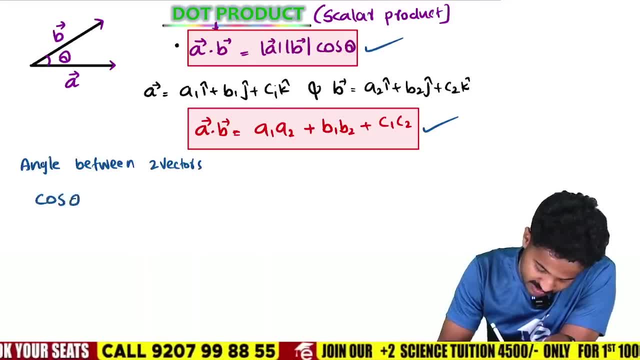 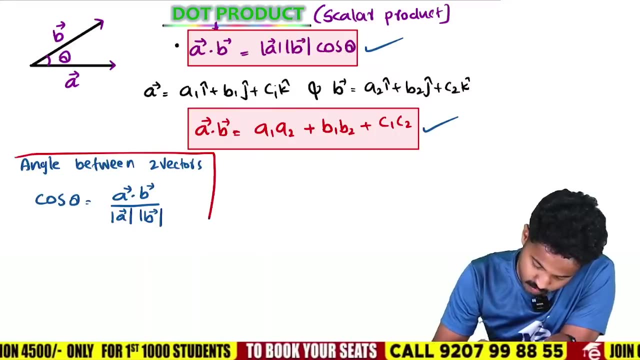 Bring the other one If the cos theta is there. the other one is a dot b. Along with that, the magnitude a and magnitude b will come here. The angle between two vectors is this: Angle between two vectors, a dot b, by magnitude a. 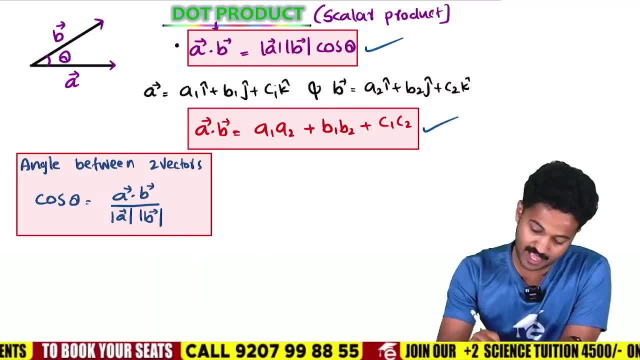 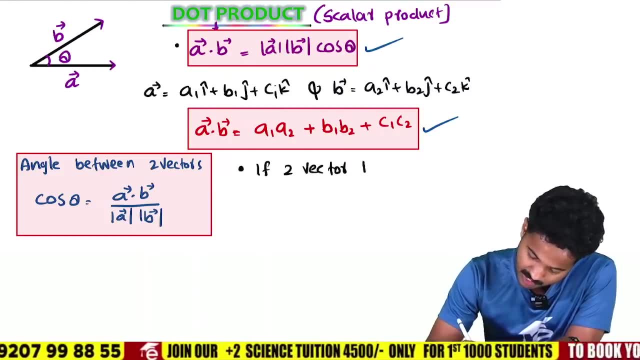 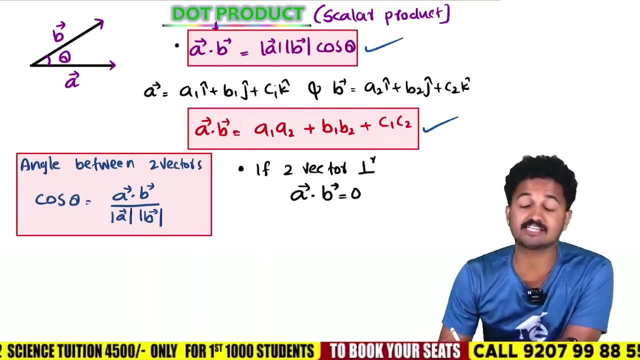 into magnitude b. Easy right, That is also simple. Next thing: If two vectors are perpendicular. if two vectors are perpendicular, if they are perpendicular, note this: a dot b equal to zero. Sir, how does it come If two vectors are perpendicular? 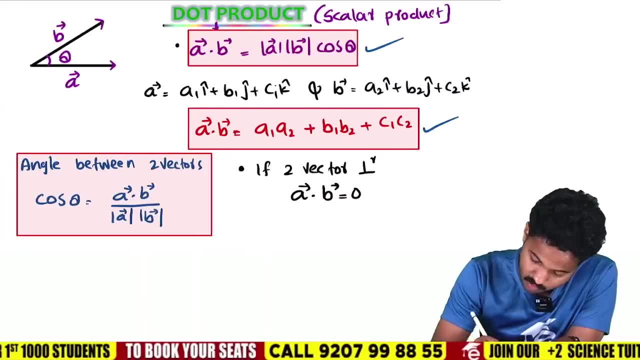 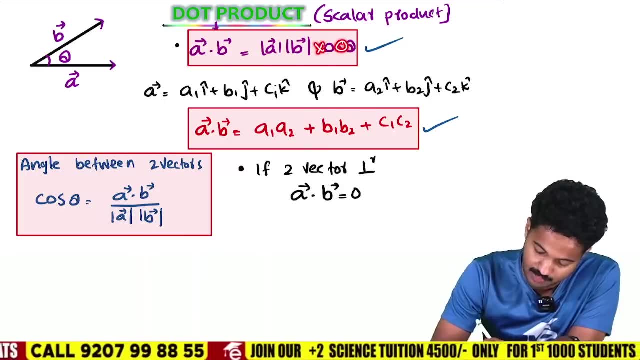 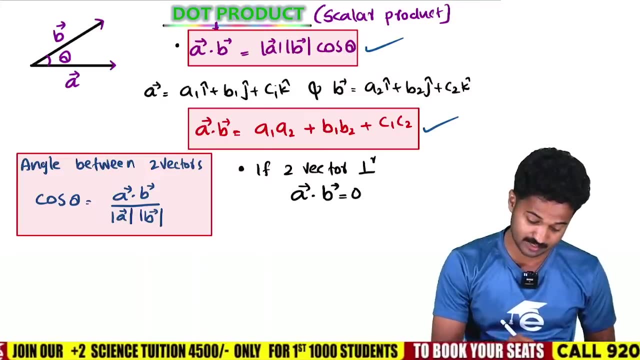 a dot b is zero. How does it come Magnitude a and magnitude b If they are perpendicular? cos 90 will come here. Cos 90 is zero. Then what is the answer? Into zero? What will be the answer? 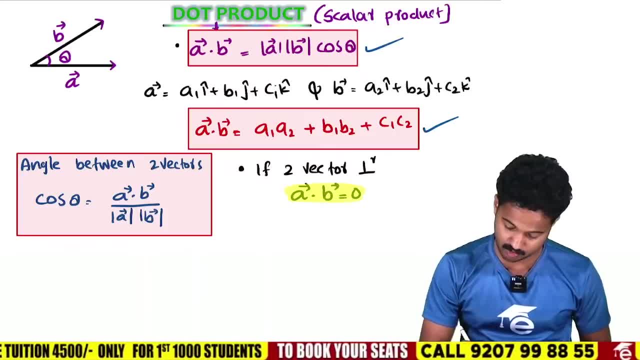 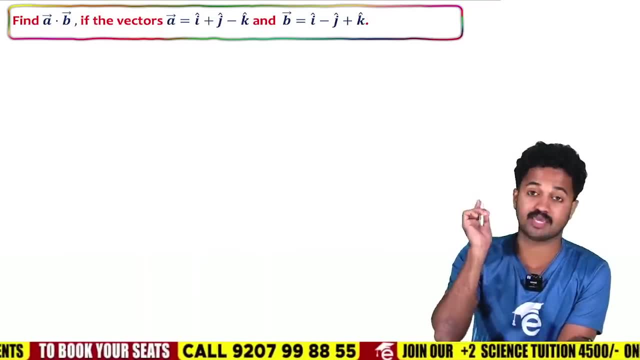 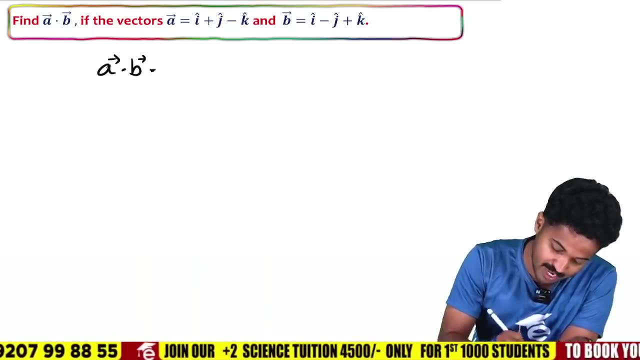 It is zero. If two vectors are perpendicular, it will come here. It is easy. So look a dot b. Sir, I forgot How to do it. We have not given cos theta here. We can do it easily here. 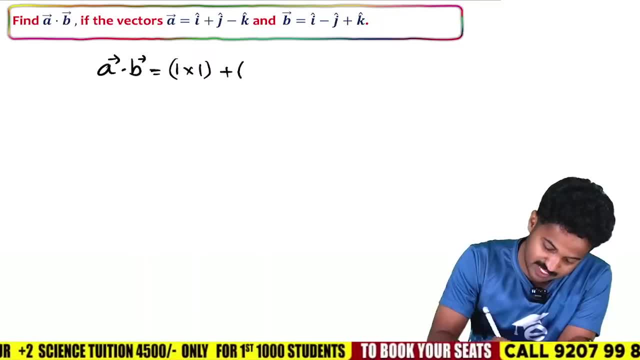 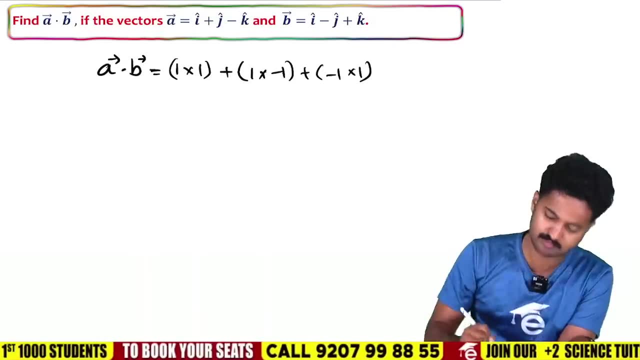 a. dot b is 1 over i, 1 over i is 1.. 1 over i is 1.. 1 over j is 1.. 1 over j is minus 1.. 1 over k is minus 1.. 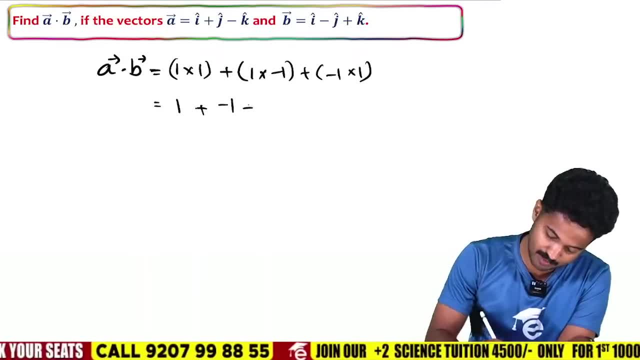 1 over k is 1.. 1 over k is minus 1.. Plus minus 1 into 1 is minus 1.. So 1 minus 1 minus 1.. 1 minus 1 again becomes 0.. 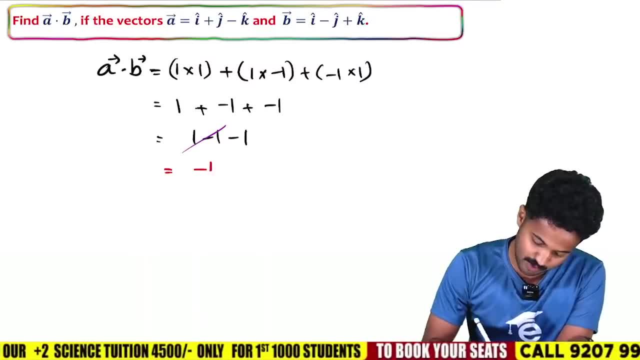 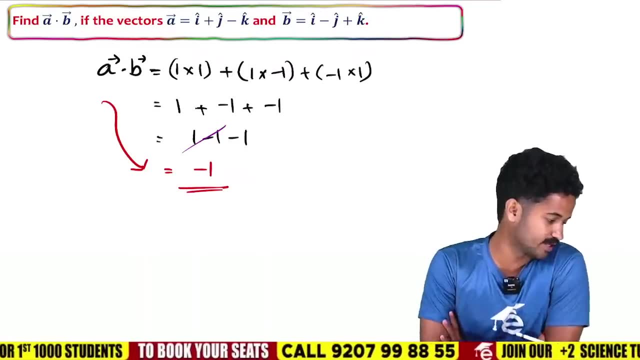 So the final answer will be minus 1.. So the final answer will be minus 1.. So a dot b is always obtained only in scalar form. That is why we call it as scalar component, Sir. when to start 3D. 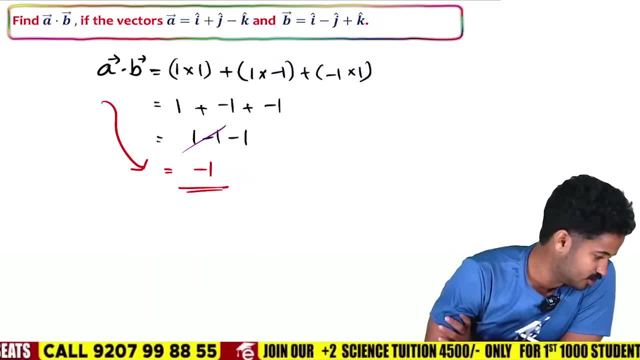 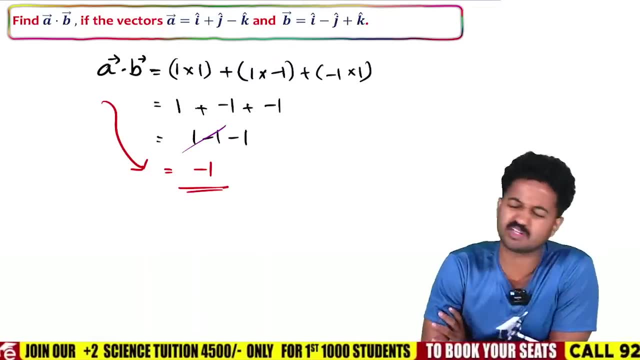 We can start 3D in 10 minutes. Not that It is about separating y denominators. I didn't understand that. If we give each denominator separately, Ah, Okay, It's in the vector, right In the vector. I asked, like this right. 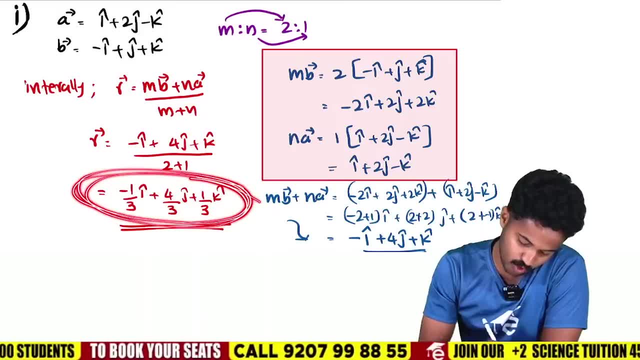 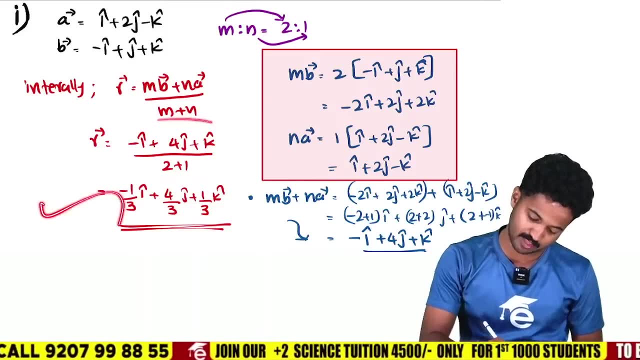 I understood. I asked this: Give it separately, like this: It's better if you give it separately, Because this is the correct component form. This is the correct component form, right? It's better if you give it Now, even if you stop here, there's no problem. 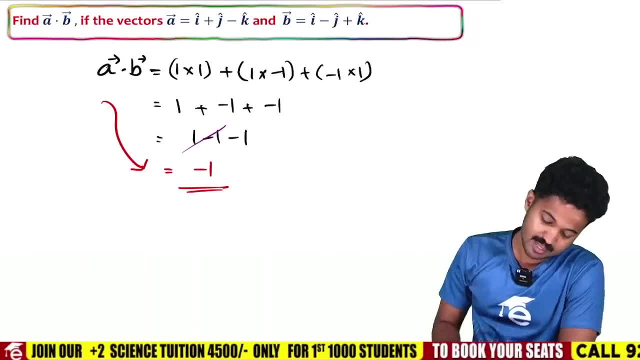 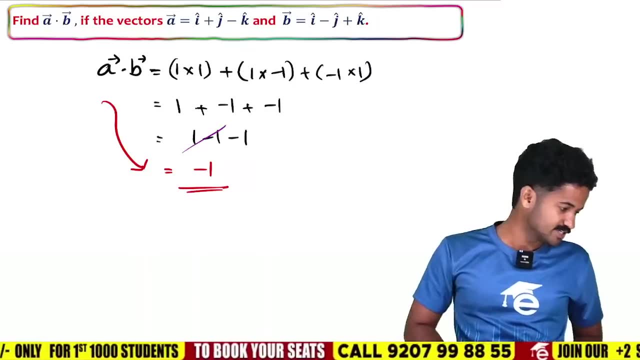 That's what I asked. Now I understood. Okay, Ready, Ready. So look, So those who got minus 1, say it quickly: Minus 1.. Minus 1.. Okay, sir, Yes, got minus 1, got minus 1, got no issue. got no issue. got minus 1.. 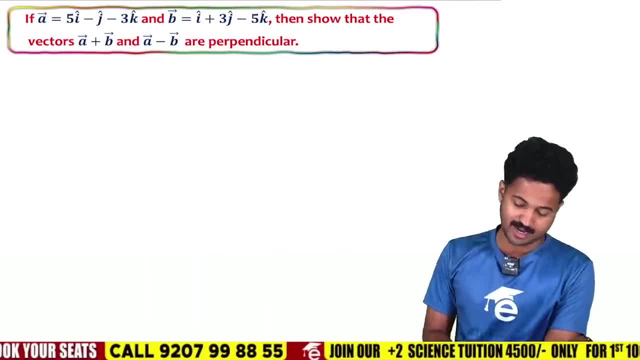 So there's no problem, sir. So far it's very good. So if that's the case, look at the next question. Next question, sir. Next question. Read the question carefully. A and B have been given. 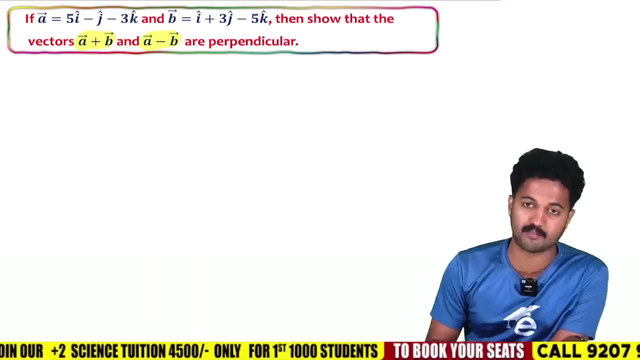 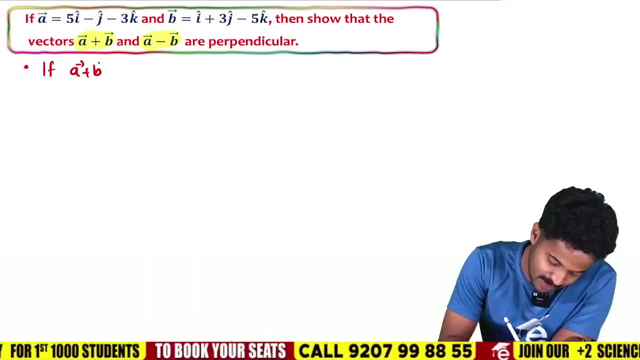 I told you that A plus B and A minus B are perpendicular. If A plus B and A minus B are perpendicular, if A plus B and A minus B, A plus B is a vector And A minus B is a vector. If A plus B and A minus B are perpendicular. 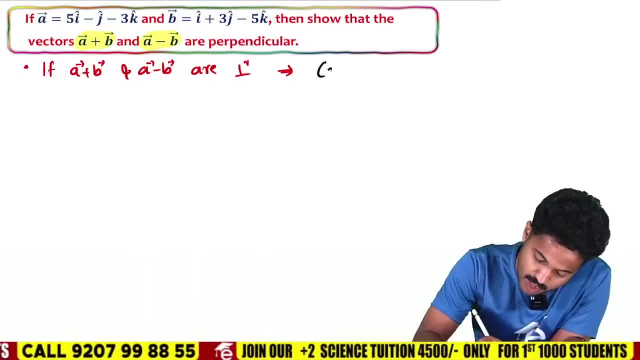 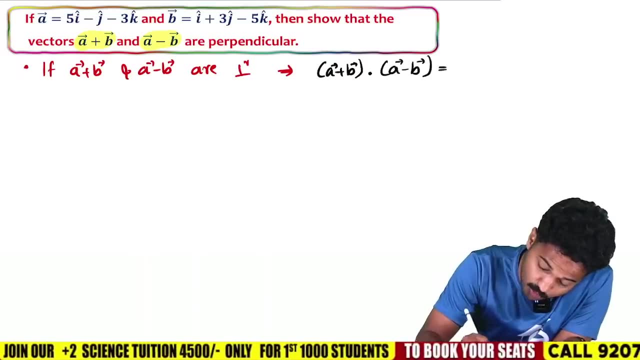 if these two are perpendicular, you have to do this: A plus B and A plus B will get a vector. Similarly, A minus B will get a vector. What will be the dot product of these two? It will be 0. So where the two vectors are perpendicular, 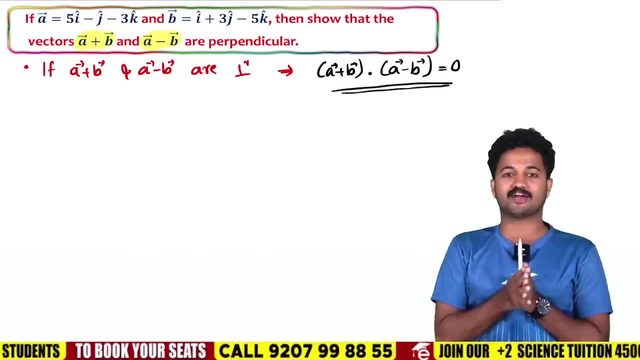 understand that there The dot product of those two vectors. sir, what will that be? It will be 0.. Okay, Ready right, No problem. So it's easy, sir. So what do we have to do first? 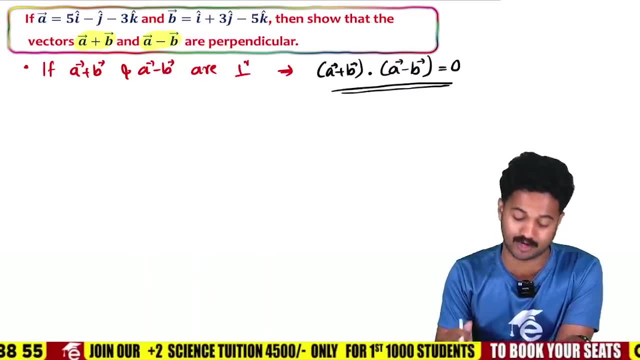 We have to find A plus B and A minus B, And then we can determine whether the dot product is 0 or not. So first we have to find what is A plus B. I am doing A plus B in a simple way. 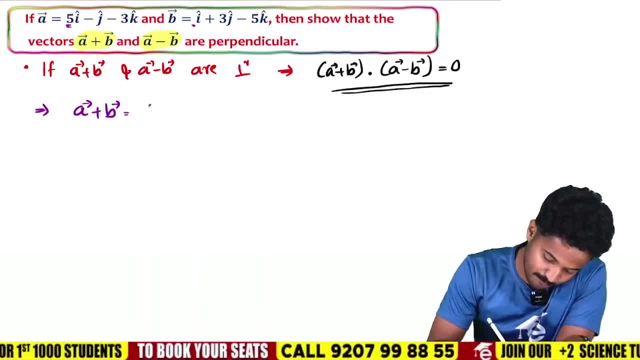 I am doing it easily Here 5.. Here 1.. So 5 plus 1.. 5 plus 1, I Similarly plus Second, here minus 1. There J plus 3.. 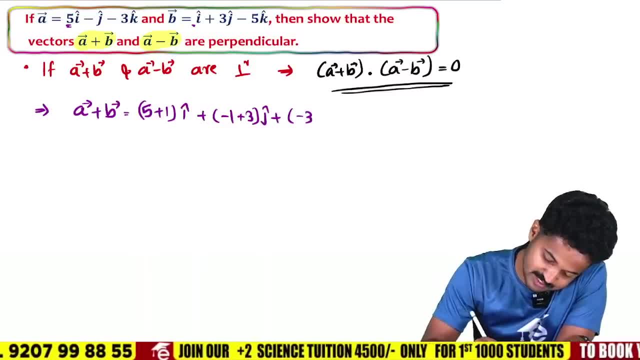 So minus 1 plus 3, J, And next K plus minus 3.. Plus there K plus minus 1.. So the answer is: Look 5 plus 1 into 6.. Sorry, 5 plus 1 is 6.. 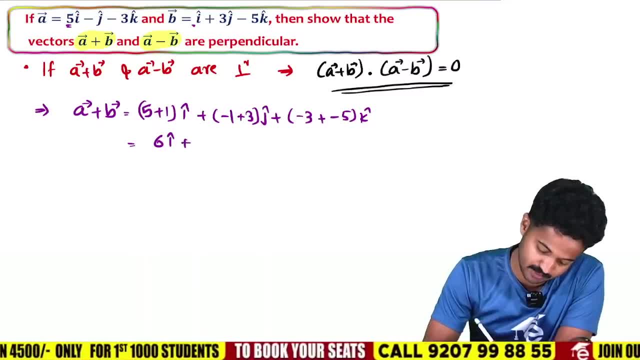 So 6I Minus 1 plus 3 is 2.. So 2I, So 2I, So 2J. Look, it is easy. As you know, I am doing it very easily. 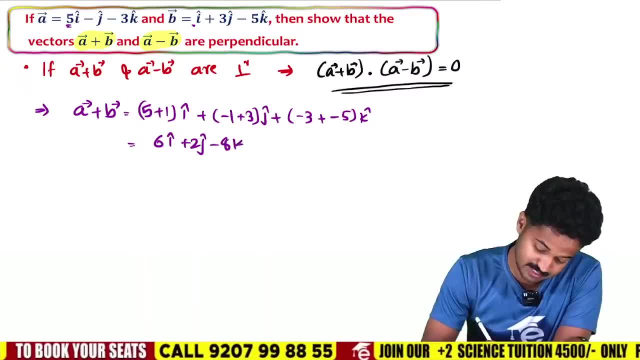 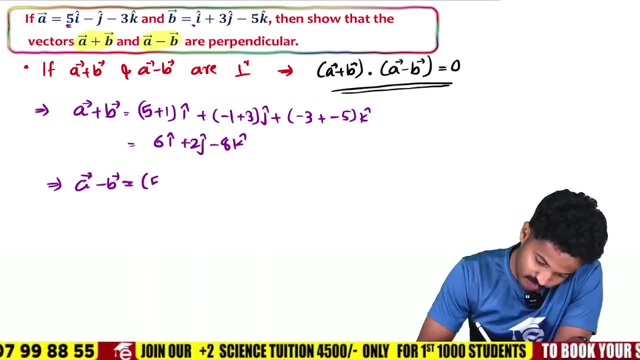 Minus 3 plus minus 5 minus 8.. So minus 8K. This is A plus B. And what is A minus B? What will be A minus B? It is simple, What is A minus B? 5 minus I into 1.. 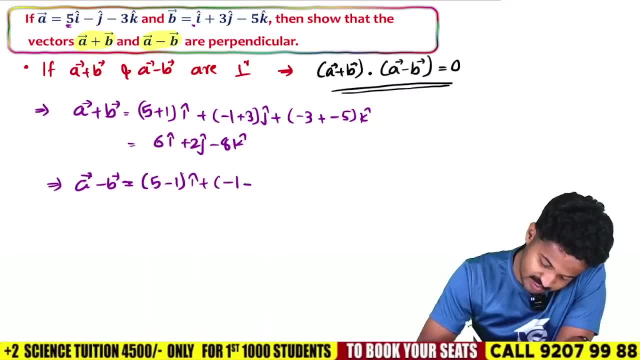 So I Then J into minus 1.. Minus There, J into 3. And J plus Here, K into minus 3.. Minus There K into minus 5.. So K, So look. 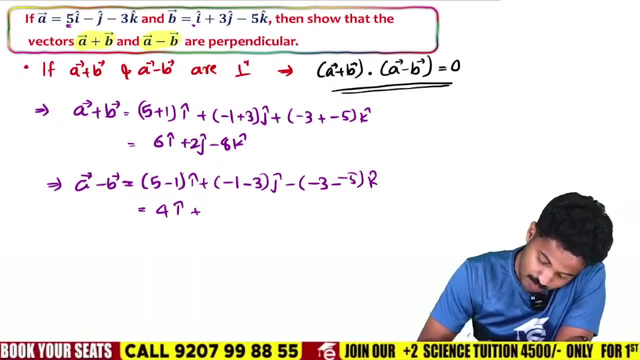 What is the answer? 5 minus 1 means 4.. 4I, 4I Plus Minus 1, minus 3 means minus 4.. So minus 4J, Minus, Minus 3.. 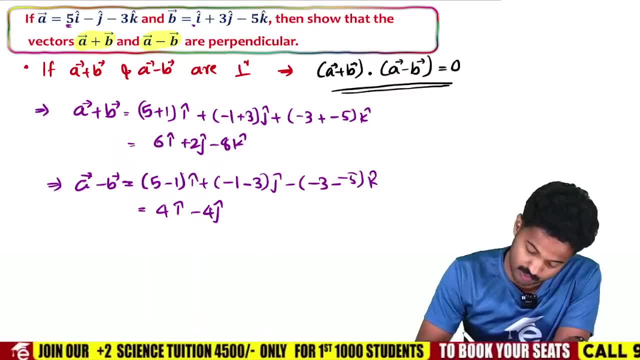 Minus minus Y, Minus 3 plus Y, So this is 2.. There is a plus in front of 2.. So what is this? Plus 2K? So this is A minus B. Sir, it is simple. 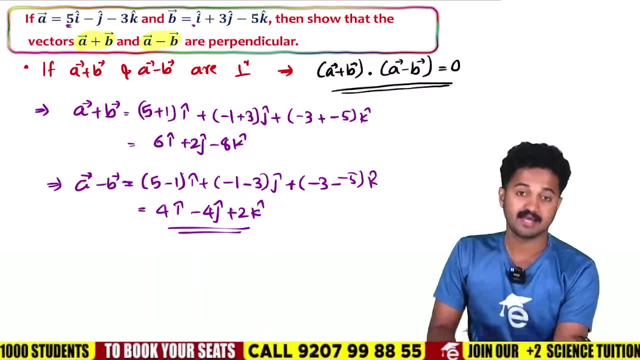 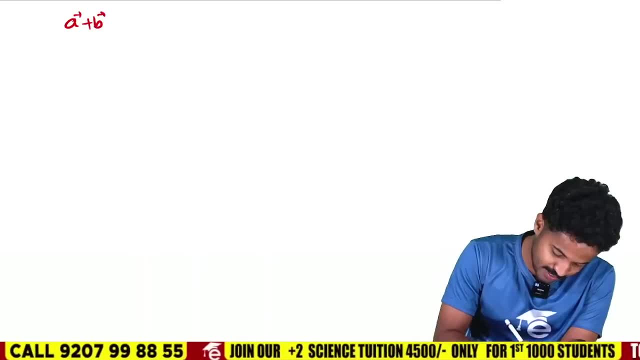 There are no problems, It is okay. So what do you have to do? Hey, if you have to do this perpendicular, find the dot product of that. What is the dot product? Hey, A plus B, A plus B. 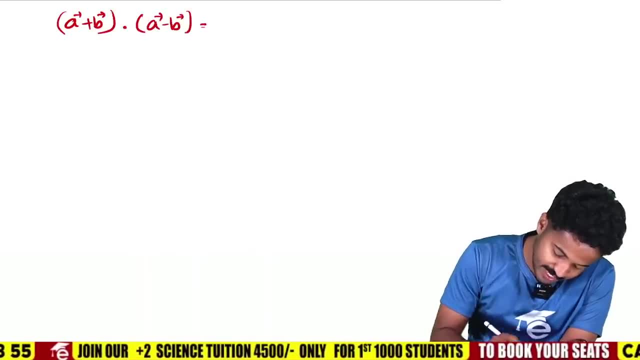 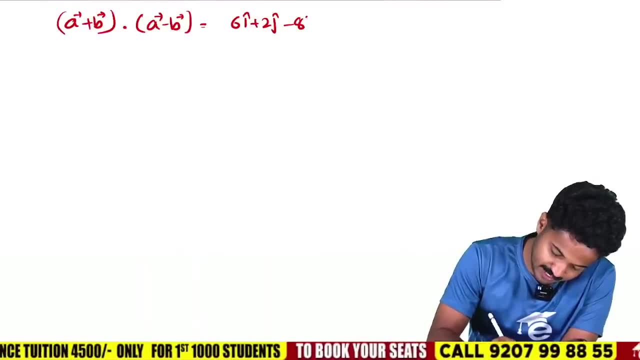 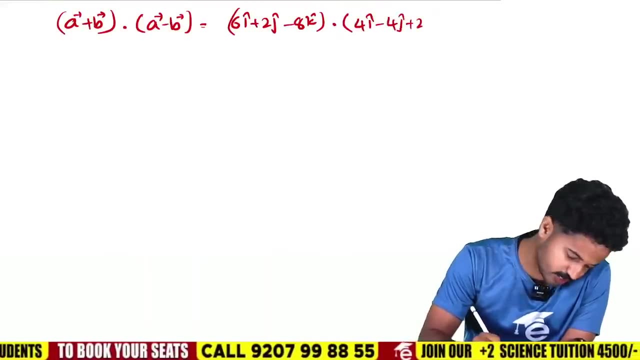 8. 6I plus 2J minus 8K. Dot Dot. Dot product. Next is 4I. 4I minus 4J plus 2K. Okay, Dot product. Find it. Look at this. 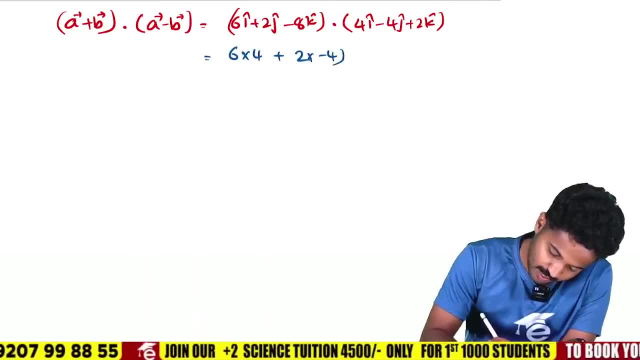 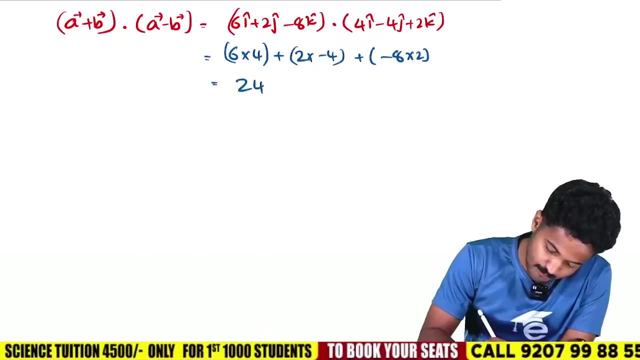 6 into 4, plus 2 into minus 4.. We can do that Multiply with J, With K, Minus 8 into 2.. So 6 into 4 means 24.. Plus 2 into minus 4 means 2K. 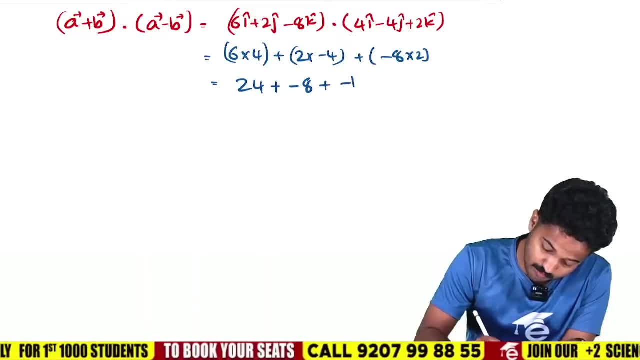 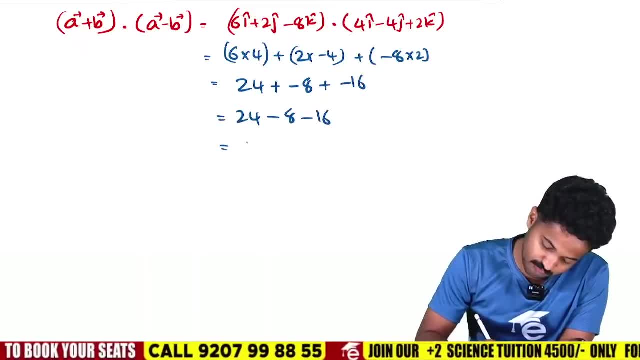 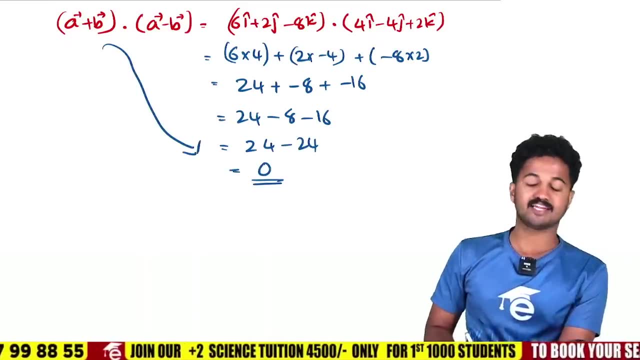 That is 24 minus 8 minus 16.. 24. Minus 8 minus 16 is 0.. So look: a plus b, dot a minus b, That is dot product 0. So what can we say? 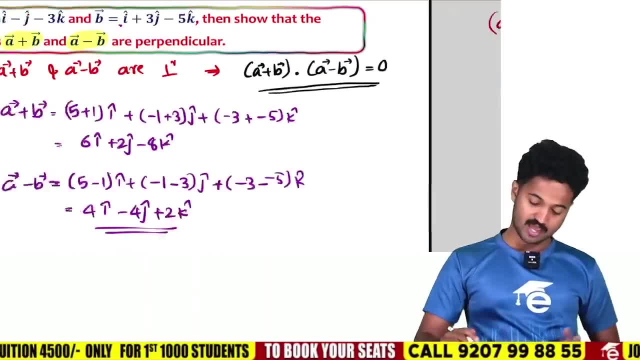 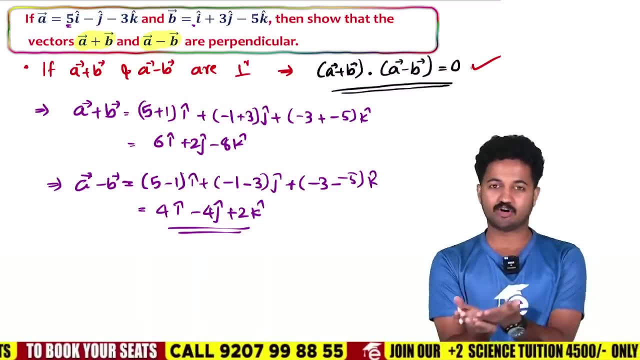 So both of them are perpendicular. In that case, dot product is 0.. What is the condition of perpendicular Dot product is 0.. Both of them are 0.. Here ask a and b. Ask a, dot b is 0.. 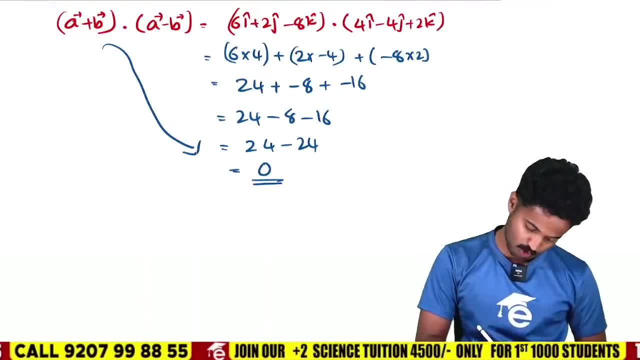 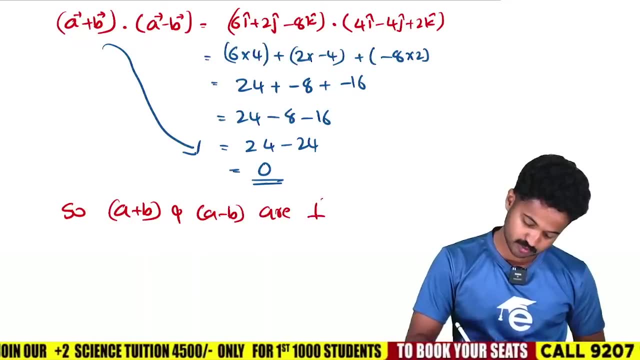 I said a plus b and a minus b, No problem. So what can we say? a plus b and a minus b are perpendicular, Easy, No problem, It is good. Okay, sir Ready, Do you know that it is 0?? 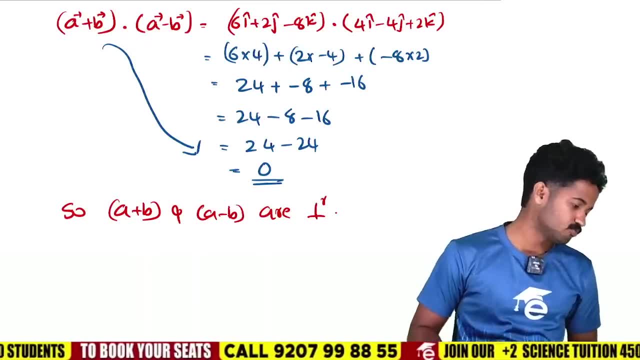 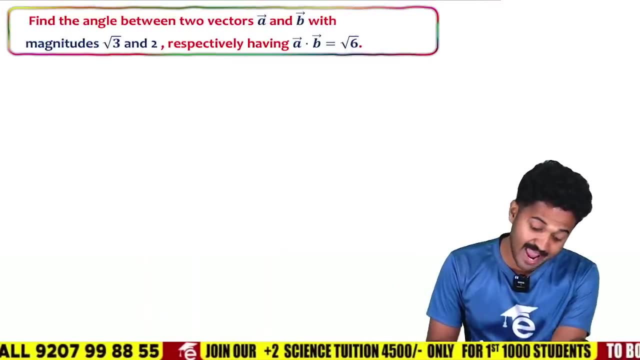 No, We have to do 0.. What happens if it is 0?? What happens? Yes, It is perpendicular, Ready, Okay, No problem, It is simple. Next question: Find the angle between two vectors, A and b, with magnitude root 3 and 2.. 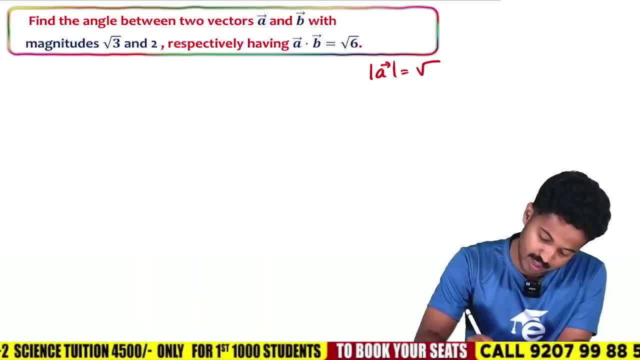 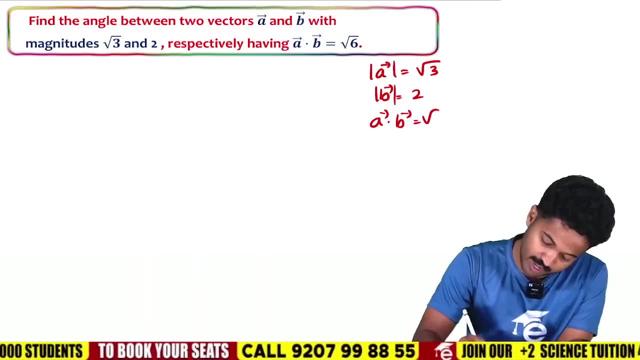 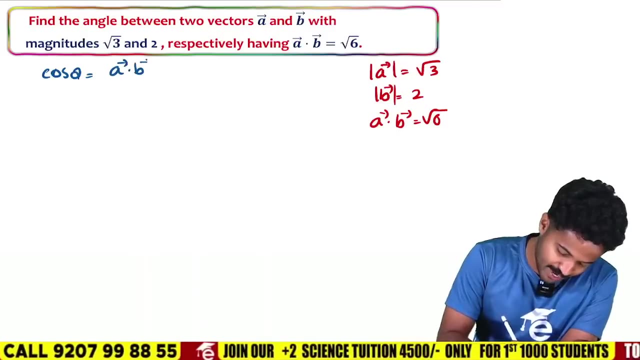 That is, magnitude a is root 3.. Magnitude b is 2.. And a dot b is root 6.. If so, it is easy to ask: angle between a and b Cos theta equal to What was the area there? a dot b by magnitude a into magnitude b. 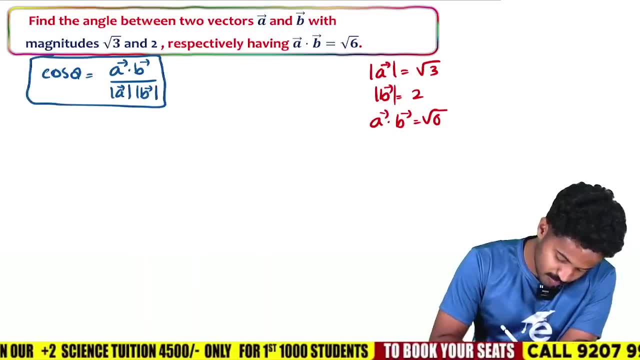 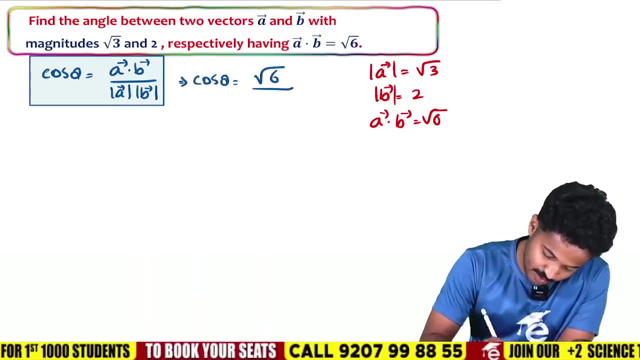 If you remember this equation, you can do this. Okay. If you remember this equation, you can do this easily. Okay. What is cos? theta equal to a? dot. b is root. 6 divided by magnitude a is root 3.. Magnitude b is 2.. 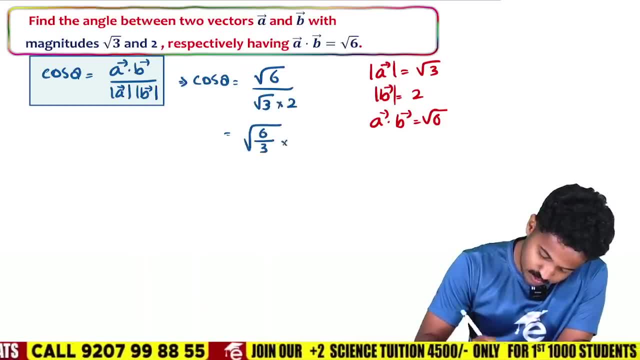 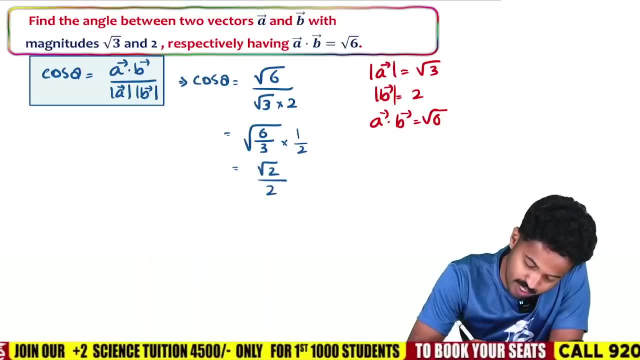 If you simplify it again, it is root 6 by 3 into 2.. That is 1 by 2.. That is root. 6 by 3 is root 2.. So root 2 by 2 is this. 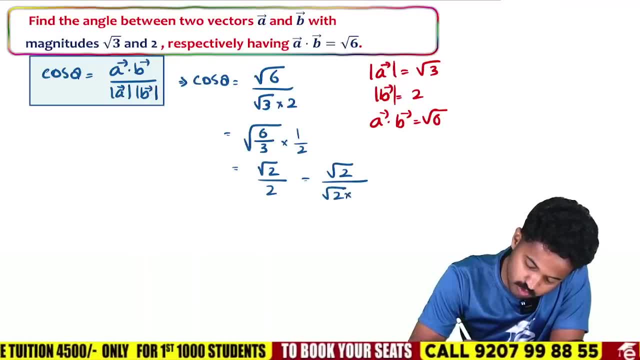 If you make it more interesting, root 2 by 2 is root 2 into root 2.. Oh, this, is it So. root 2 and root 2 are cancelled. So in the next step we will get answer. 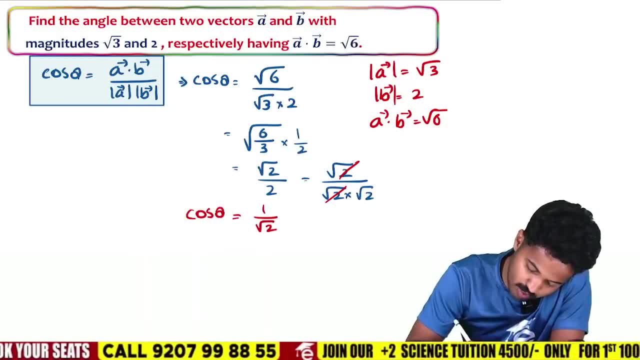 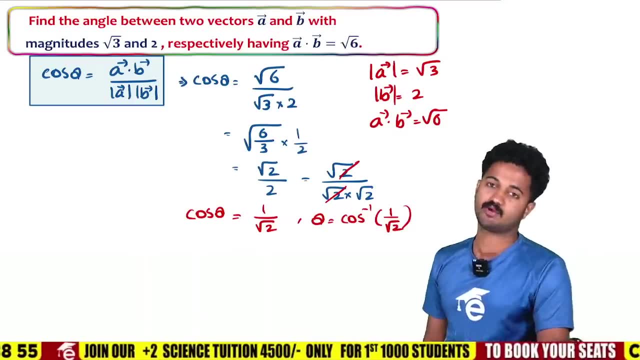 We will get 1 by root 2.. If cos theta is 1 by root 2, then theta is equal to cos inverse 1 by root 2.. Where is theta 1 by root 2?? Sorry, where is cos 1 by root 2?? 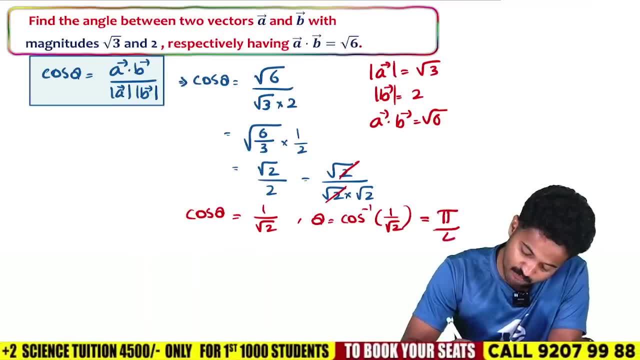 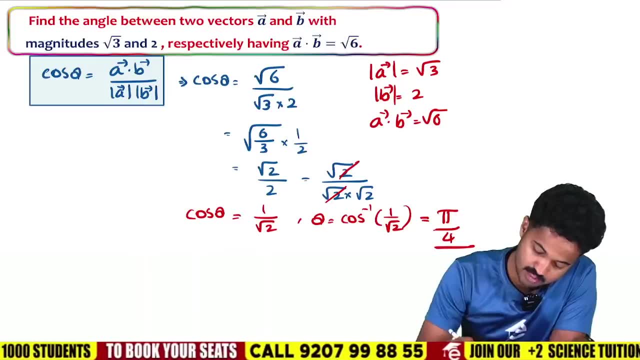 It is in pi by 4.. Simple Pi by 4 is 45. If it is 45,, then theta is 1 by 4.. Very good, Answer is 45.. Yes, very good, Simple, Easy. So that is the angle. 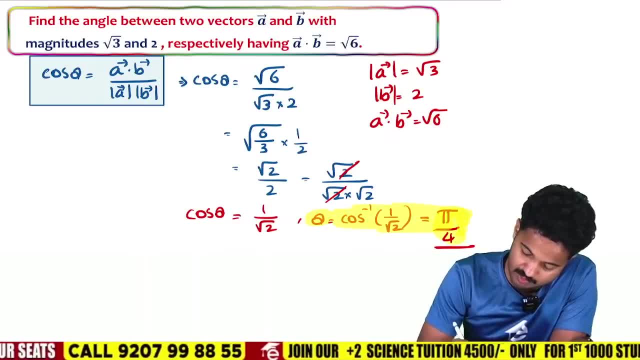 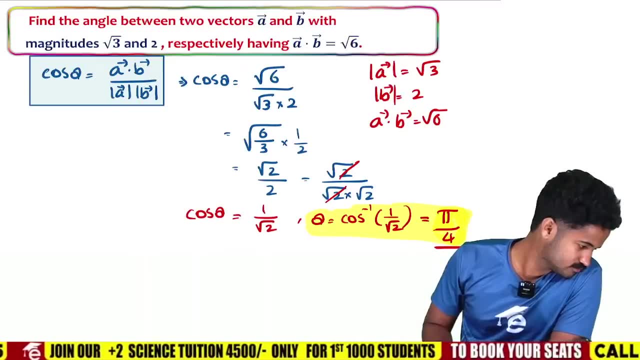 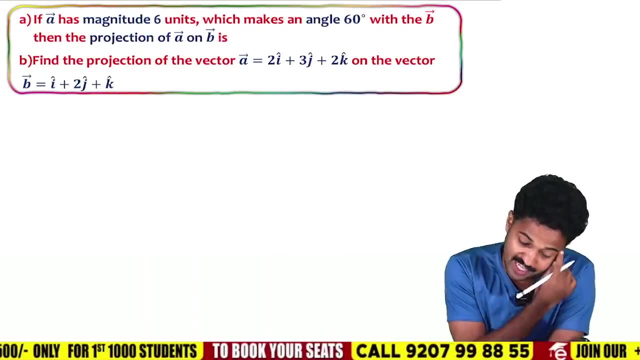 Pi by 4.. Theta is cos inverse 1 by root 2.. So the answer will be pi by 4.. It is easy. Okay, It is easy and simple. So that is how it is. Next, If A has magnitude 6 unit, which makes an angle 60 degree with B, 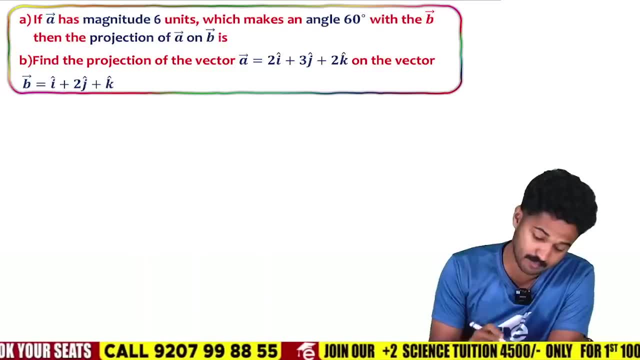 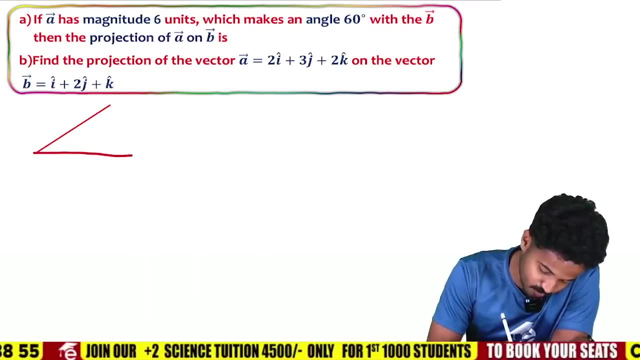 then the projection of A on B Projection. It is very important. You should have studied it, Sir. what is projection? I will tell you what projection is first. So you can find projection in two ways. Look, In my hand there is a vector called A. 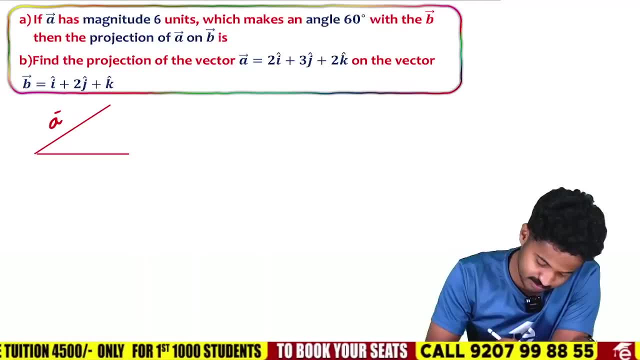 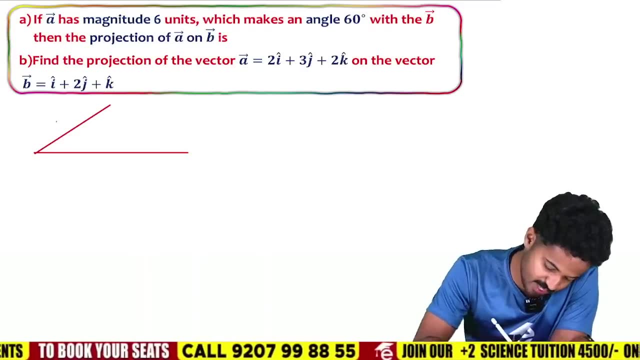 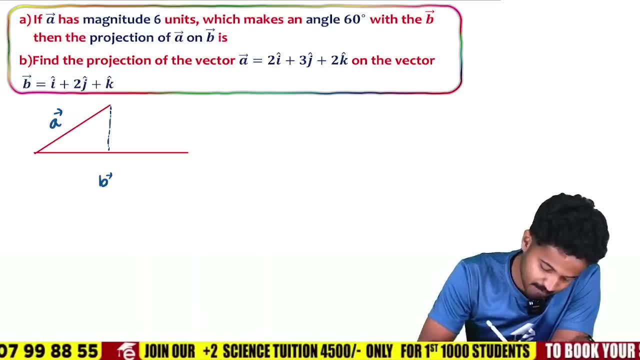 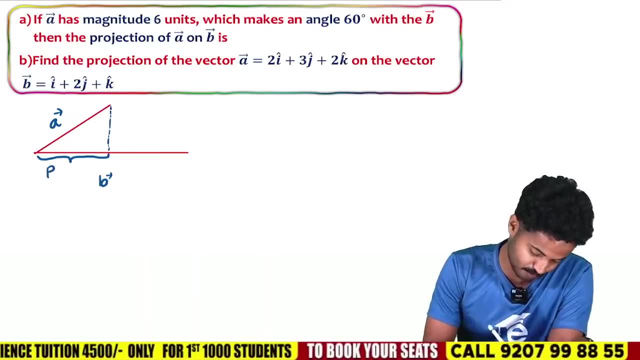 I drew a perpendicular from here to here. So the vector called A is called shadow. That is projection, So this is called projection. Okay, This is projection. So the B vector is at the bottom. This is B vector. 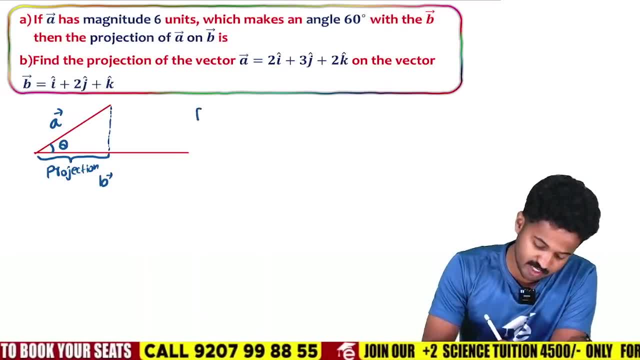 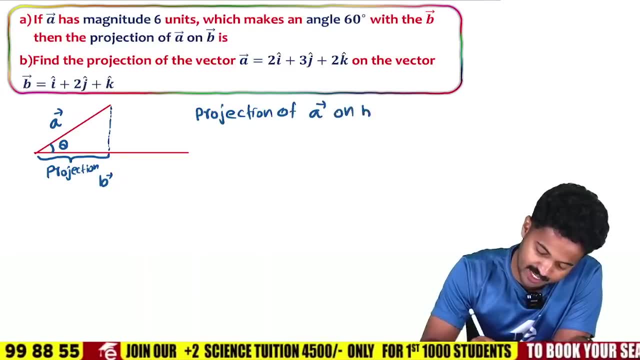 This is B vector And the angle between these are theta. So you need to learn the projection of the equation: Projection of A on B, The projection of A on B. If a projection is made in B, then this is one equation. 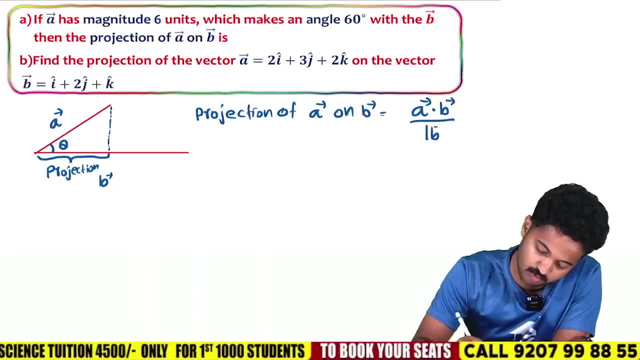 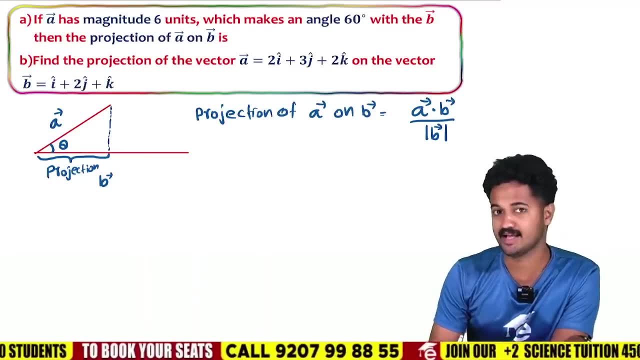 A dot B by Magnitude B. It is not necessary that you should know either it will come or not. Study the equation If the projection of A on B is A dot B by Magnitude B. Similarly, this is done If the projection of A on B is: 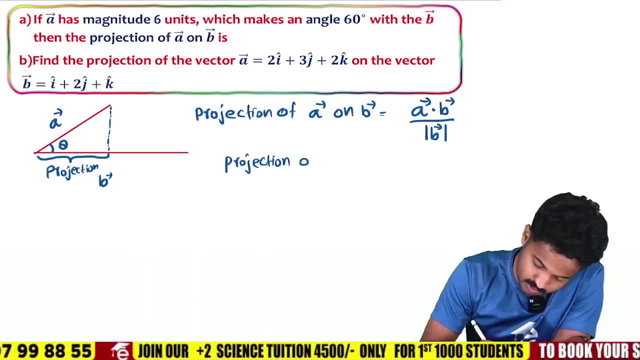 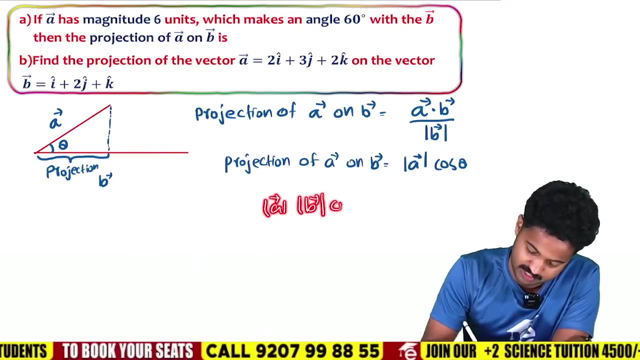 projection of A on B, of A on B. projection of A on B. then the next equation you write is: magnitude A cos theta, magnitude A cos theta. think about it: A dot B is magnitude A into magnitude B into cos theta. divided by. I have added a magnitude B. 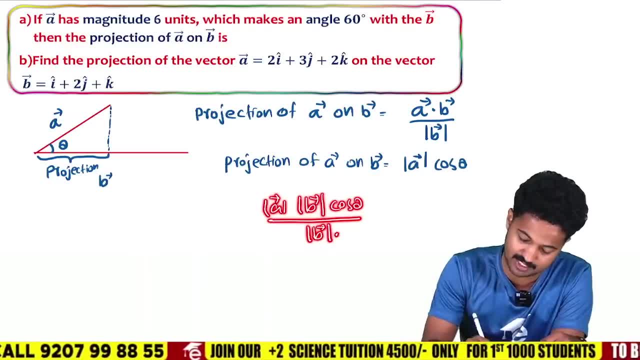 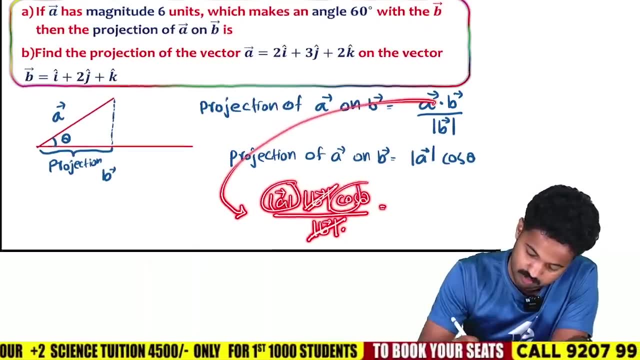 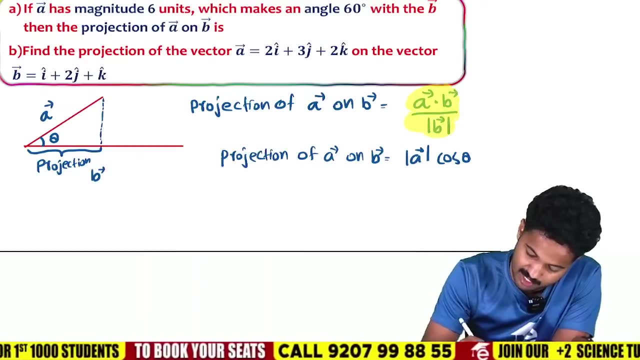 magnitude B. this is the projection. this magnitude B, this magnitude B is cancelled. then the answer is: root A cos theta. learn that there are two equations for projection. first one is A dot B by magnitude B, same as that magnitude A cos theta. these two equations are very important. 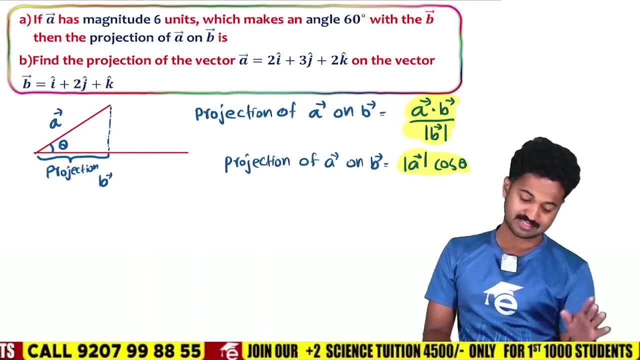 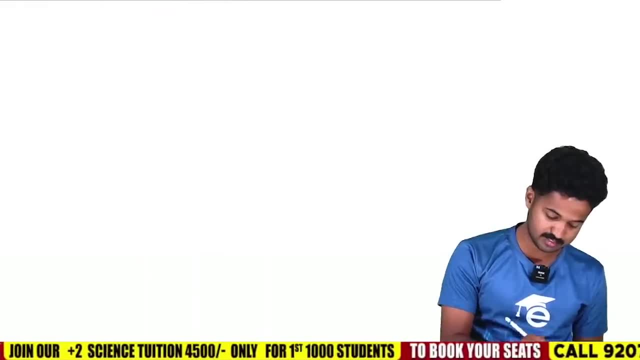 then look, if A has magnitude 6 unit, which makes an angle 60 degree with that is theta, then what is the answer of A first question? A's answer is easy. look: theta is equal to 60 degree and magnitude A cos, theta is equal to 60 degree. 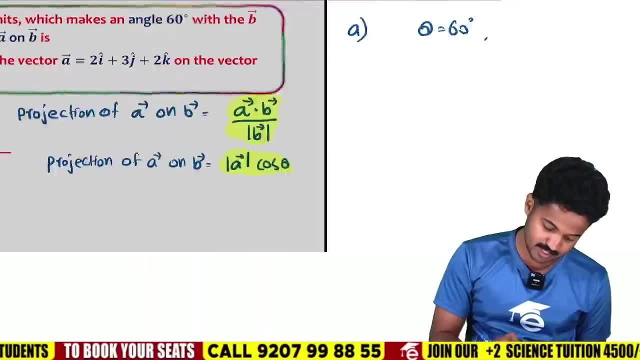 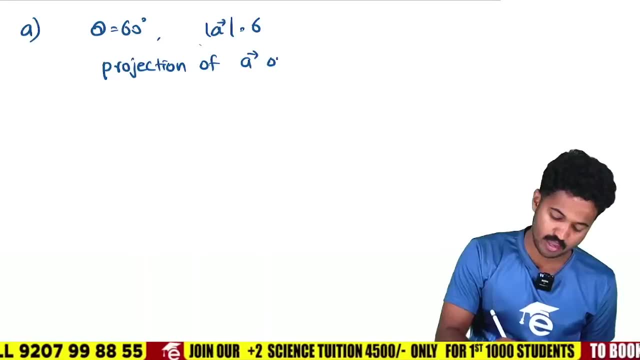 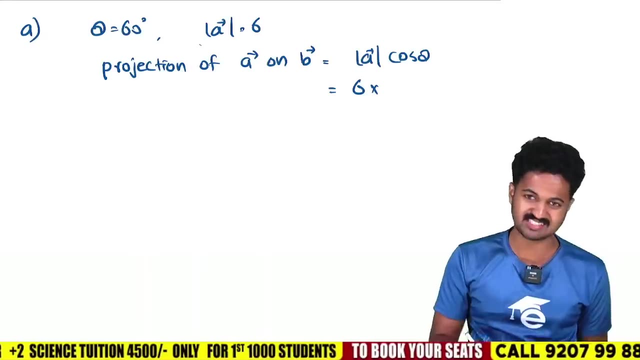 A equal to magnitude A is 60 unit. that is projection projection, projection of A on B. this is a question asked for an exam. if A on B, magnitude A, cos theta, magnitude A is 6, cos 60, cos 60 is 1 by 2. 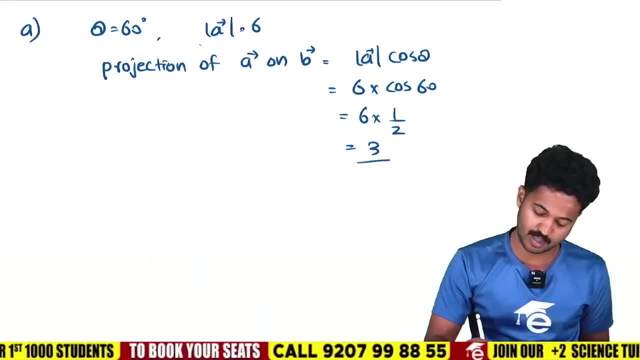 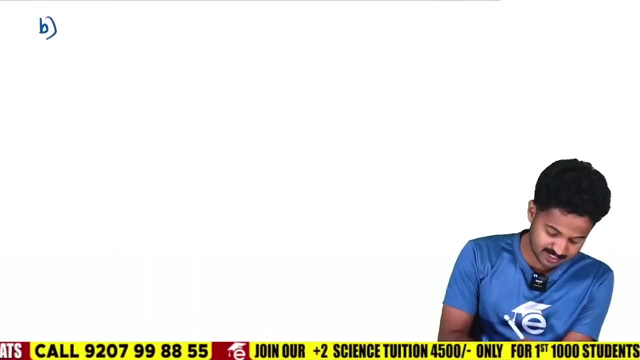 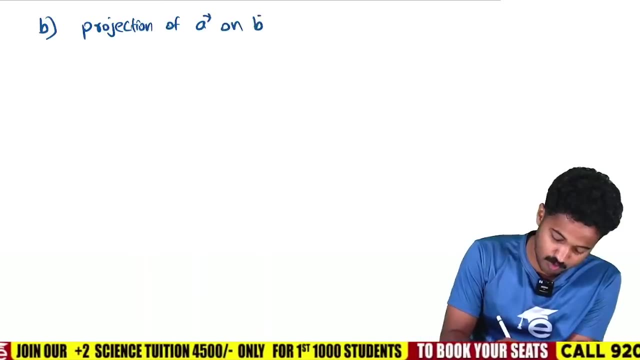 6 into 1 by 2, that is, the answer will be 3. this is projection 3. 3 is the projection same as that. 3 is the projection if we answer B question. projection of A by B. projection of A on B if we answer B question. 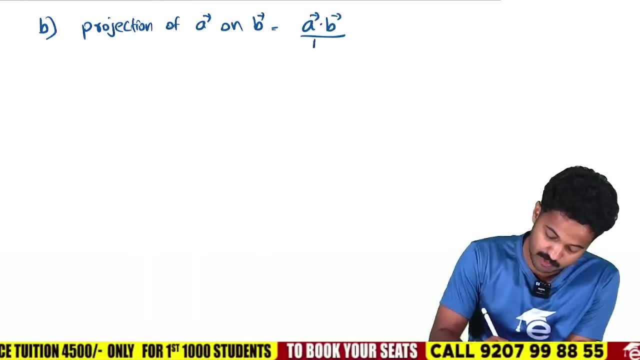 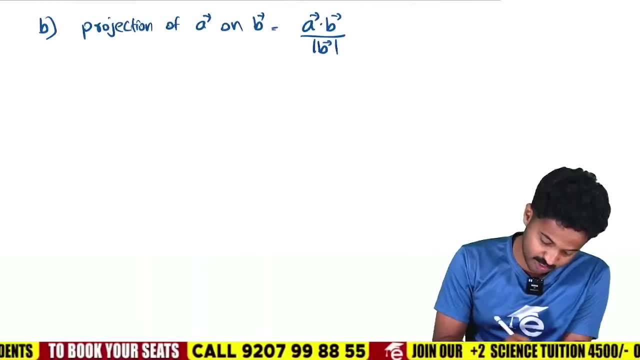 then we have to use this equation A dot B by magnitude B. this is because there we are given two vectors. A and B are vectors. we have to find A dot B first. so this is what is A and this is B. which vector is A? 2,, 3,, 2. 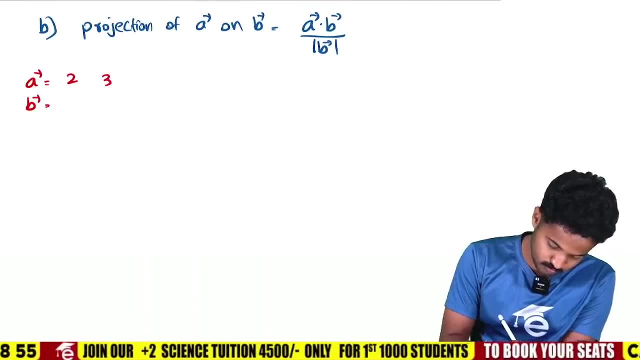 1, 2, 1, 2, 3, 2, 1, 2, 1, 2, 3, 2. I'm going to write 2 Ip's, if I can get A, b and B. 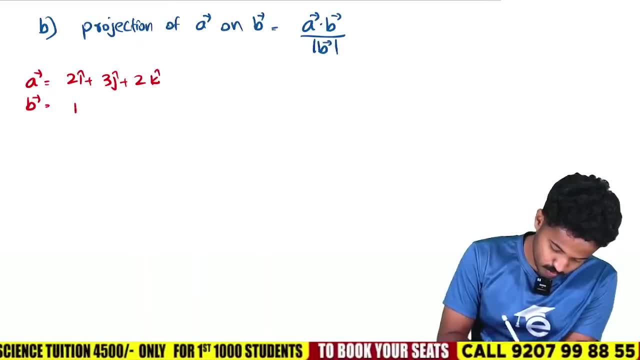 plus 3j plus 2k, 2, 3, 2, 1,, 2,, 1.. So i plus 2j plus k 1, 2, 1,, right, So i plus 2j plus k. okay, ready. 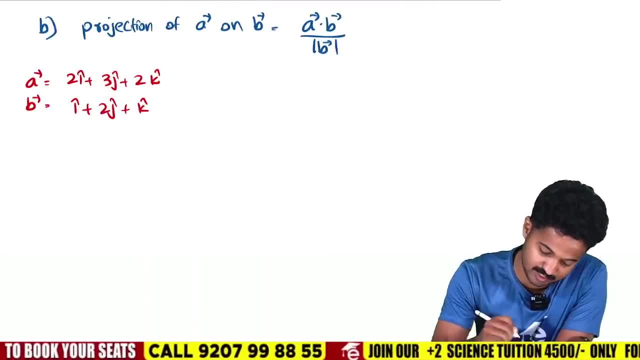 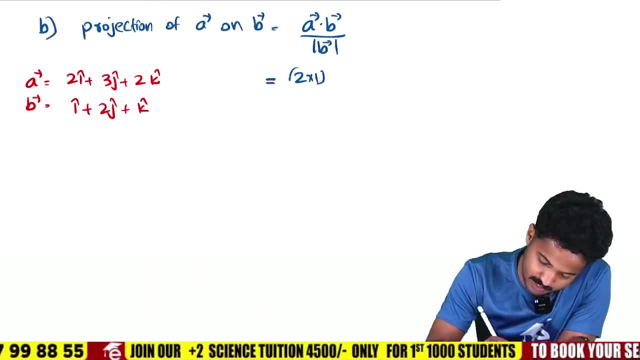 Now see what we need. here is: the first find we need to do is a dot b. So see, you can do it from here itself. a dot b is 2 into 1 plus 3 into 2 plus 2 into 1.. 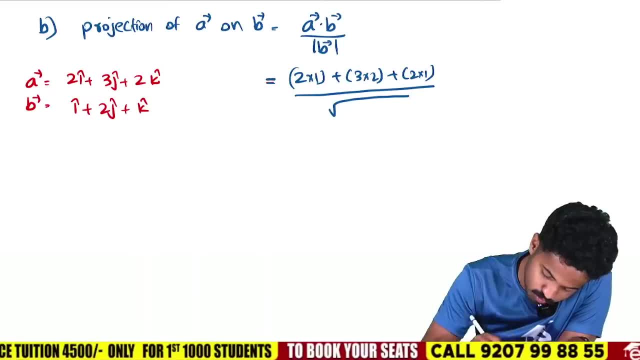 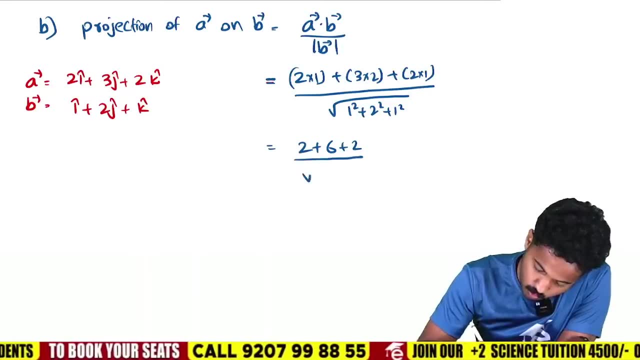 Similarly magnitude b. magnitude b is root of 1 square plus 2 square plus 1 square. So the answer is 2 plus 6 plus 2, divided by root, 1 plus 4 plus 4, sorry, 1 plus 4 plus 1.. 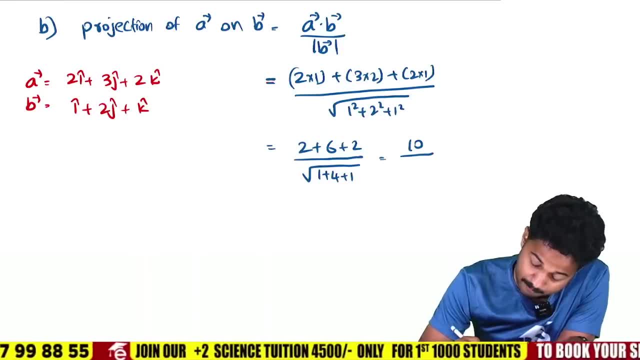 So we got the answer: 10 by 10 by 1 plus 4 plus 1 is root 6.. So your answer is 10 by root 6.. This is the projection. I told you that the projection is the shadow. 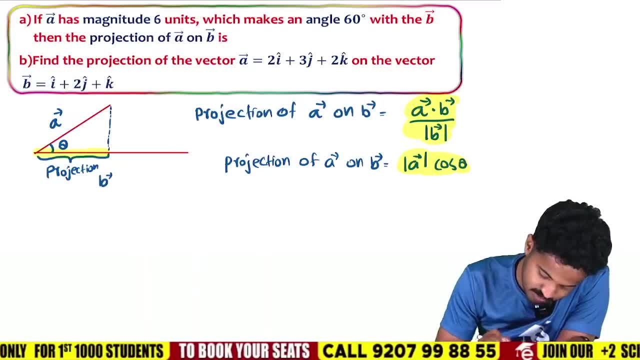 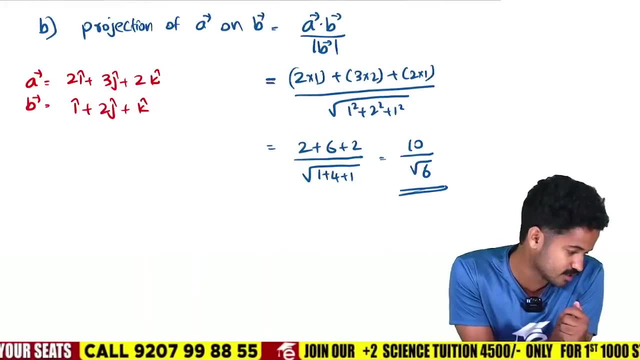 What do we give for this length? We give projection for this length, Okay. so that is the answer there: 10 by root 6.. Okay, 10 by root 6, right, Root 6, right, Okay, 10 by root 6.. 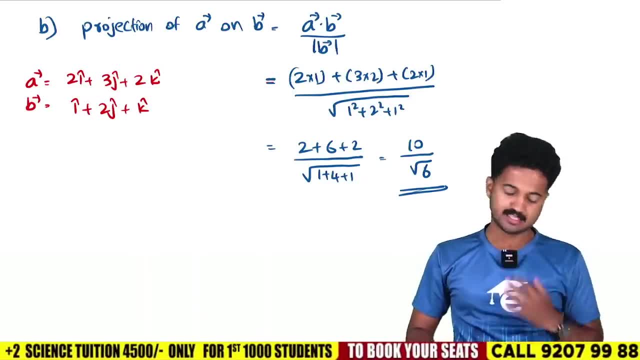 Okay, very good, very good. Okay, If you get it, quickly get a green ticket. If you get this, if this is okay, quickly get a green ticket. This is very simple. Now the next thing to learn is cross product. 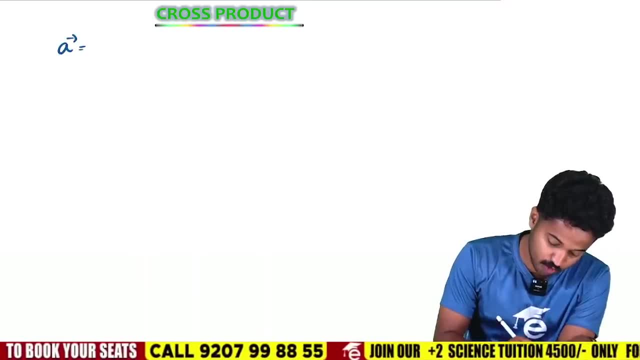 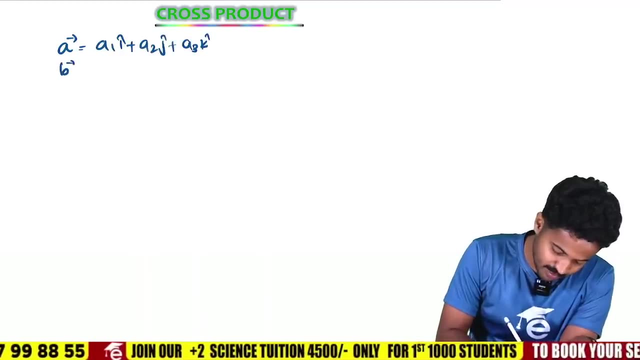 If you say cross product, you can think of the same thing. Cross product A is a1i plus a2j plus a3k, And b is b1i plus b2j. This is b2j plus b3k. 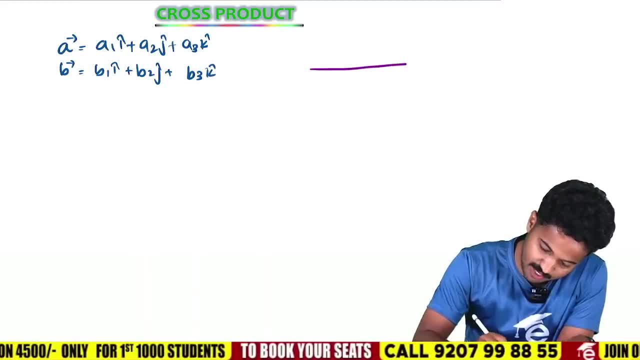 Let it be like this: As I said earlier, we consider two vectors. Look at this: We consider two vectors. This is the vector called a and this is the vector called b. Okay, So look at this: There is a vector called a and there is a vector called b in our hand. 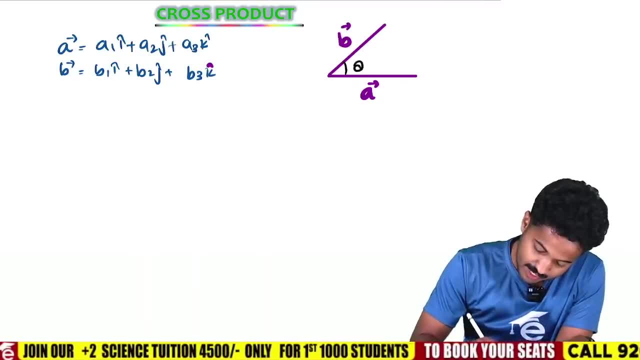 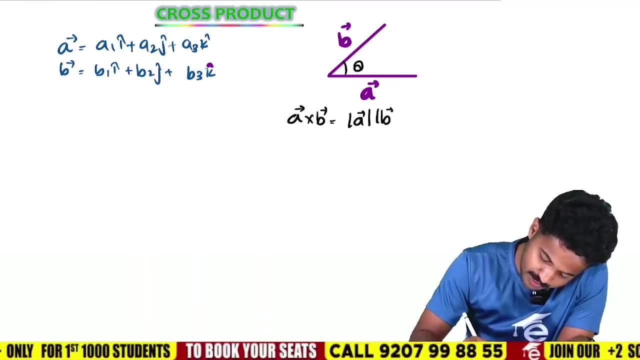 If that is the case, if we take the angle between these two and take the theta, do you know how to define a cross b, a cross b? a cross b means magnitude a, magnitude b, And here the effect is sine theta. 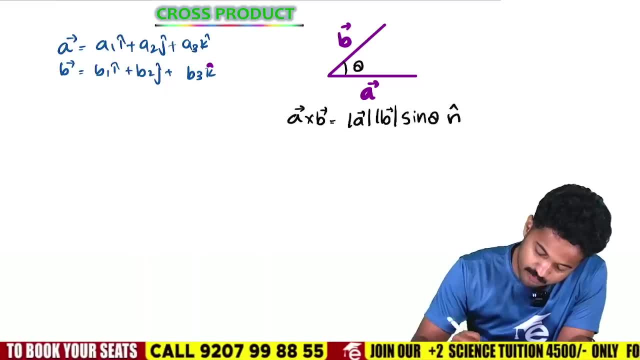 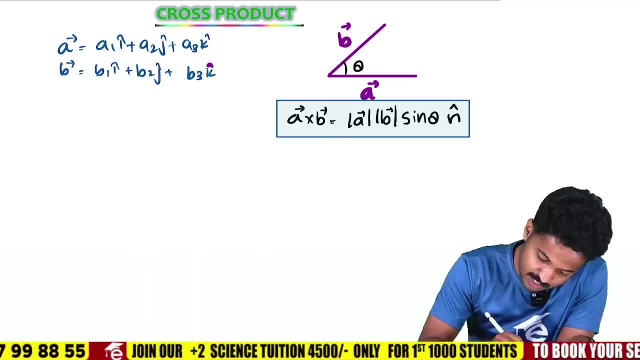 Last time I said: cosine here is sine theta And it will be multiplied into n cap. What is n cap? It is a unit vector. It is a unit vector, That's all. So here is the answer. Look at this. 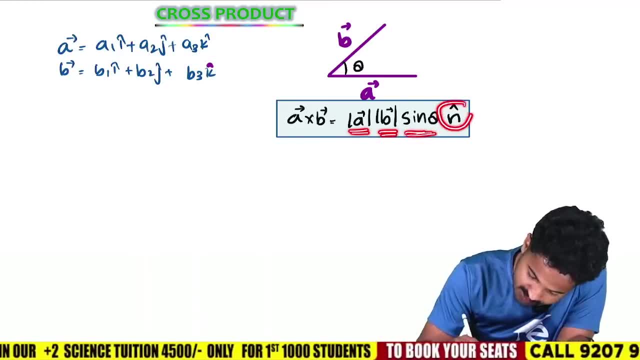 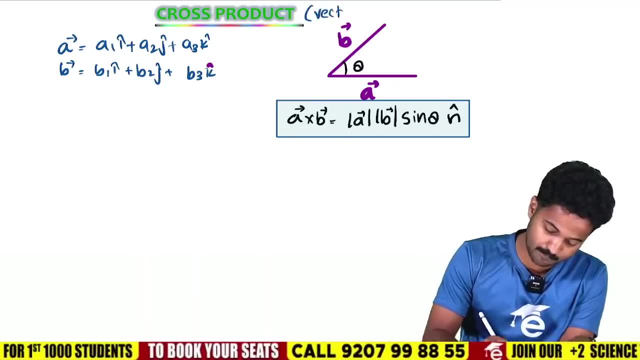 This is magnitude, This is constant, This is constant, This is constant. But when you multiply with this n cap, your answer will be a vector. So what do we call this? We call it vector product, Cross product or vector product. 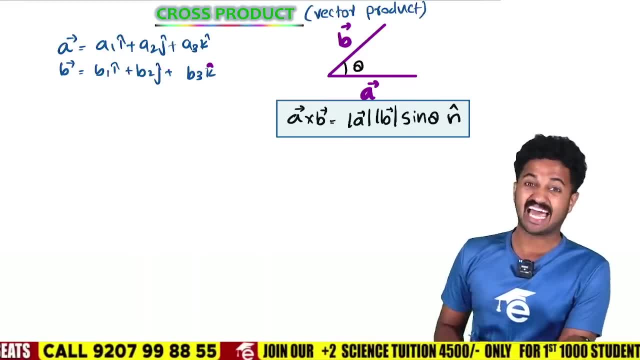 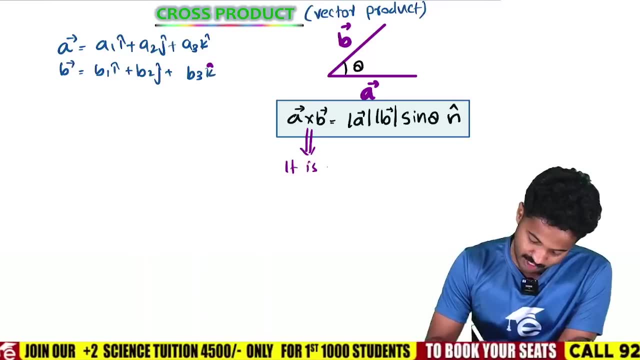 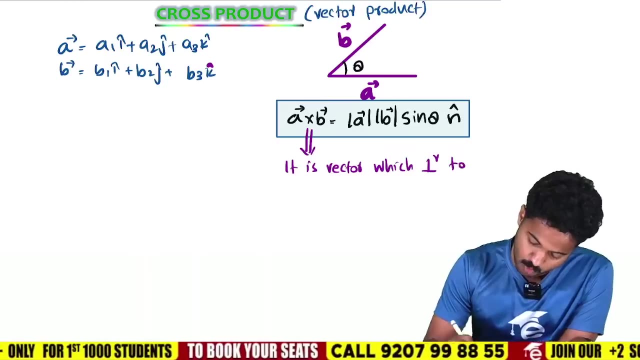 So understand this: A cross b is magnitude, a, magnitude of b, sine theta n cap. One more thing to think about This: a cross b, it is a vector which is perpendicular to both a and b. This is the question asked. 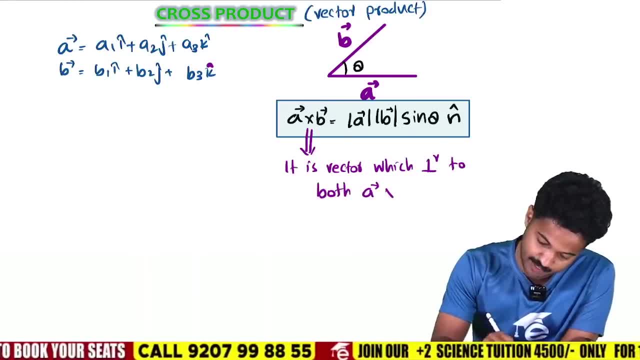 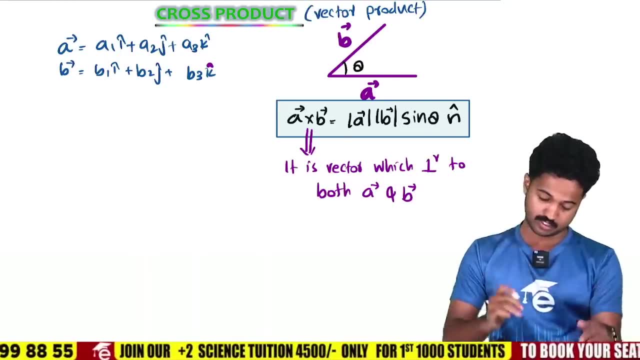 Find a vector which is perpendicular to both a and b. A and b are perpendicular to each other. That would be a cross b. That is important. Think about that. This is how we do a cross b problem. We take our determinant. 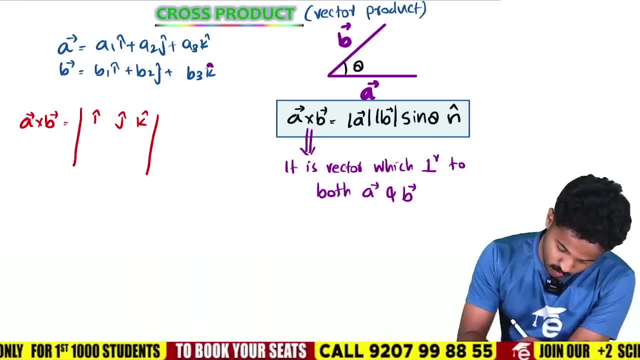 We put i, j and k in it, Then we put a1, a2, a3 and b components b1, b2, b3.. This is how we do it. This is the method we use to find cross product. 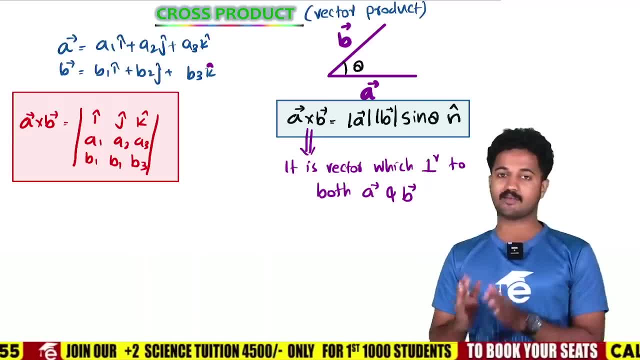 This is the method we use to find cross product. We learned two equations: Magnitude i, magnitude b, sine theta n cap. Then we put i, j, k in the determinant A, components a1, a2, a3. 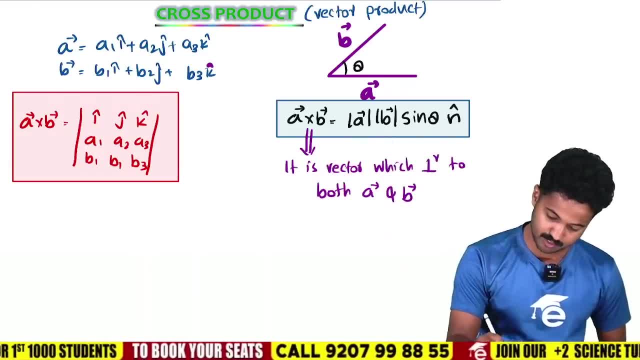 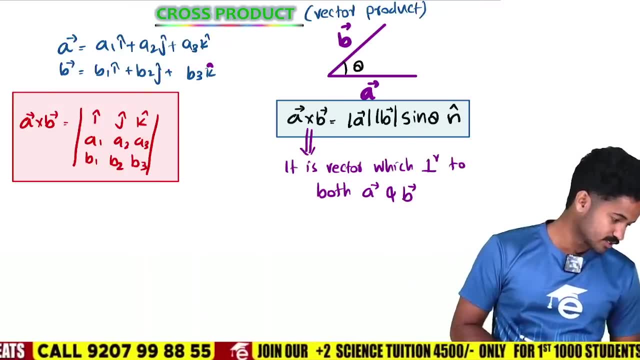 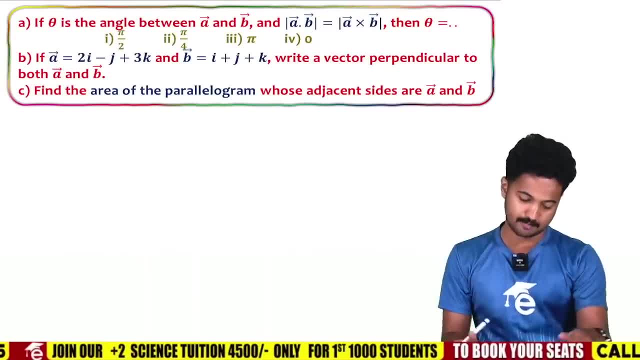 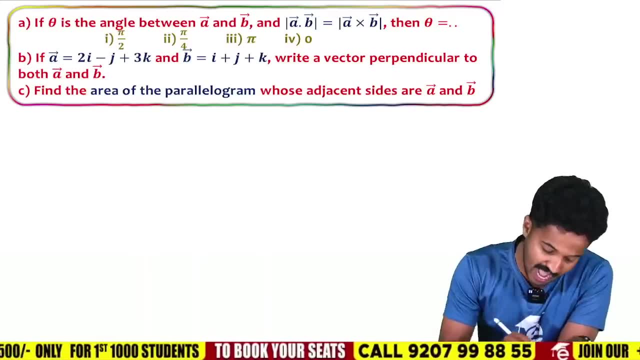 What will you get if this is the number A cross b? Let's see. This is easy. If theta is the angle between a and b, Find magnitude of a dot b and magnitude of a cross b. Let's see how to do it. 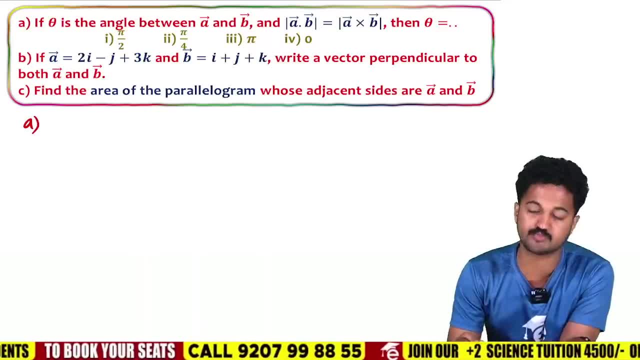 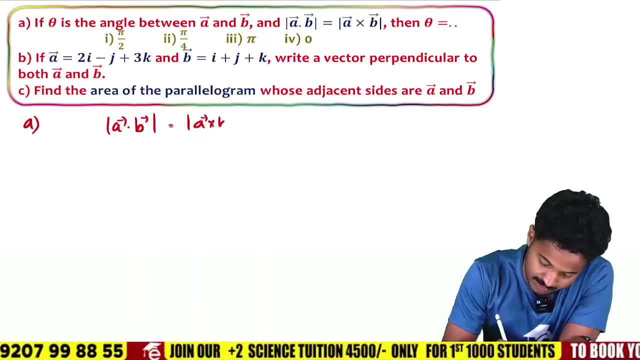 Easy. If magnitude of a dot b and magnitude of a cross b is equal, what is theta If magnitude of a dot b and magnitude of a cross b is equal? what is theta If magnitude of a dot b and magnitude of a cross b is equal? 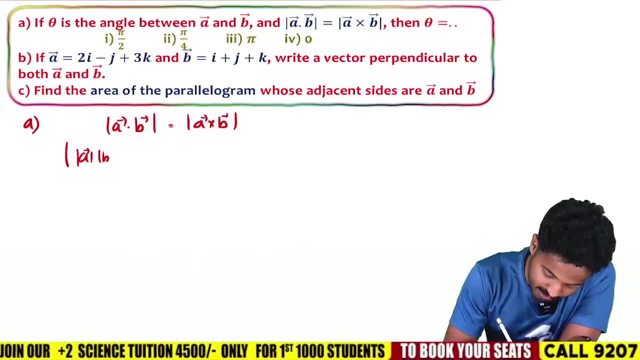 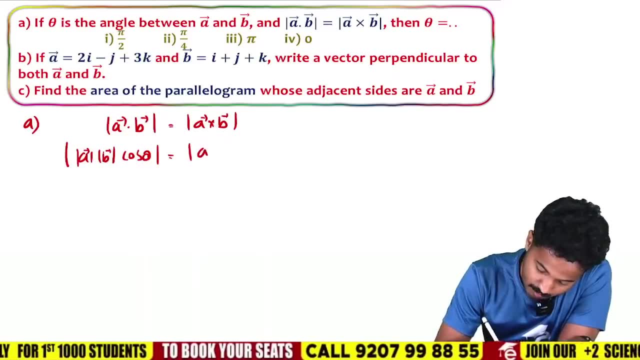 what is theta? See A dot b is written like this: Magnitude A, magnitude B cos theta. Okay, Equal to That's it No problem If this is: magnitude A cross B, magnitude A, magnitude B sine theta. sine theta. 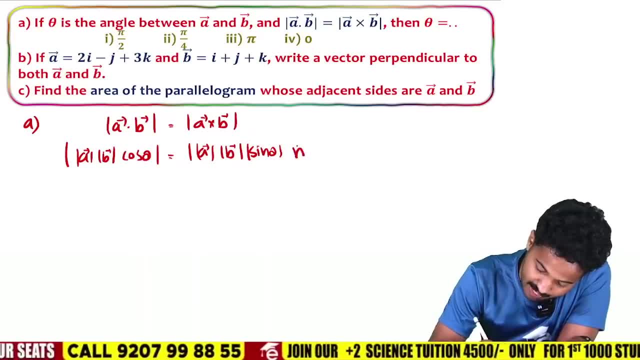 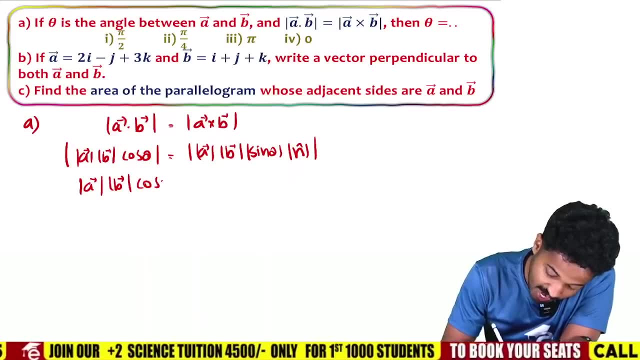 magnitude of that and n cap the magnitude of that n cap. You can write it like this: Magnitude A magnitude B cos theta. You can write it like this: Magnitude A magnitude B sine theta. Magnitude A magnitude B sine theta. 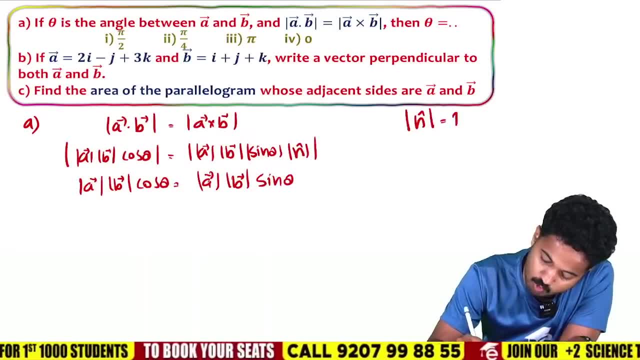 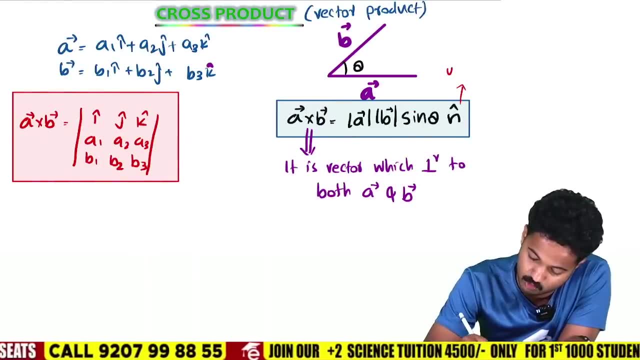 What is the magnitude of n cap? n cap is a unit vector, Isn't it? I told you that n cap is a unit vector. What is n cap? n cap is a unit vector, So its magnitude will always be 1.. 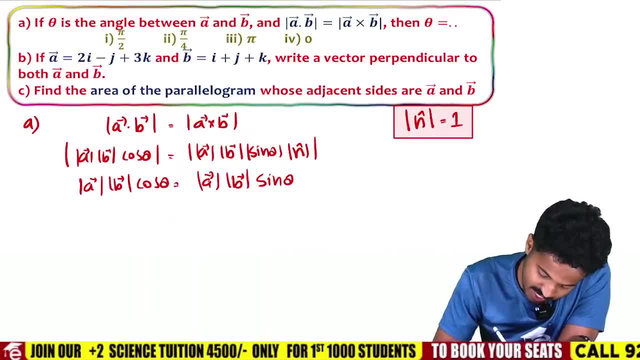 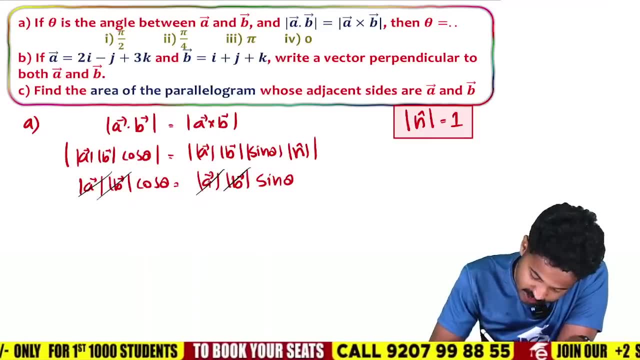 And you can write it like this: So see: 1. This magnitude A and this magnitude B will be cancelled. That is cos theta equal to sine theta. Easy, If this cos theta comes here. 1 equal to sine theta by cos theta. 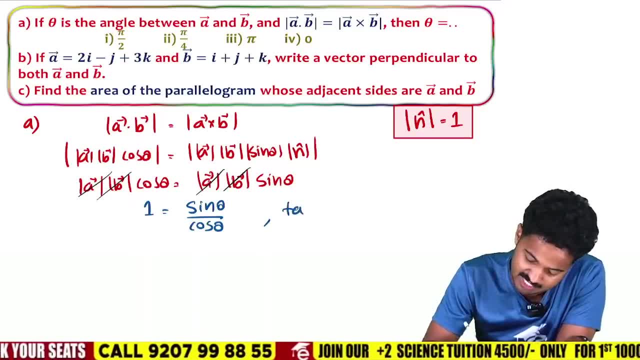 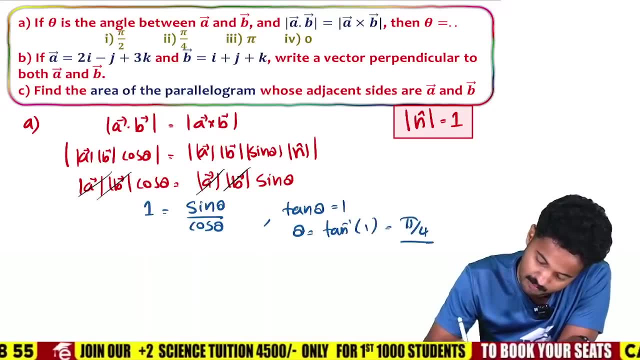 What is sine theta? by cos theta, tan theta. If tan theta is 1, theta will be tan inverse 1.. tan inverse 1.. Where is tan 1? In pi by 4.. So what is the answer to this? 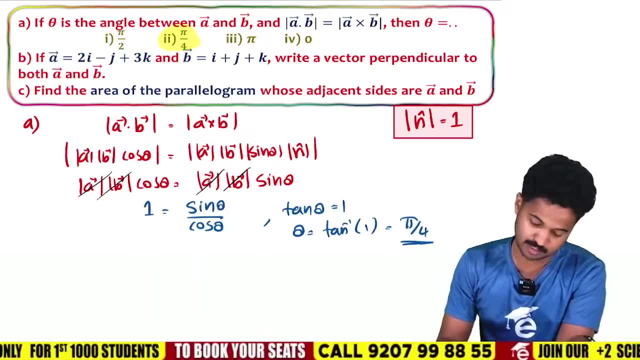 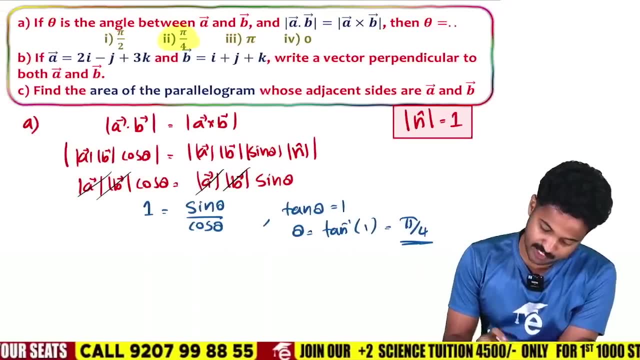 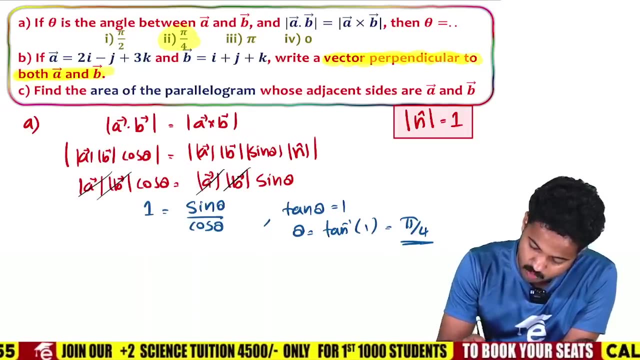 That is pi by 4.. Yes, Yes, Very important. See: A equal to a vector, B equal to a vector. Write a vector perpendicular to both A and B. Write a vector perpendicular to both A and B. So we have to find that. 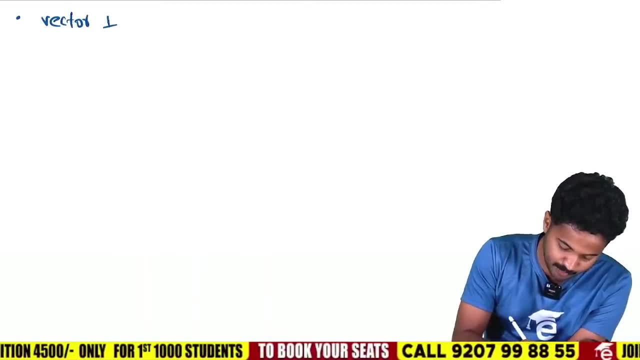 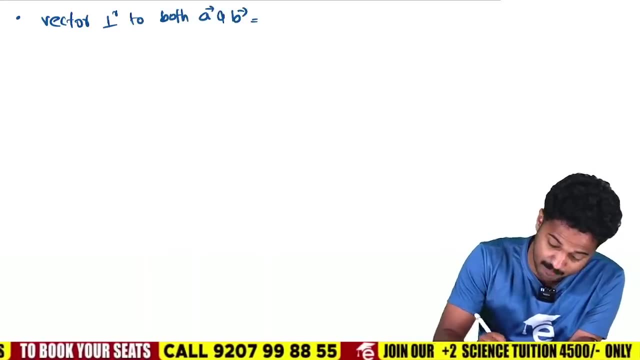 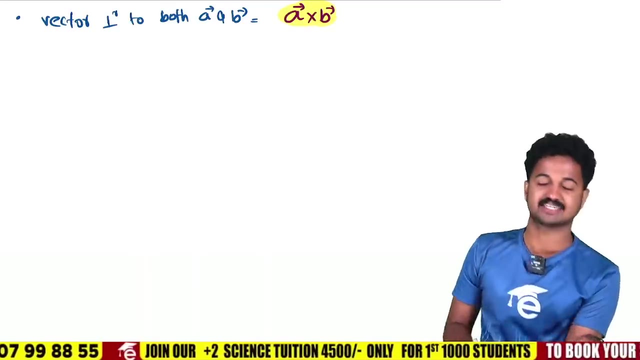 So see: Vector: perpendicular to both A and B. A and B are perpendicular. How can we find that A cross B, A cross B is perpendicular to A and B is easy: If we say A cross B, A will be perpendicular and B will be perpendicular. 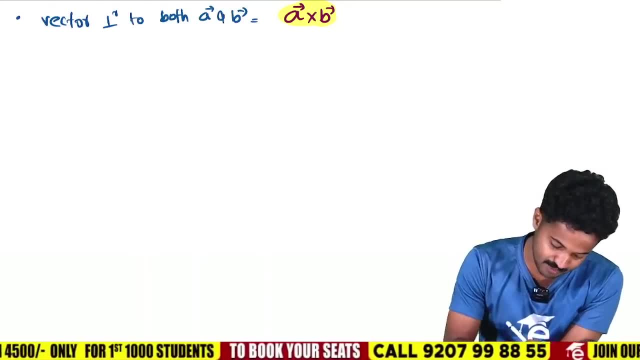 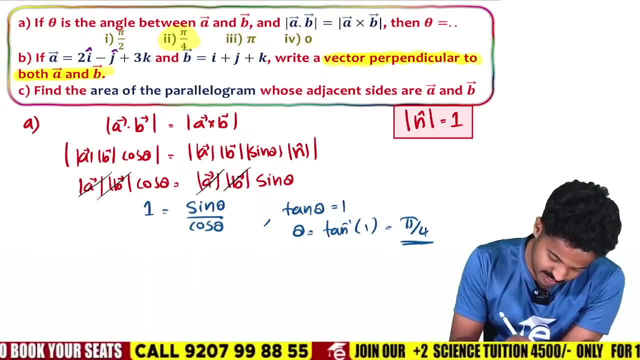 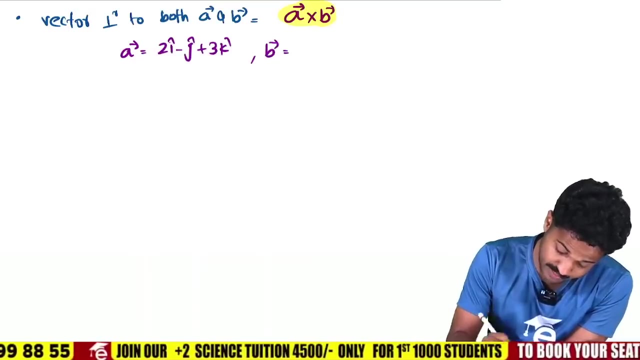 A cross B is the vector we get. If so, you can find the answer simply: What is A? What did A give here? 2I minus J plus 3K, 2I minus J plus 3K, and what is your B? 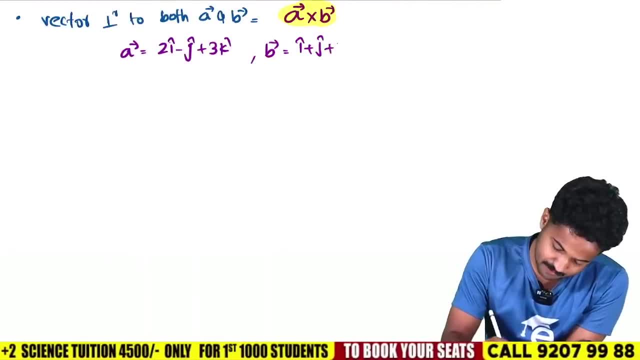 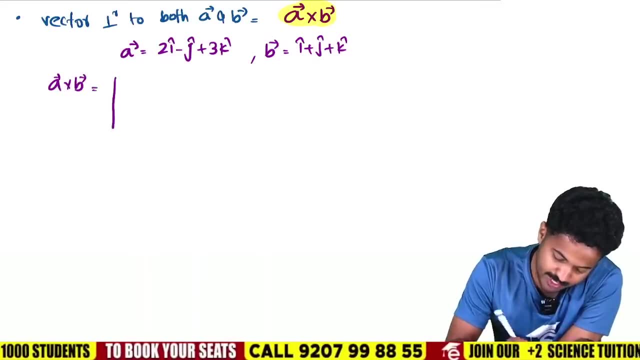 What is your B? I plus J plus K. I plus J plus K, What is A cross B? A cross B is a very nice letter. It is very nice. A cross B is IJK Ready, Ready. 2 minus 1 is 3. 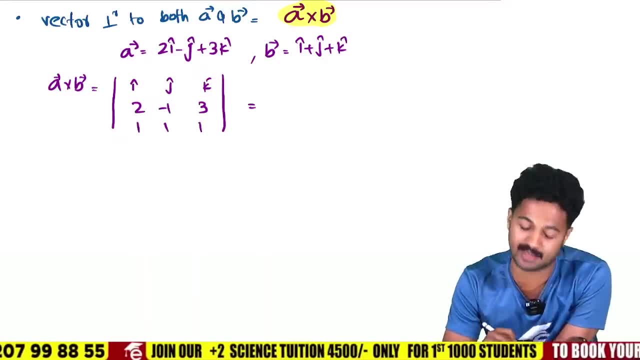 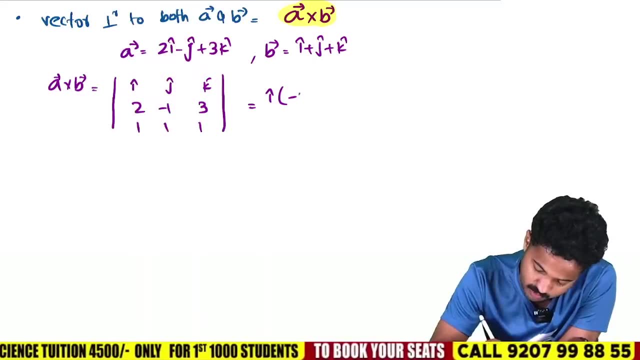 1 is 1. How do we find it with a determinant I? 1 into minus 1. 1 into minus 1 is minus 1. minus 1 into 3 is 3. You know it right For the second one. 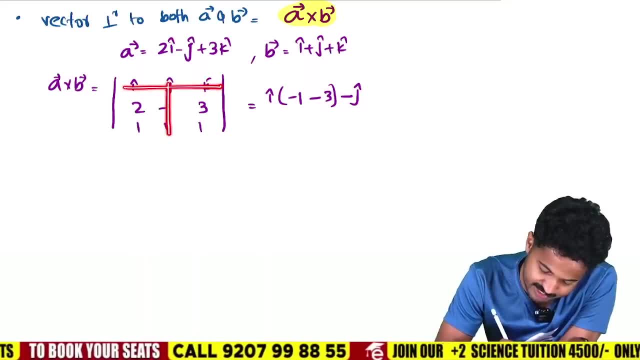 minus 1 is 3 minus 1 is 3 minus 1, is 3 minus j. It is a determinant. It is purely a determinant. It cancels the rowing code 2 into 1, 2 minus 1 into 3, 2 into 1. 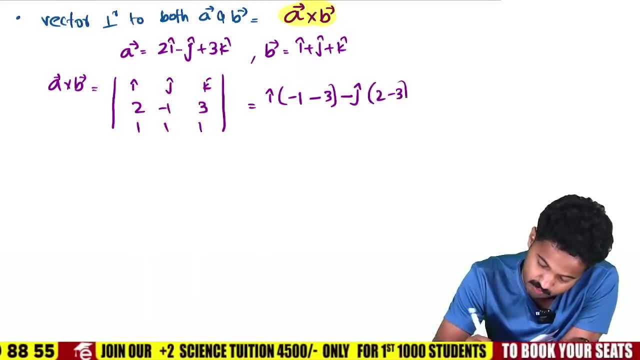 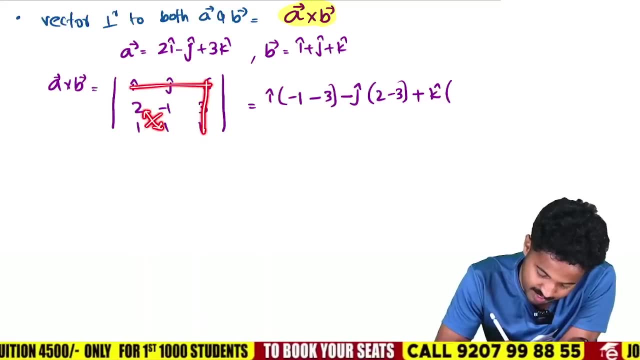 2 minus 1 into 3. 2 minus 3 plus. for the next one plus K. The next rowing code cancels it. 2 into 1 minus 1 into minus 1. 2 into 1 means 2. Your answer is: 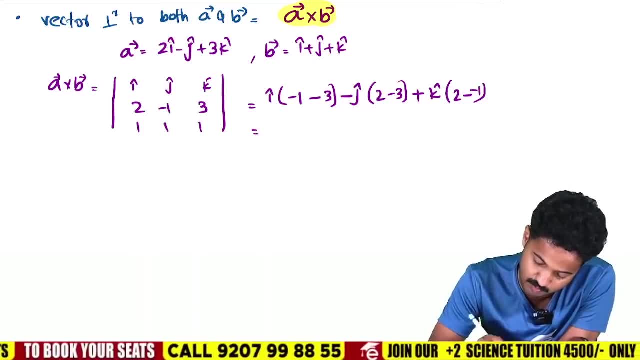 2 minus 1 into minus 1 means minus 1. So the answer will be: minus 1 minus 3 means minus 4, minus over I. 2 minus 3 minus 1 minus 1 into minus j plus j. okay, plus k into 2 minus minus 1. 2 plus 1, that is 3, that is: 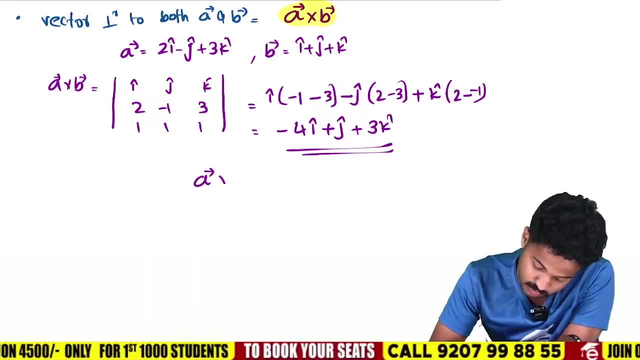 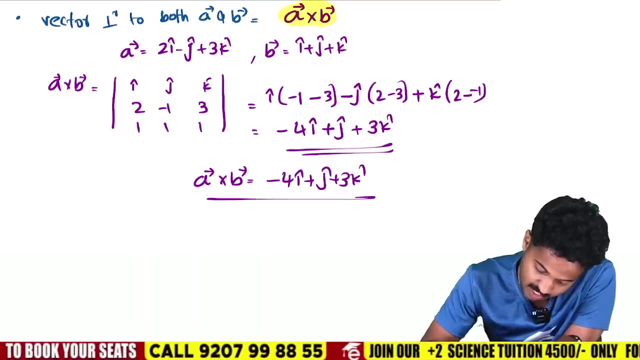 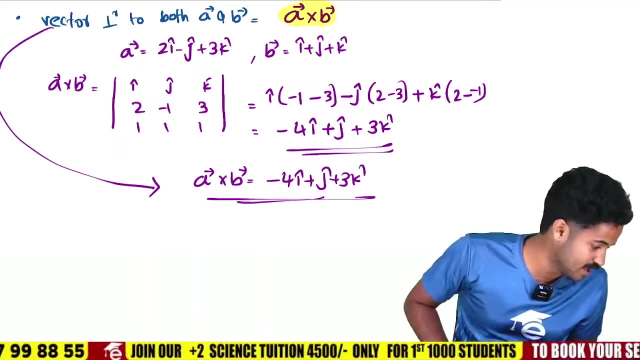 3k. so what we got? what we got: a cross b. we got a cross b is minus 4i plus j plus 3k. this is what a and b are perpendicular. a and b are perpendicular. a vector, that is a cross b, magnitude: a cross b. 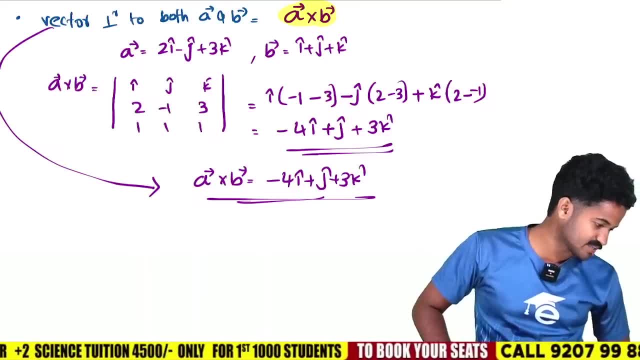 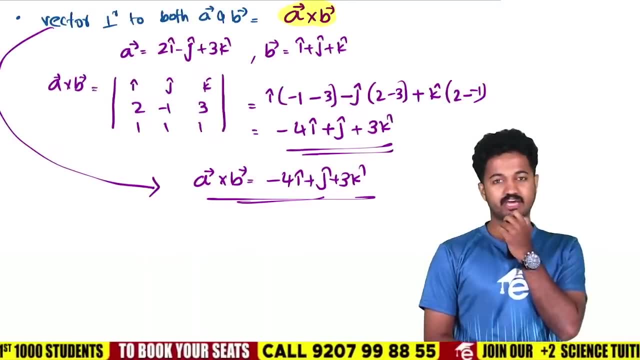 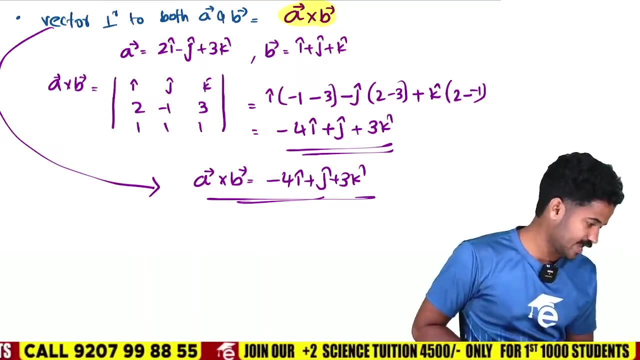 right, right, when that class is over, we have 7 hours left now. if we do this for 2 more days, your cross product is over, and then after that, after 30-35 minutes, 3d will also be over. so ready, okay, we are getting it right. we are getting the answer: vector perpendicular to both a and b. 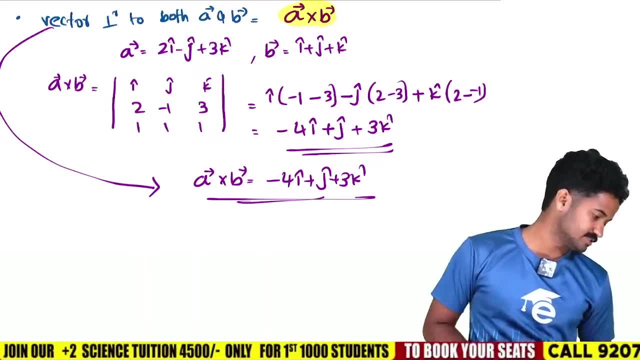 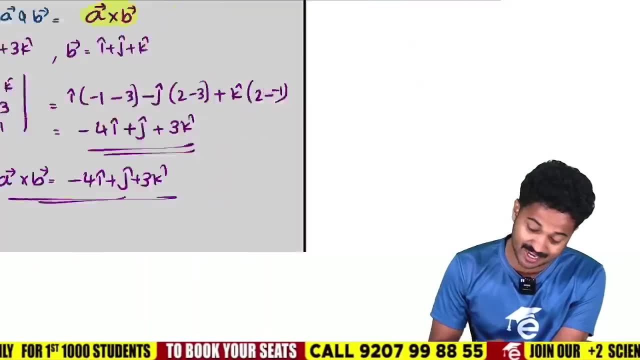 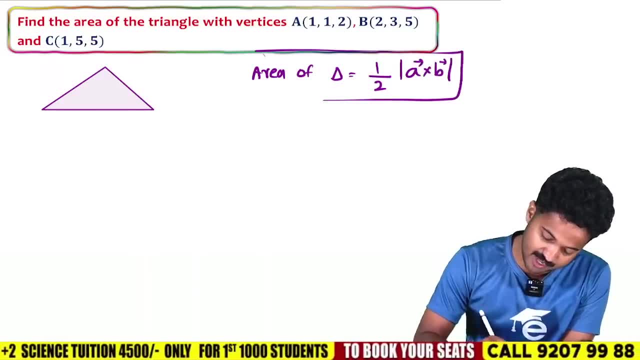 you have got a parallelogram whose adjacent side are a and b. that is easy. If it is a diagram, it is the magnitude of A cross B. If it is a triangle, it is half into A cross B. So look here. 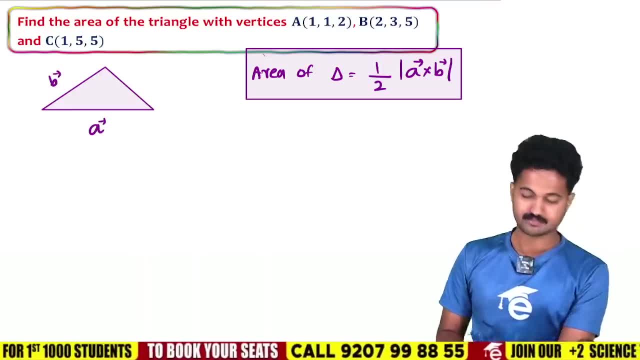 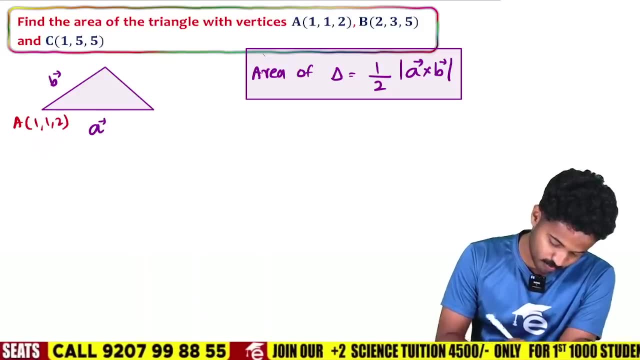 One vector. this vector is A and this vector is B, So we get A. So what is given here? Here the position vector of A is given as coordinate 1, 1, 2.. B is given here as B. 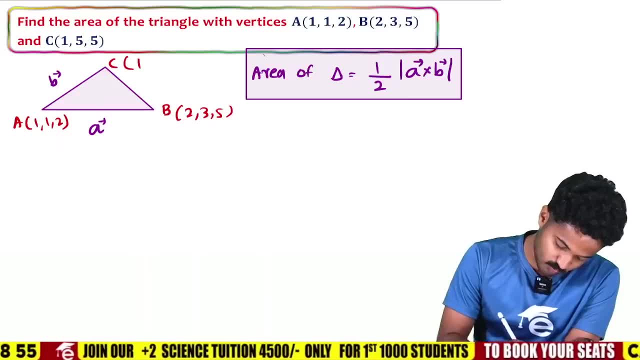 B, 2,, 3, 5.. And C is given as 1,, 5, 5.. So we have to write two vectors, First the vector A. How to write the vector A. How to write the vector A. 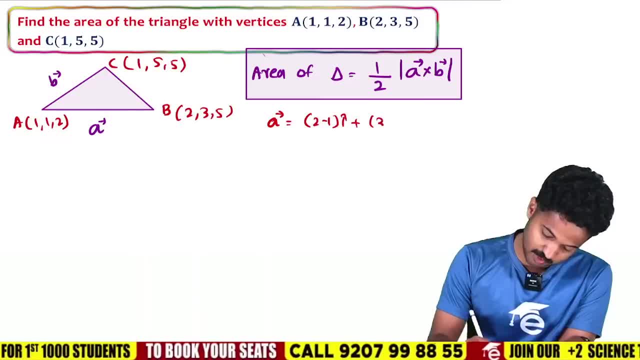 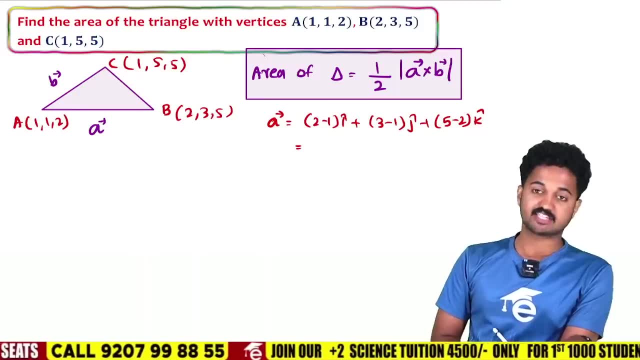 Simple: 2, minus 1, I plus 3, minus 1, J plus 5, minus 2.. So you know that it is a vector given by two points. So it is A vector. When we say A vector, we have to find AB. 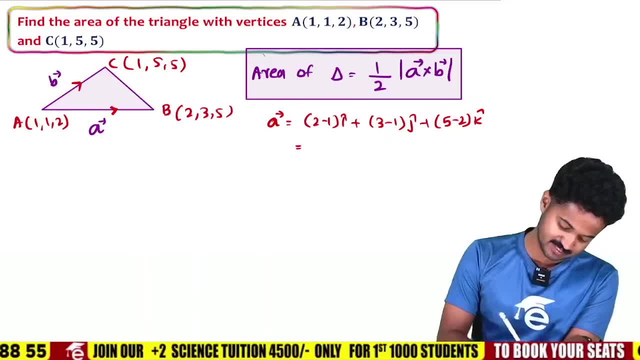 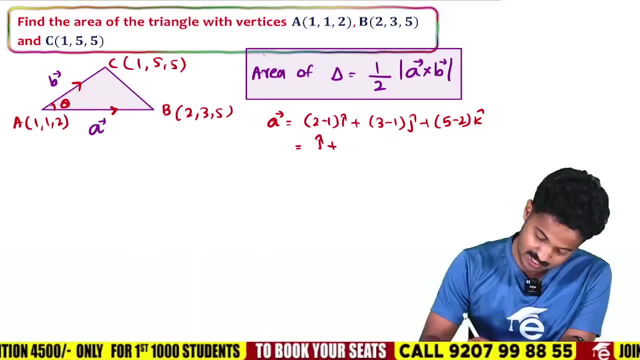 AB, AB, And we have to find AC, AC. If the angle between these two directions is the same, then our area becomes half into A cross B. So look here: I plus 2J, plus 5, minus 2, 3.. 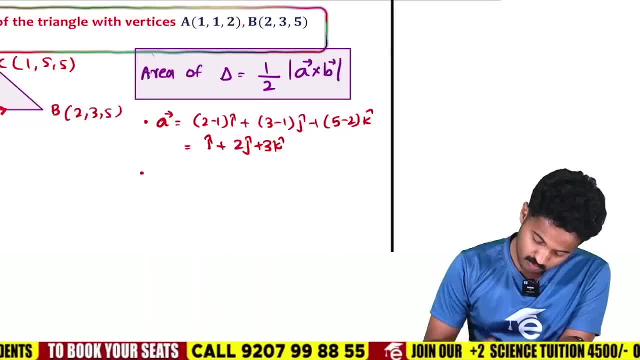 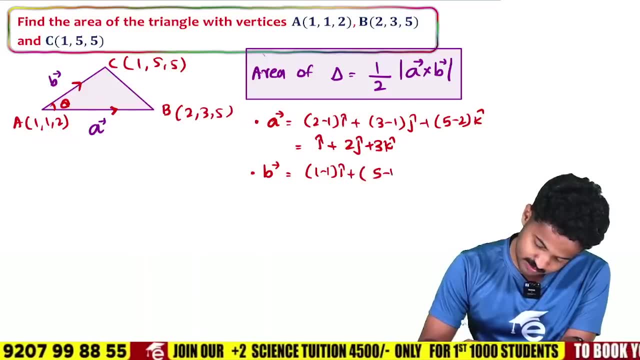 So 3K. So we get A. Now find B. What is B? What is B? B is 1, minus 1, I plus 5, minus 1, J plus 5, minus 2, K. 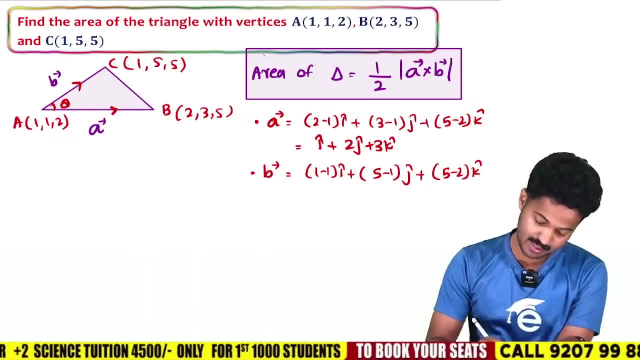 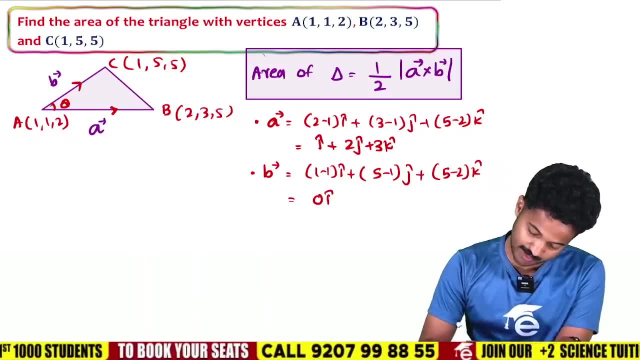 OK, If B is AC, then we have to find AC. If B is AC vector and A is AB vector, then the answer is 0, I plus 4, J plus 3, K. OK, Easy. 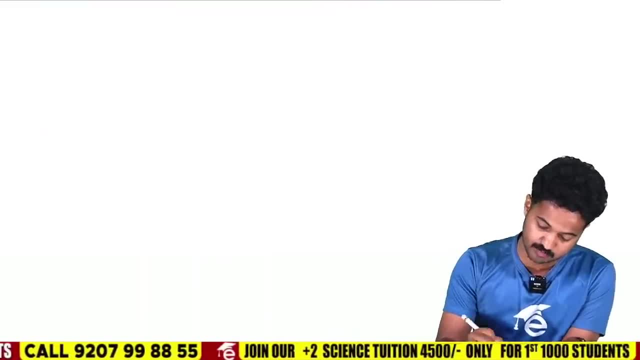 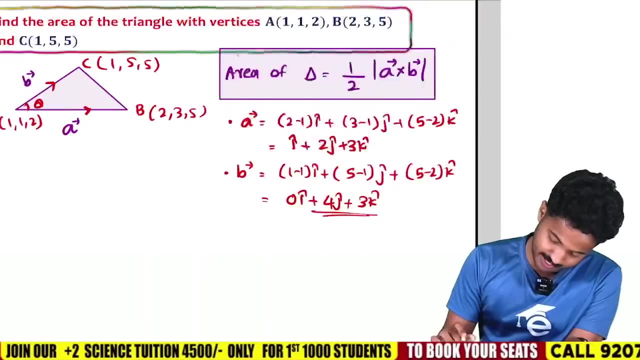 Ready. If we want the area, we need A cross B. So first let's find A cross B. Let's find A cross B. A cross B equals to I, A cross B equals to I, J K and 1, 2, 3, 1, 2, 3, then. 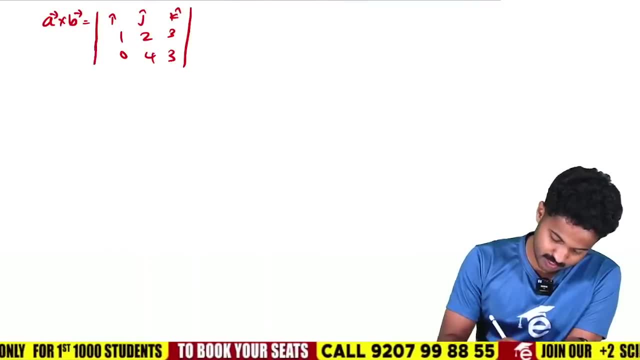 the same way: 0, 4, 3, 0, 4, 3.. OK, Easy. So look here I into cross multiply. This is row cancel: column cancel: 2 into 3, 6 minus 3 into 4, 12, minus J into row cancel. 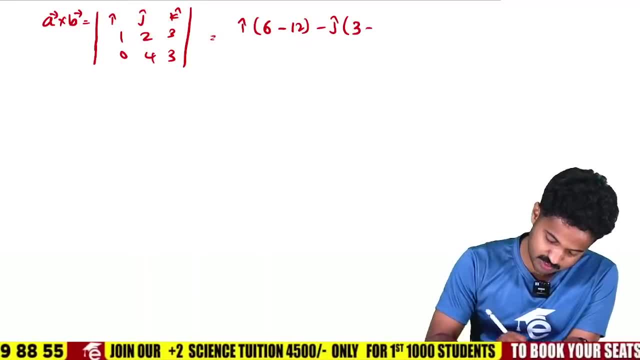 column cancel: 1 into 3, 3, 3, minus 0 into 3, 0, plus K into row cancel. column cancel. So look here: 1 into 4, 4, minus 2 into 0, 0.. 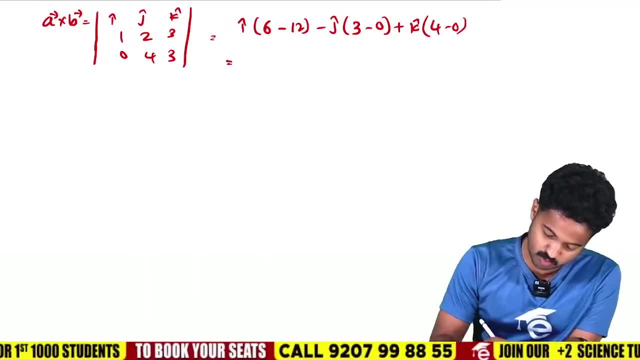 4. 4 minus 0 into 0. So the answer will be 6 minus 12, minus 6. So minus 6, I, 3 minus 0, 3. So minus 3, J. 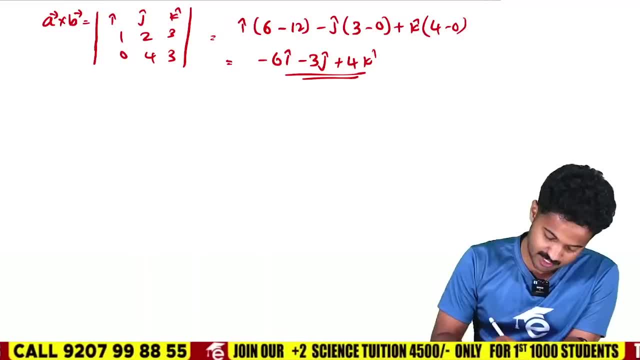 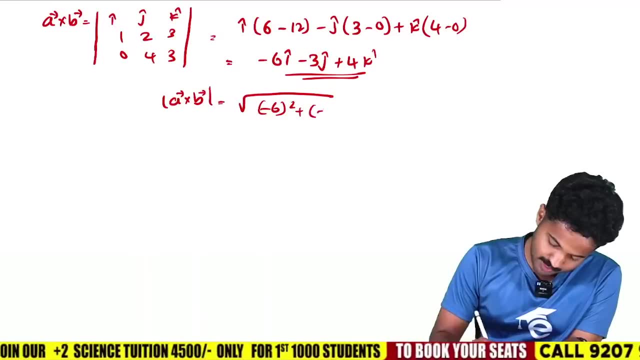 4 minus 0, 4.. So 4, K. OK, This is the answer And the magnitude of this, the magnitude of A cross B. we get the root of minus 6 square plus minus 3 square plus 4 square. 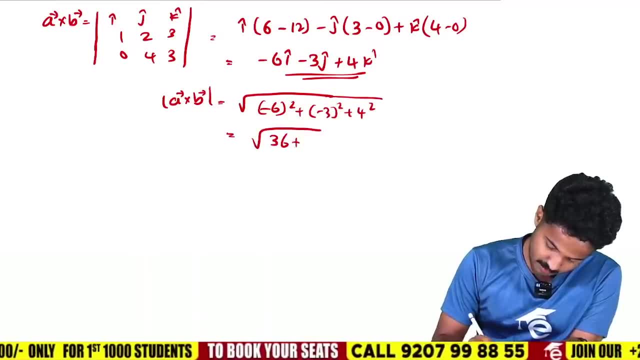 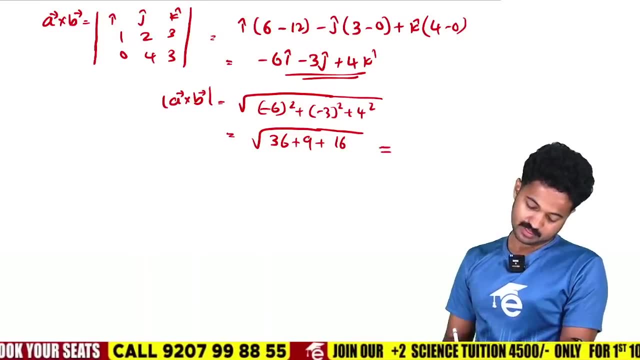 That is, the answer is 36 plus minus 3 is 9, plus 4 is 16.. So you get the answer 36 plus 9.. 45 plus 10,, 55 plus 6 is 61.. 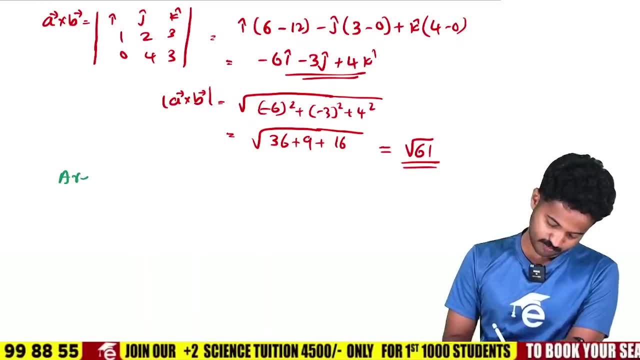 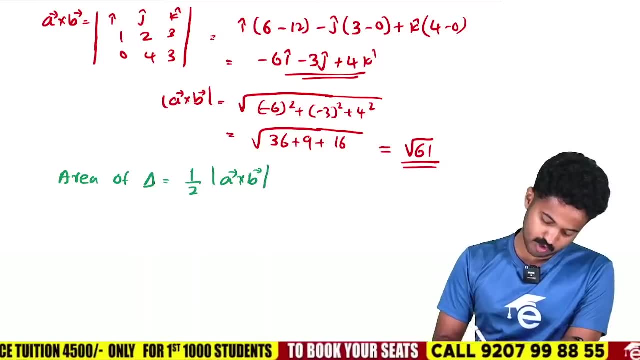 So the root is 61. That is the area. If we find the area of triangle, the equation for finding the triangle area is half into magnitude of A cross B. A and B are adjacent sides, So how much is half into magnitude of A cross B? 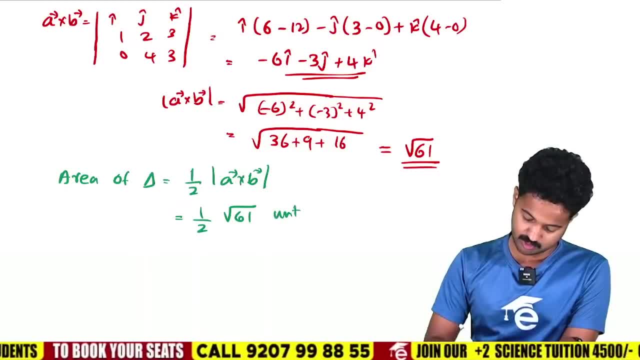 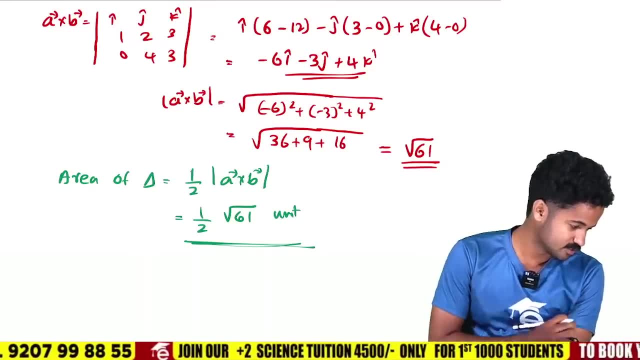 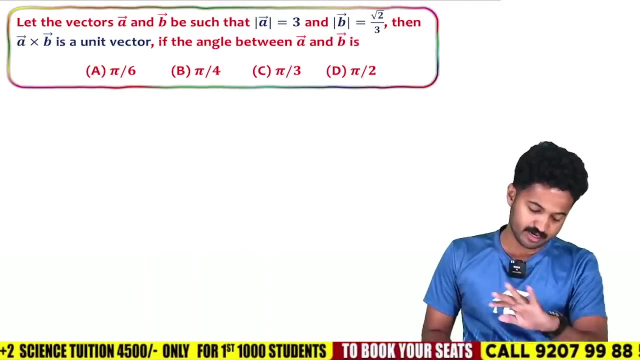 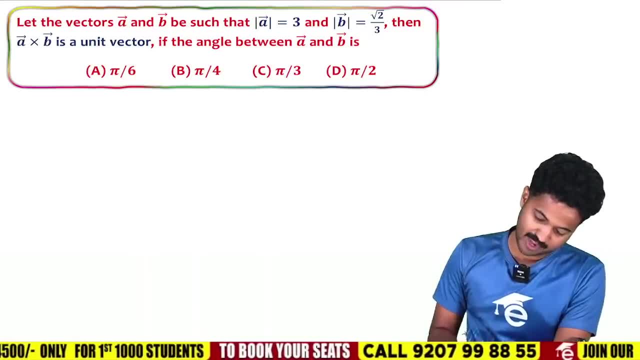 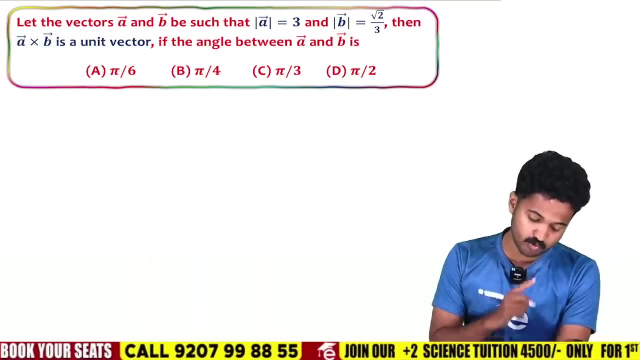 The vector is over. Next is 3D. AB is such that magnitude A3.. Magnitude B root 2 by 3. Then A cross B is a unit vector. The angle between A and B. If A cross B is a unit vector, what does it mean? 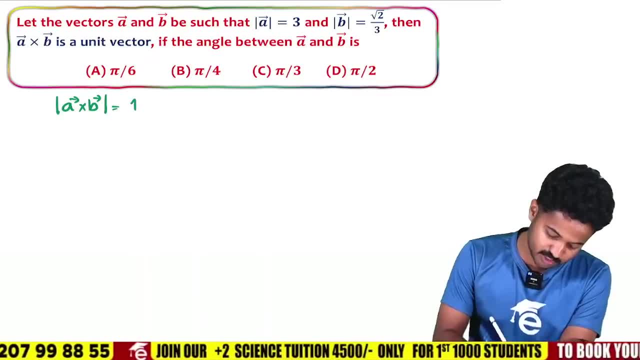 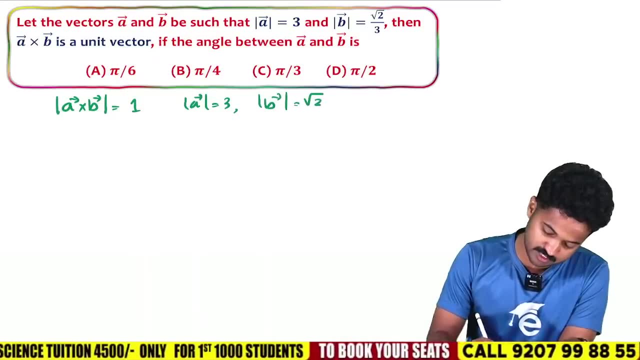 If A cross B is a unit vector, the magnitude of A cross B is 1. Easy right And magnitude A equals 3.. Magnitude B equals root 2 by 3. The angle you asked is the value. 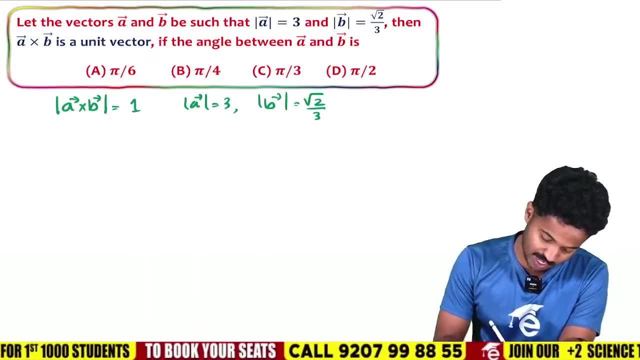 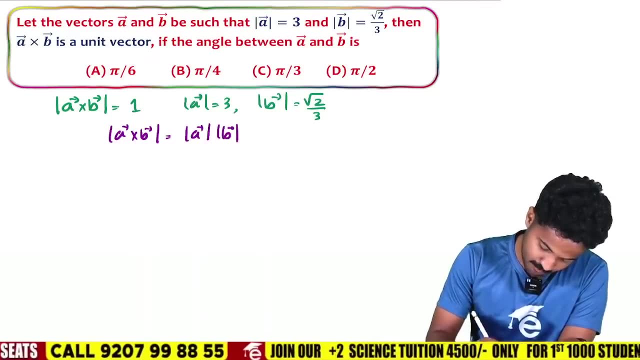 So let the magnitude be 3.. If we give a cross b, we can find the angle like this. There is nothing like that. I told you that a cross b is magnitude a, magnitude b as well as sine theta and magnitude n cap. 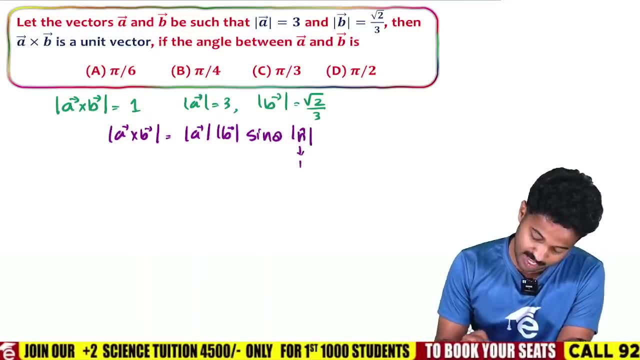 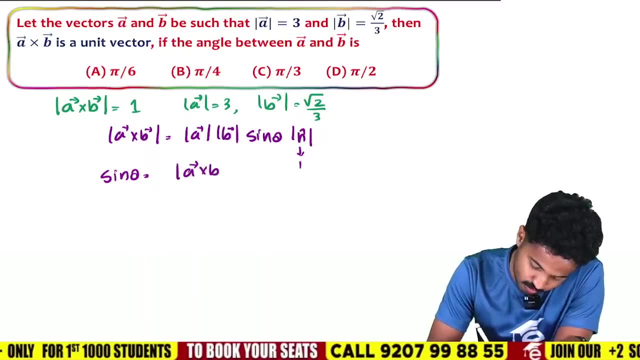 This is one. So what do we do? We do the same thing. So if we find the angle sine theta, what do we do? Sine theta equal? to just bring it here, That is magnitude a cross b, divided by magnitude a into magnitude b. 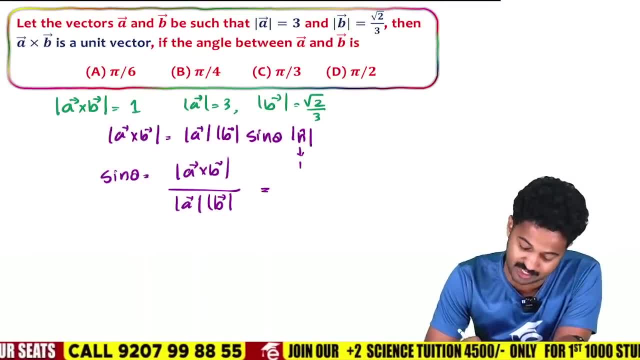 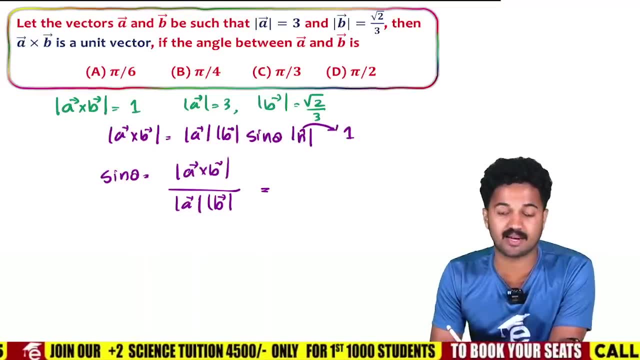 If we find the angle, usually we are in the term of cos theta, But here what we are going to do is because it is in the term of sine theta, sorry, because it is in the term of cross product sine theta. a, cross b. magnitude is 1 divided by magnitude a is 3,. 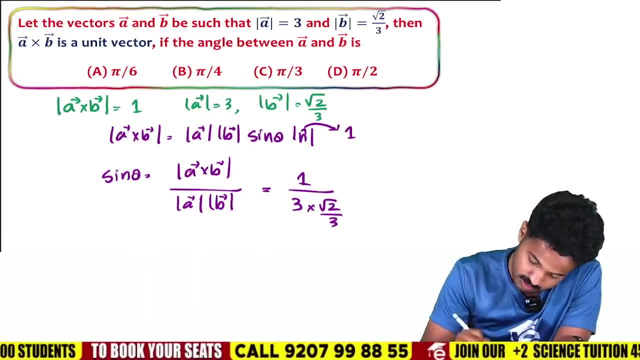 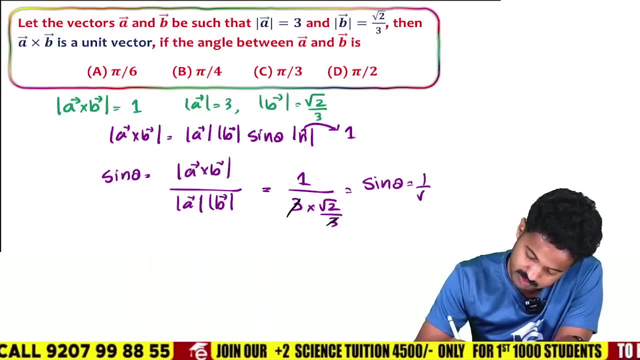 magnitude b is root 2 by 3.. Easy See this 3 and this 3 can be cancelled. So sine theta is 1 by root, 2.. Sine theta equal to 1 by root 2. Sine theta is 1 by root, 2.. 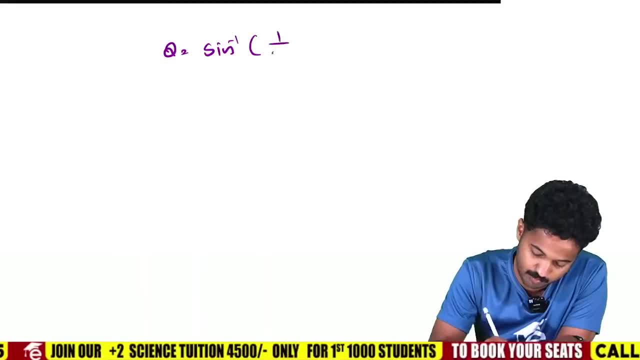 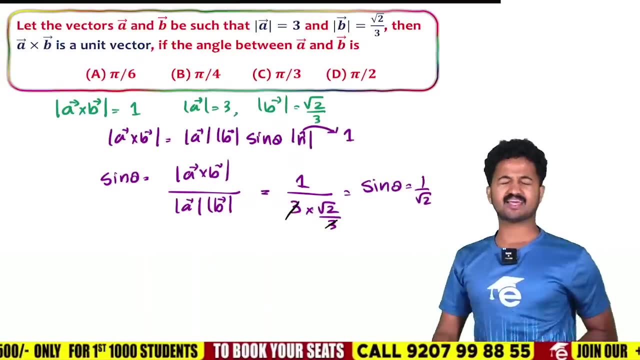 What is theta? Theta equal to sine inverse 1 by root 2.. Sine 1 by root 2 is here. Yes, that is pi by 4.. So theta is pi by 4.. Easy. So, no matter how you come, you should do the questions from vector well. 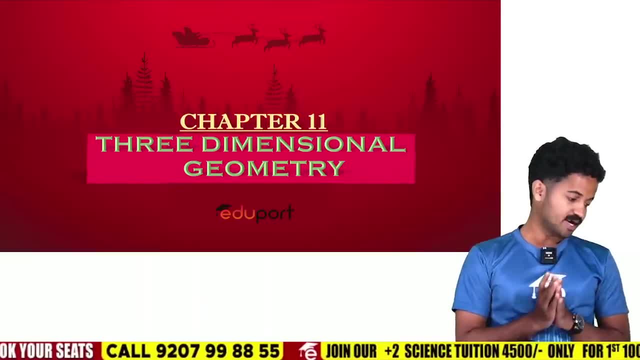 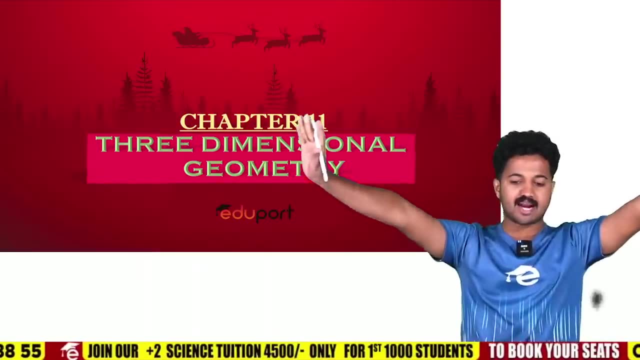 Easy, No problem. So far it is easy, So we think that it is ready. It is ok, right, Set Ok After studying vector. if it is ok, like this, I can start 3D, no problem. 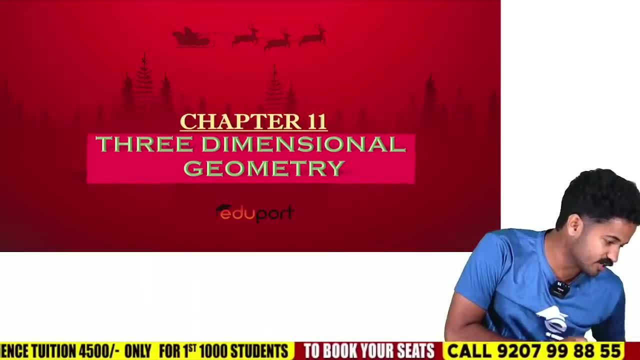 If it is ok like this, I can drink a little water. If it is ok like this, I can start 3D. no problem, If you are ok with this, you can do it in 3D for 30 minutes. 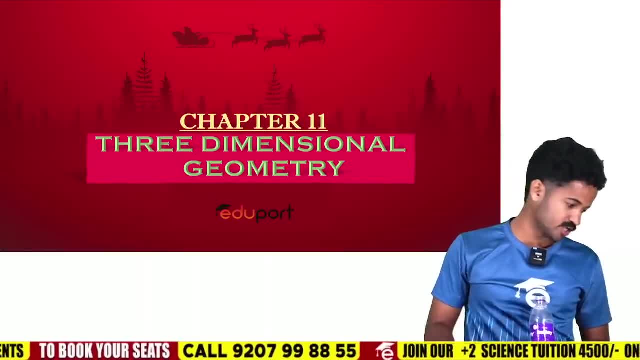 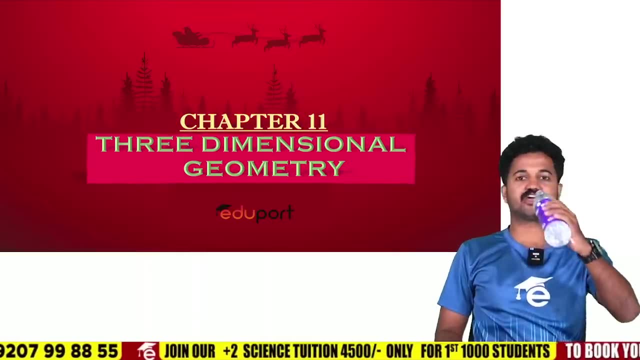 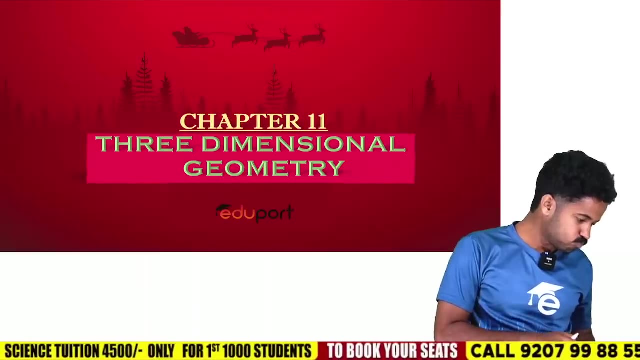 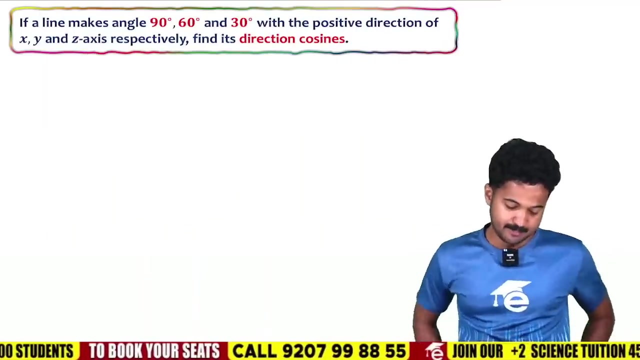 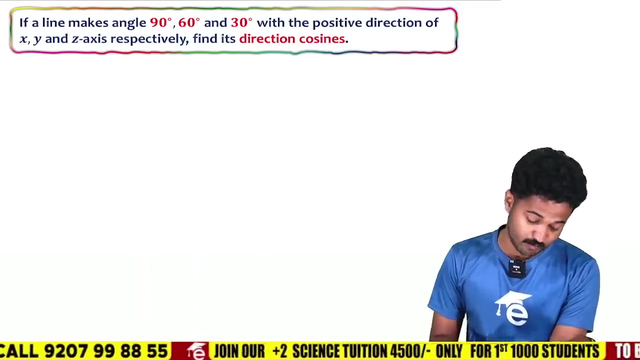 I will finish it in 30 minutes. If you are ok with this, you can get a green ticket. That's how we can start. Let me drink some water. Ok, sir. 3D, A line makes angle 90,, 60,, 30 degree with positive direction of x and y, z axis, then direction cosine. 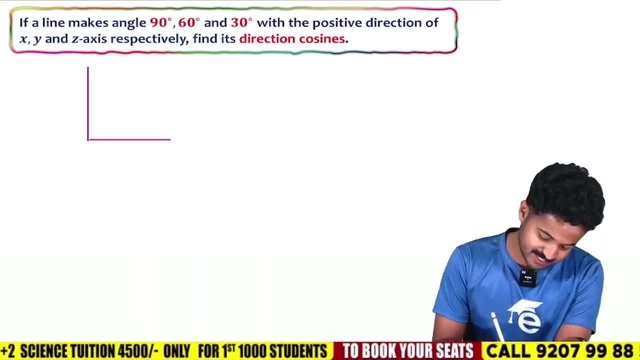 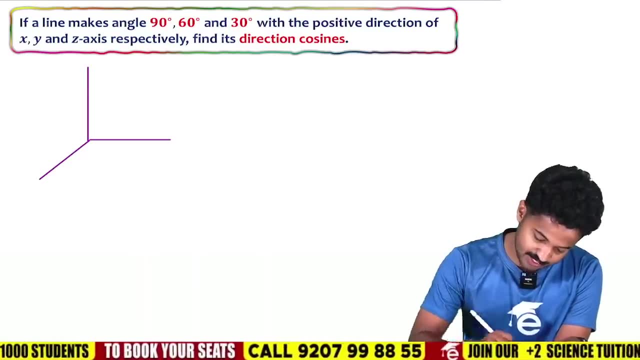 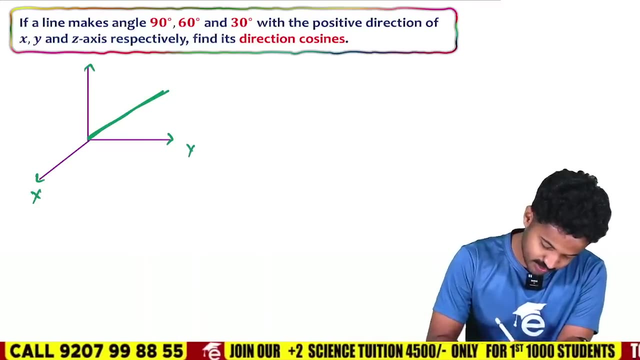 We have x, y and z axis in our hands. It is a three dimensional space. We learn this in geometry. Take this as a line. This is the line in our hand. This is an x, y and z axis. This is x, this is y and this is z. 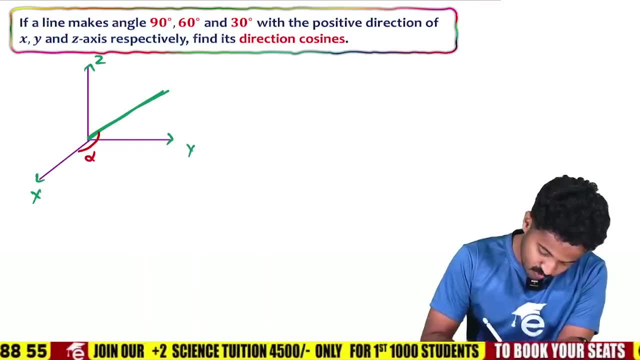 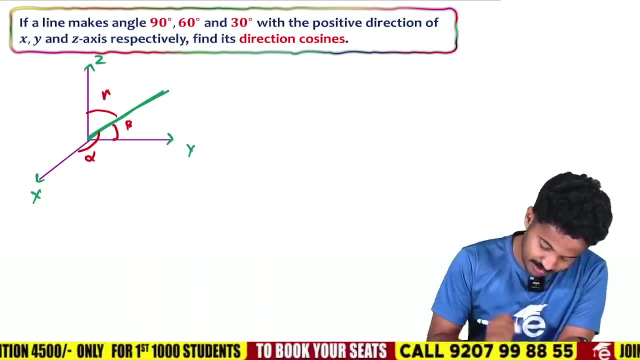 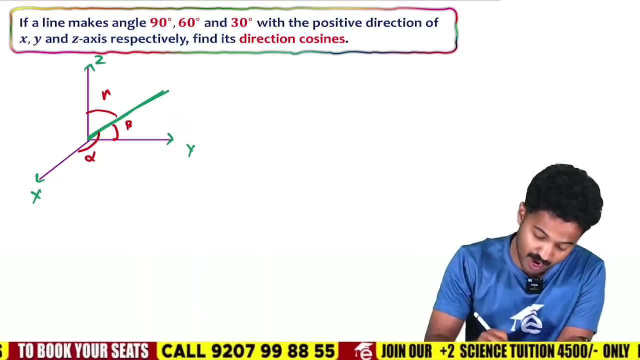 Let's see: Angle of x axis is alpha, angle of y axis is beta and angle of z axis is gamma. If a line is positive x, positive y, positive z, then it is alpha, beta, gamma. Let's see: 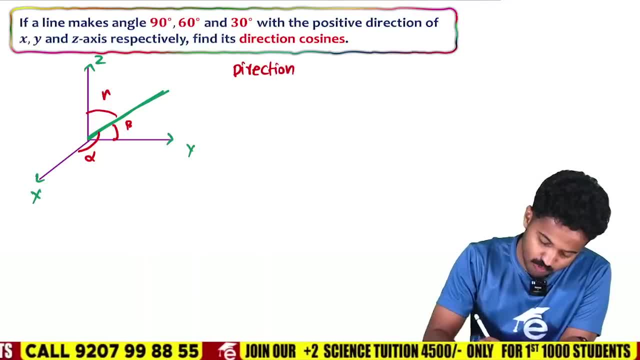 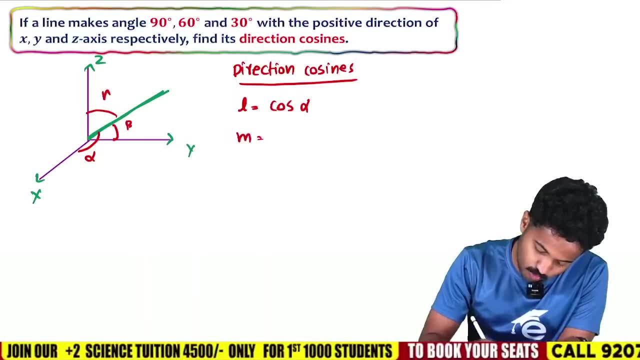 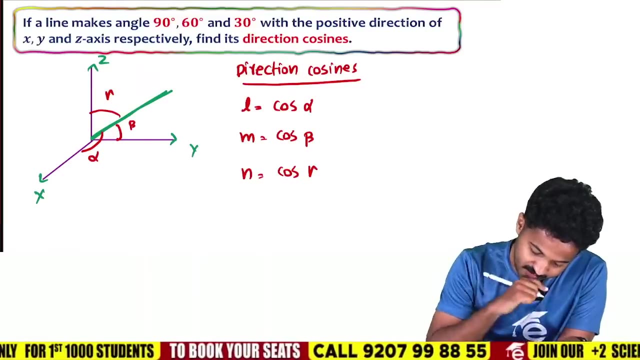 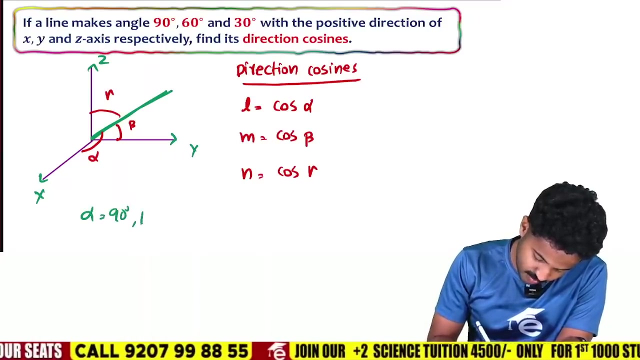 Its direction cosines are L equal to cos alpha, M equal to cos beta direction cosines are N equal to cos gamma. So that's how it is Easy right. Look at all the angles given here. Alpha is 90,, beta is 60, and zx is 30. 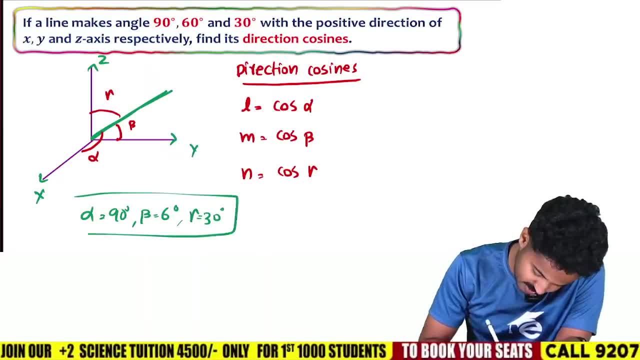 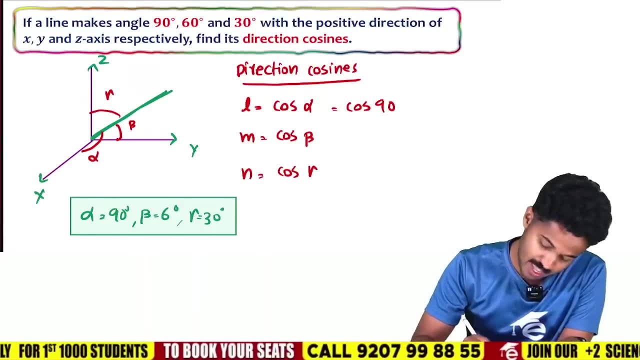 Gamma is 30.. This is what we got in the question. If so, let's find the direction. cosines, It's very easy: Cos 90,, cos 60, and cos 30. So look at that, Cos 90.. 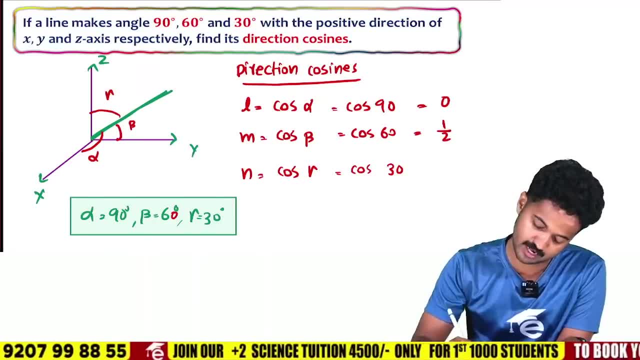 Cos 90,, that is 0,. sir Cos 60,, that is 1 by 2,. sir Cos 30,, that is root 3 by 2, sir Easy: 0, 1 by 2, root 3 by 2.. 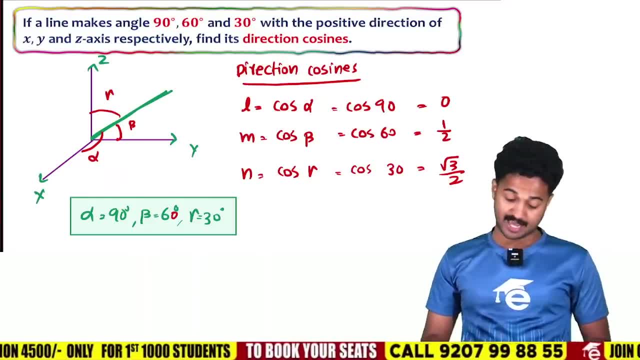 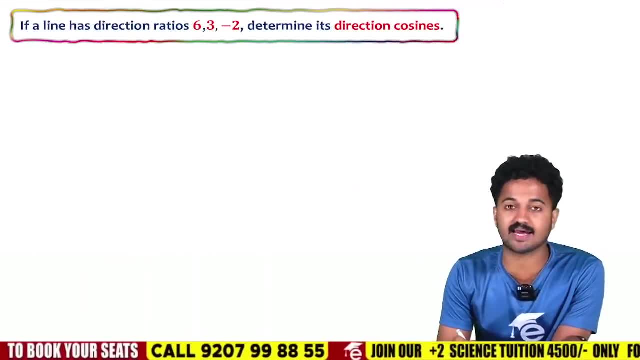 Yes, very good. 0,, 1 by 2, root 3 by 2.. This is how you find the direction cosines. It's simple, No problem. One more thing. The next question: If you give direction ratios, how will you find the direction cosines? 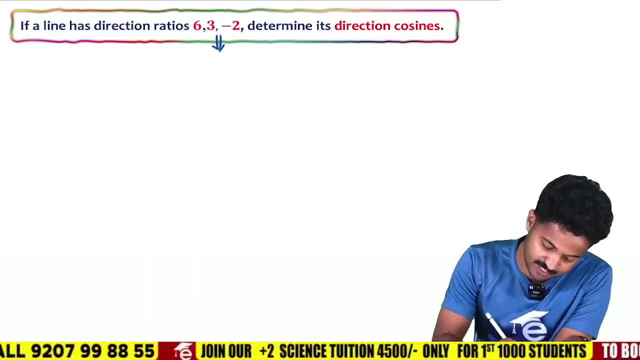 We already said this: If you give direction ratios, what will be the vector? If it's a vector called a, it's 6i plus 3i, 6i plus 3i, 3j minus 2k. 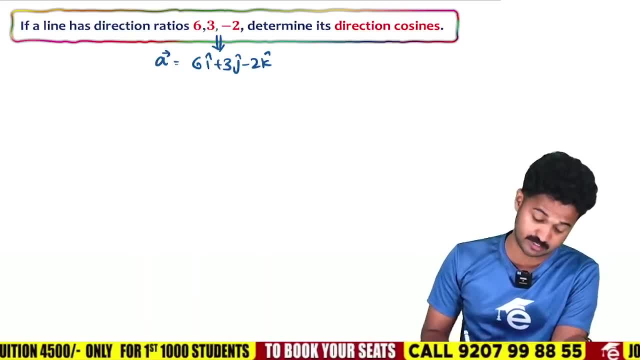 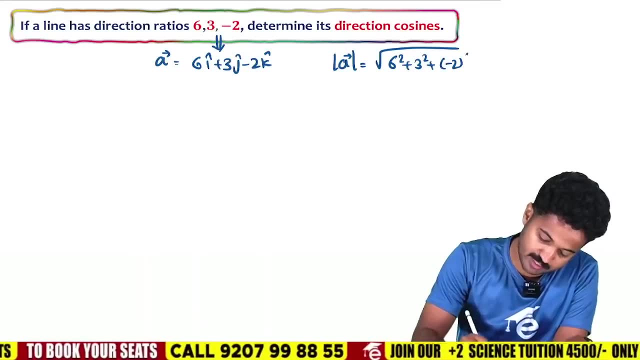 The same thing we said earlier. If you give direction ratios, how will you find the direction cosines? First, what is the magnitude of this? The magnitude is root of 6 square plus 3 square minus 2 square. So the answer will be 36 plus 9 plus 4.. 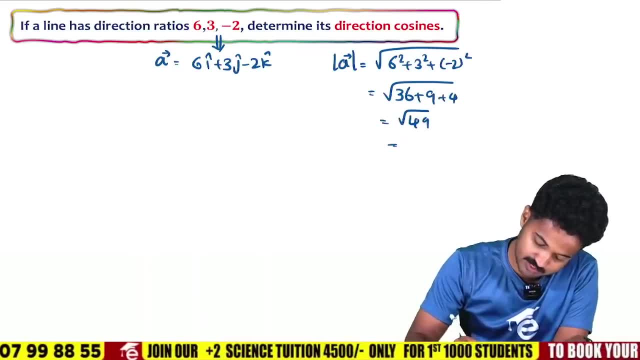 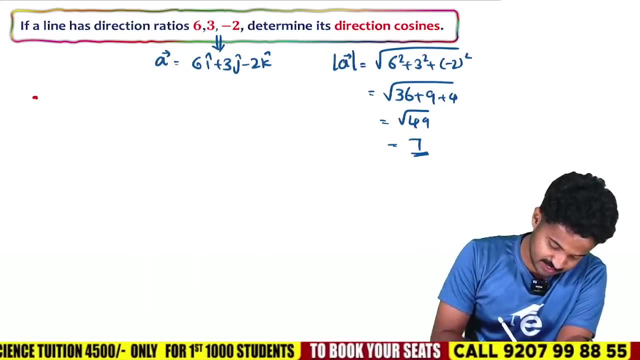 That is root 49.. If you say root 49, it's 7.. Okay, Ready, What is this? The magnitude of this? Sorry, Yes, That is the direction, cosines, It's easy. L is needed. 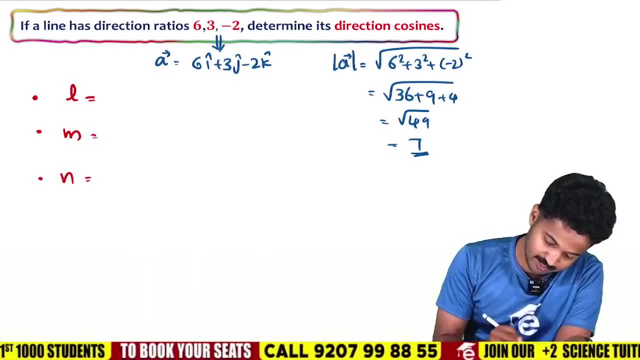 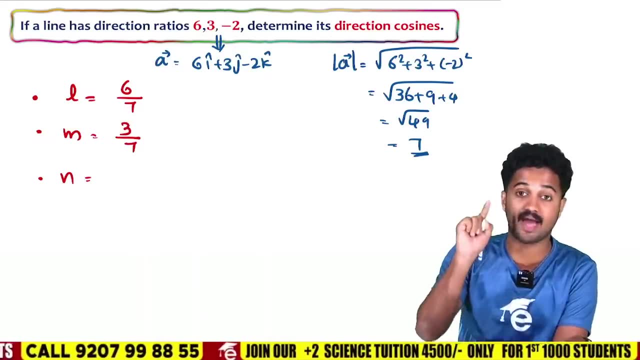 And M is needed, And M is needed, And N is needed. If we say L, it's very simple: 6 by 7.. If we say M, it's 3 by 7.. Direction ratio by magnitude of our vector. 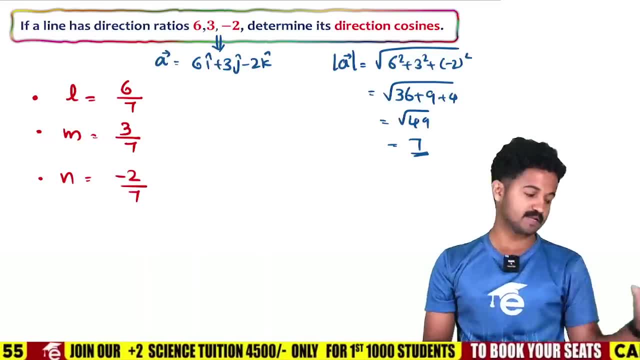 If we say N, it's minus 2 by 7.. I'm speeding all this. It's the problem we did earlier. It's the same thing we did in the previous chapter. It's the same thing we did in the previous chapter. 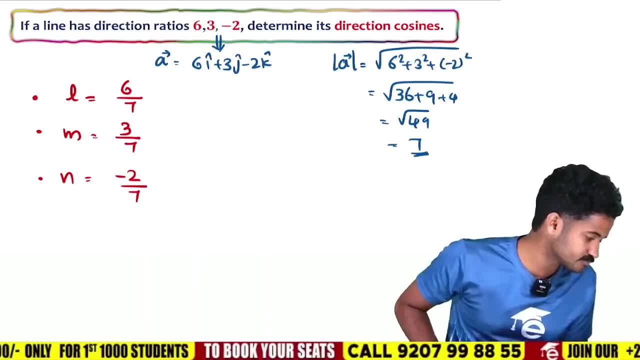 It's the same thing we did in the previous chapter, So there's no problem. Okay, 6 by 7,, 3 by 7, minus 2 by 7.. Do you know one thing I need to know? Do you know one thing I need to know? 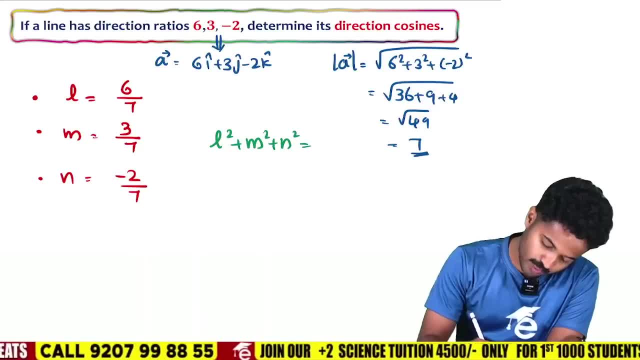 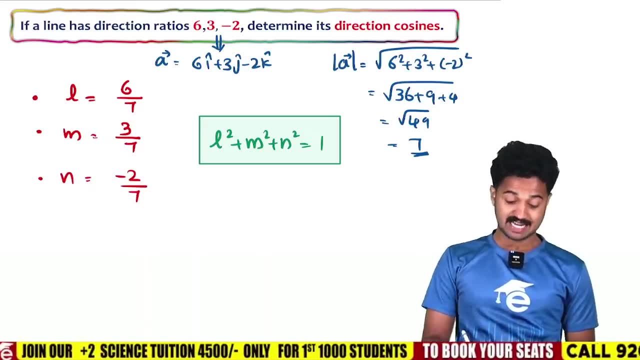 L square plus M square plus N N square is always 1.. Do you know? L square plus M square plus N square is always 1. Always. do you know What will you get if you take the sum of direction cosines? 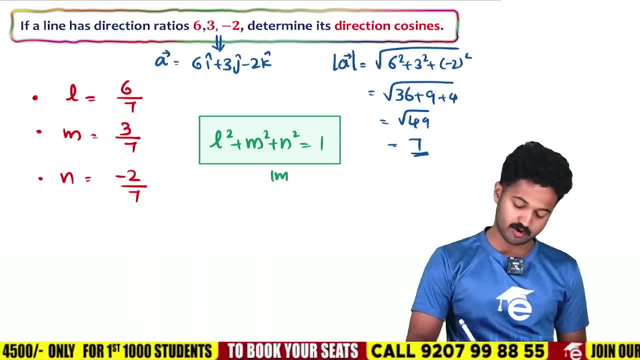 It will be 1.. What will you get if you take the sum of squares? It will be 1.. It will be 1.. There's a chance to ask one word or an exam. L square plus M square plus N square is equal to 1.. 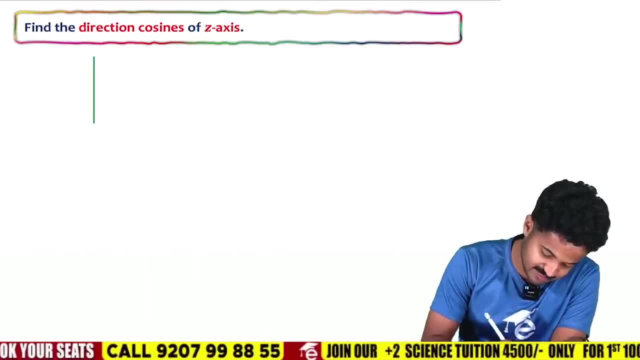 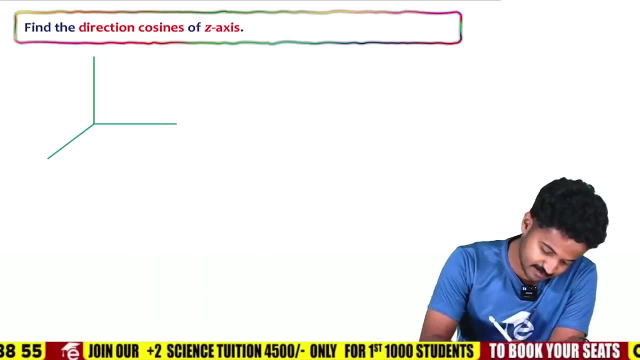 Next, look Direction cosines of Z axis. How do you do that, sir? It's easy. Look Direction cosines of Z axis. Direction cosines of Z axis, Our Z axis. This is Z axis, This is X. 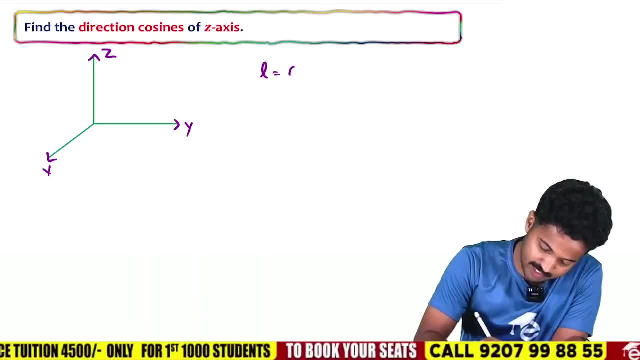 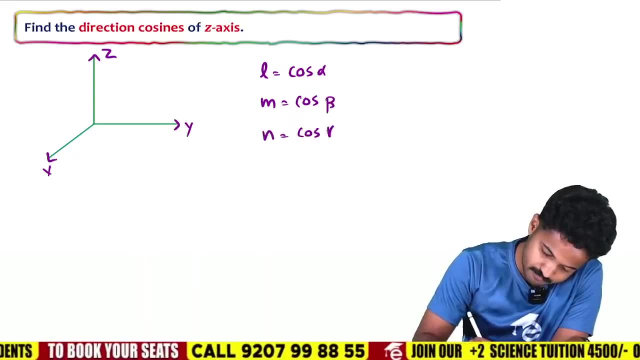 This is Y First direction, cosines. is this equation: L equal to cos alpha, M equal to cos beta, N equal to cos gamma? Think of one thing: Z axis is what I said, So Z axis is this Same. 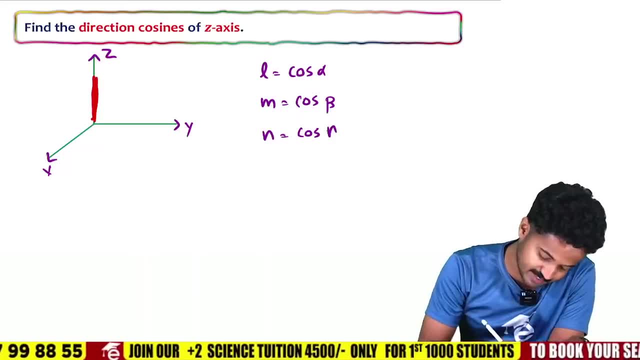 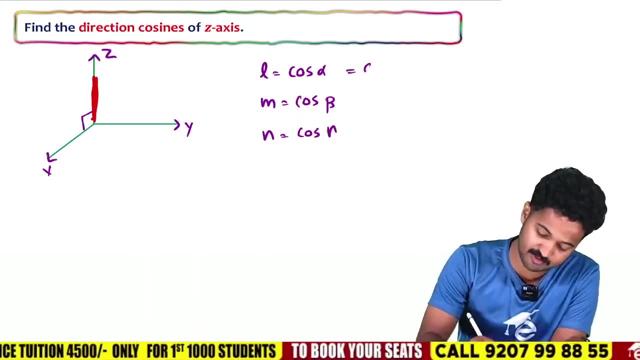 So this axis, The angle that Z axis makes with X, The angle that our line makes with X, is not alpha. So the angle that Z axis makes with X is 90.. So what is the answer to this? If it is alpha, it is 90.. 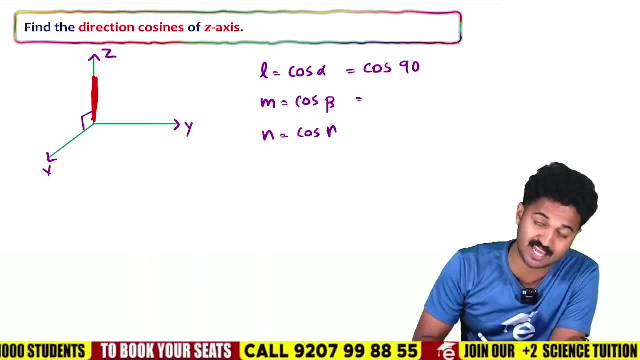 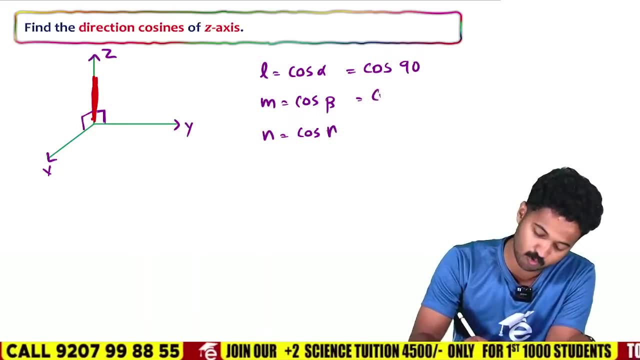 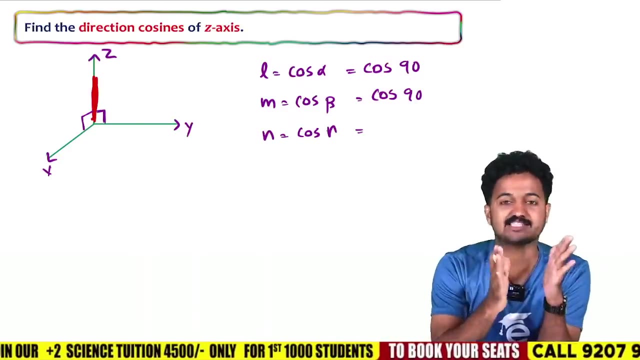 Cos 90.. If it is beta, then the angle made by Z axis. Is it the angle where Z is made by Z axis? If it is Z axis 90, then the line is made by Z axis. This is also 0. 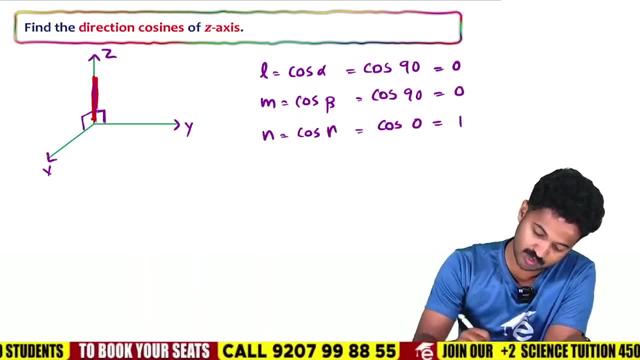 So cos 90 is 0.. cos 90 is 0.. cos 0 is 1.. So these are the direction ratios: 0, This is Z axis, And this is Z axis. If it is Z axis, it is also 0.. 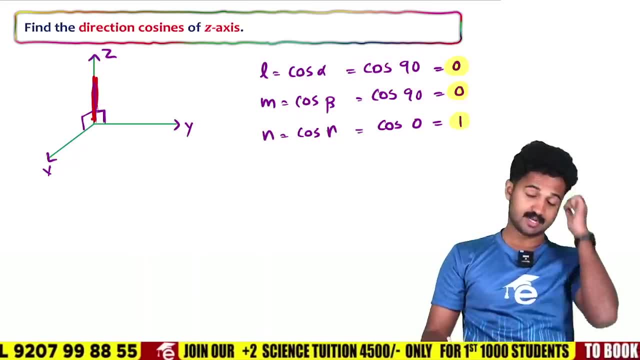 Cos 90 is 0.. Cos 90 is 0.. Cos 0 is 1.. So these are the direction ratios: 0, 1,, 0,, 0,, 1.. That's what direction ratios are. 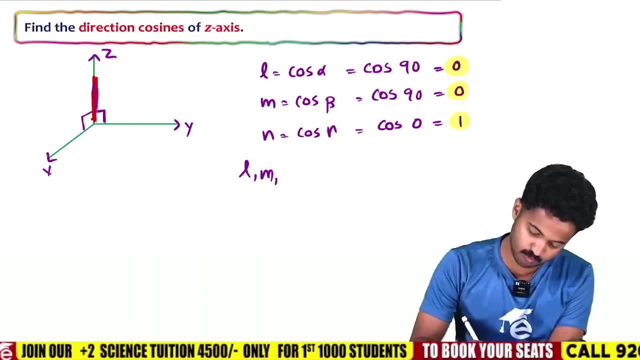 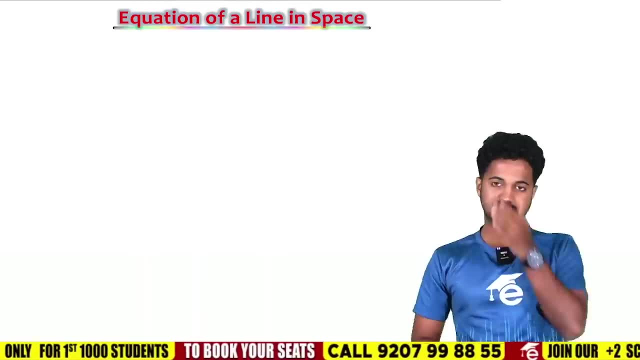 Okay, simple. So what did we get? L M N equal to 0, 0,, 1.. Easy, So, just like that, you can write any axis as well. Easy, Simple. Now, the most important thing in this chapter is: 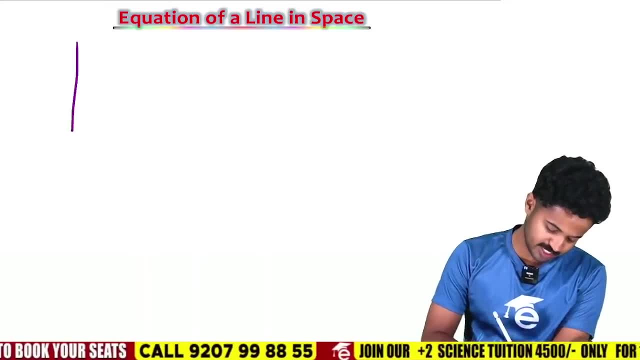 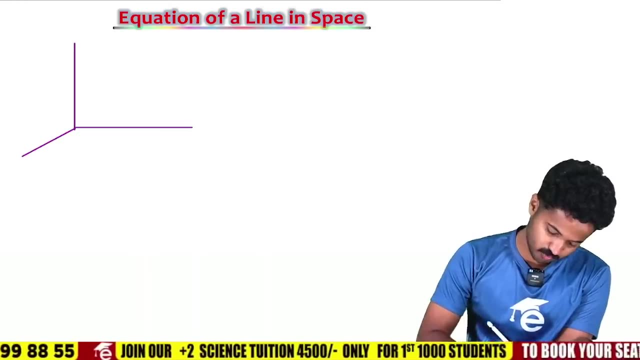 the exam. You can ask anything. We have a three-dimensional space. Look, We have a three-dimensional space. I drew a line here. A line, Okay, I drew a line. I marked a point in this line. I marked a point in this line. 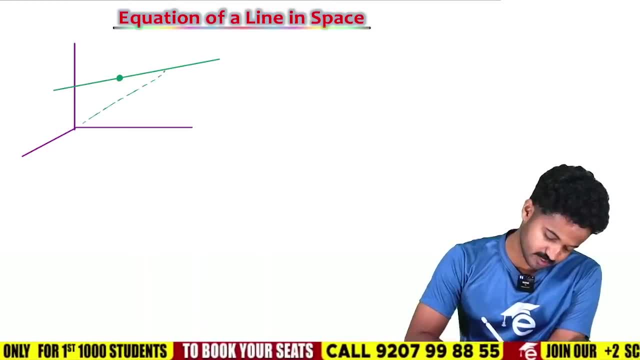 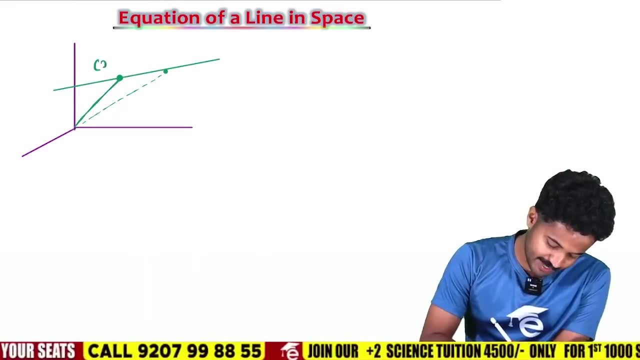 I am drawing a position vector here as well. This is a position vector Generally, it is a position vector. This position vector is drawn here as well. I thought this point is: x1, y1, z1.. x1, y1, z1.. 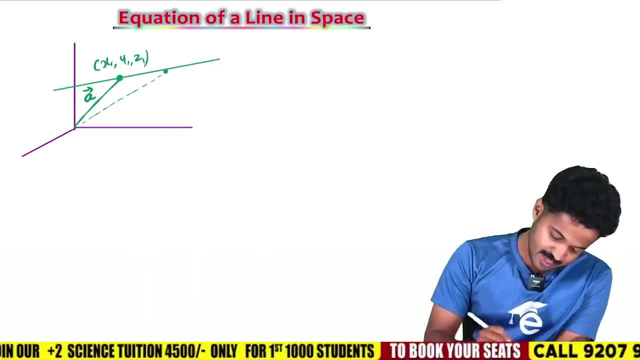 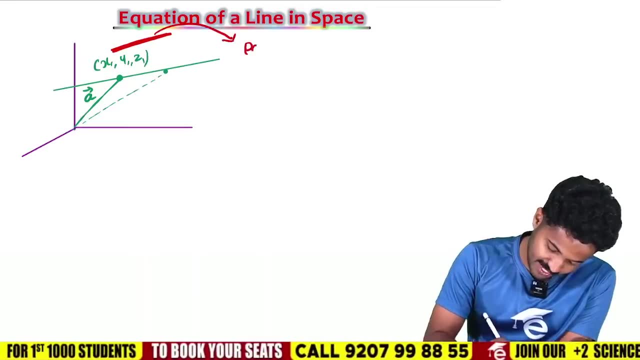 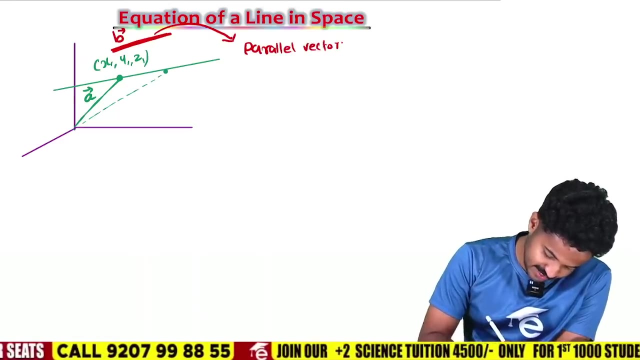 I gave this position vector as a. Anyway, this line has another vector parallel to it, Parallel to another vector, Parallel vector, Parallel vector. This vector is denoted as b, Parallel vector b. Okay, That is also fine. This is your r vector. 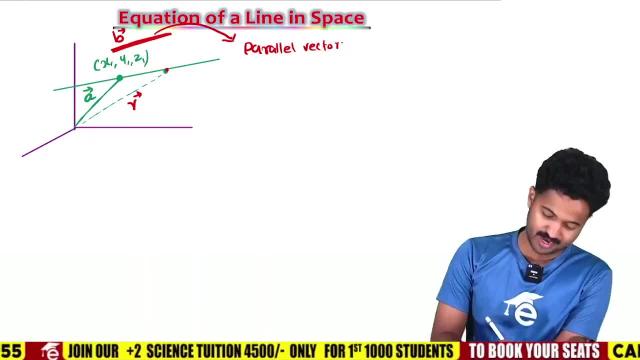 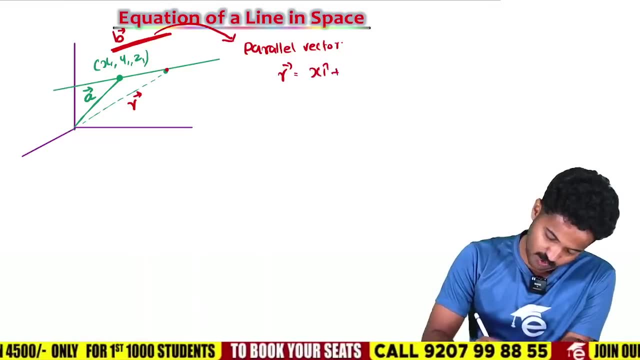 r. Position vector right r. This is the general point. We wrote x y z. Okay, There is no problem. Now look What is r x y z. That is the point I am marking here is x y z. 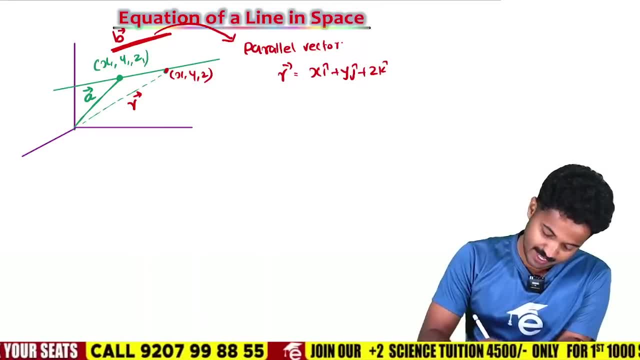 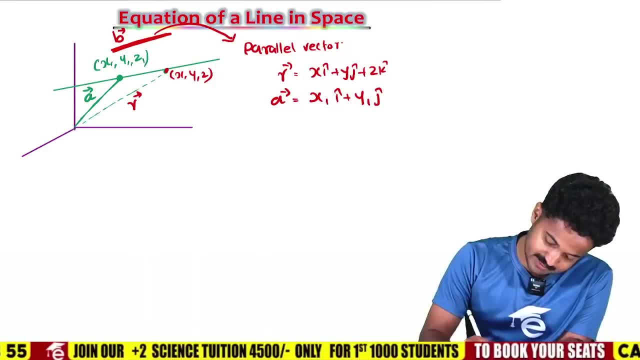 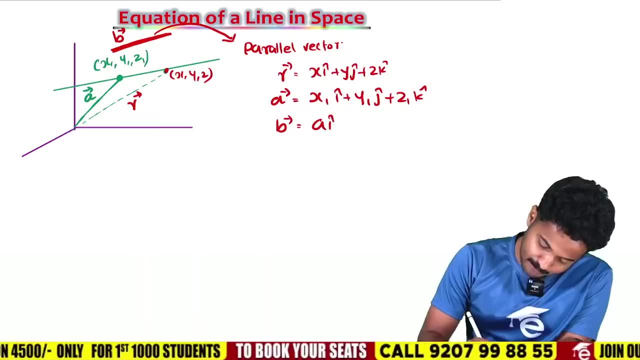 x1, i+, y1, j+, z1, k. Okay, If b is a parallel vector, that is, a, i+, b, j+, c, k. Okay, If you know all these things, if you know all these things. 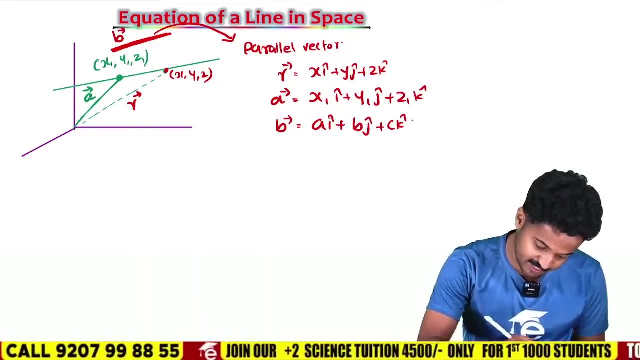 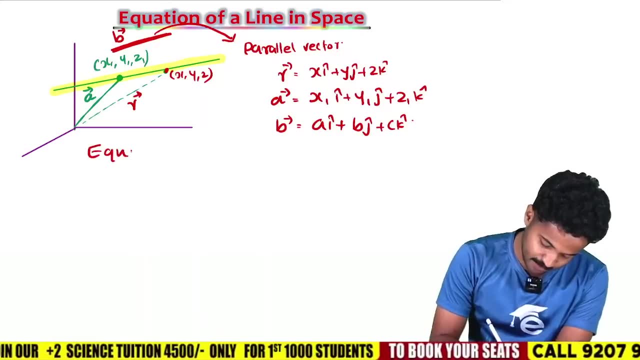 that line equation is necessary. This is the line we consider. Okay, This is the line in our hand, That line equation. Equation of line. Write it in two ways. Equation of line. Write it in two ways. One is vector equation. 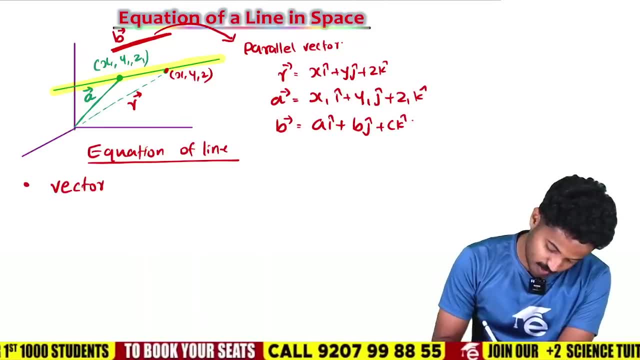 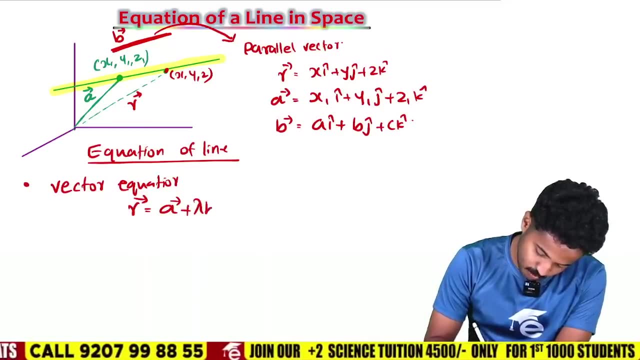 Second is Cartesian equation, Vector equation. Sir, how to write vector equation? It is easy, It is simple: r equal to a plus lambda b. Note it: Vector equation is: r equal to a plus lambda b. Easy, Simple, No problem. 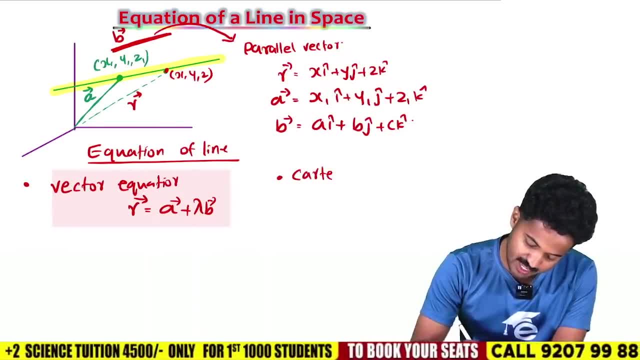 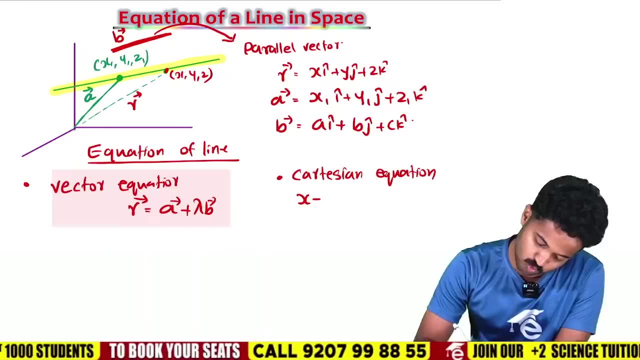 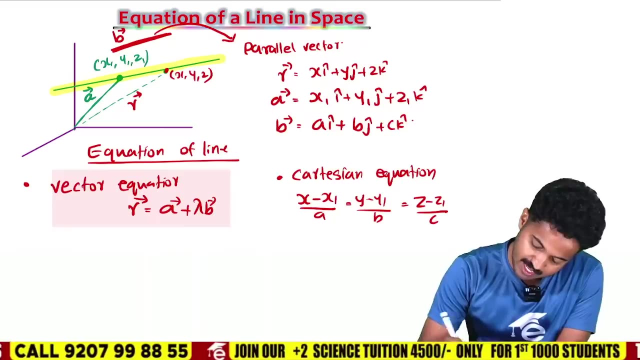 Similarly, Cartesian equation is also simple. We have to learn both. Important is x minus x1 by a, equal to y minus y1 by b, equal to z minus z1 by c. What is x1, y1, z1? You know it clearly. 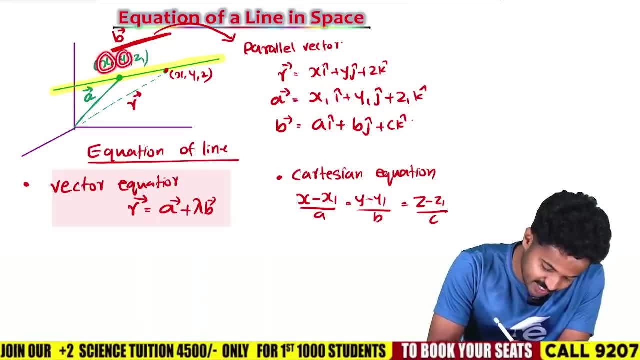 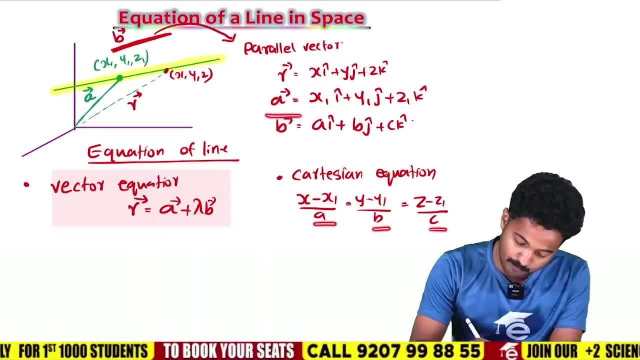 x1, y1, z1.. The direction ratios of the position vectors are x1, y1, z1.. a and b and c are parallel vectors. The scalar components or direction ratios of them. The parallel vectors: The scalar components or direction ratios of them. 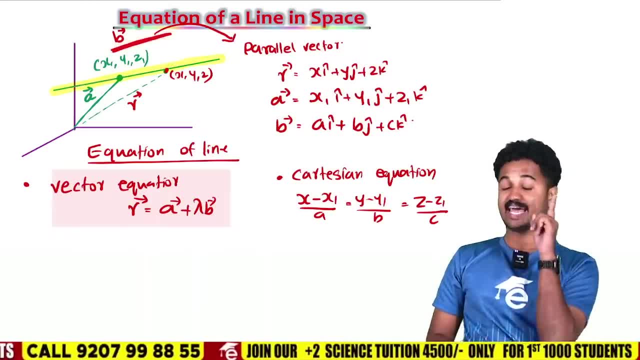 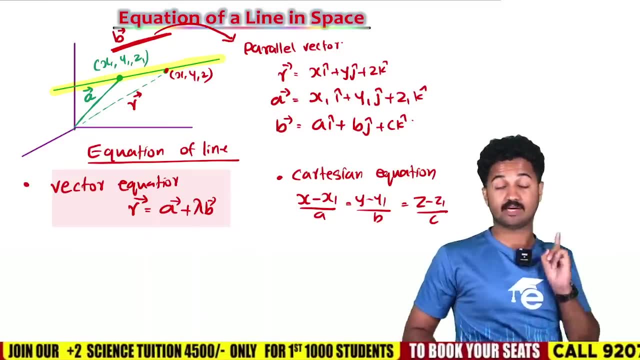 The parallel vectors. The direction ratios of the given line parallel vectors are: a, b, c. Okay Ready, x minus x1 by a, y minus y1 by b, equal to z minus z1 by c. We have to learn both. 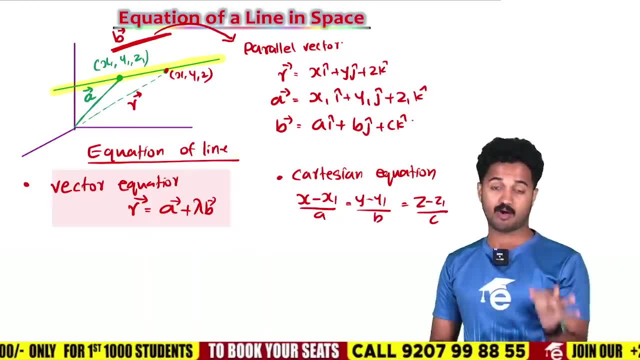 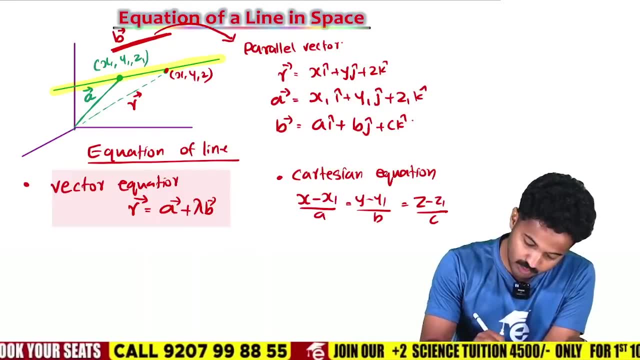 r equal to a plus lambda b, x minus x1 by a, y minus y1 by b, z minus z1 by c. If you want, you can give it as constant. What can you give as constant? Give a lambda here. 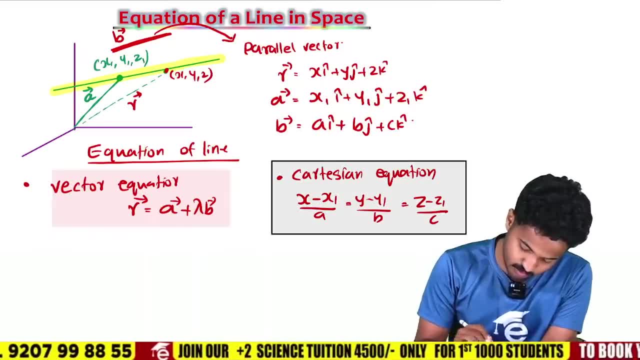 No problem. So these two equations are very important. Why don't you learn it? by understanding it, You can learn it Ready. If so, we are going to do the problems of this. We are going to do the problems of this. 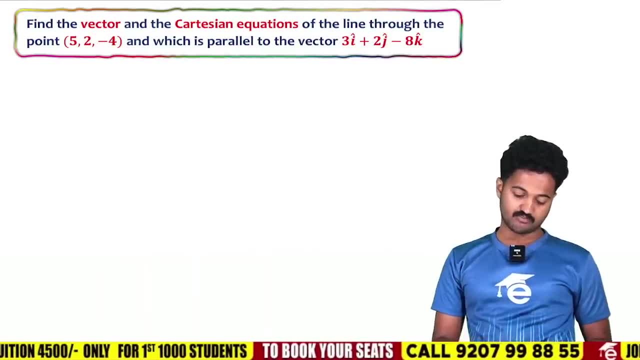 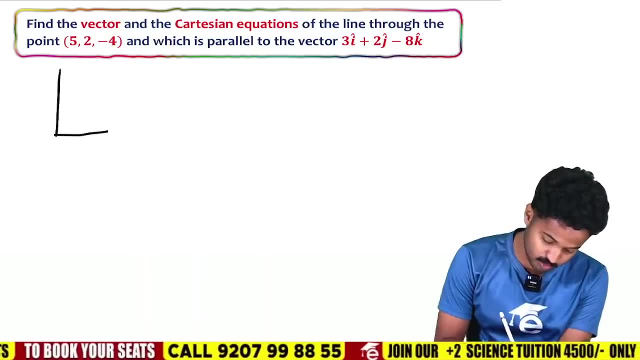 Okay, Look, Find the vector and Cartesian equation of a line through the point 5, 2, minus 4 and which is parallel to the vector 3i plus 2j minus 8k. Look what I have said: Our three-dimensional space is exactly here. 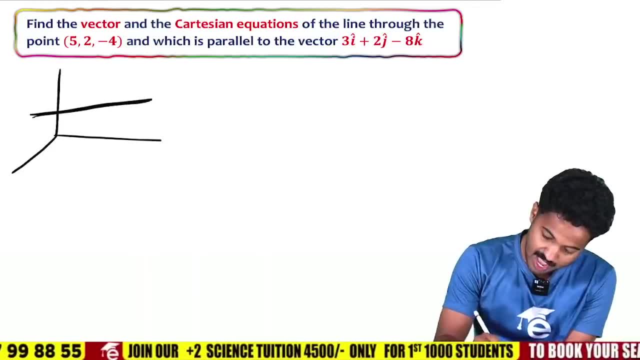 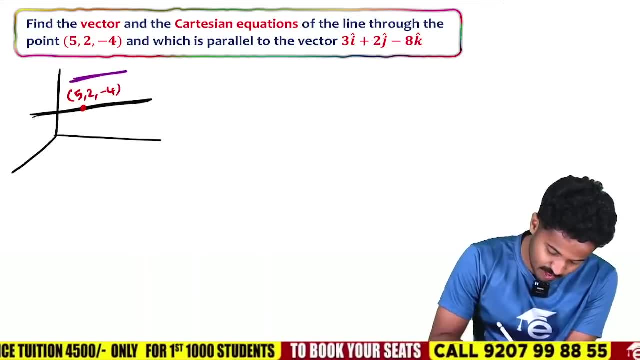 You have a line, A line. This is your line. That line passes a point 5, 2, minus 4.. And this line is a parallel vector, Parallel vector b. b is a parallel vector. Parallel vector means 3i plus 2j minus 8k. 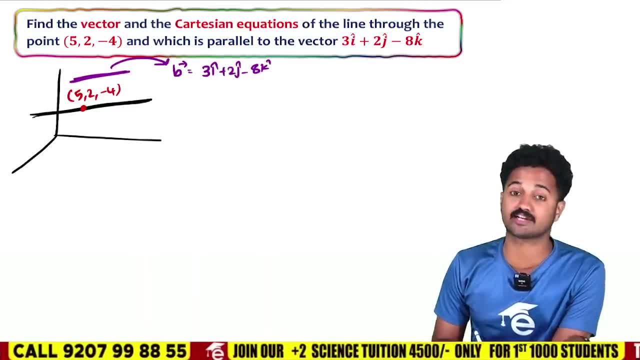 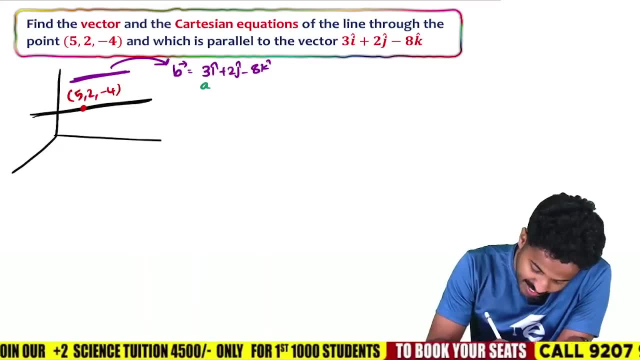 Easy. If so, you have to write the Cartesian equation and vector equation of this. So if you want Cartesian equation and vector equation, you will get b- as simple as this. We have written b as ai plus bj plus ck, So we have a and b and c. 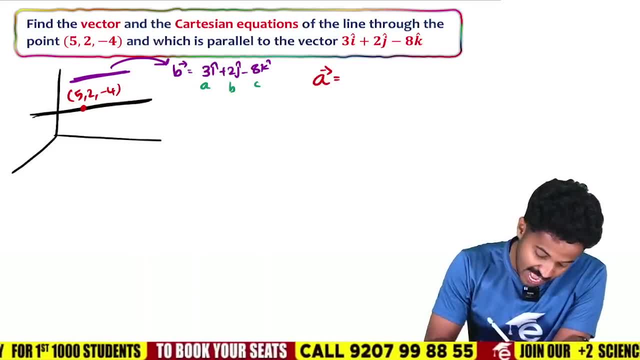 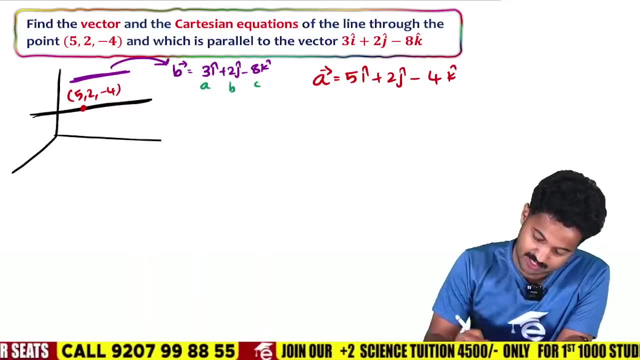 Now, what is a vector Here? a vector means if the point of that line is 5,, 2, minus 4,, then it is 5i plus 2j, 2j minus 4k. is your a vector? 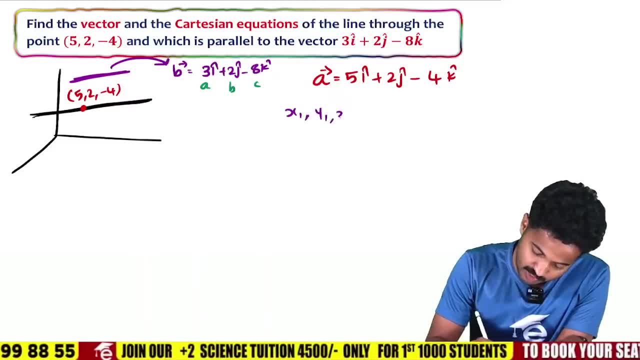 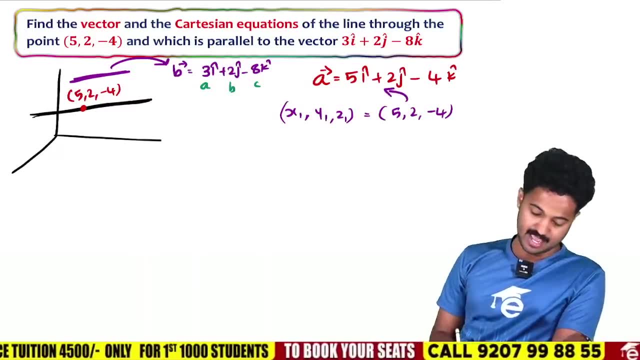 Which means your x1, y1, z1 is the point. That point is 5, 2, minus 4.. Using this, we can write a vector. Easy, isn't it? So b is in your hand. 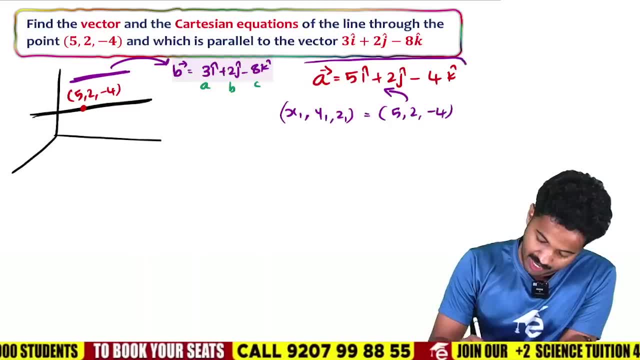 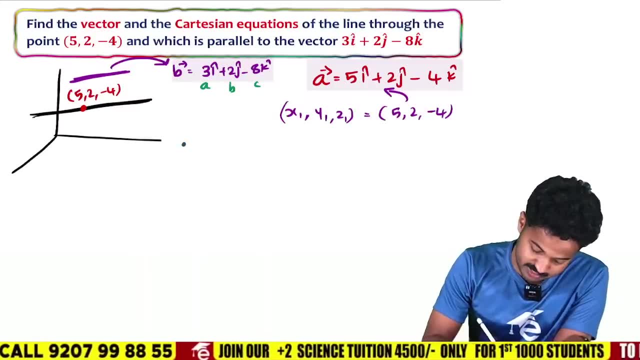 b is in your hand, Okay, b is not a problem. Similarly, a is in your hand, Okay, No problem. So x1, y1, z1 and a, b, c are there? What is vector equation? 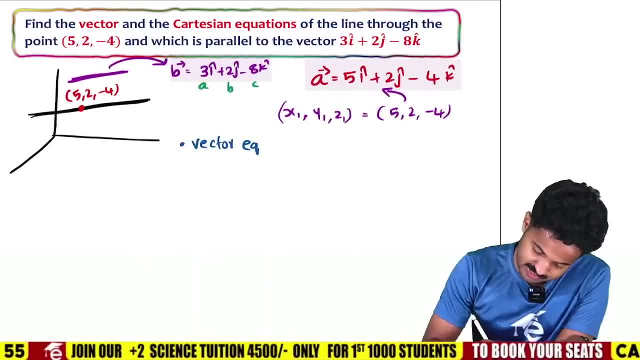 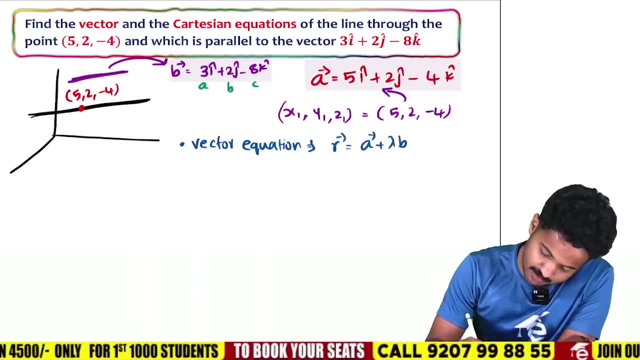 Vector equation is very simple. Now I will give you a vector equation very easily. How was the vector equation r equal to a plus lambda b? You just have to give r. Look r equal to What is the vector that says a? 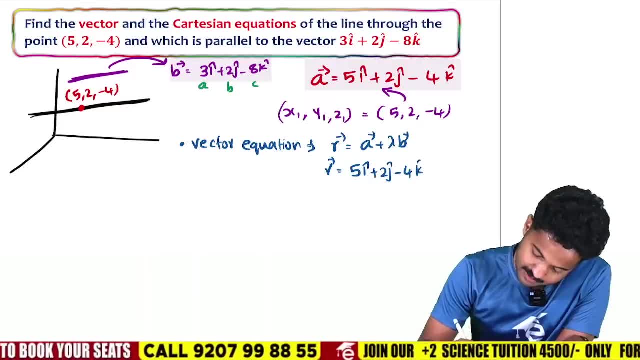 5i plus 2j minus 4k plus lambda. What is the vector that says b? 3i plus 2j minus 8k? 3i plus 2j minus 8k. Okay, Got it. 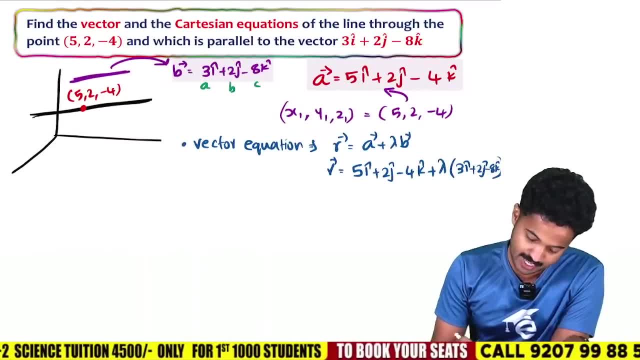 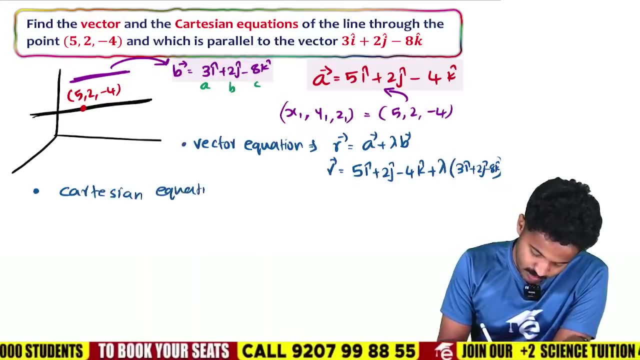 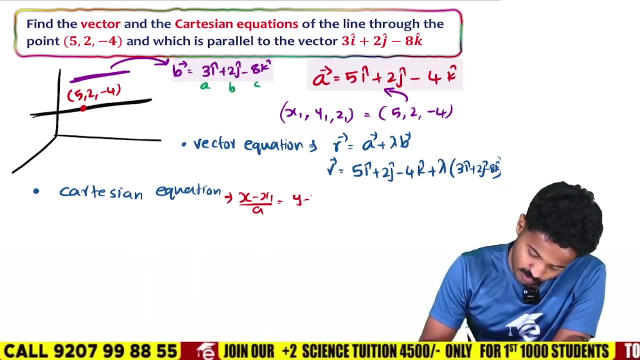 Easy sir, No problem, right? If that is the case, we got that too. Next, what do you want? Cartesian equation: How do you write the Cartesian equation? Cartesian equation- Easy sir. Cartesian equation is x minus x1 by a, y minus y1 by b, equal to z minus z1 by c. 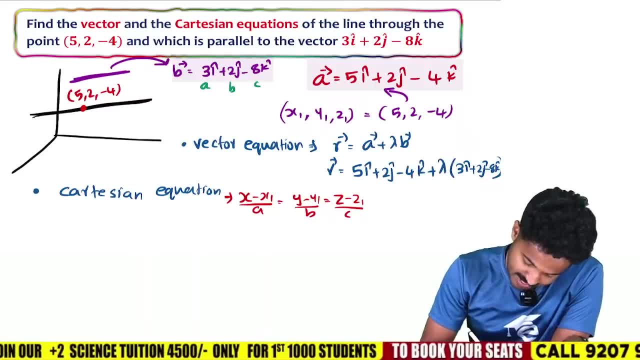 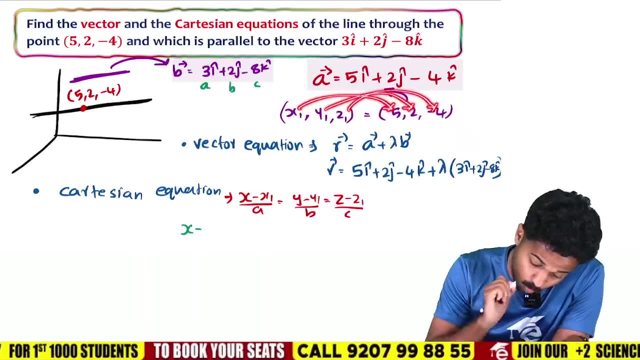 If that is the case, look at the Cartesian equation. How do you write it? If it is x minus x1,, this is x1,, this is y1, and this is z1.. That is the points. This is x1, y1, and z1. 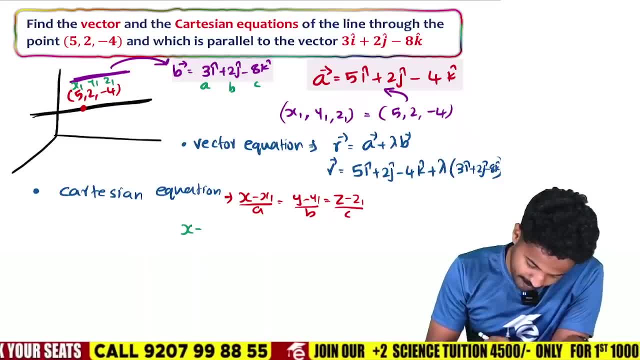 You have to understand this clearly, Okay, Okay, This is x1, y1, z1.. So x minus. look at this. You have to give x minus x minus 5 divided by a. Look at this: This is 3.. 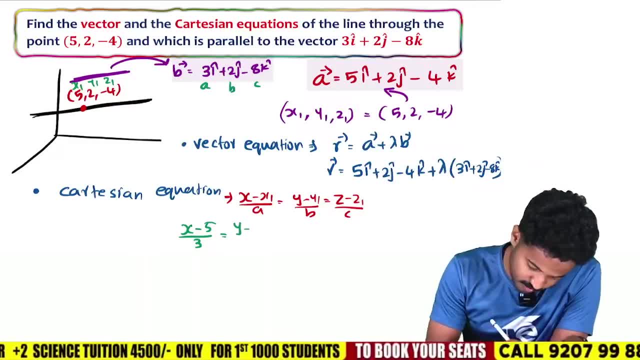 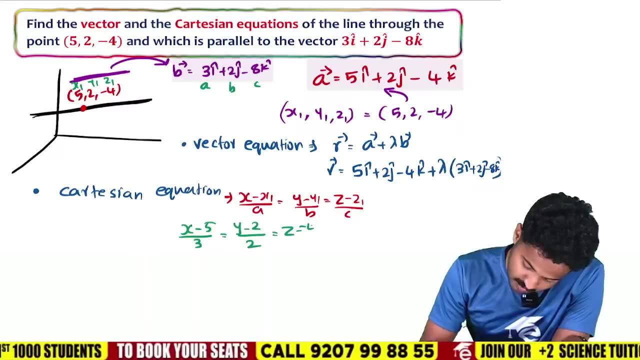 This is equal to y minus This is y1.. This is y1.. This is 2.. So y minus 2 by b is 2.. This is equal to z minus z1 is minus 4.. So z minus minus 4 by c is minus 8.. 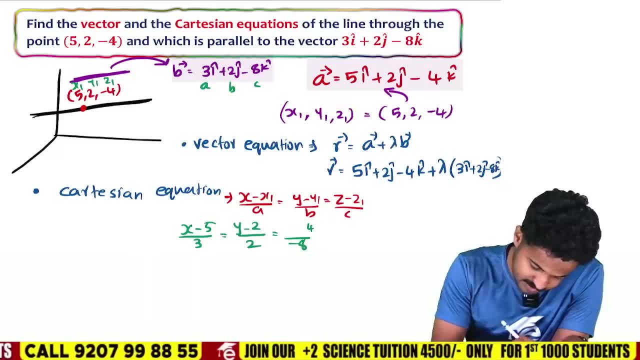 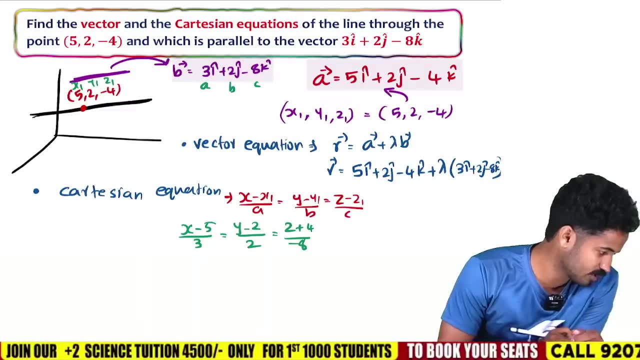 So this is it. If you want this minus and minus, what do you do? This is plus, So z plus 4 will be the answer. Ready, Ready, Okay, Okay, fine, So this is how you write the Cartesian equation and vector equation. 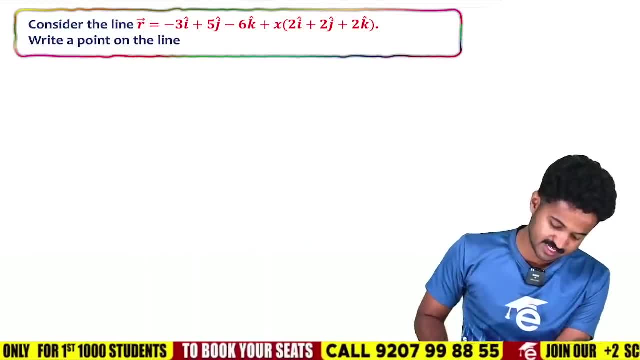 It's simple. It's easy. Now look at this. Consider the line. I have given you a line. Write a point on the line. I told you to write a point on this line. Say it fast. How do we write a point on this line? 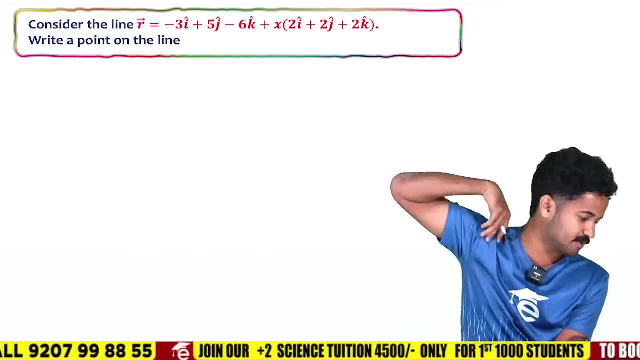 How is it? Is it okay? Do you get a green ticket fast? You don't have to comment on the answer in the comment box, You just have to get a green ticket, If it's okay. you don't have to do it without time. 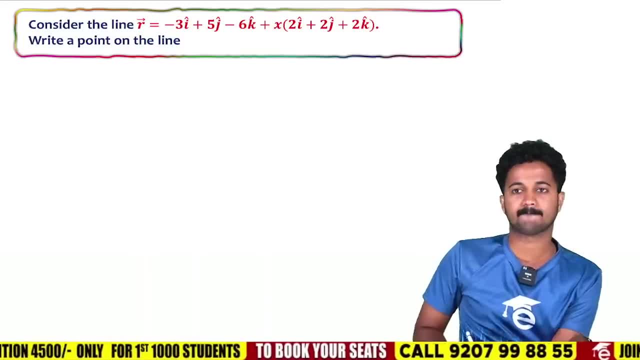 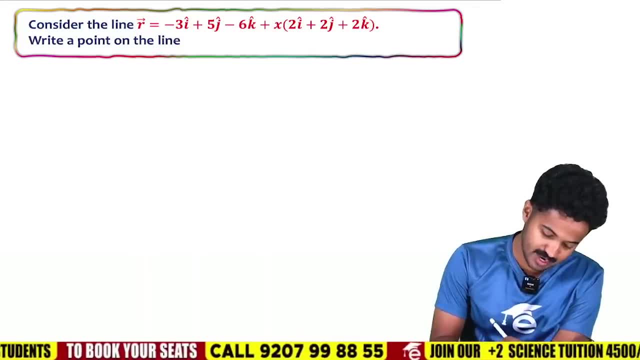 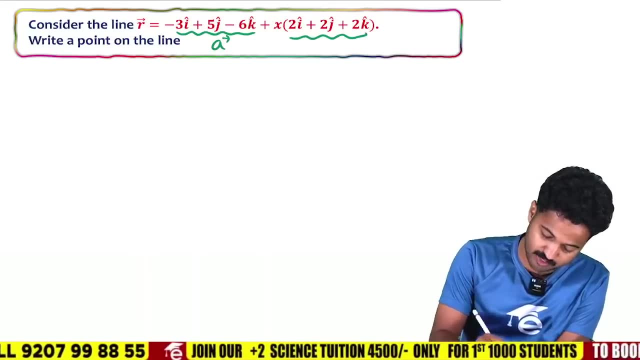 Sorry, I have given you the equation of this line. I asked you a point on this line. If you give me the equation of this line, you can write it correctly. This is A vector R, equal to A plus lambda B. This is B vector. 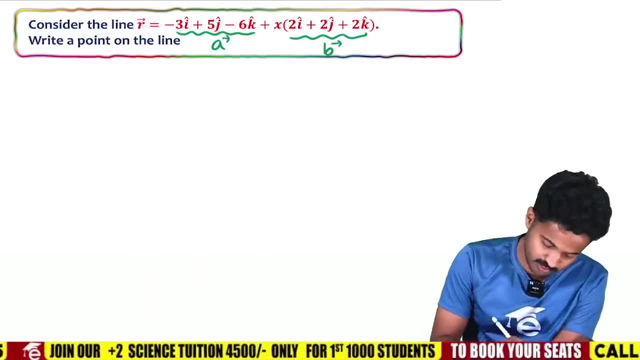 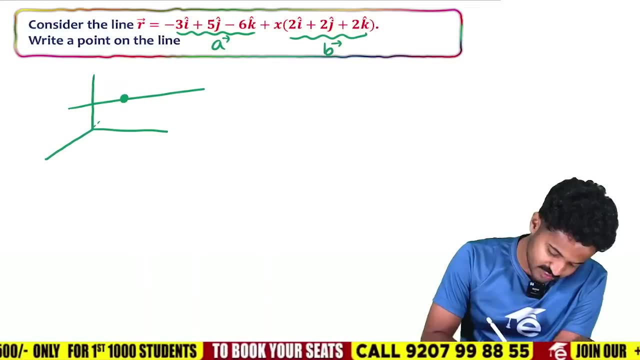 Okay. So if that's the case, Okay, Very good, Very good, Very good. You have told me the answer. That is, if you get the equation of that line, there will be a point on that line And this will be the vector A. 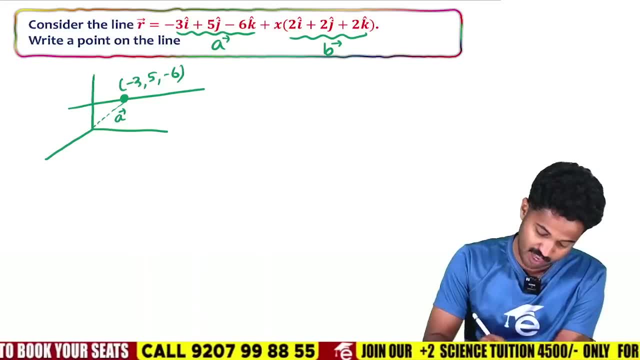 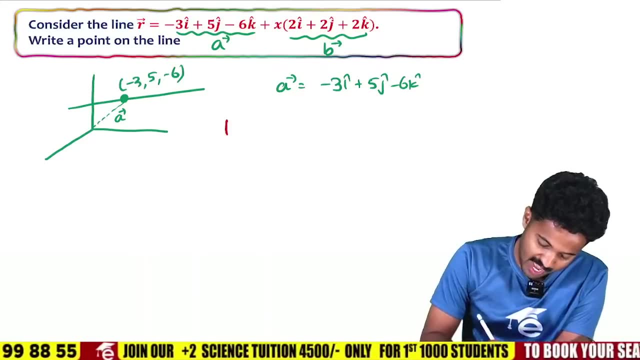 That is minus 3.. 5. Minus 6. Isn't it A vector? If you get A vector minus 3, I plus 5, J minus 6, K, point. If you have told me a point on that line. 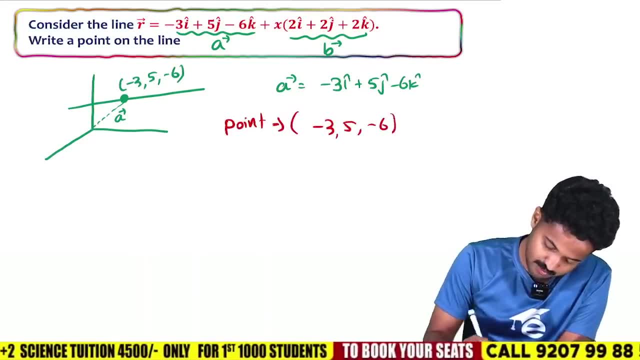 it is very easy: Minus 3,, 5, minus 6.. You can write it yourself Easy: Minus 3,, 4.. Minus 3, 5, minus 6.. Okay, Ready, Okay. 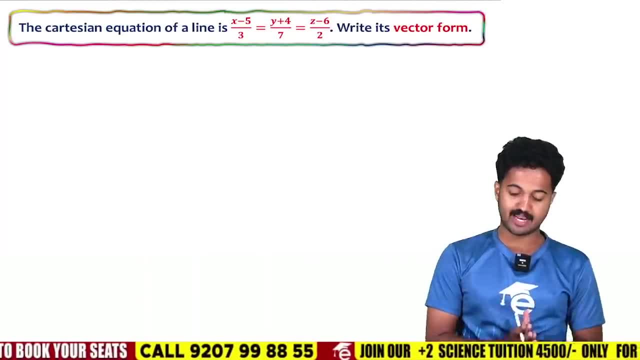 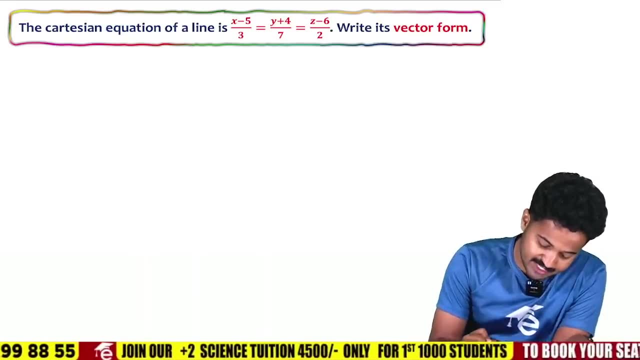 No problem. So, if that's the case, the Cartesian equation of a line. I have given you the Cartesian equation. How do you make a vector out of it? It is very easy. Look, We have to remember the Cartesian equation. 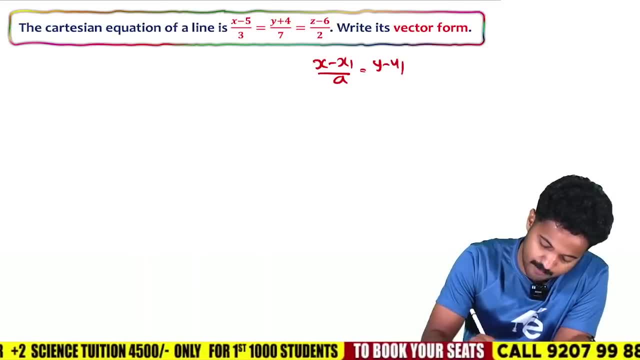 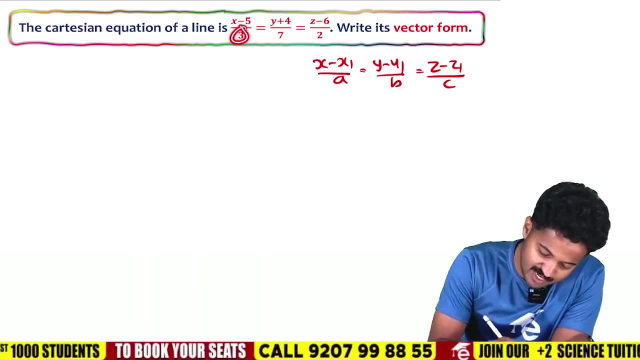 X minus X1 by A, equal to Y minus Y1 by B, equal to Z minus Z1 by C. And that's what you said. First, what is there in the denominator That would be the parallel vector with A, B and C? 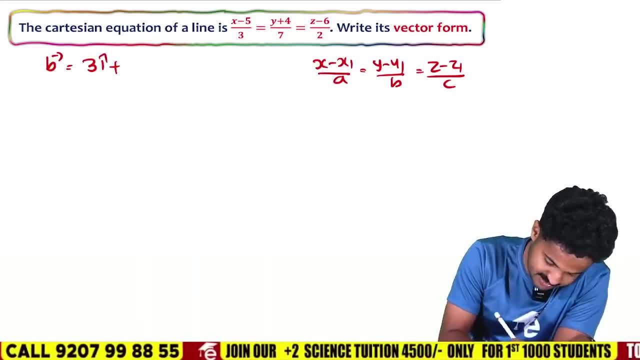 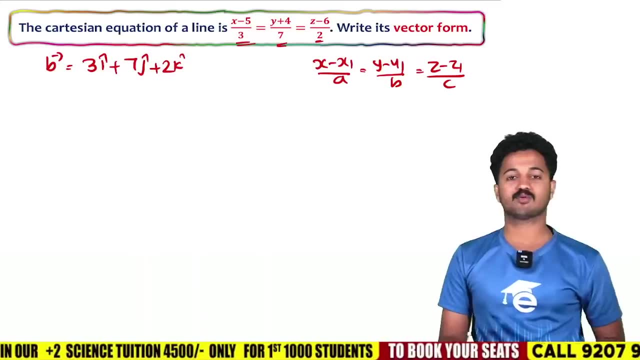 That's B. What would be the B vector 3 I plus 7, J plus 2 K? What is there in the denominator, That is the parallel vector X minus X1 by A, Y minus Y1 by B, Z minus Z1 by B? 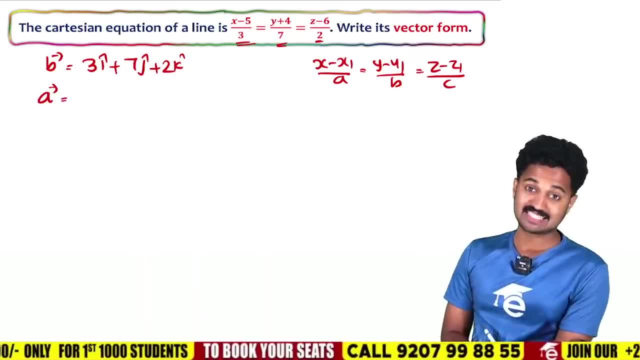 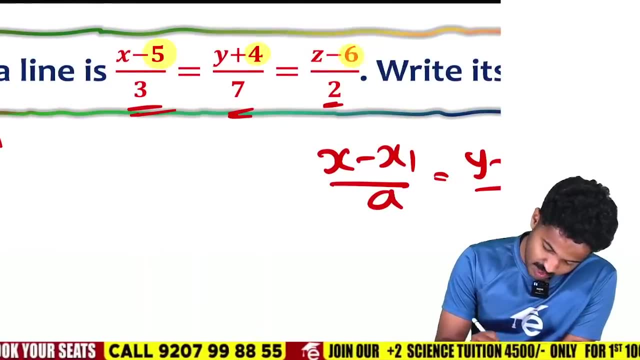 Z minus Z1 by C, What is the A vector, X minus X1.. Pay attention to that Here. look What is given here. What is given here. That is not what you have written There. you have checked whether there is a minus in front of it. 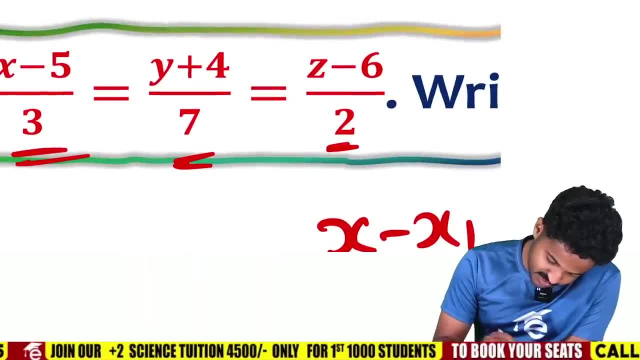 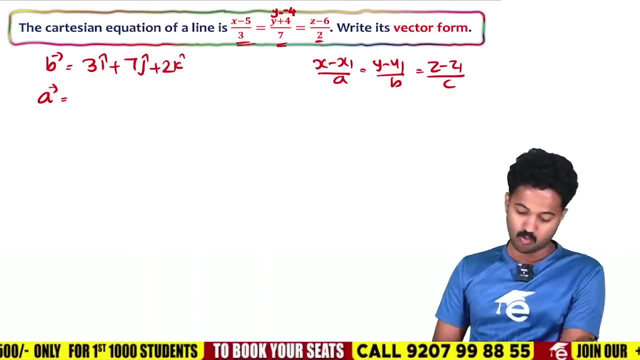 So look, X minus 4.. That is okay. Here you have Y plus 4.. You have to remove that. You have to write Y minus minus 4.. And then you will do it. You have to write Y minus minus 4.. You have to write Y minus minus 4 in that formula. You have to write Y minus minus 4 in that formula. That is necessary. That is necessary. You have to write Y minus minus 4 in that formula. That is necessary. 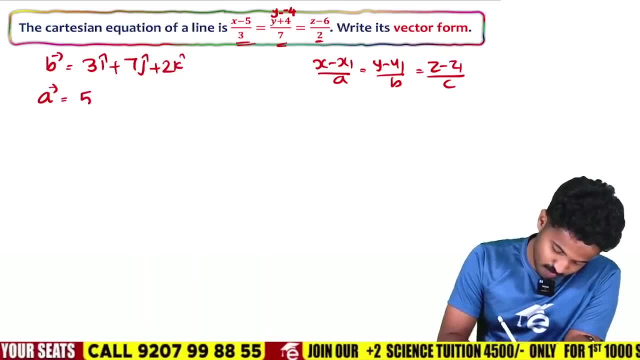 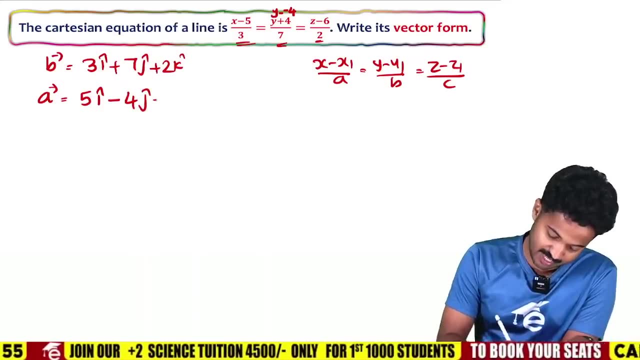 So look, X1 is 5.. So you have to write 5I. Then what is Y1?? It is not 4.. It is minus 4.. So it is minus 4J. What is K there? 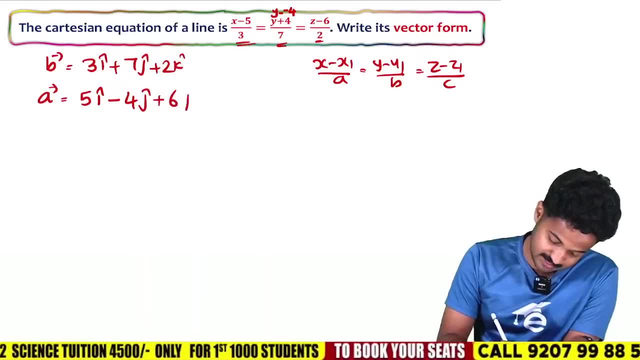 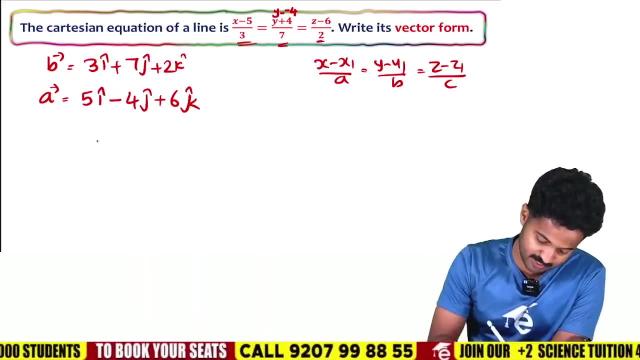 Sorry, What is Z, X1, Y1, Z1.. That is 6J, Sorry, 6K. Okay, ready. So you have got all these things. You have got A, B and C. Now it is easy to write the vector form of this. 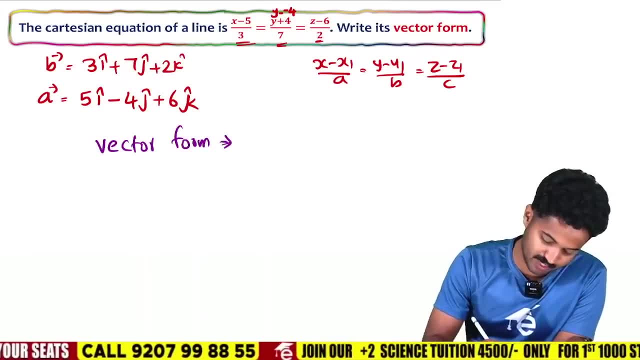 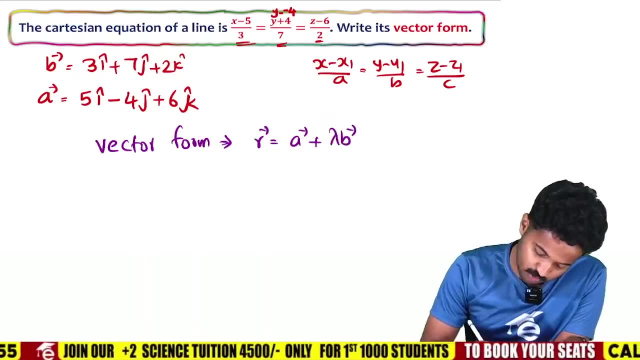 Vector form. Vector form. Okay, If you say vector form, you can comment on the vector equation: R equal to A plus lambda B. Yes, very good, If that is so. look, If you say A, it is 5I minus 4J plus 6K. 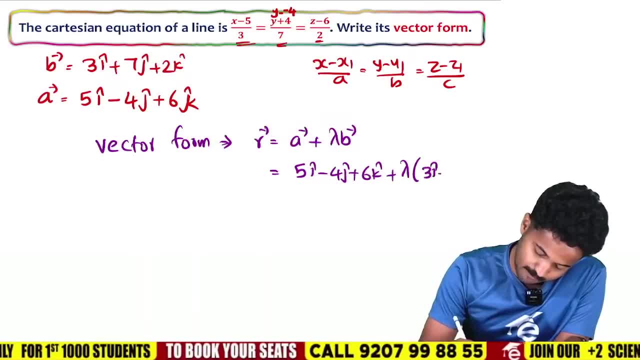 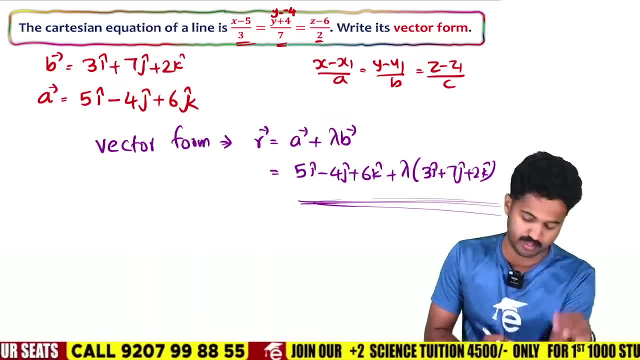 plus lambda into B is 3I plus 7J plus 2K. Got it Easy. If it is easy, if it is simple. if it is simple, very good. K You can write. K You can write lambda. 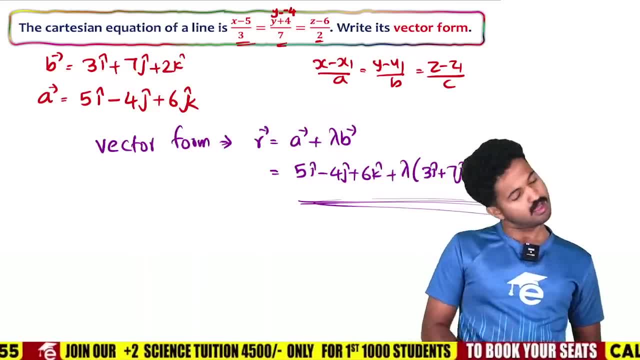 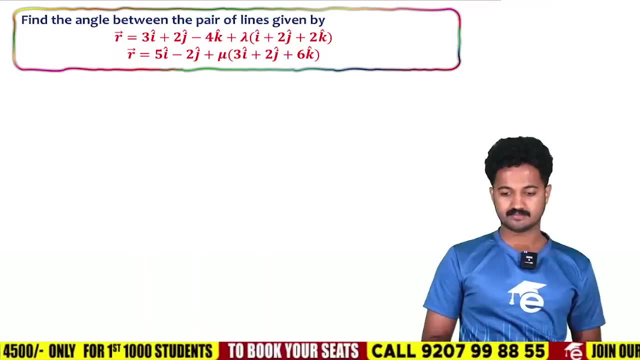 It is not constant. If you write K, you will get the component K. So this is the answer. It is easy, No problem. No problem. Next, Each. This is an important thing in this chapter. You should have studied this. 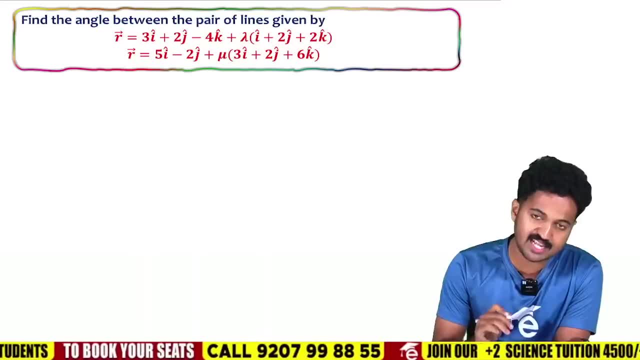 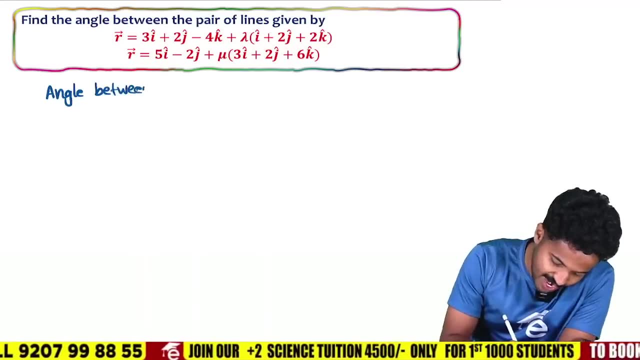 You should have known this correctly. Okay, Look, If you have given the equation of two lines- angle between two lines, Angle between two lines- You can learn the equation. Angle between two lines is easy, It is very simple Look. 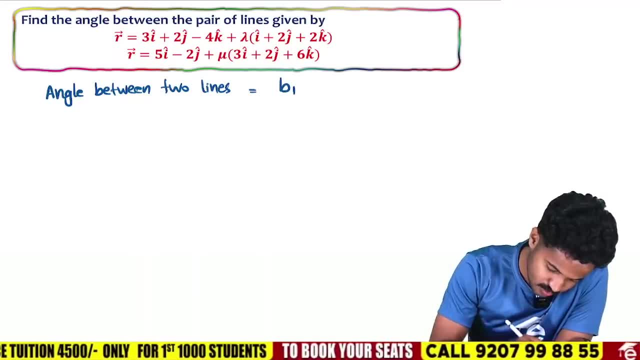 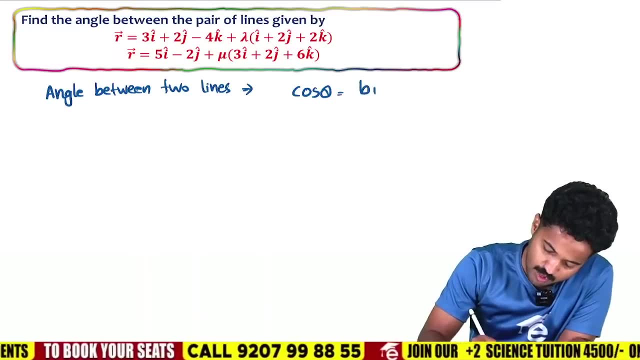 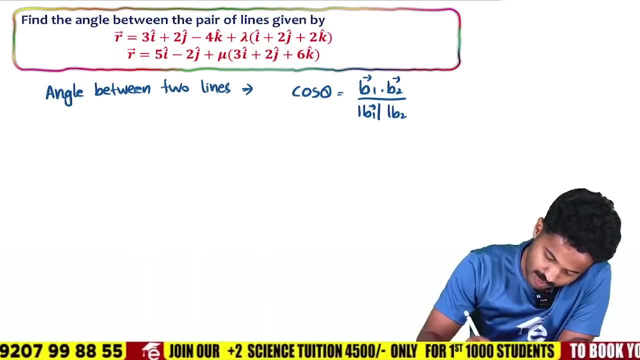 B1 dot B2.. You have to take cos theta right Angle between two lines is equal to this, Like this: Like we said earlier, there is no big difference Cos theta is equal B1 dot B2, divided by magnitude B1 into magnitude B2.. 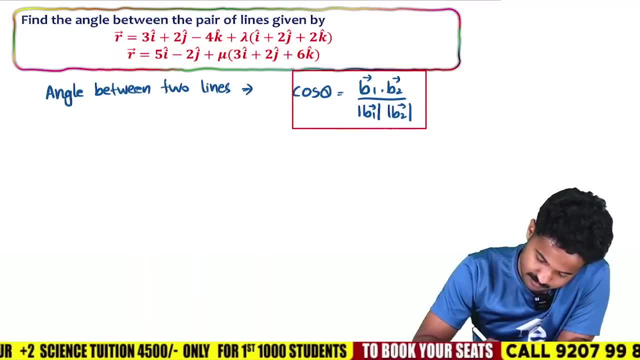 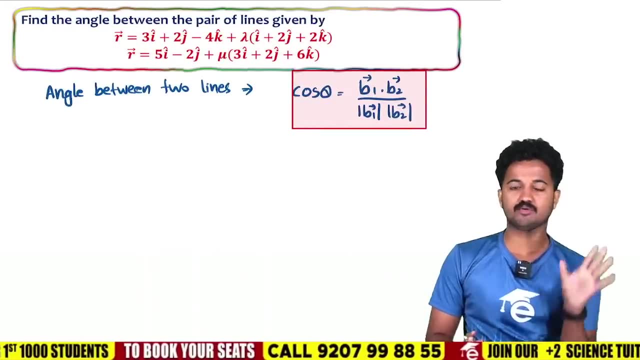 This is the angle between two vectors. Sorry, Angle between two lines, Sar. So we need to know two things: B1 and B2 are the same. If we write the equation of a line, we will write it as R equal to. 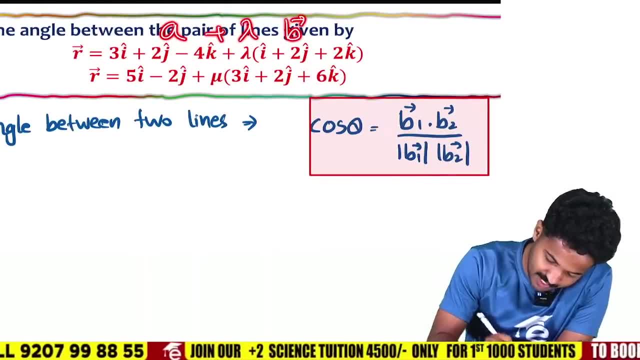 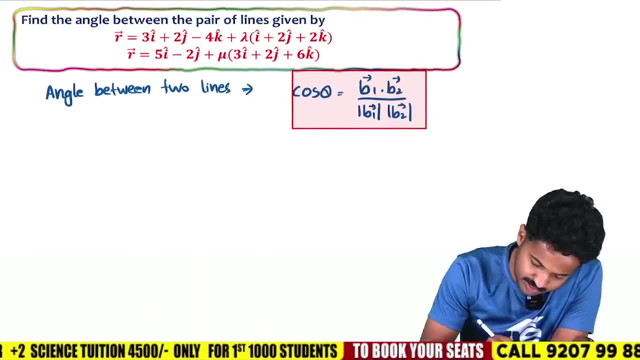 Look, Isn't it R equal to A plus lambda B? Isn't R equal to B2? if there is a second line, It is easy, sir, It is simple. Look. So this vector right, This vector. Similarly, this vector right. 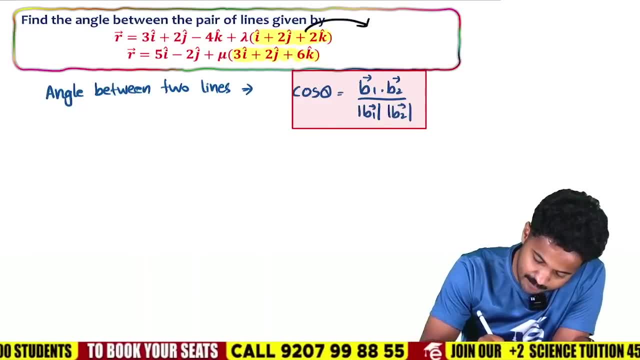 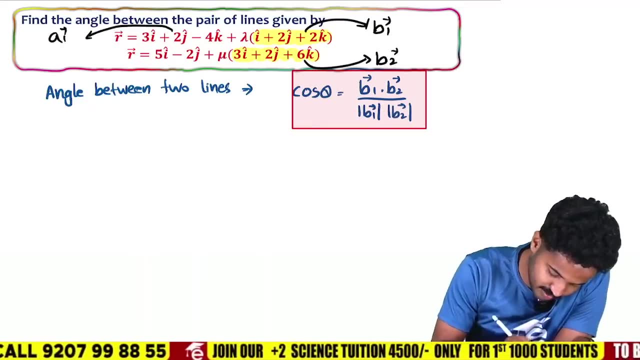 These two vectors should be considered, Which means this is the vector called B1.. And this is the vector called B2.. Okay, right, So this will be the vector called A1.. This will be the vector called A2.. 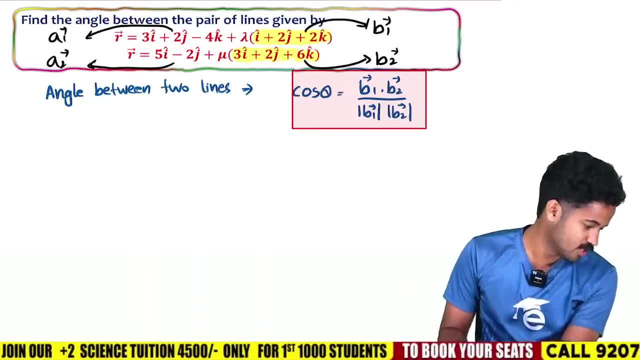 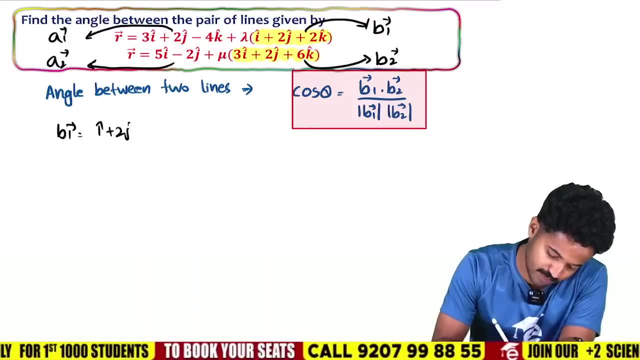 We need B1 and B2 here. very much, Right, Sir? when will we get it Time? You have to give me 15 more minutes. That is mandatory. B1 is i plus 2j plus 2k, And what is B2, sir? 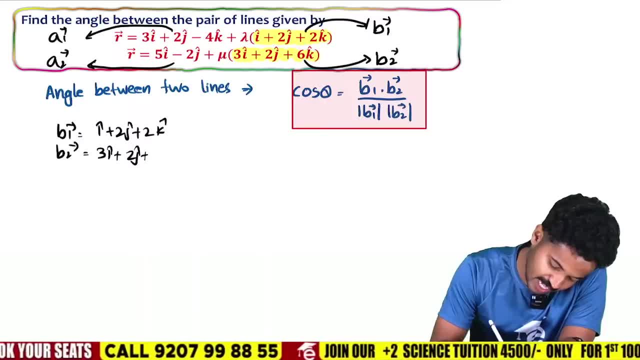 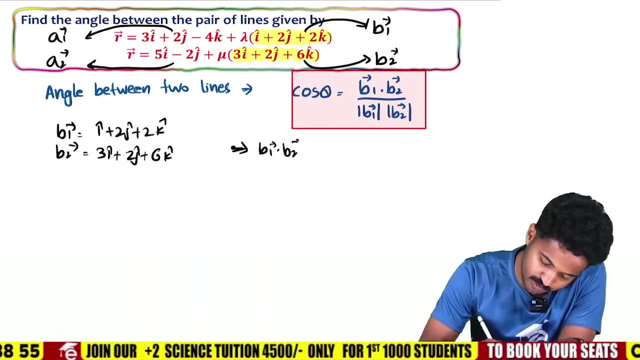 B2 is 3i plus 2j plus 6k right? Yes, We know that too. Find out everything you need First. First, What is B1 dot B2?? B1 dot B2 is 1 into 3.. 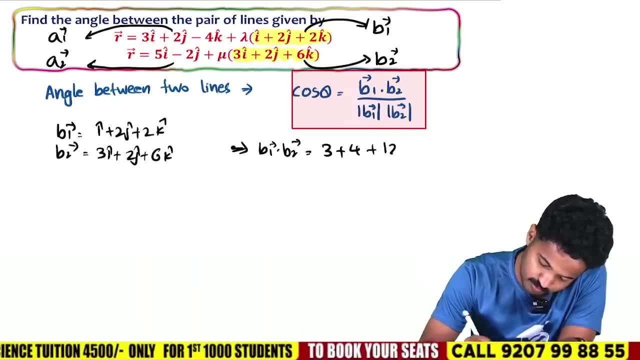 3 plus 2 into 2 is 4 plus 2 into 6 is 12.. Okay, let's do it like this. Okay, right, I am not telling you in detail. 3 plus 4 is 7, plus 12 is 19.. 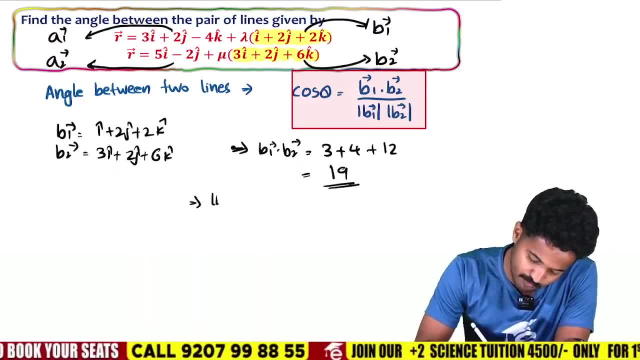 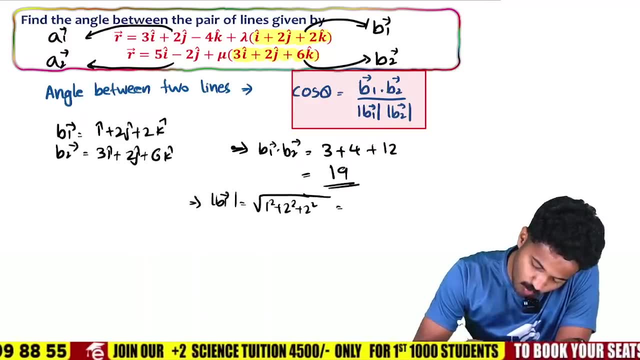 Let's find out Now what is magnitude B1?. What is magnitude B1?? Magnitude B1 is root of 1 square plus 2 square plus 2 square, That is, 1 plus 4 plus 4.. That is root 9, which is equal to 3.. 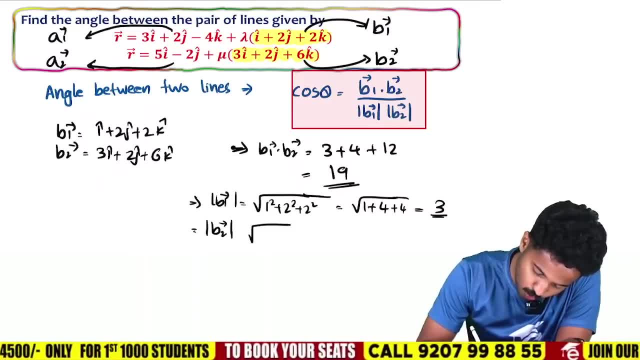 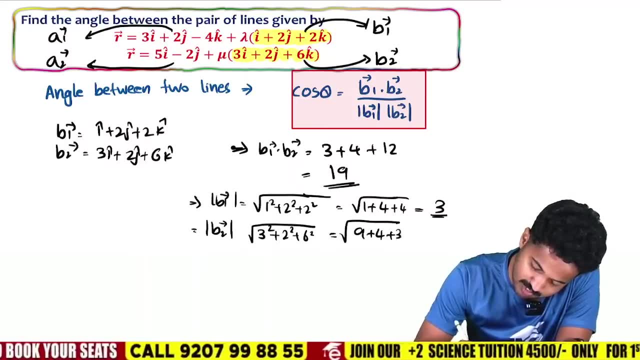 Now, if you say magnitude B2 is root of 3 square plus 2 square plus 6 square, That is 9 plus 4 plus 6 square is 36.. So which means the root of 49 is 7.. 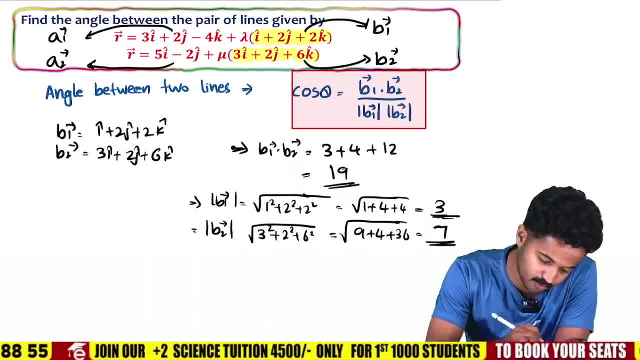 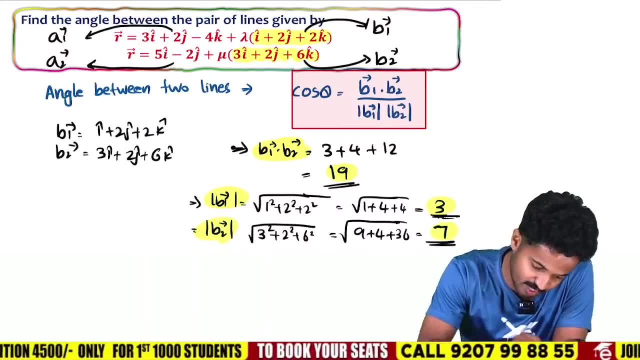 Okay, Yes, find it, Find it. The answer is being commented. Now look, You got everything you need. You got B1, dot. B2 is 19.. You got magnitude B1 is 3.. You got magnitude B2 is 7.. 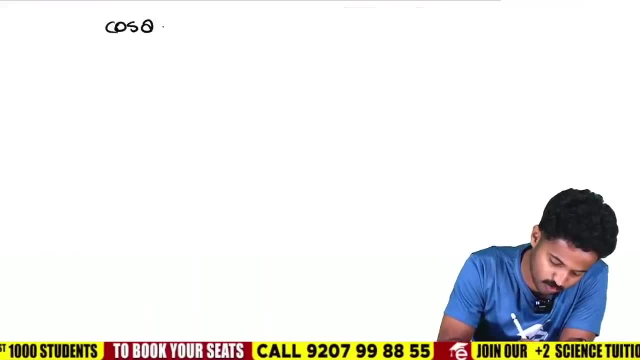 Now find the answer. Okay, Cos theta is equal to Look: B1 dot B2 is 19.. 19 divided by magnitude B1 is 3.. Magnitude B2 is 7.. So theta is equal to cos inverse 19 by 21.. 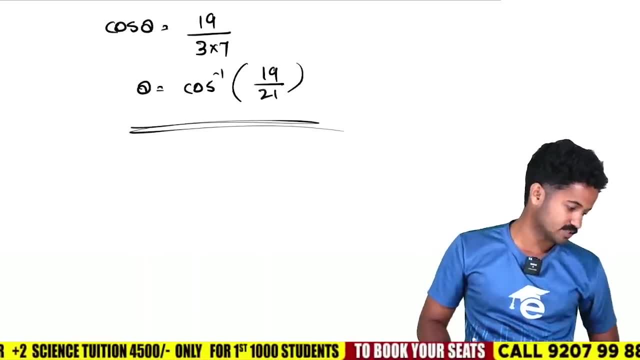 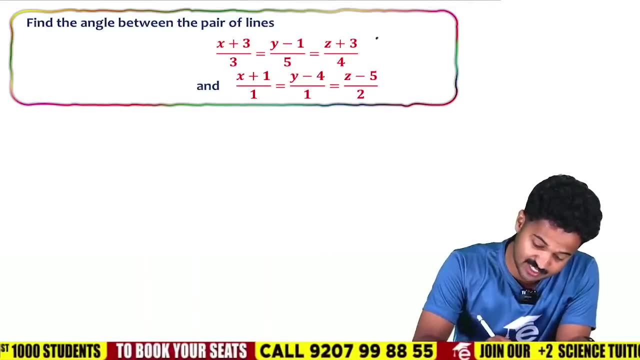 This is the final answer. It is easy, right? It is simple, right? Yes, 19 by 17 is not 19 by 21.. Easy: Find the angle between the pair of lines. Here you got Cartesian form. 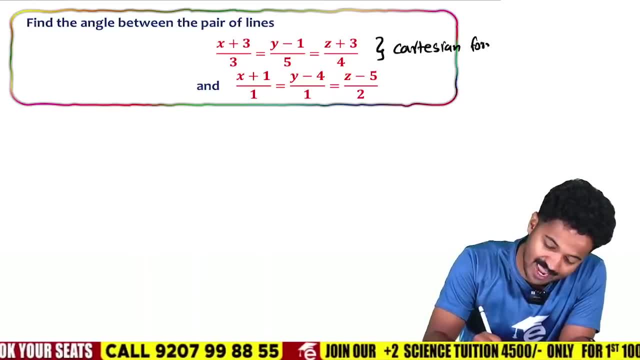 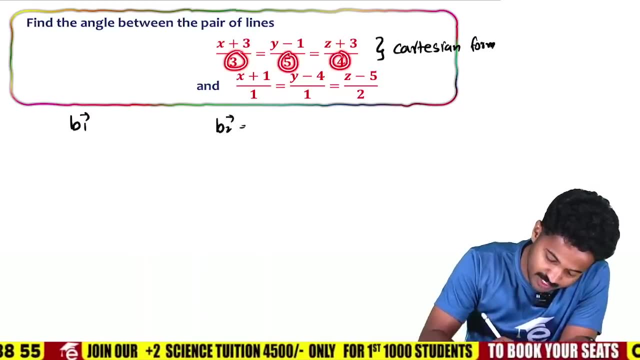 Cartesian equation is Cartesian form. So we need to find the angle between B1 and B2.. Parallel vector is what I have told you. If you add this in denominator, what will be the parallel vector? That is how B1 is. 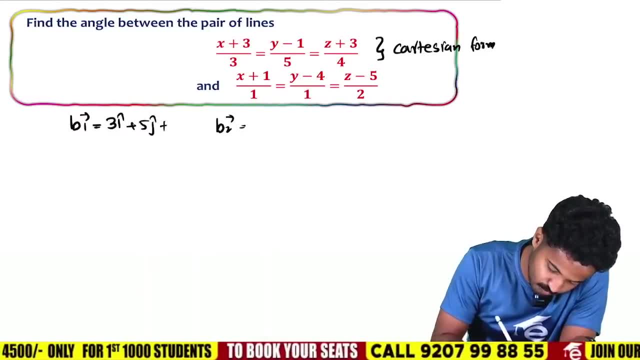 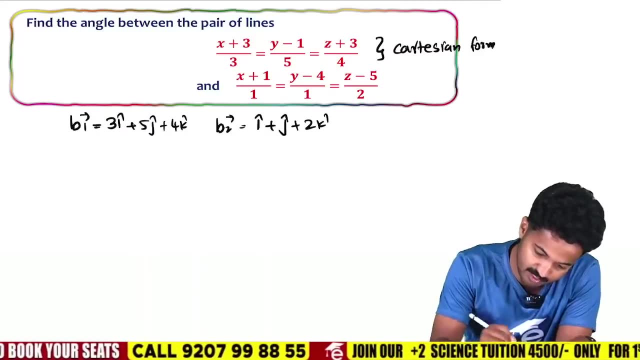 First line is 3i plus 5j plus 4k Easy, And B2 is 1 into i, B plus 1 into j, j plus 2k Easy. right Now what you need is magnitude B1.. 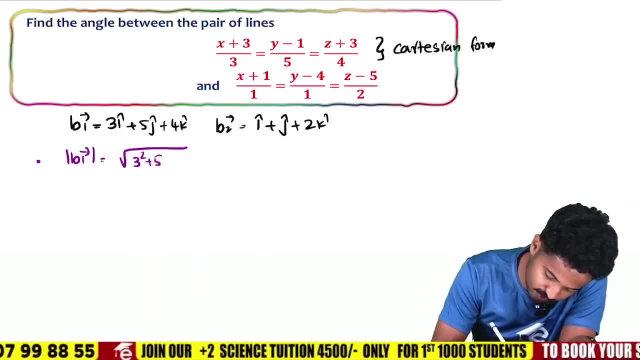 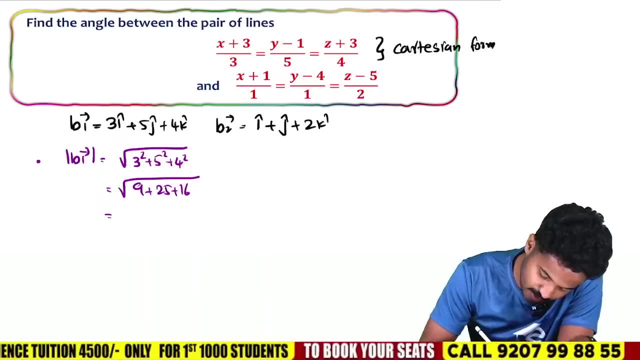 Magnitude B1 is root of 3 square plus 5 square plus 4 square, That is 9 plus 25 plus 16.. So the answer will be root 50.. Okay, Now, what is magnitude B2?? Magnitude B2 is root of 1 square plus 1 square plus 2 square. 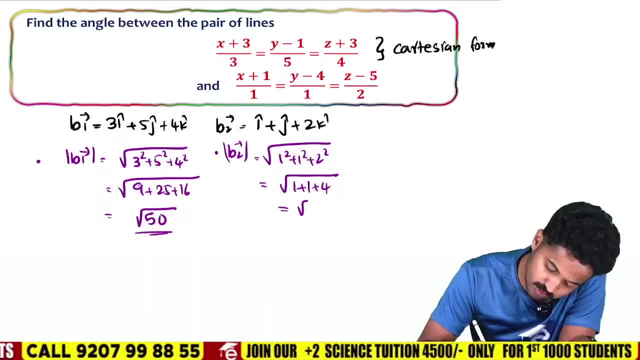 That is 1 plus 1 plus 4, which means root 6.. Okay, And what is B1 dot B2?? How do we find B1 dot B2?? It should be written in more detail: 3 into 1.. 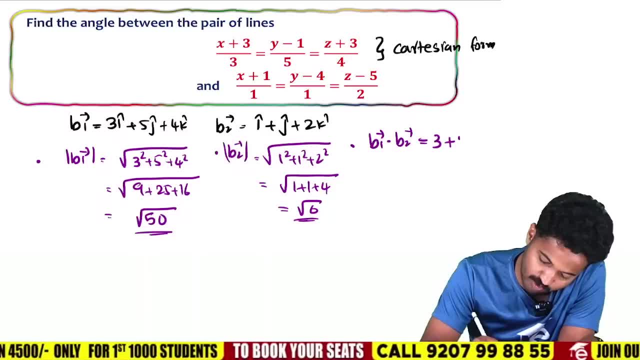 3 plus 5.. We will take 2 plus j. 5 plus 1 is 5.. 5 into 1 is 5.. 2 into 4 is 8.. So the answer is: 3 plus 5 is 8.. 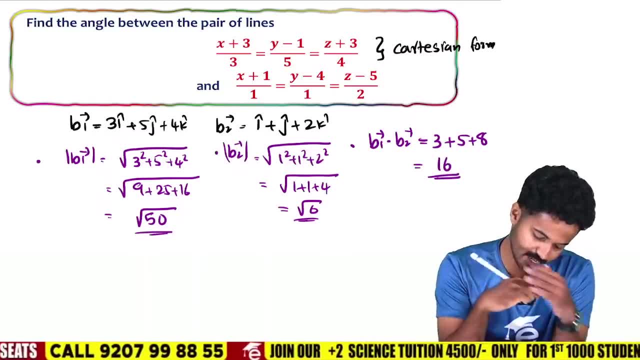 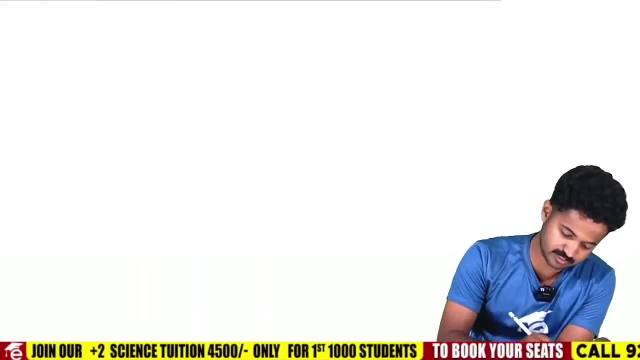 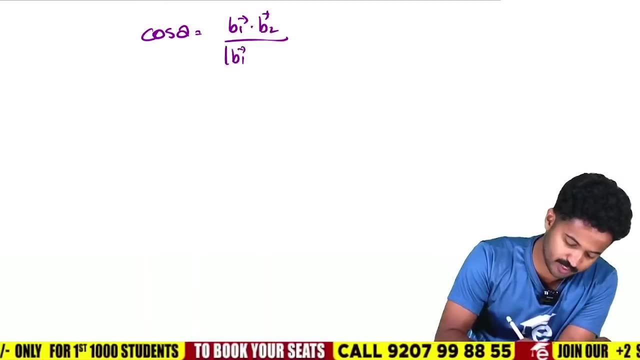 8 plus 8 is 16.. Okay, Are you ready? Comment the answer: Root 15.. Root 6.. So look, Got it. Cos theta is equal to Cos theta is equal to B1 dot B2 divided by magnitude B1 into magnitude B2.. 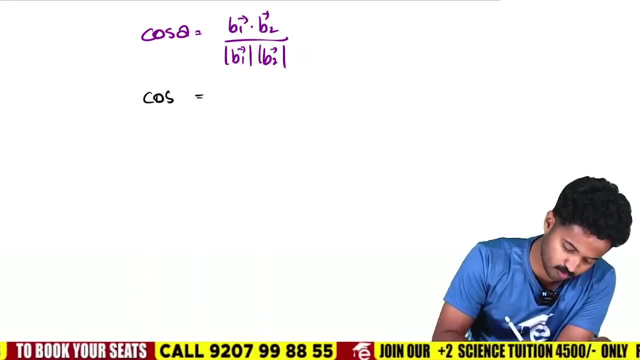 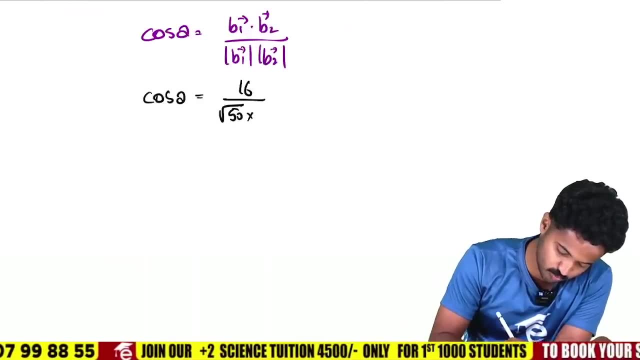 Angle between two lines. So the answer: cos theta is equal to B1 dot. B2 is 16.. 16 by magnitude. There is root 50 into root 6.. So theta is equal to cos inverse. Write it like this: 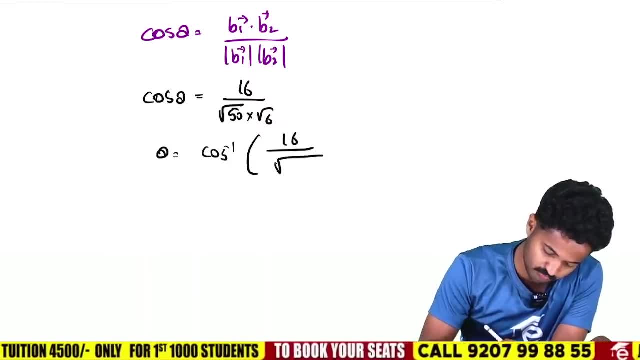 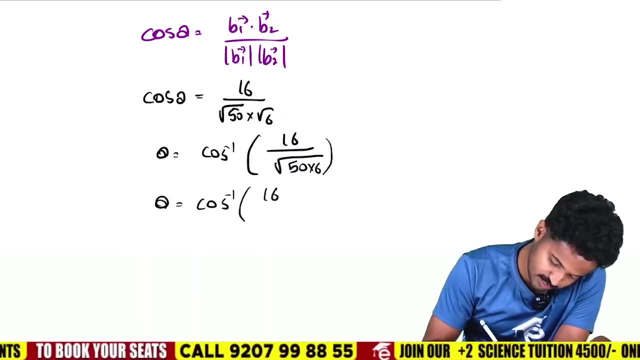 Don't make any big changes. 16 by. If you want, you can write root of 50 into 6 like this. Write it like this, There is no problem. So theta is equal to cos. inverse. 16 by 5 over 6 is 30.. 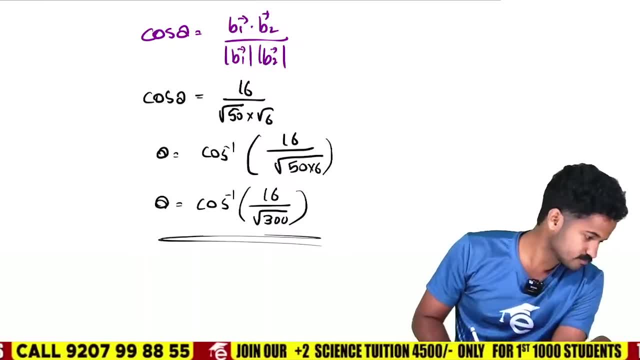 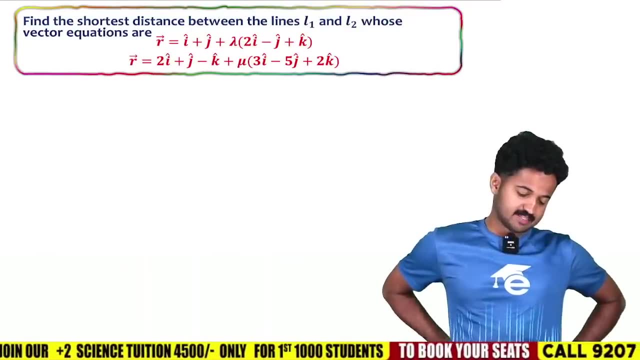 So the root is 300.. So this is the answer. Okay, Ready, Okay right. So it's simple and easy. And the next one: Find the shortest distance. You should definitely learn this: If you give two lines and give the shortest distance between them. 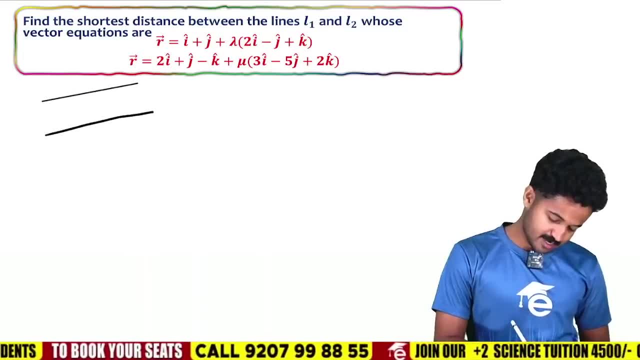 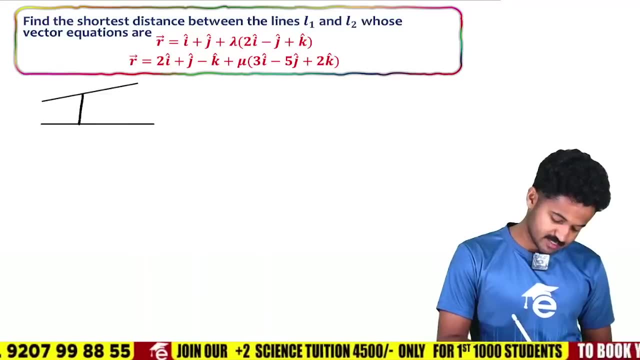 That is, there are two lines. Look, there are two lines. There are two lines. It's not parallel, It will be a skew line somehow. So consider the shortest distance between the two lines. The shortest distance is the perpendicular distance. 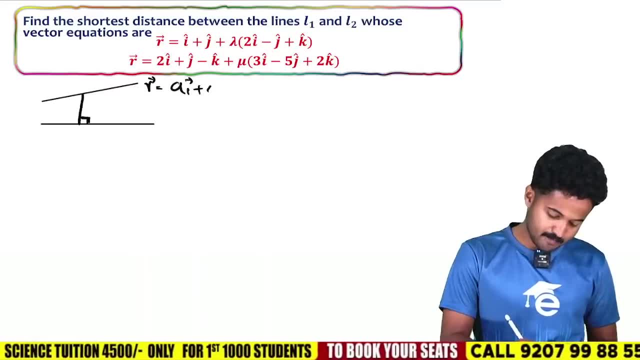 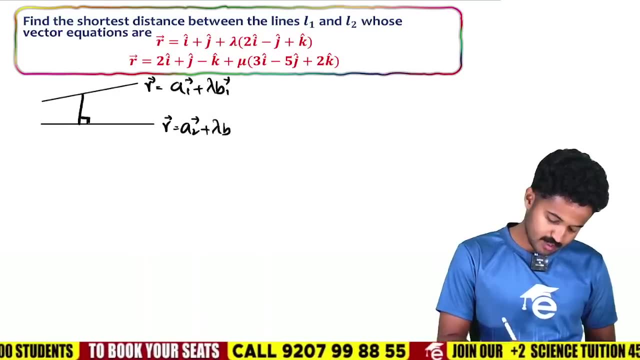 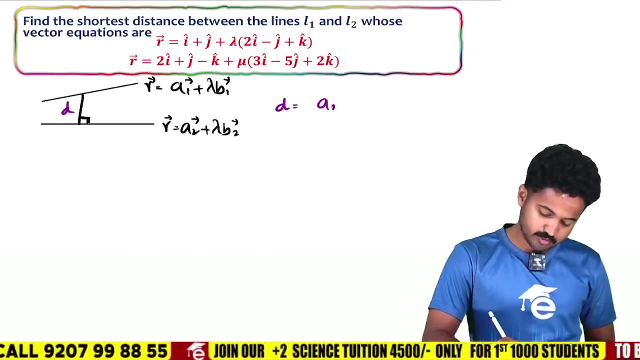 This is r equal to a1 plus lambda b1.. Similarly, if this is r equal to a2 plus lambda b2, the shortest distance between these two lines is d. It's a very simple equation. Try to learn it. d equal to a2 minus a1. 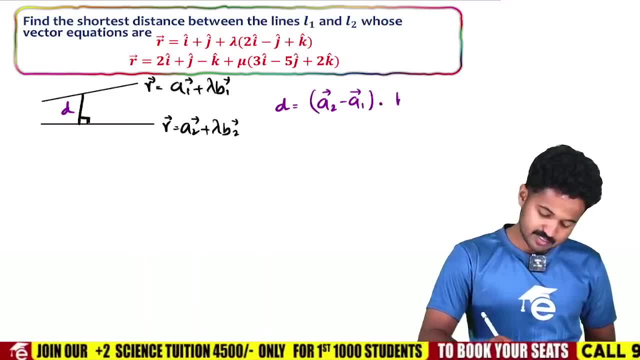 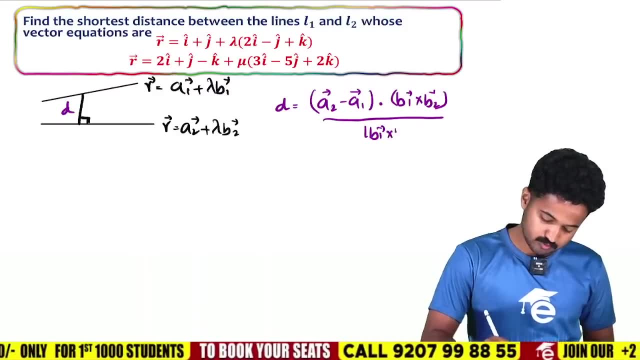 a2 minus a1. Dot. Then you have to do dot as b1 and b2 cross Divided by magnitude of b1 cross b2.. It will be a big problem. It's a simple thing to do. I will give you one problem in this. 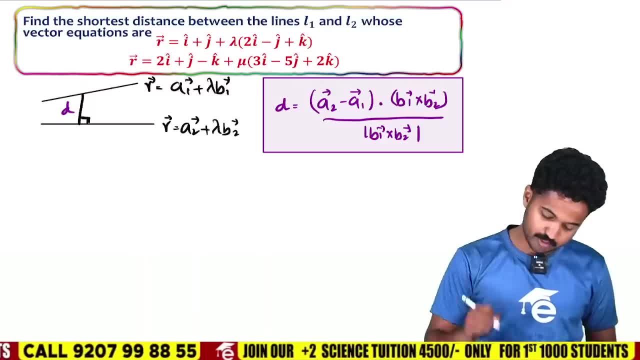 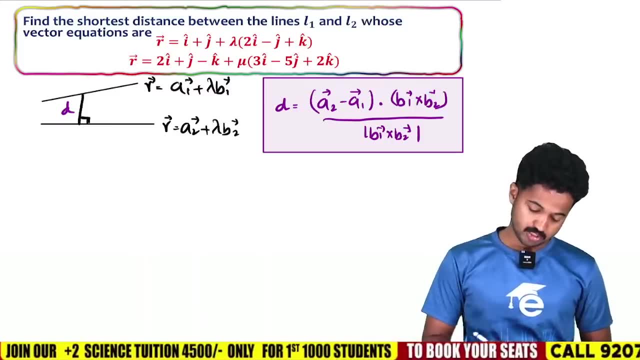 You have to do one problem as homework. It will be in the Cartesian formula, So you have to learn the equation first. That's what you have to do. It's easy, right? There are no problems, right? So the equation is essential. 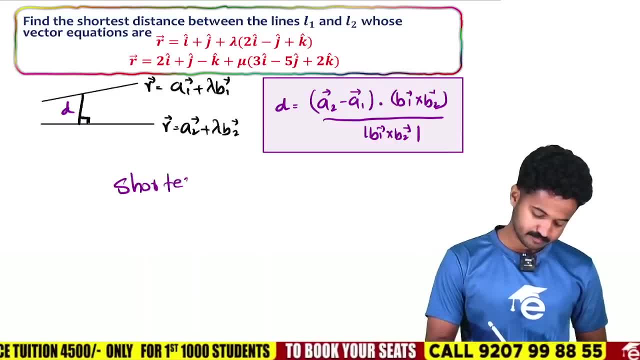 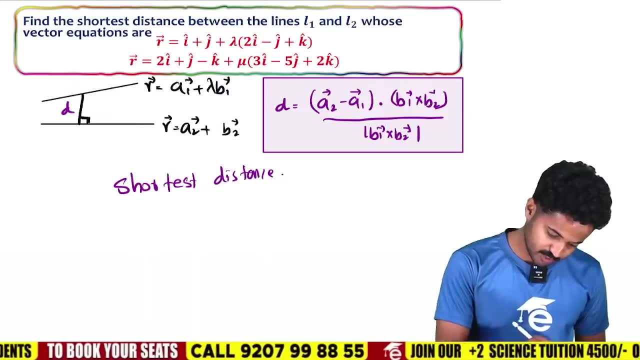 Shortest distance. The equation of shortest distance is the shortest distance. Okay, You don't have to put lambda here. You don't have to put lambda here. You give another letter here, like mu Mu. They are both constant, right? 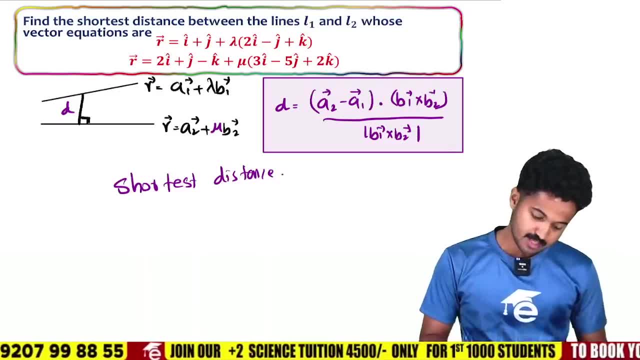 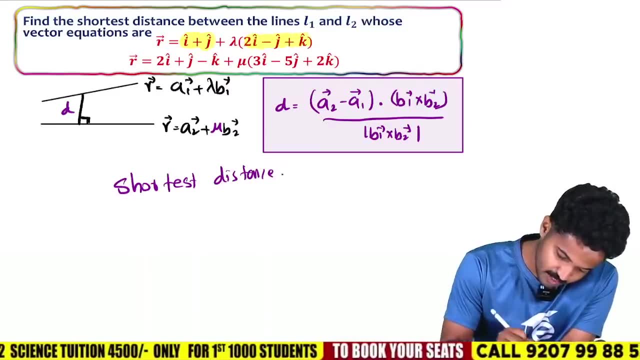 If they are both constant, then it will be different. Ready, Okay, simple. So, sir, as I said earlier, right, Just as I said earlier, This is a1.. This is b1.. Okay, right, What is a2?? 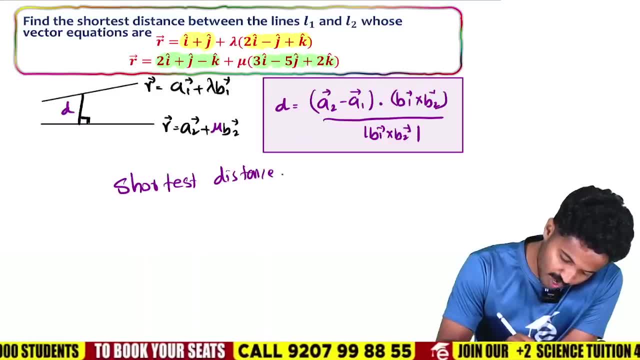 And what is this? b2.. It's okay, right? So see, Add those things to your mind first, right? This is a1 and this is b1.. And this is B2 and this is A2.. If you have understood these things properly, you can do all these things. 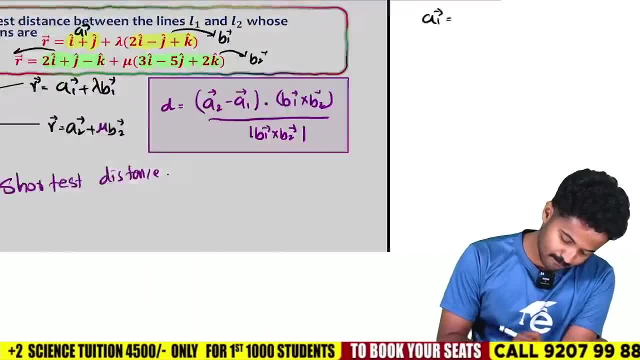 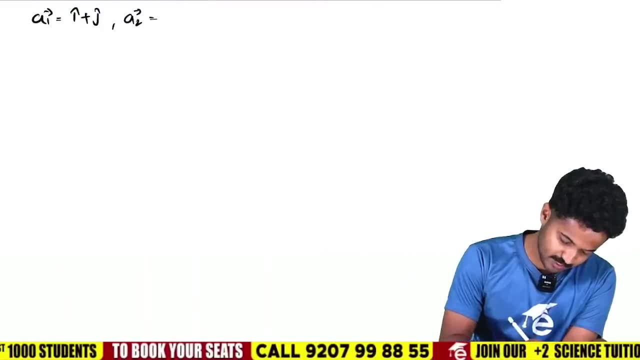 Just write it down. We need everything. A1 is I plus J. If you have said A2, what is A2?? Vector A2 is 2I plus J minus K, 2I plus J minus K And the next one. 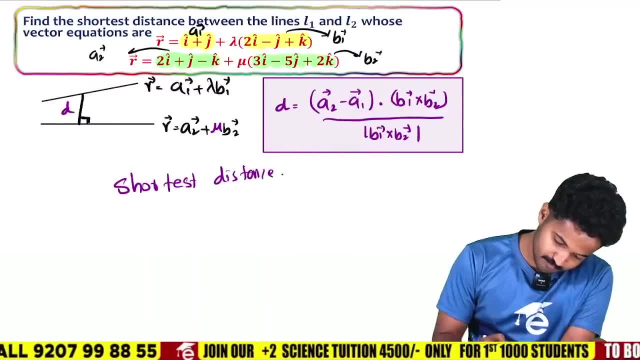 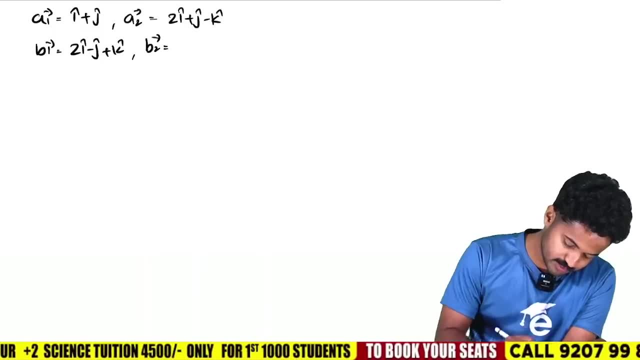 We have got that. Now. what is B1?? B1 is 2I minus J plus K. What is B2?? If you have said B2, it is 3I minus 5J plus 2K. Got it. 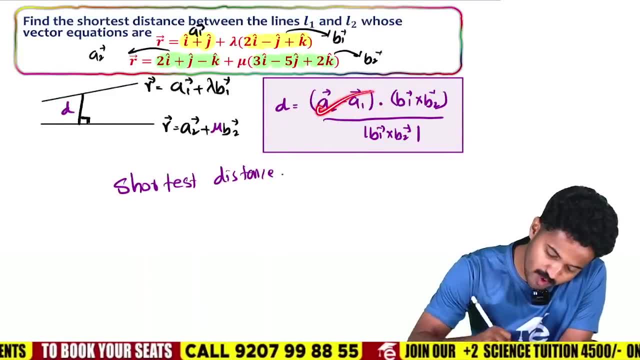 We have got everything we need. Now let's find out what we need. We need to find A2 minus A1.. We need to find B1 cross B2.. So let's do it one by one and get to the final answer. 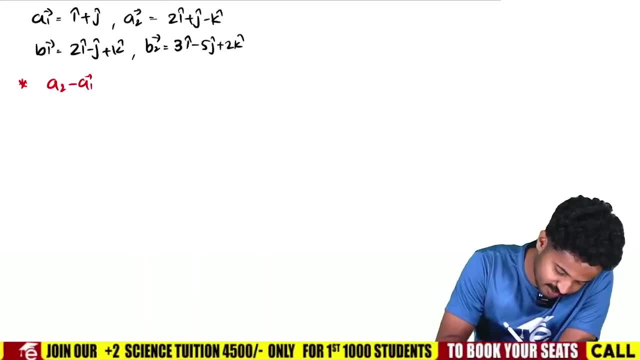 Look First: A2 minus A1.. This is easy to find: A2 minus A1.. Look, I plus 2 minus 1.. 2 minus 1 is 1.. So I Plus J Minus J. 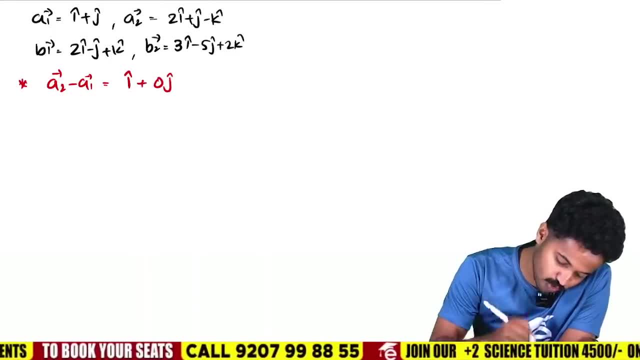 0.. It is 0.. So 0J Minus 1.. There is nothing there. So minus 1 minus 0 is minus K, Okay. So the answer for this is: I minus K, Okay. 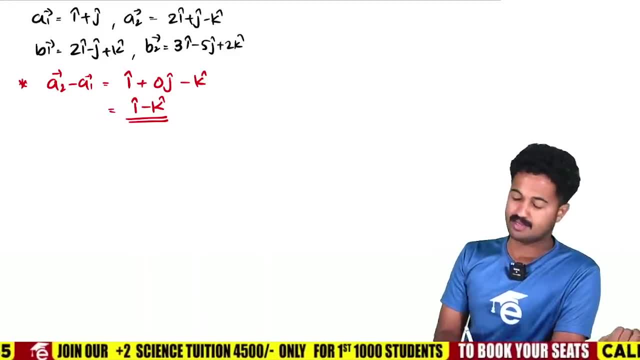 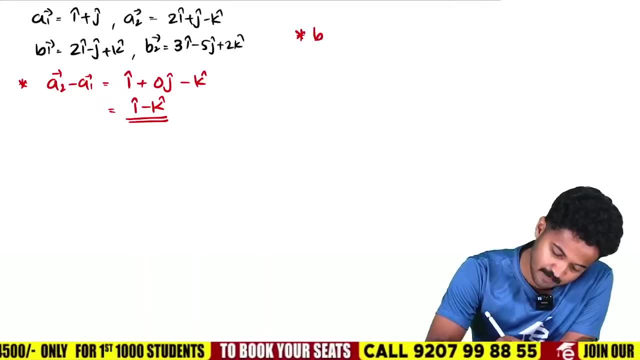 I minus K, Or I plus 0J minus K, That is A2 minus A1.. That is very simple. We can do it without any big problem. Now the next one you need is B1 cross B2.. Look. 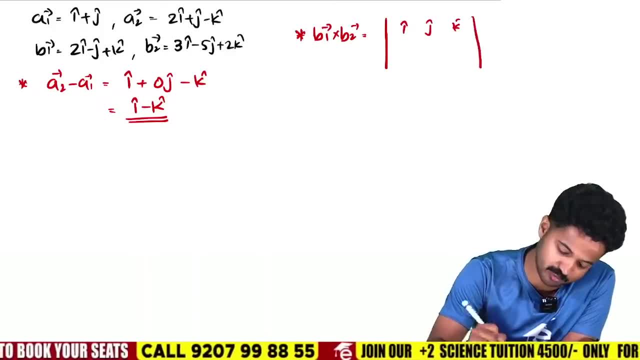 B1 cross B2.. Look, First row is I J K, Second row is B1.. What is this? It is 2 minus 1. K plus 1. B2, 3 minus 5, 2.. 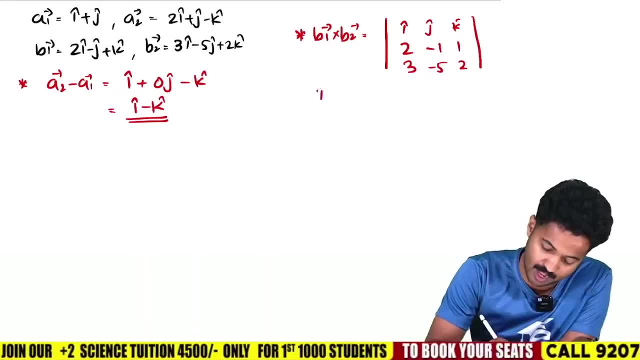 Do it like this. What are the components of this? Just give this- So that is I- into row. cancel colon. cancel 2 into minus 1, minus 2.. Minus 1 into minus 5, minus 5.. 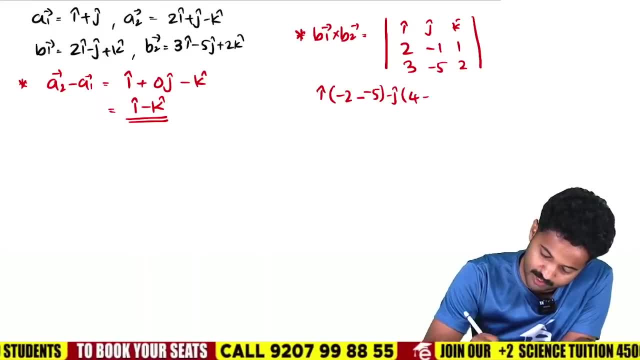 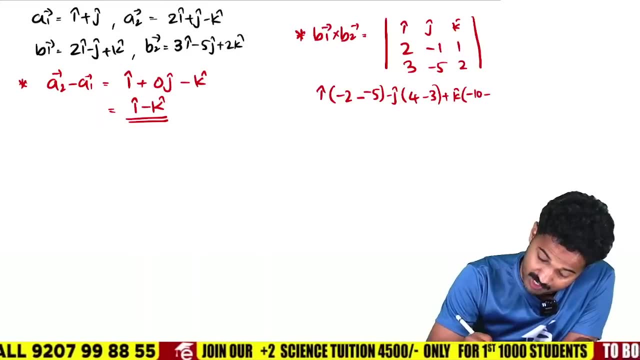 Minus J into row cancel colon cancel 2 into 2, 4.. Minus 1 into 3, 3.. Plus K into row cancel colon cancel 2 into minus 5, minus 10.. Minus 1 into 3, minus 3.. 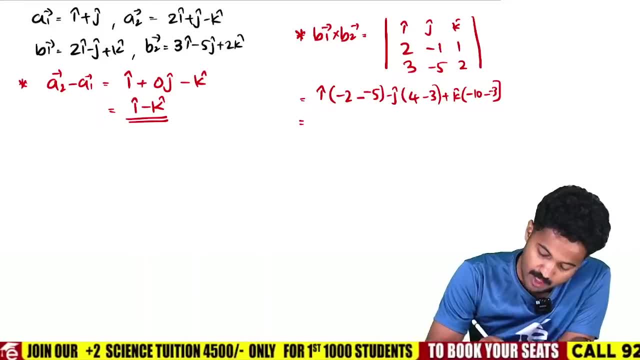 This is with the belief that you know how to do it. So look, Minus 2 plus 5, 3.. So 3I. 4 minus 3 means 1. 1 into J J, So minus J. 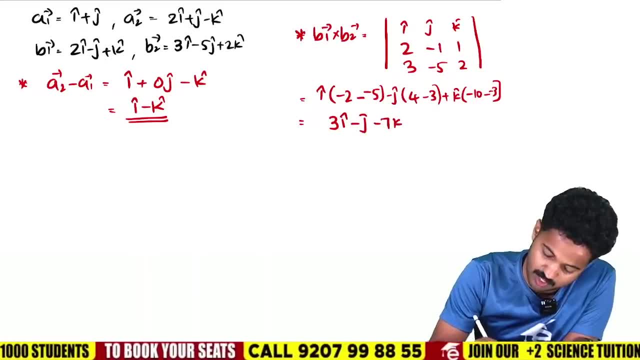 Minus 10 plus 3 means minus 7.. So minus 7K. Okay, Ready, No problem. Now let us find the magnitude of this. We need that too. So magnitude: B1 cross B2.. Magnitude: B1 cross B2 means: 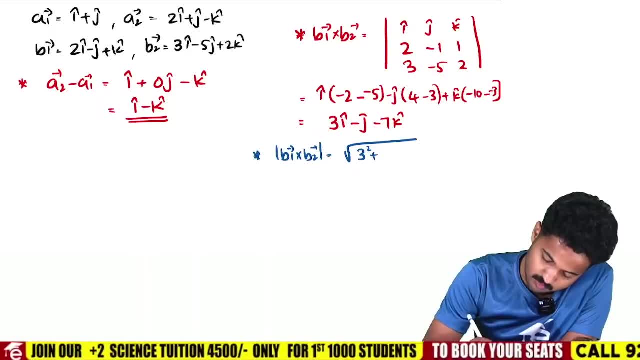 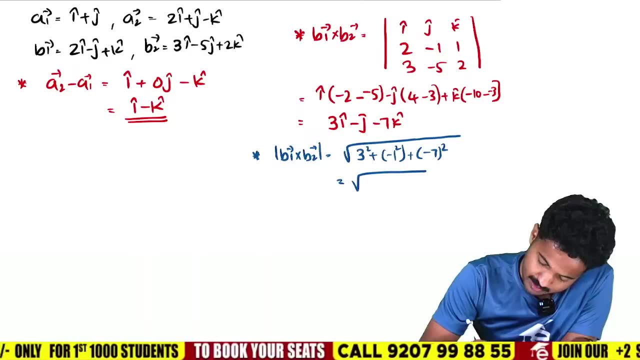 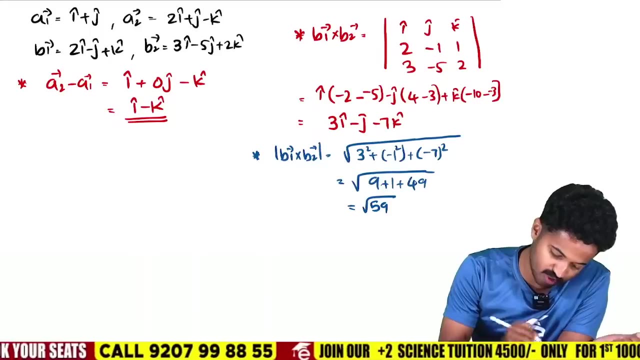 root of 3 square plus minus 1 square plus minus 7 square, That is 9 plus 1 plus 49.. So the answer will be root of 59.. Okay, We got that too, So we are finding everything we need here. 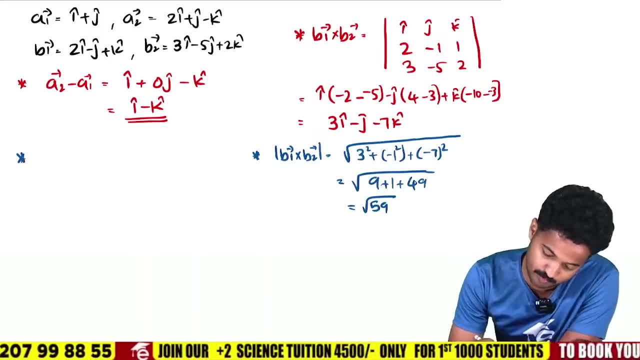 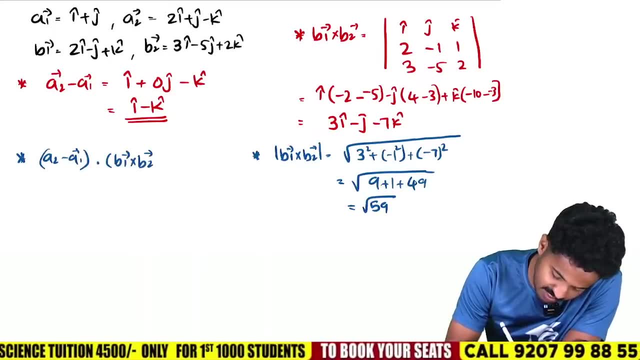 Do we need one more person? The next thing we need is A2 minus A1 dot B1 cross B2.. A2 minus A1 dot B1 cross B2.. All these are what we need. We are finding only what we need. 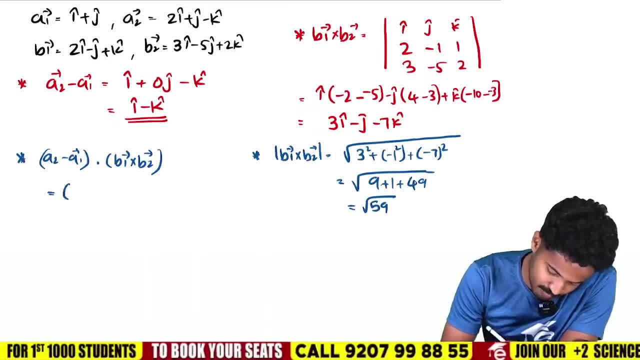 So look, We have A2 minus A1 and B1 cross B2.. So we multiply, The i of this is 1. So there is 3.. So 1 into 3 plus Here there is no one with J. 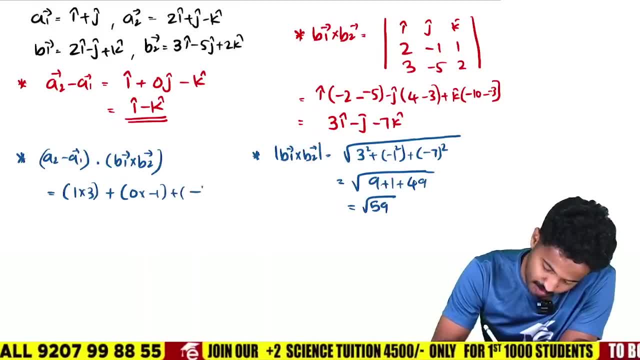 So it is 0.. With J it is minus 1, plus With K it is minus 1.. And A2 minus A1 is this Understand. A2 minus A1 is this, And this is our magnitude: B1 cross B2.. 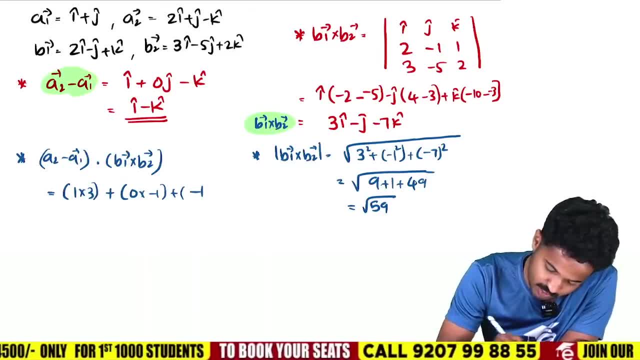 This is what we call B1 cross B2.. So these two are the dot product. So look: With K it is minus 1.. There it is minus 7.. So it is minus 1 into minus 7.. 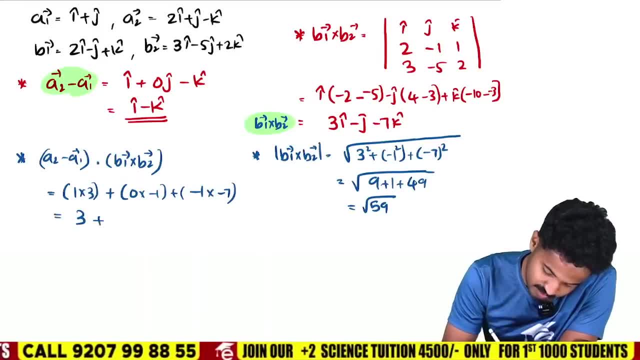 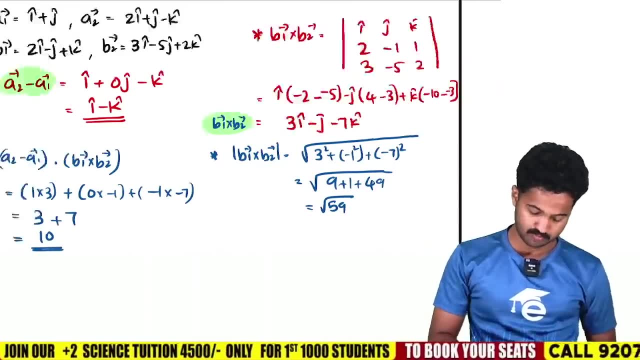 So the answer is: 3 plus 0 into minus 1 is 0.. Minus 1 into minus 7 is 7.. 3 plus 7 is 10.. Okay, So look, This is the answer: Yes. 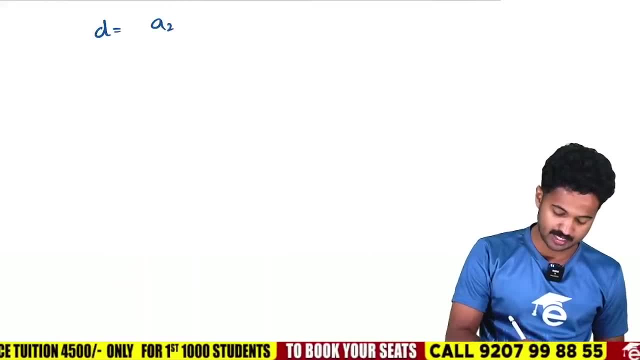 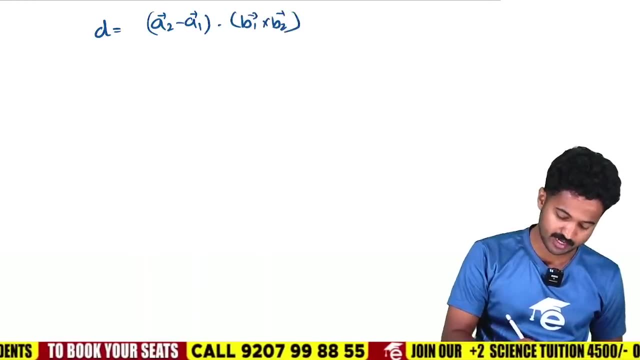 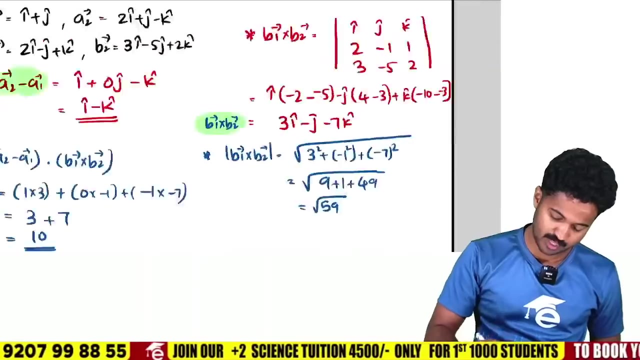 The answer is 10 by root of 59. So the shortest distance D is equal to A2 minus A1.. A2 minus A1 dot B1 cross B2 divided by magnitude of magnitude of B1 cross B2.. You have to put a magnitude in this question. 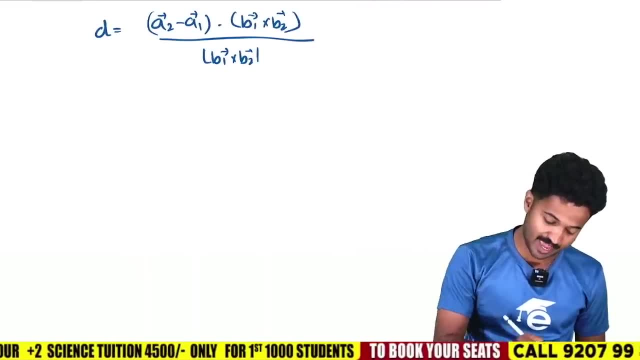 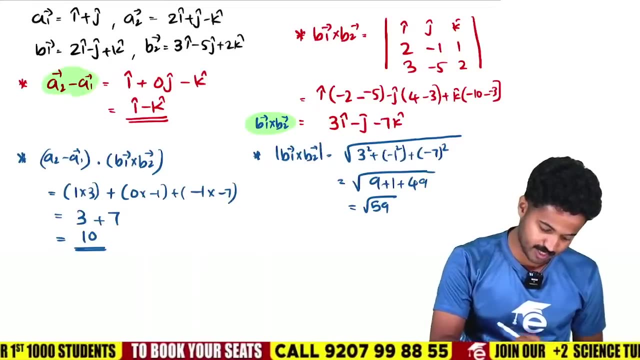 If the answer is negative, then D is equal to A2 minus A1.. We got A2 minus A1 dot B1 cross B2.. Look at the answer: A2 minus A1 dot B1 cross B2.. So you have done cleaning yourself. 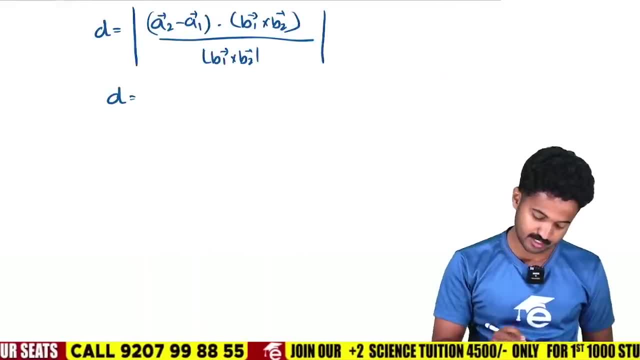 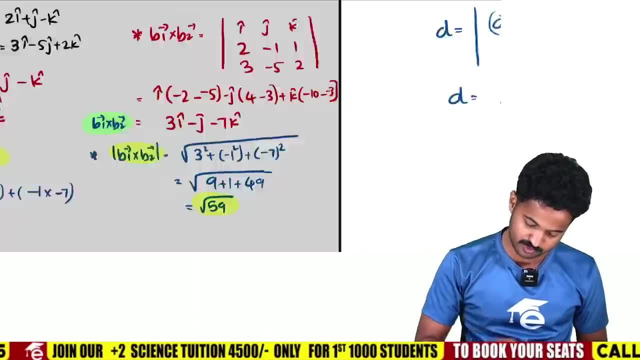 Take a look 10 by Look at the magnitude of B1 cross B2.. Mggt of B1 cross B2 is root of 59. So this is divided by root of 59. This is also in unit. This is in distance. 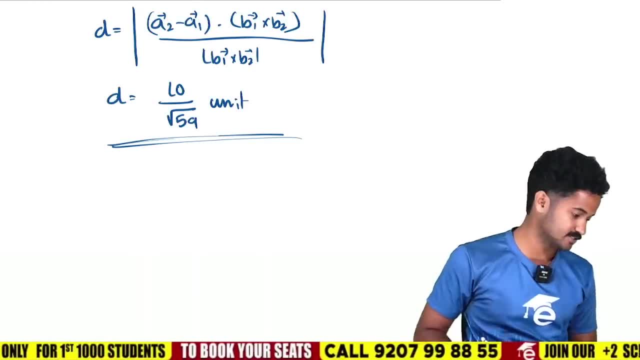 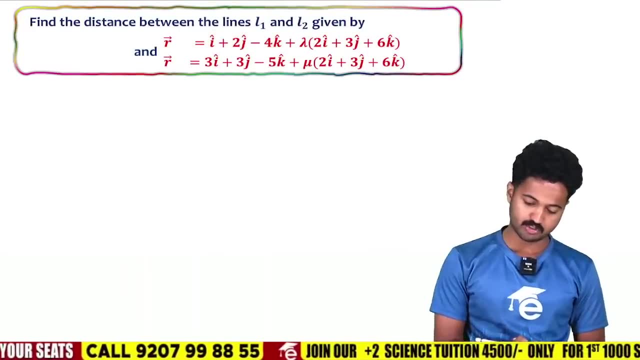 And here this will be a unit. Now this is also in unit, which is the distance. So this is the last question. This is not the last question. we have only one question to ask is left, So we will do this question. 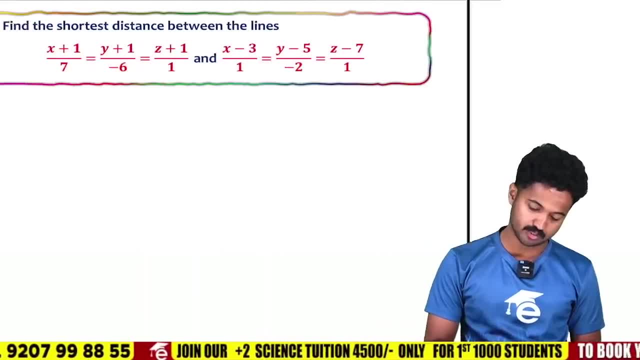 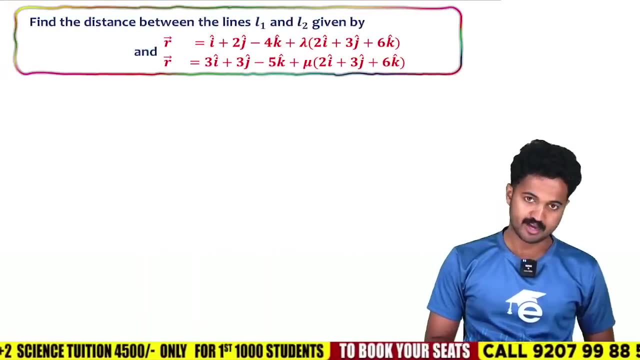 together and this will give you work. If you are done with that, we will stop. The last question is what we are going to do. Is it okay, Ready, Ready, Ready, Ready. Look at this, Sir. what is the difference here? 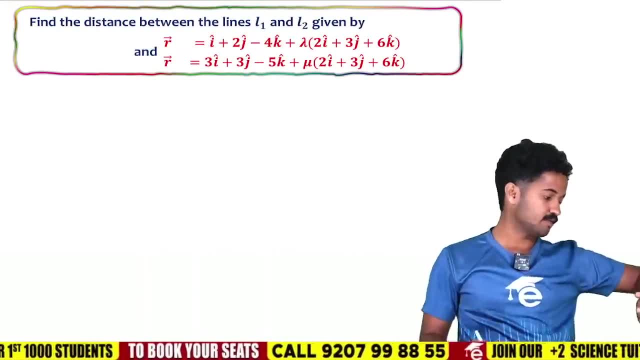 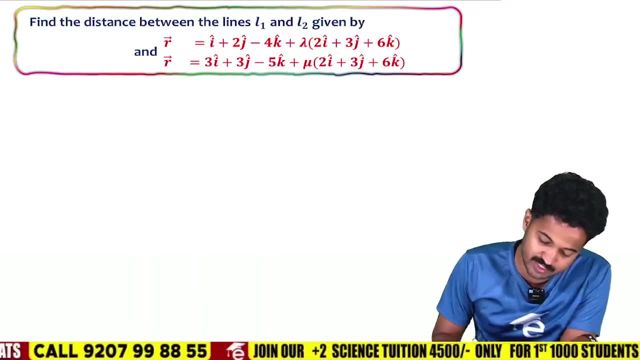 We will do this question alone. It is the last question. The time is almost up. Okay, Ready, Fine, Look at this. We have to pay attention to one thing. Look at this. The vector here is 2i plus 3j plus 6k. 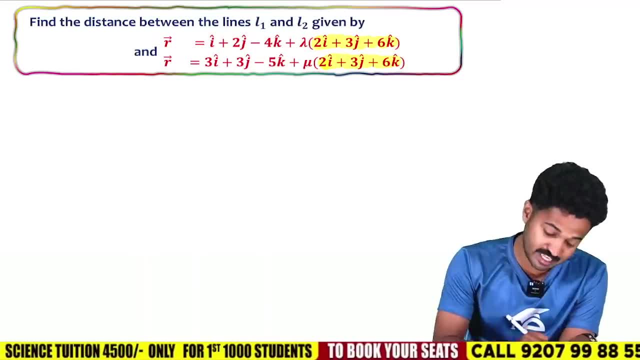 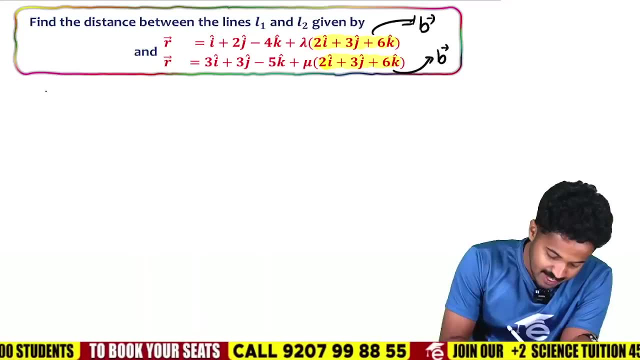 The vector here is 2i plus 3j plus 6k. These two are the same. These two are the same. I gave this as b and this is also b because both are the same, That is, if we find the distance between these two. 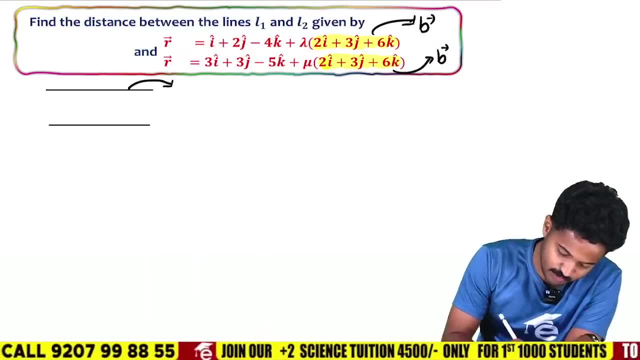 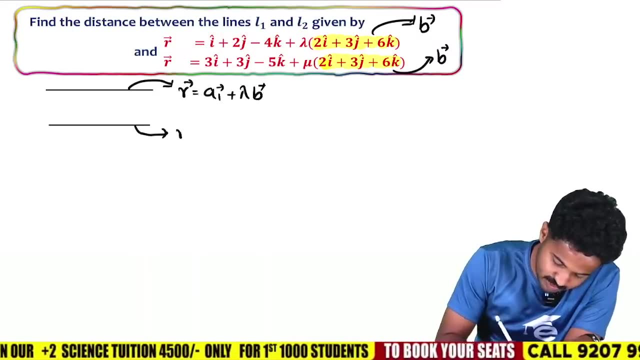 we will change the equation. This line equation r is equal to a1 plus lambda. A is different. Lambda is b. This line equation r is equal to a2 plus lambda. a2 plus lambda is equal to mu. We thought mu is b. 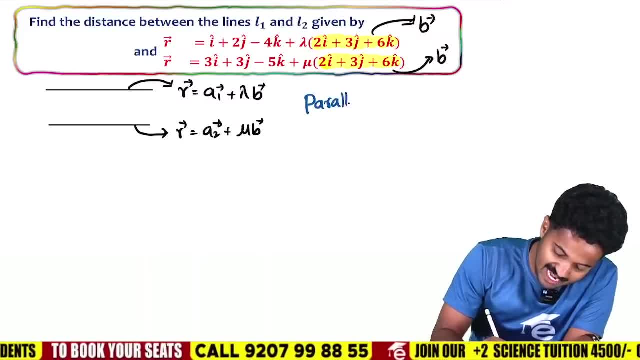 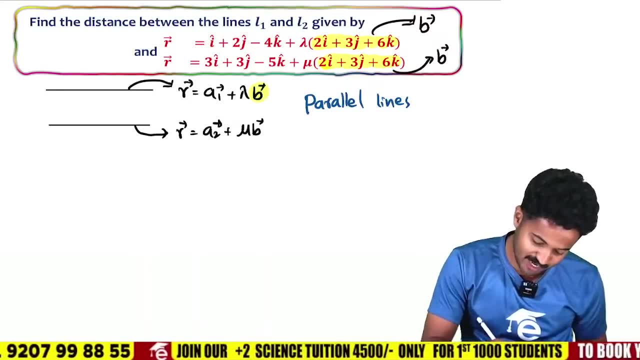 These two lines are parallel lines. How do we understand parallel lines If b vector is the same? if b vector is the same, what will those two lines be? They are parallel lines. They are parallel lines. Earlier they were two lines. 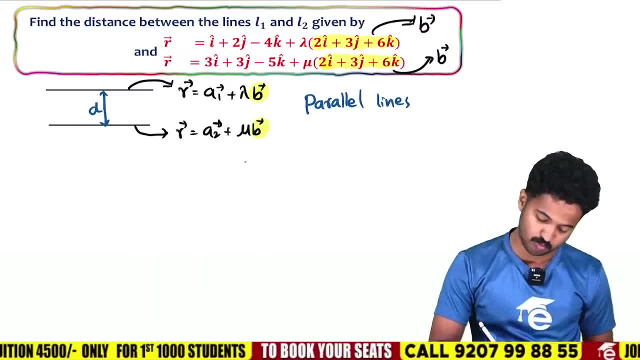 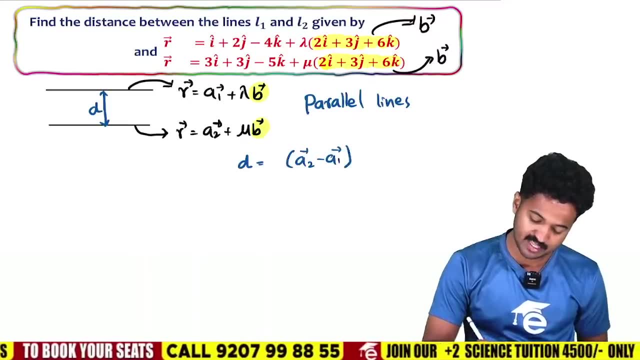 If we define the distance between these two, our equation will change. d is equal to the shortest distance. If we do the same as we did earlier, a2 minus a1 will be equal to a2 minus b2. But a2 minus a1 is equal to. 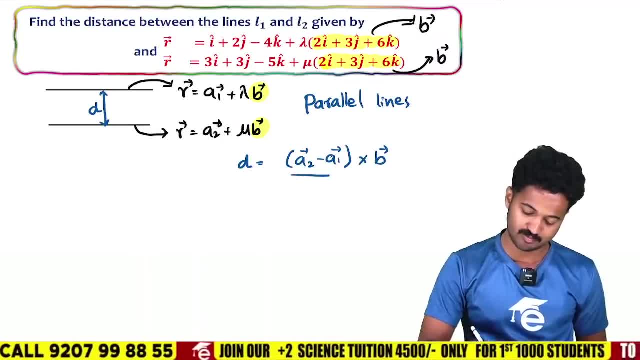 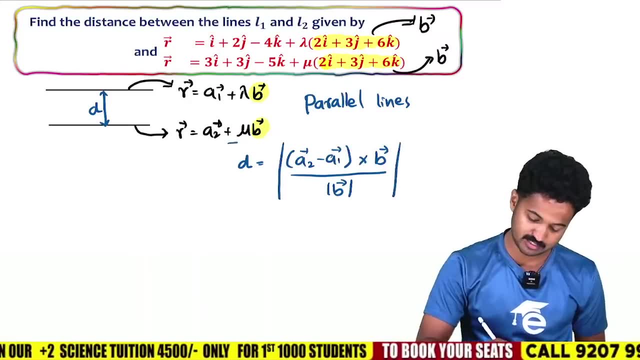 b1 plus b2.. Then if we do dot b1 cross b2, instead of that we will do cross b divided by magnitude b. The answer to this will be the magnitude That is the shortest distance between two parallel lines. 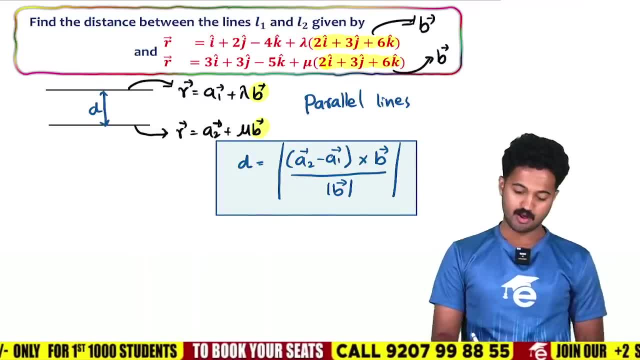 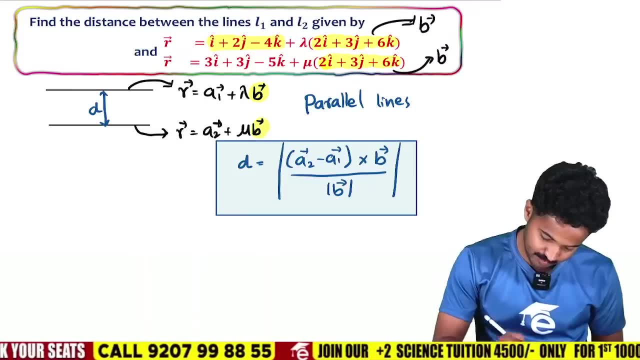 Is it okay? Are you ready? So we have to study this, Is it okay? Then you can see here. here we have got the easy things. what is this? This is our a1.. What is this? 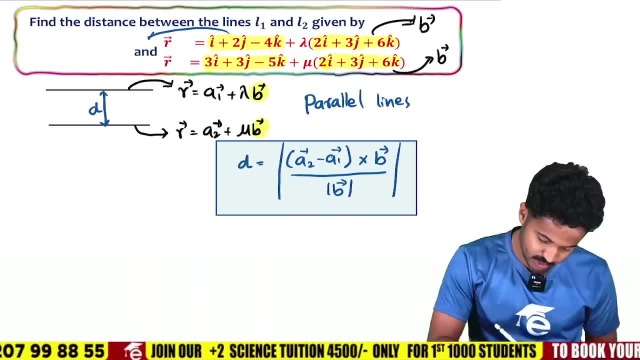 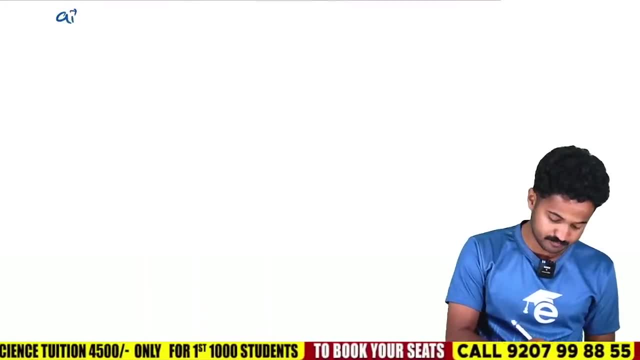 Our a2.. Is it okay? Is it easy? The last question is: This is a1 and this is a2.. Okay, ready. So, after getting both of them, what is a1 and a2?? What is a1 and a2?? 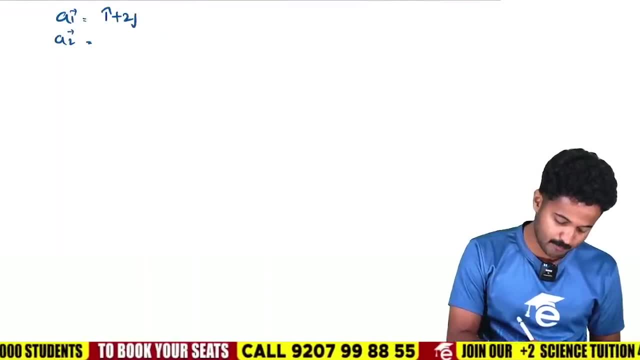 Look: a1 is i plus 2j minus 4k. i plus 2j minus 4k. And what is a2?? a2 is 3i plus 3j minus 4k. 3i plus 3j minus 4k is 5k. right. 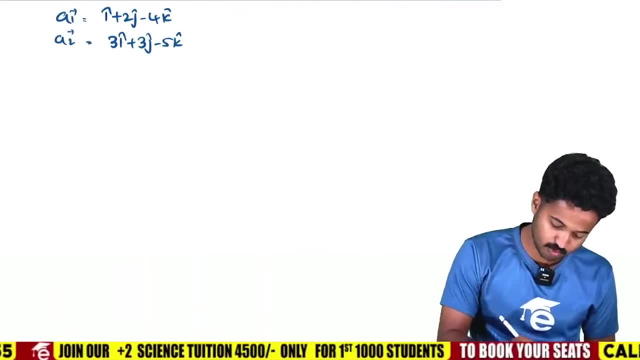 Yes, And b 2,, 3,, 6, right. Look at the vector b 2,, 3,, 6.. 2i plus 3j plus 6k- Ready Now? look at that. 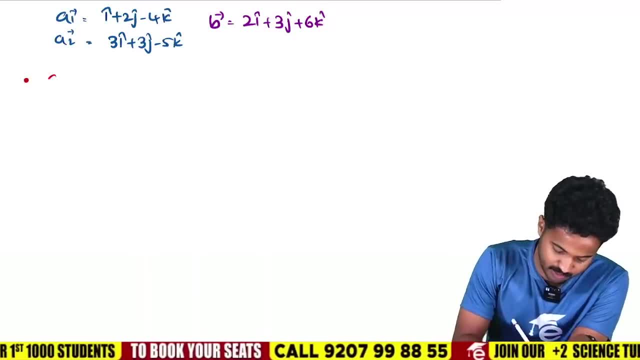 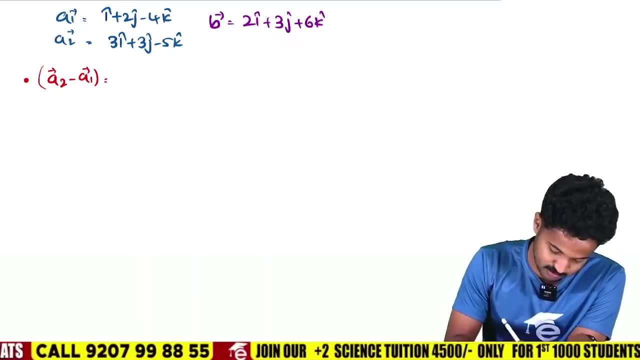 First we have to find a2 minus a1.. We have to find all of them. First let's find a2 minus a1.. What is a2 minus a1?? Look at that. a2 is a1.. 3 minus 1 is 2i. 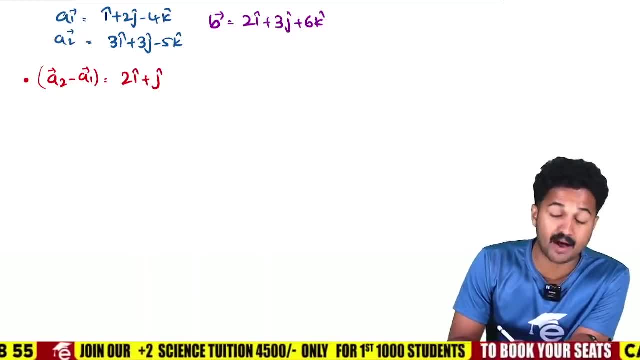 3 minus 2 is 1.. So 1 into j. Minus 5 minus minus 4.. Minus 5 plus 4 is minus 5 plus 4.. So minus 1 minus 1 into k minus k. 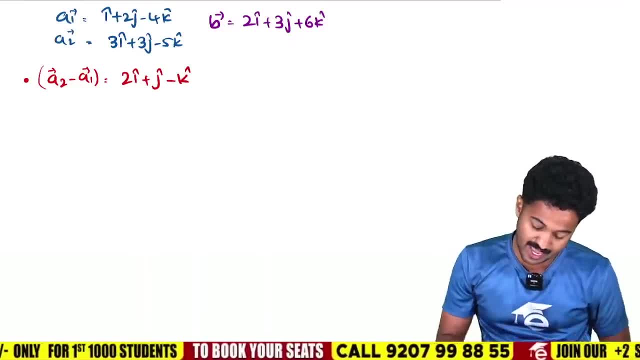 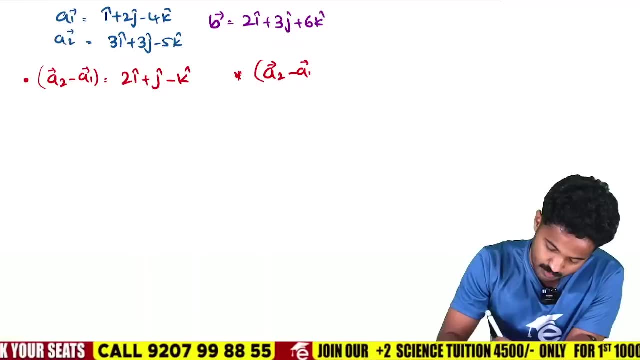 So look at that. So we get that too Easy, No problems. Now look at that: a2 minus a1 cross b. That is what we have to find next. Look at that: a2 minus a1 cross b. 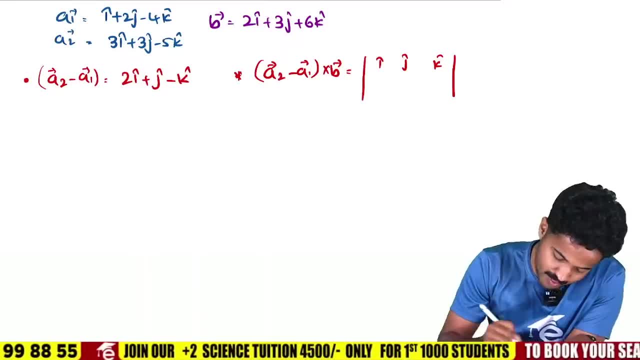 That is ijk Now the component of a2 minus a1 is 2, 1, minus 1.. 2, 1, minus 1.. Now b, b is 2, 3, 6.. 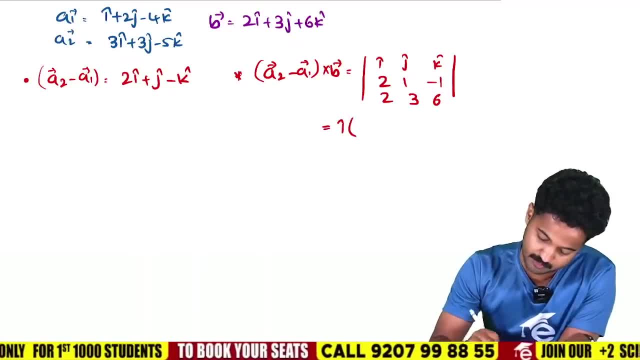 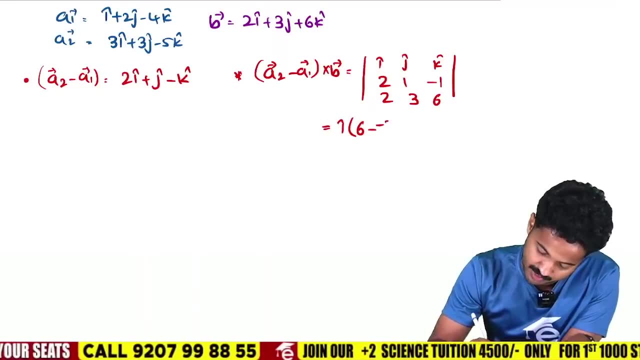 2, 3, 6.. If so, the determinant is: i Look at that Row cancel column cancel Row cancel column cancel 1 into 6 is 6.. Minus 6 minus 3 into minus 1 is minus 3.. 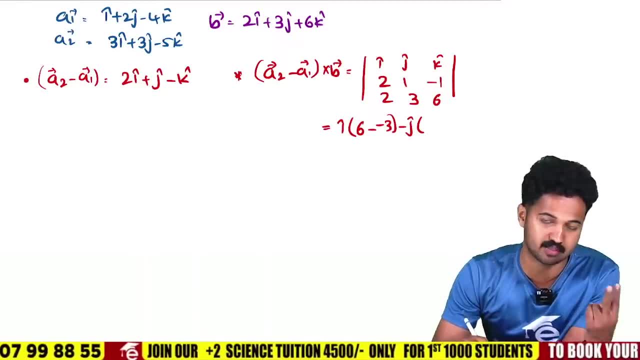 Minus j, j is minus. Look at that Before that. in the second one, the determinant is always minus, isn't it? Row cancel, column cancel. So if we cancel row and column, we get 6 into 2, 12.. 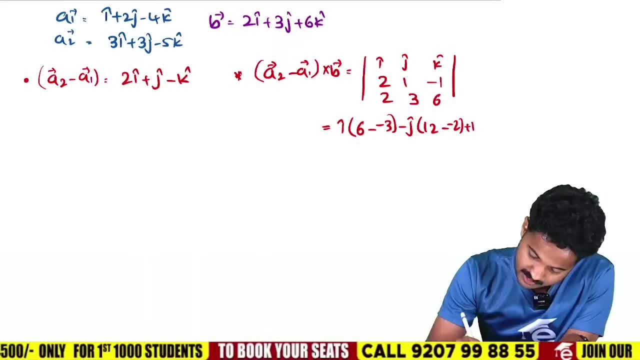 Minus. If it is minus 1 into 2, we get minus 2.. Plus k into k into Row: cancel colon. cancel 3 into 2, 6. 6 minus 1 into 2, 2.. 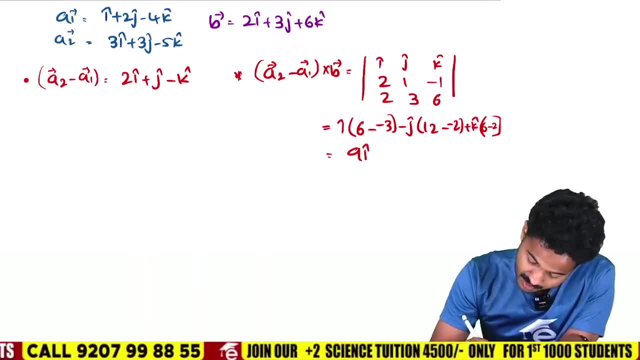 That's it. So 6 plus 3, 9i Minus 12 plus 2 is 14.. So it is minus. Before that it is minus. so it is minus 14j. 6 minus 2 is 4.. 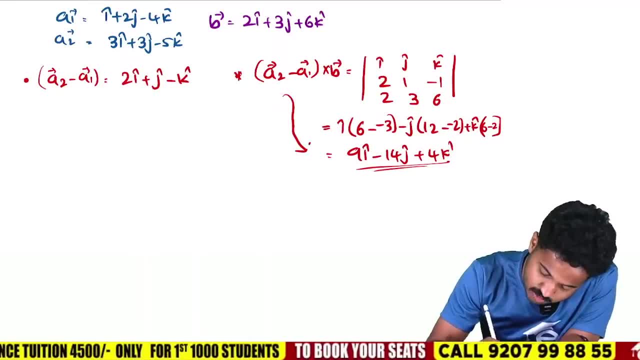 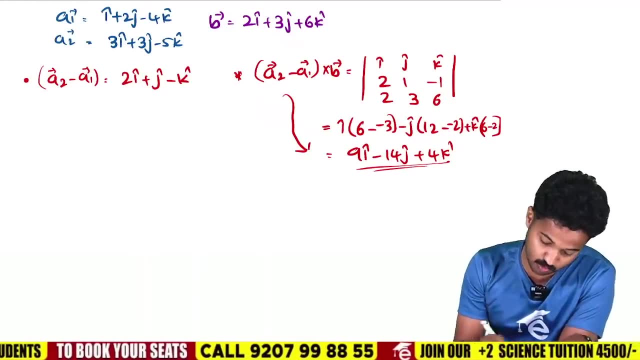 So 4k is the answer Ready. So what you get now it is a2 minus a1 dot. Sorry, a2 minus a1 cross b, Easy, No problem. Now what else do we need? Let's see. 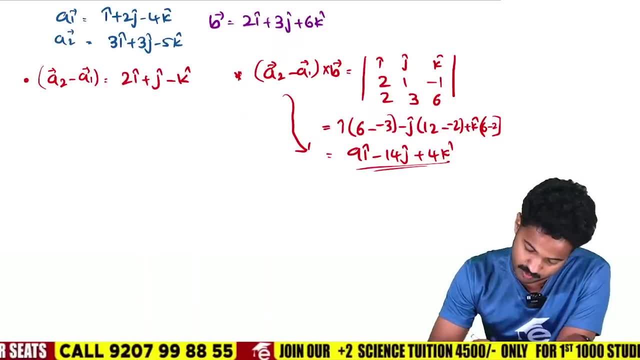 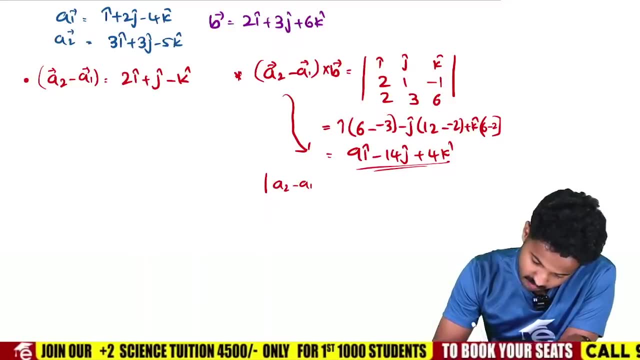 When you find the distance. do you need the magnitude of this? Do you need the magnitude of this? So, if you want to find the magnitude of this, let's find the magnitude of this: a2 minus a1.. And do you need the magnitude of this? 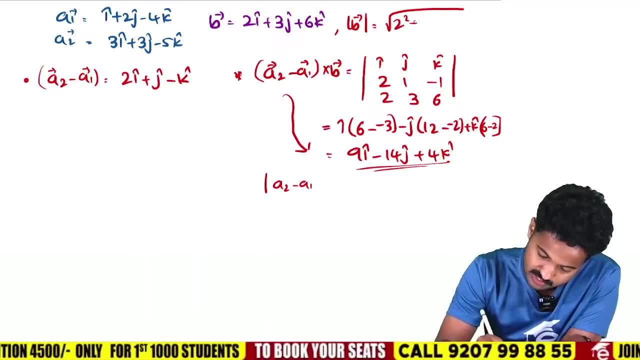 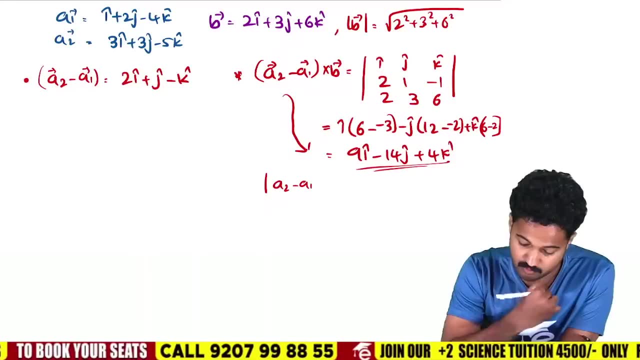 Do you need the magnitude of b? Let's find it: 2 square plus 3 square plus 6 square, That is, if you add all these, you get 2 square 4, 3 square 9, 6 square 14n. 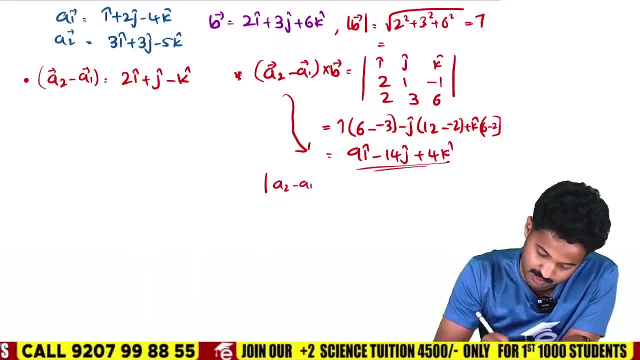 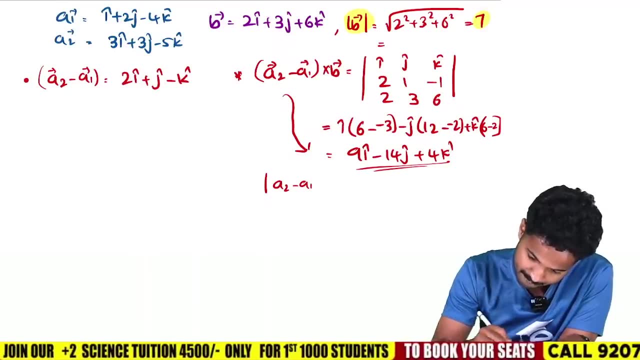 If you do this, you will get 7.. If you say magnitude b, you will get 7.. Okay ready. So if we find this too, we will get the distance a2 minus a1.. Where, Where? 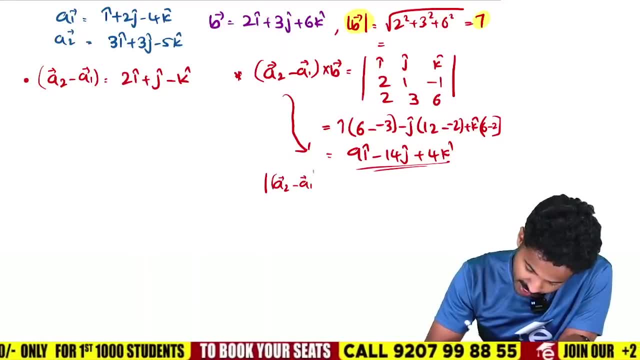 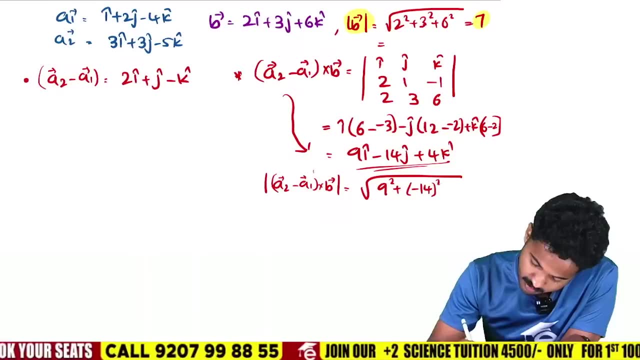 Yes, So a2 minus a1.. We have this in our hand And cross b The magnitude of this. That is root of this answer. 9 square plus minus 14 square plus 4 square Easy, 9 square is 81.. 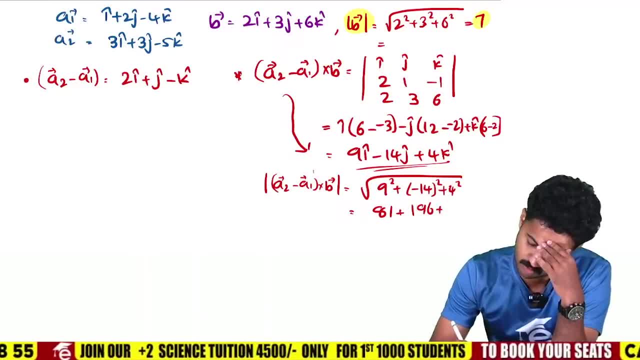 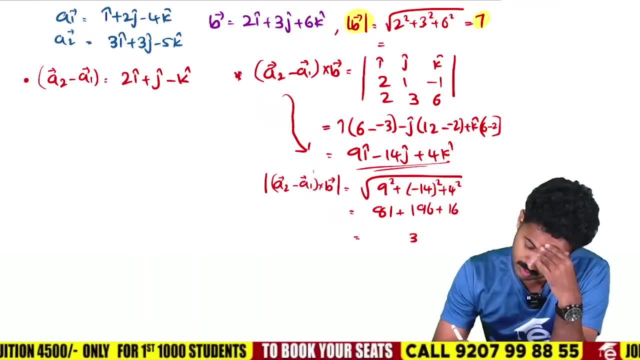 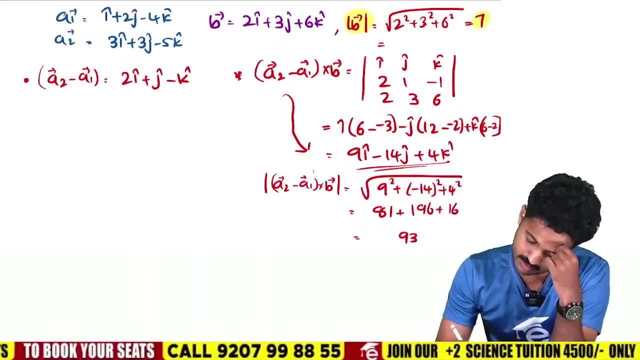 Guess the answer: 6, 6,, 12,, 13,, 3.. Tomorrow 12ruk, 11s, 9,, 10,, 11,, 8,, 9 and 12.. 2 make 2.. 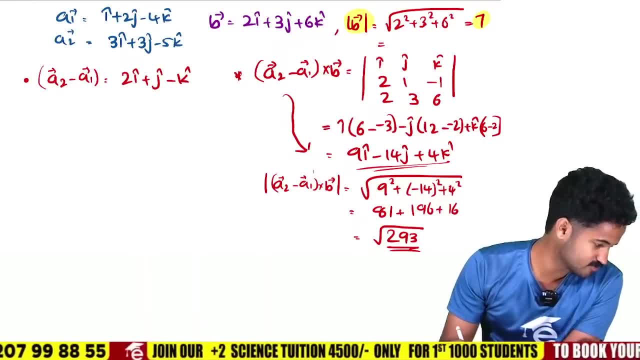 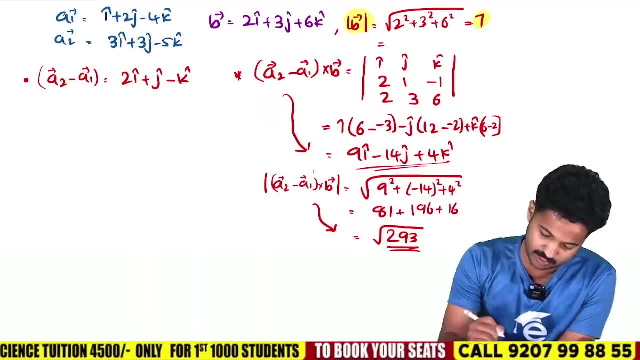 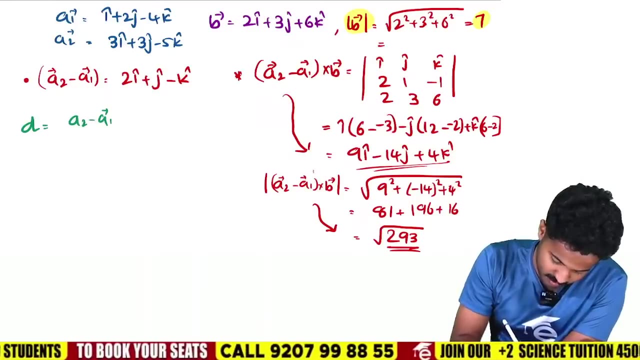 I'll say 293.. Thanks for answering my question. Oh, I just now guess a 192.. Affistry is Okay, sir, And that's good If it is. look. Shortest distance. Shortest distance. D equal to A2 minus A1.. A2 minus A1 cross B. 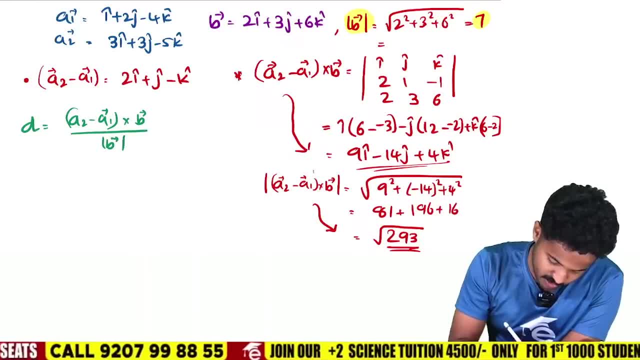 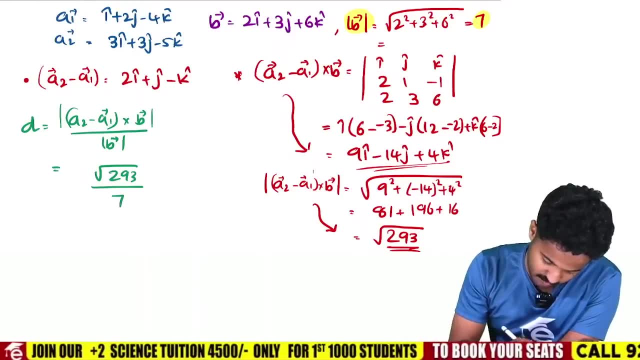 A2 minus A1 cross B by magnitude B. So there is a magnitude for this. We are giving magnitude to the whole thing. So the answer for that is: root 293 divided by magnitude B is 7.. So this is the answer for that. 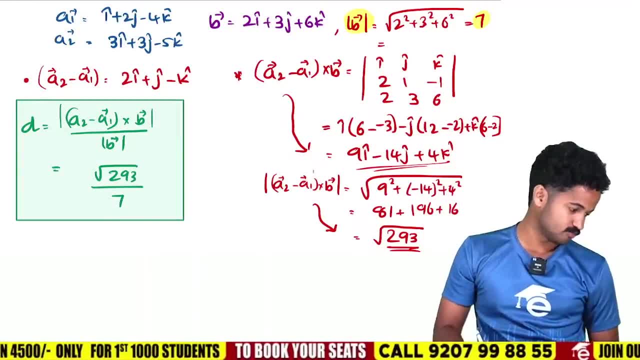 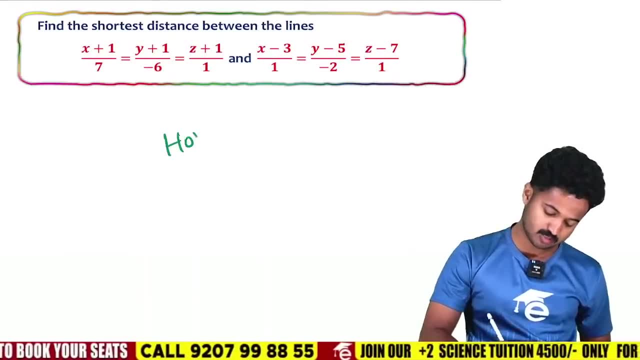 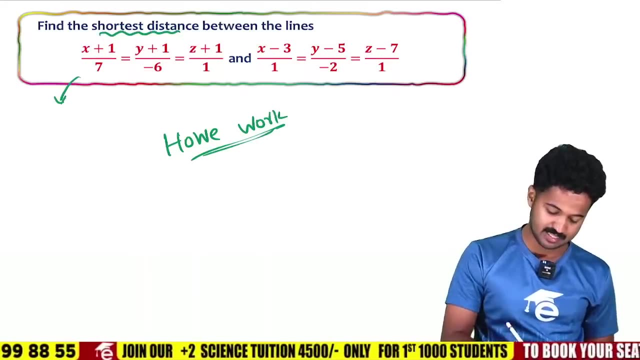 It is easy, It is simple, There is no problem. So this is it Done. Got it? So this is it. So try to understand the things we have done, And this question is homework for you. This question is homework for you: Find the shortest distance. I asked. So, from this, what do you do? 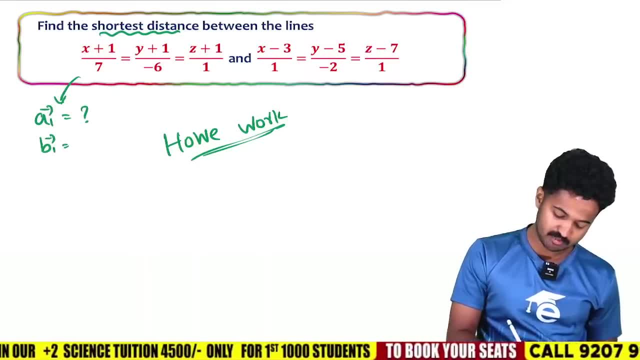 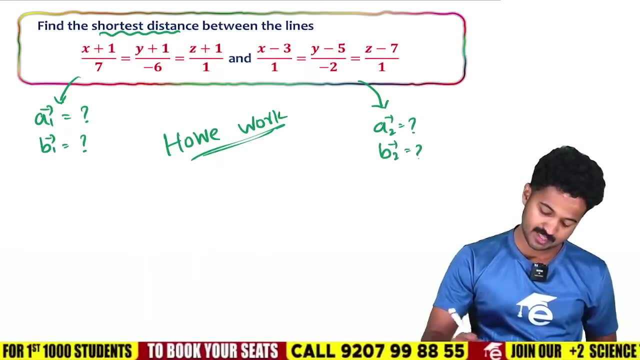 Find out what is A1 and what is B1. I am not telling you, You know. And from this question, find out what is A2 and what is B2 also. And then our D, equal to shortest distance, is not parallel lines. If it is parallel lines, it will be the same. 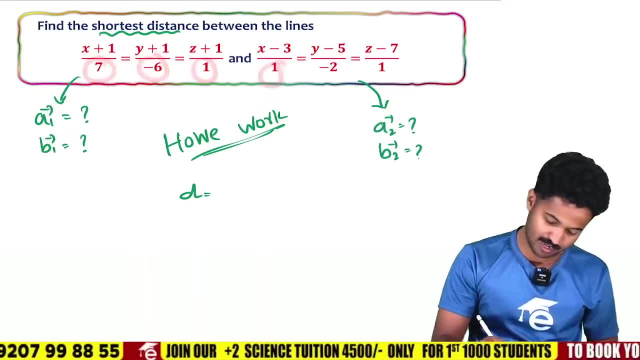 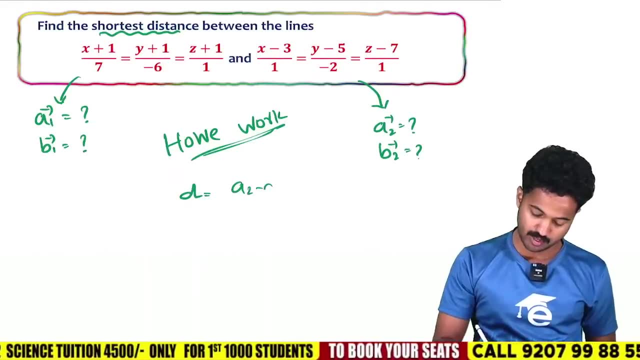 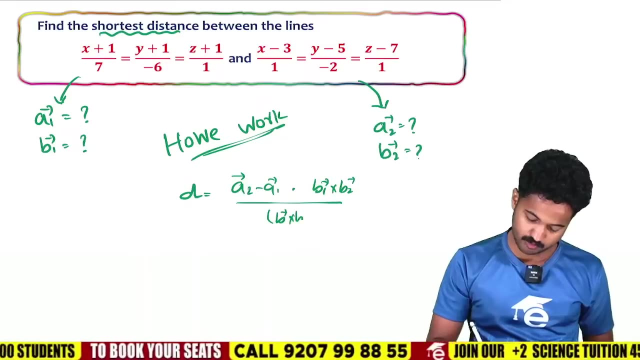 We are done. We are done, This will be the same. So, since this is not the same, it is not parallel. Okay, That is it, And if so, you have to define the homework. You know the equation: A2 minus A1 dot. B1 cross B2 divided by magnitude of B1 cross B2.. 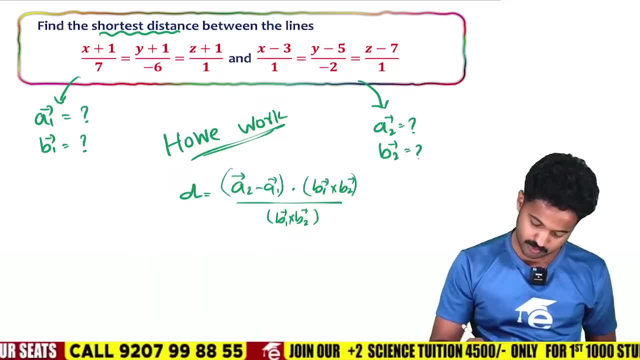 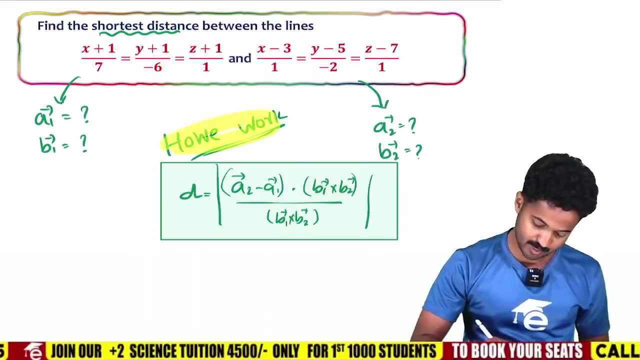 So this is it: A2 minus A1 dot. B1 cross B2 by magnitude of B1 cross B2.. So what do you do with this? Find the distance. This is a homework question for you, So do it, Do it? 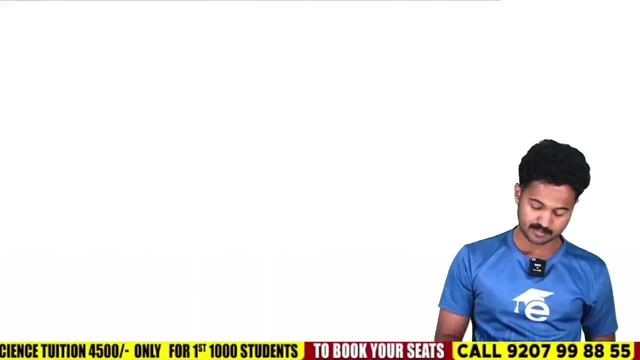 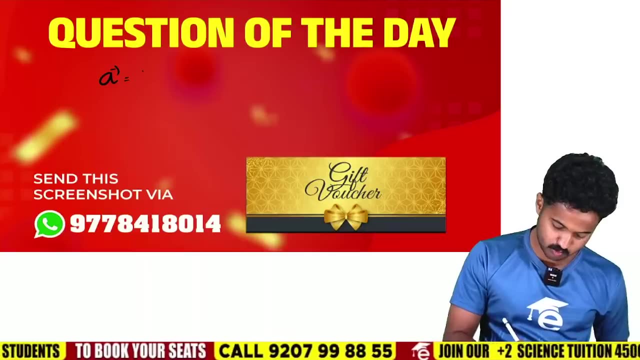 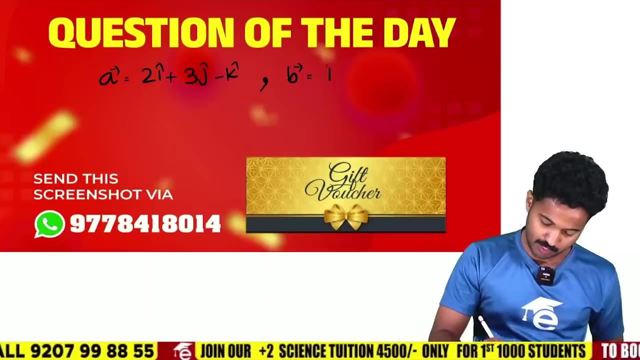 It is a must. Okay, Ready. Thank you, sir, Chapter set. Okay, That is it. It is simple Question of the day. Do you have a question? Answer this question. A equal to 2I plus 3J minus K. B equal to I minus 2K plus 5.. I minus 2K is enough. 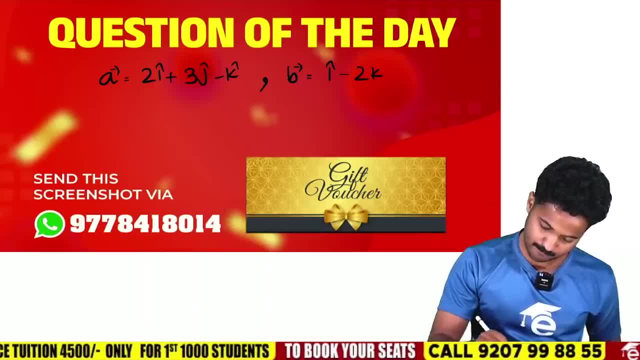